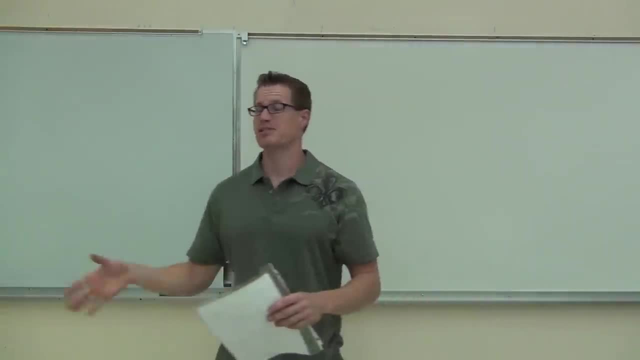 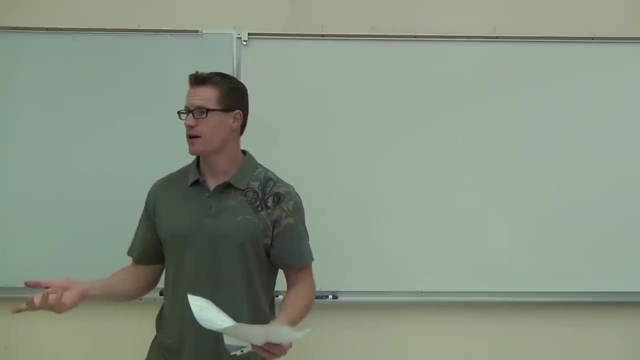 So today we are going to talk about something called rational exponents. Now, when we say the word rational, what does rational actually mean? We've dealt with rational functions, right? Say that again: A fraction or something. Yeah, that's actually exactly what it means. It means a fraction. 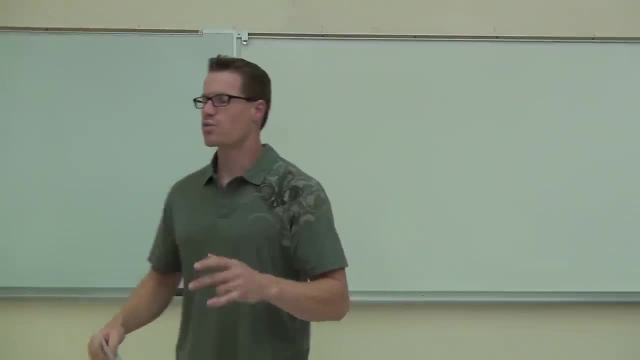 So rational means ratio or a fraction. So when we're dealing with rational exponents, this is going to seem kind of weird to you, but we're going to deal with exponents that are actually fractions. Isn't that kind of strange that we can have exponents that are fractions? Right now you've dealt with squares or cubes, or fourth powers. 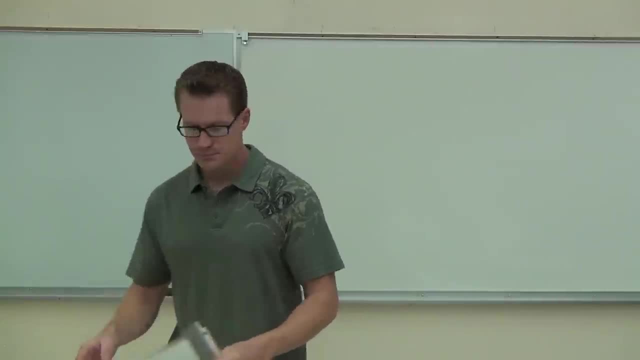 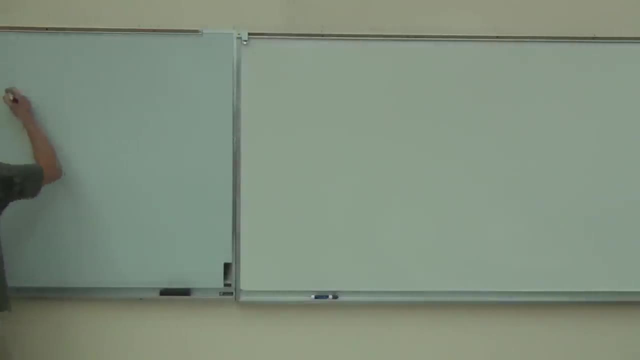 You've never actually dealt with a fractional exponent before. That's what we're going to talk about today. So rational exponents. Now, the interesting thing is that I just said you've never seen a rational exponent before, which is actually a lie. 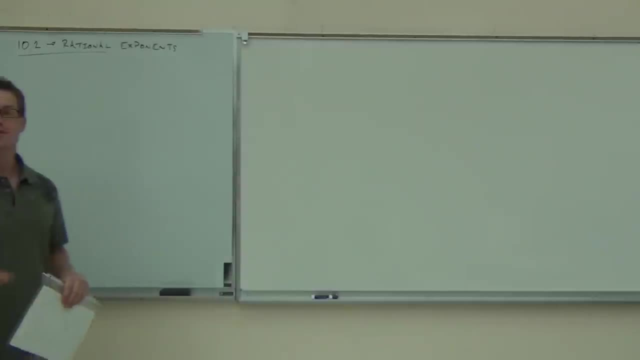 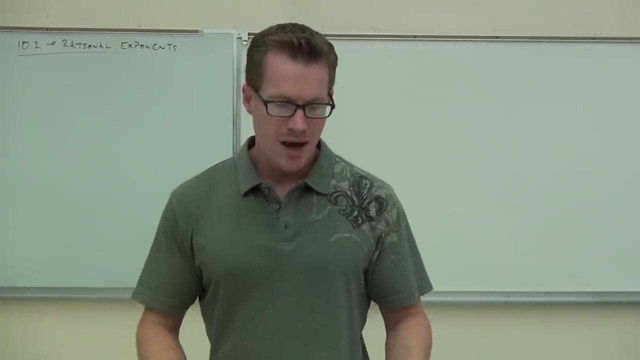 You have seen a rational exponent before. It's just that we haven't dealt with them as an exponent. Here's the whole deal about section 10.2 and why it's in this section. that has all to do with radicals. Every single time that you've seen a root, a square root or a cube root or a fourth root, actually you've been dealing. 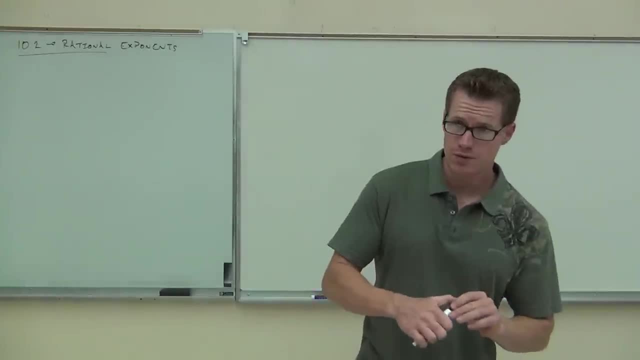 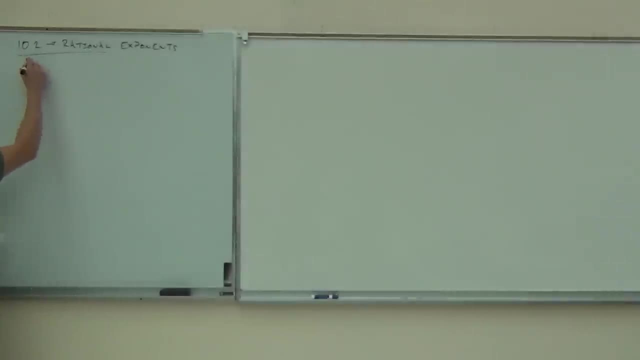 With a rational exponent. As a matter of fact, any root that we've ever seen can be represented as a rational exponent. I'm going to show you how right now. So write this down: Any root can be represented as a rational. That means fraction. 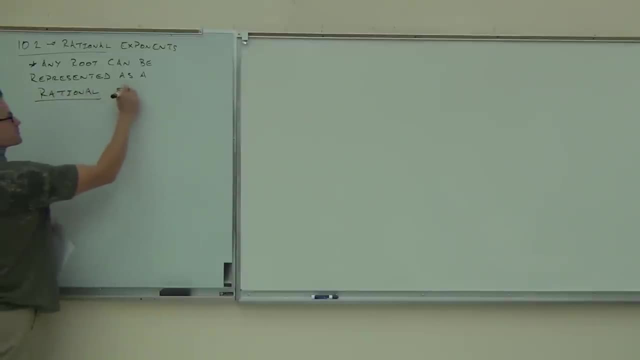 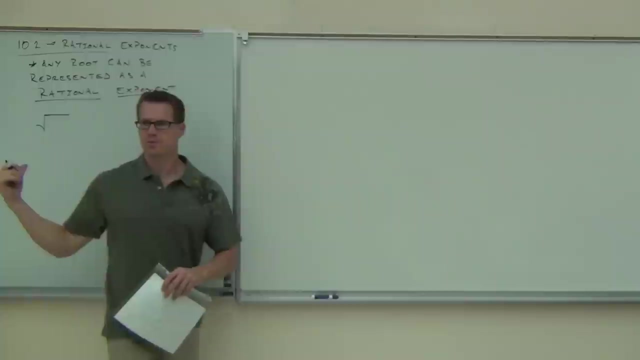 Rational exponent. Here's how You remember we were talking about those nth roots, How we had like a radical like this, And then we had some sort of root up front. Now, what would that type of root be if I just left it like that? 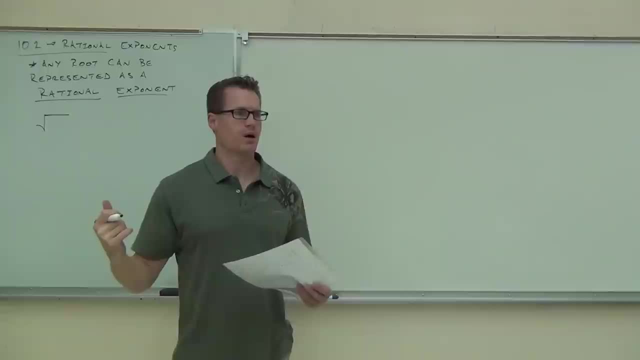 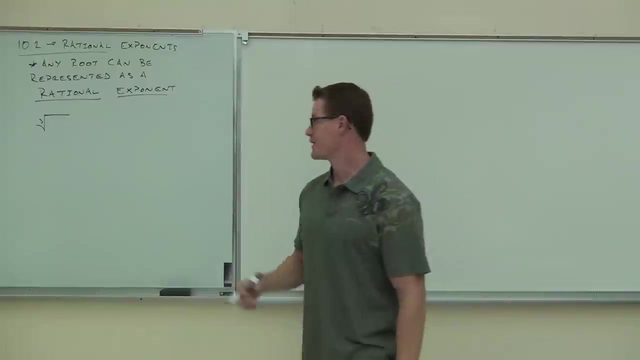 Square root. And if I had a cube root, what number would I put and where would I put it? Three Right, A little like indices, part A little crotch of this thing. Right, Right there, That little thing. That's where I put a cube root. 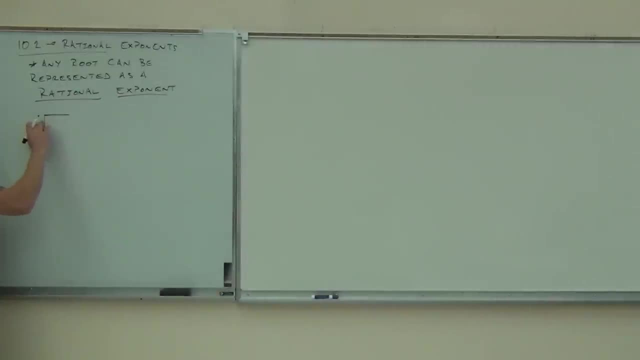 If I had a fourth root, I'd put a number four there, Or an nth root. for any root, I'd put a little n there And whatever's on the inside, we're going to represent that with an- a, So our radicand in this case is just a. 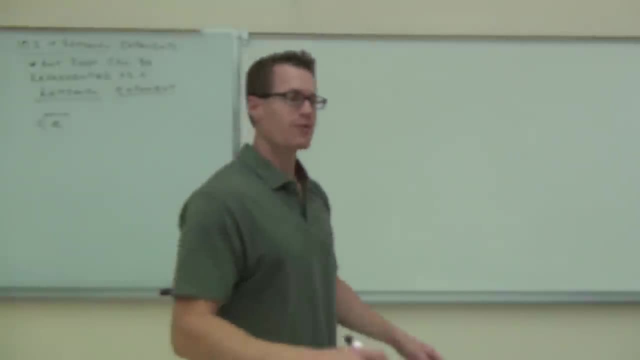 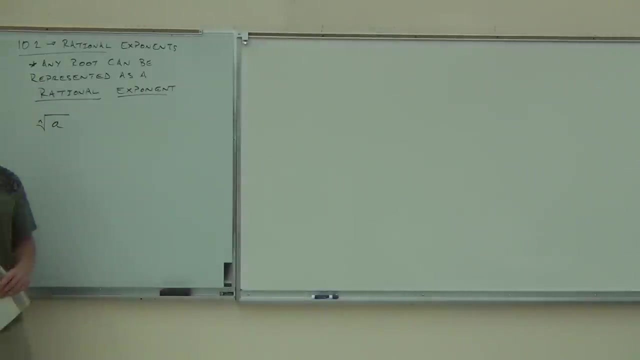 It could be anything. It could be x squared plus three. It could be whatever I want it to be. Here's the deal. This is kind of neat. Every single time you've seen something like this, this actually represents A fractional exponent. 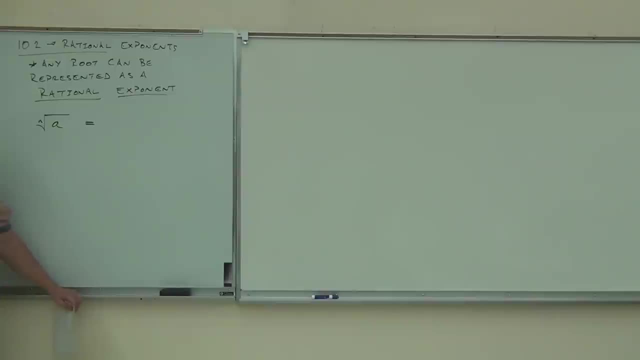 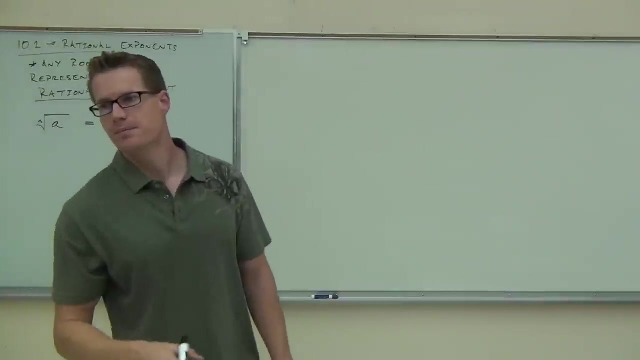 And here's how you write it You have in this case, our base is a. It's whatever our radicand is. An nth root of a is the same thing as a to the one over n power. That's how you change from a root into a fractional exponent. 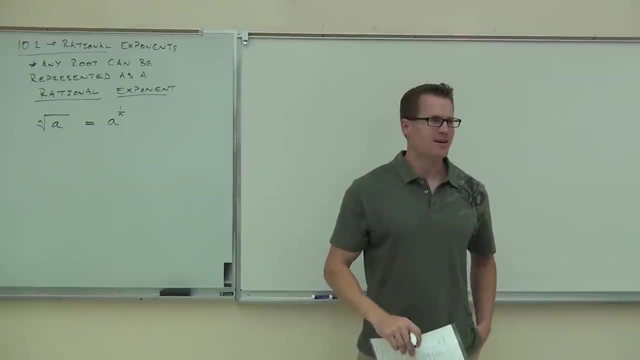 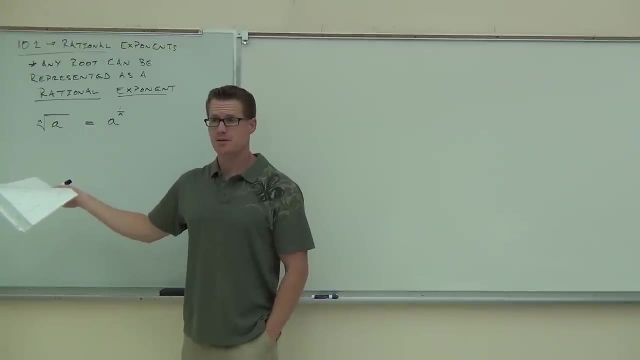 Weird huh. Why are we doing that? Why are we making these look like those? Well, I'll tell you. what Do you know? why Do you know anything about exponents? If you multiply common bases, you add exponents, right. 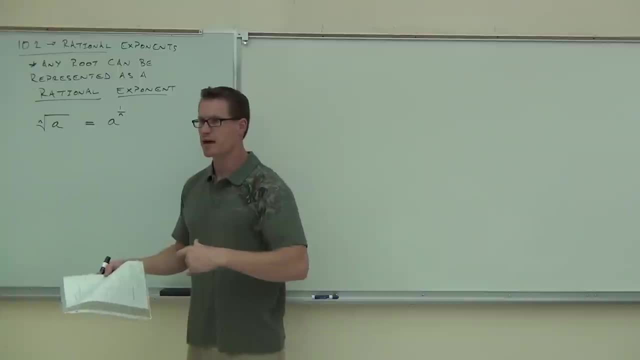 And if you have an exponent to an exponent, you multiply, And if you divide, you subtract. We can do all that stuff with our roots. now We couldn't do that here, It wouldn't make any sense to do that, But as soon as we translate to a fractional or rational exponent, 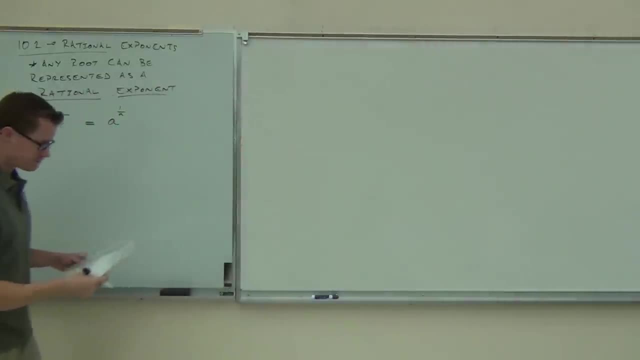 we can do all those things that you already learned. That's why we're translating these. Let's see if we can manage to change some of these from this form back into our roots. Are you guys ready to try some of this? Let's do this. 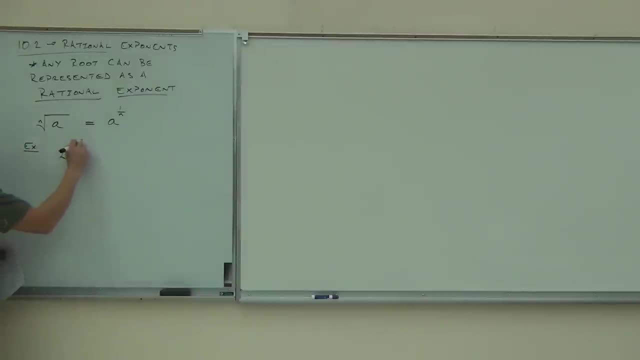 So first one, let's say that we had 25 to the 1 half power, 25 to the 1 half power. You can notice a couple things about this. Firstly, where does our n go in our fractional exponent? Where does it go? 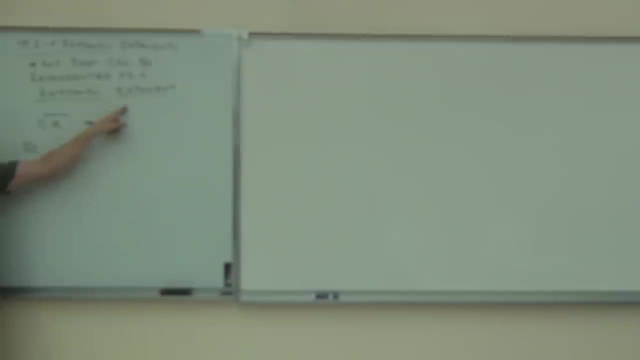 Numerator or denominator, Denominator, And where does that 1 come from? I'll show you this right now. I'm not supposed to until later, but I'm going to give you a sneak peek, okay, Where this 1 comes from. 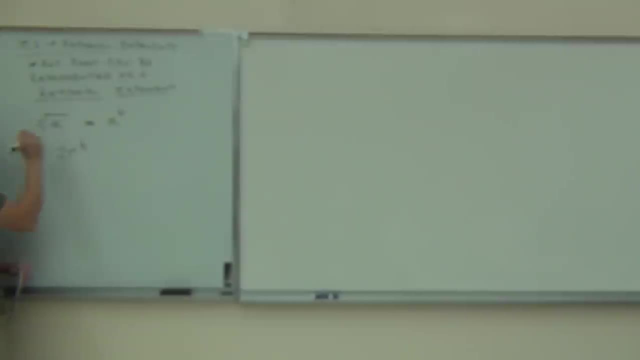 What's the power of a right here? 1. That's where the 1 comes from. So this is a little preview of where that number comes from Right now. this is just a to the first power. That's why we have a little 1 right there. 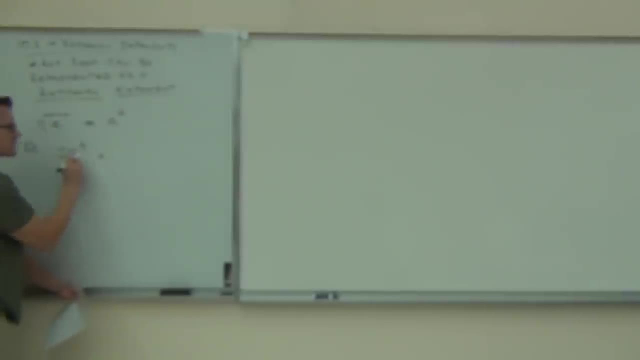 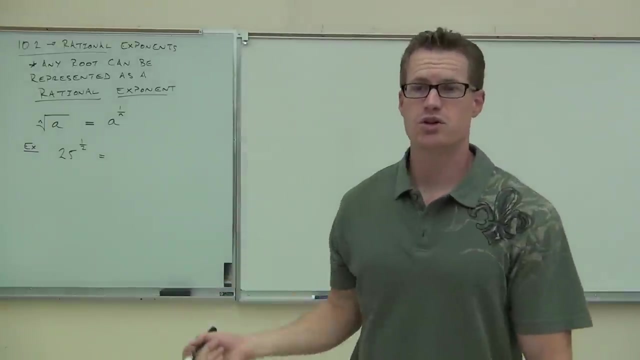 You guys okay with that. Okay, good. So question: can I represent 25 to the 1 half as a type of root? Firstly, you guys tell me what type of root is it? Is it a square root, a cube root, a fourth root? 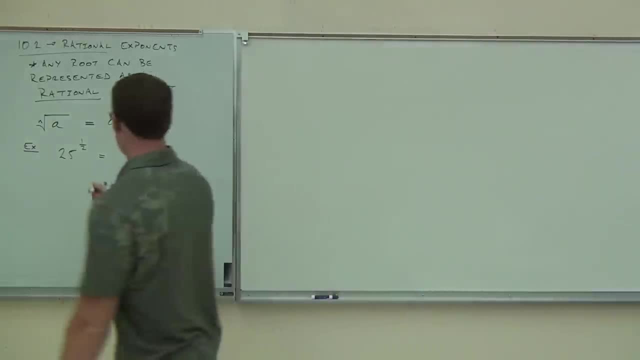 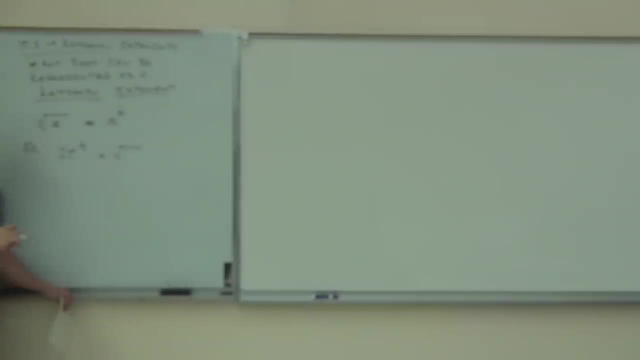 What is it? Square root? What tells you that It's a 2.. Yeah, that denominator right there tells you the type of root that you have. So if you have a 2 on the denominator, that means you're dealing with a square root. 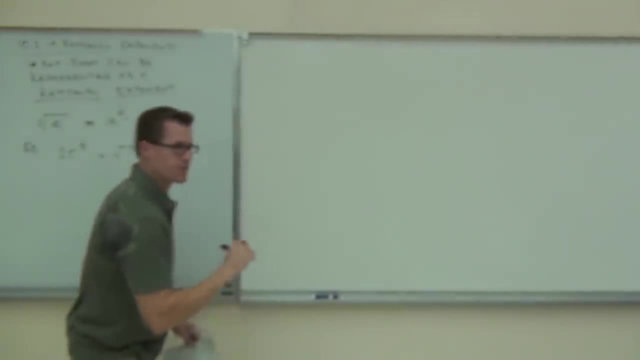 What's going to go on the inside of our square root 25.. 25 to what power? First, Yeah, the first power, because that number right there is a 1.. How many of you feel all right with this? What is 25 to the 1 half power? 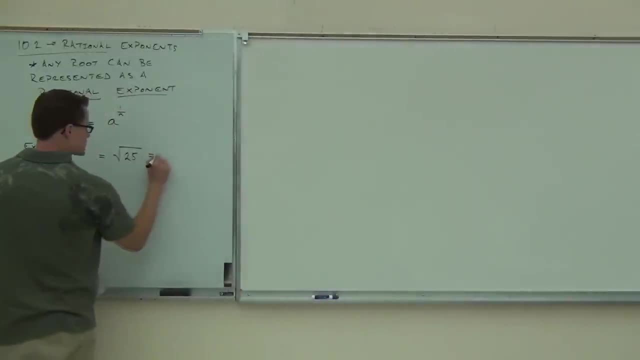 Or in other words, what's the square root of 25? 5.. Which means that you don't have to change it to this to find that number. In fact, if you have a calculator, you want to plug in 25 to the 1 half power. 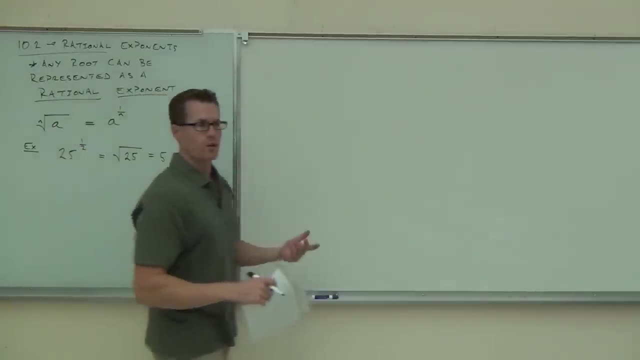 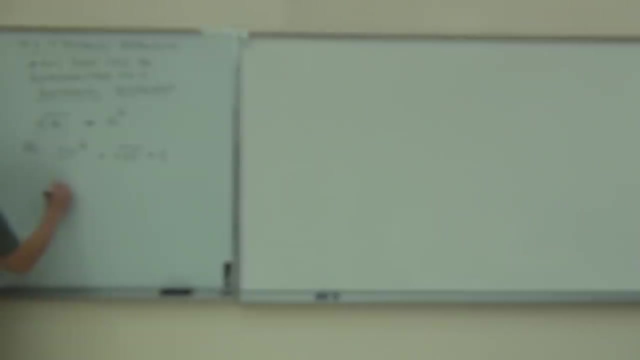 it will give you 5, because it means the same thing: 25 to the 1 half and the square root of 25 are identical. Let's try a few more. Let's try 27 to the 1 third. Can you tell me, ladies and gentlemen, what type of root does this suggest? 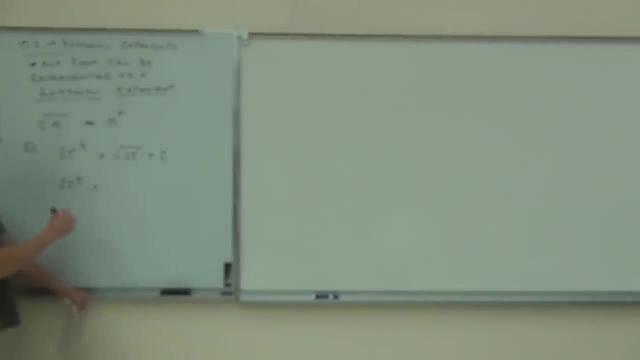 Q. Good, What tells you the Q, The denominator? Okay, So we are going to have a radical. We know that any rational exponent is the same thing as a radical. We just have to make sure that our root is the same. 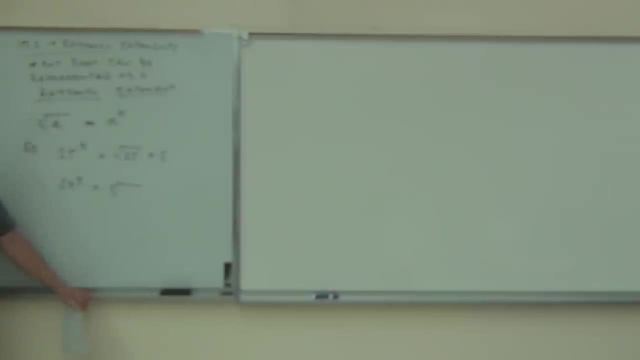 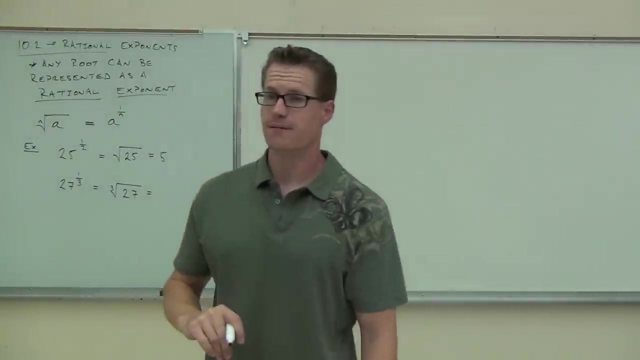 Here is square root. Here we can't forget the 3. That's a cube root. On the inside. we will have 27.. And can you tell me what is the cube root of 27?? What do you think? 3.: 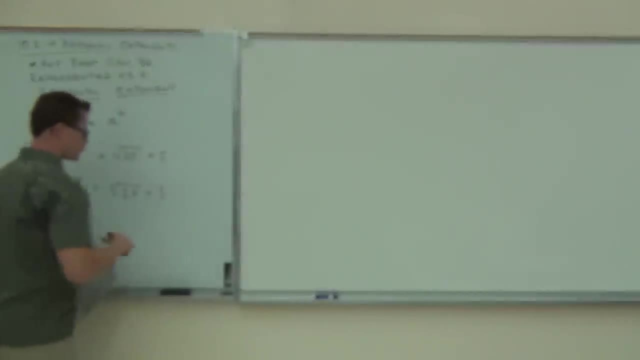 Yeah, because 3 times 3 times 3 equals 27.. We've dealt with these roots before. We're just now translating from here to here- By the way, you're going to get pretty good at this- to where you're going to be able to look at these things. 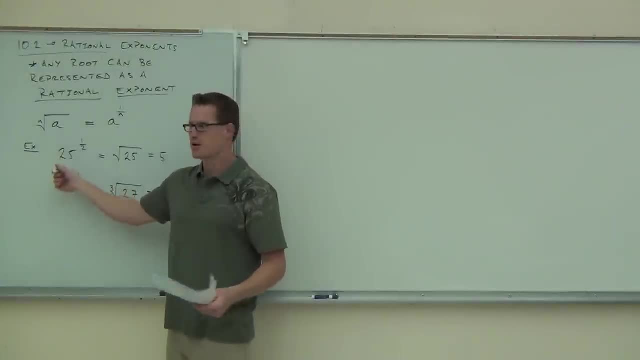 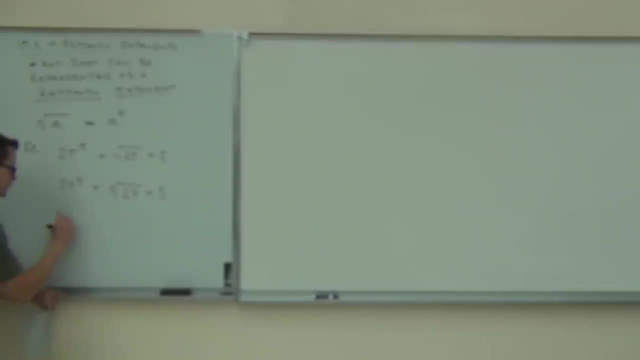 and know immediately: oh, that's 5.. That's the square root of 25.. That's 3.. That's the cube root of 3.. So you'll get pretty good at that. Can you do it with just a variable, without some numbers? 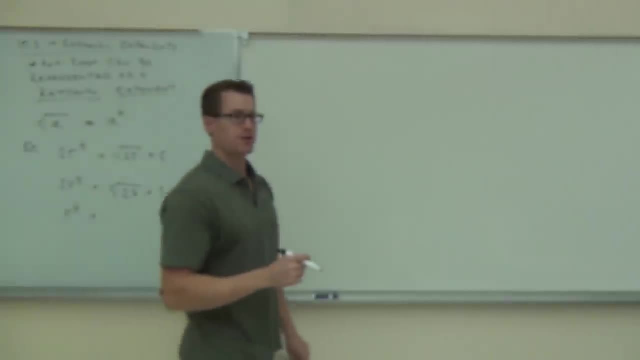 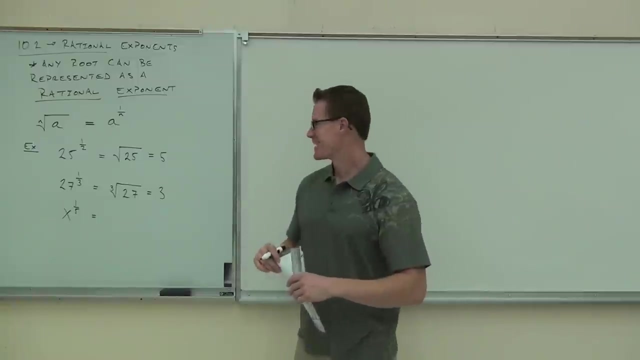 Let's see if we can translate that. Ladies and gentlemen, what type of root am I dealing with? What type Fifth root? Yeah, Flipped around in your head, didn't it? Yeah, we've got a fifth root here. 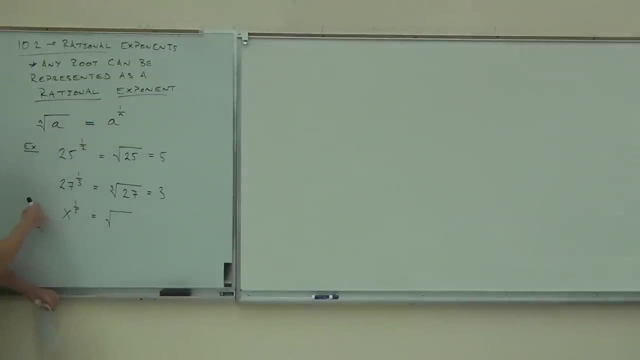 That's all right. So we'll still have a radical. The denominator simply tells you what type of root you have. What's going to go on the inside of our root- X, X- to what power First? So you're going to leave it just like that. 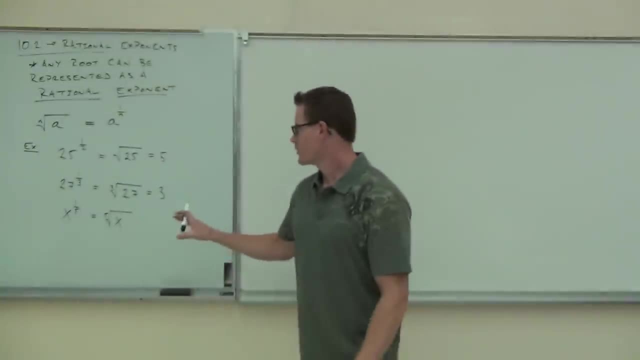 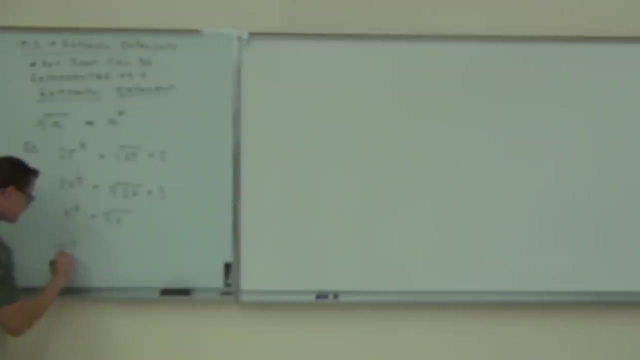 That's the fifth root of X. There's no way we can simplify that right now. There's no number, so we can't say like here was a 5,, here was a 3. We can't do that. Let's try a couple more. 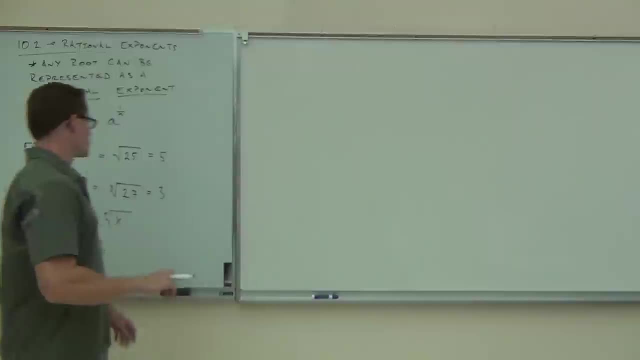 Don't answer this question out loud. I want you to think of it. OK, Now, of course, we're getting pretty good at this. We know that's going to be 5, and that's going to be 3, and this is the fifth root of X. 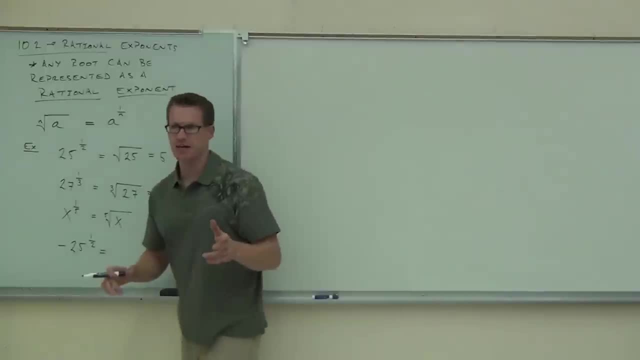 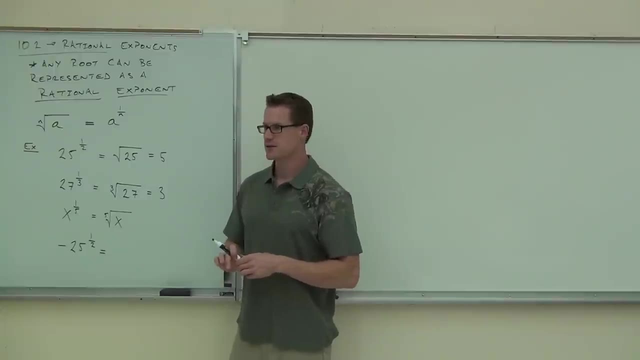 I want you to think of it. Don't answer because I'm going to tell you the answer in a second. I want you to think of if this is possible or not. Don't say it out loud, Just think I see a lot of mmm. 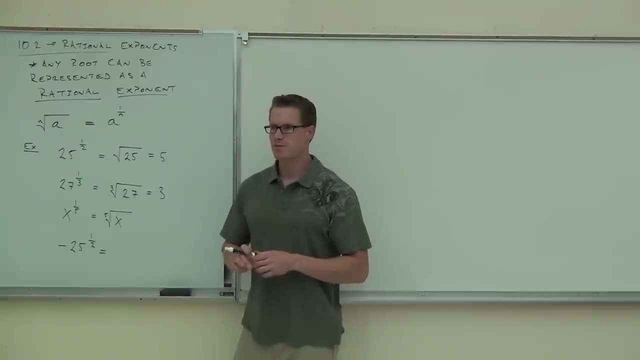 I see a lot of mmm. Now here's the deal. A lot of people are thinking no, right now, because you have a negative. And what type of root is that? Square root of X. And what you know is that you can't have a negative inside of the square root. 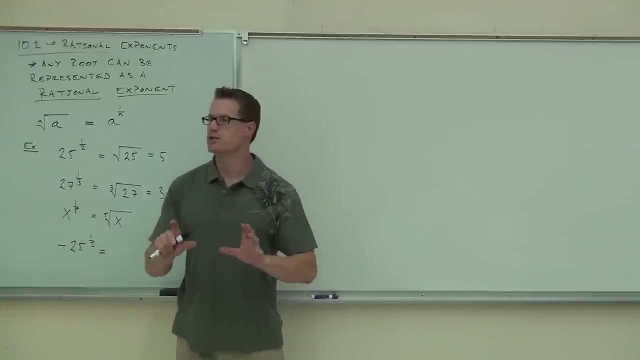 Nudge your head with me if you understand that, For sure, But here's what you need to understand When you're dealing with exponents. if you have something like this negative 4 to the third power, what this means Actually, you know what. 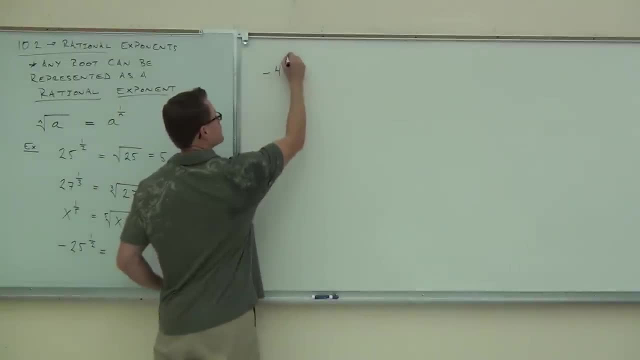 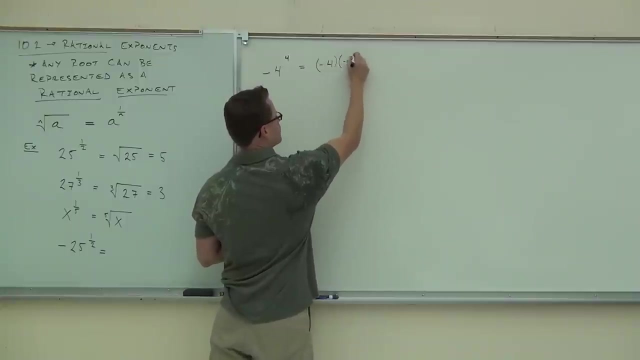 Let me make it to the fourth power. What negative 4 to the fourth power means is the opposite of 4 to the fourth. What do I mean by that? This does not equal negative 4 times negative, 4 times negative, 4 times negative, 4.. 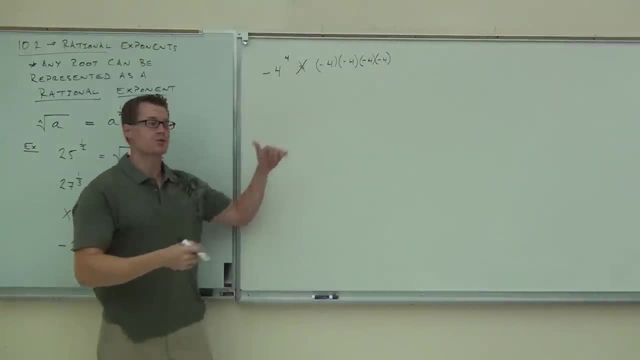 That's not the same thing. What this actually equals is Here. I'm trying to make this so you really understand it. Think of your order of operations. What comes first, multiplication or exponents? Hopefully, exponents come before multiplication, right. 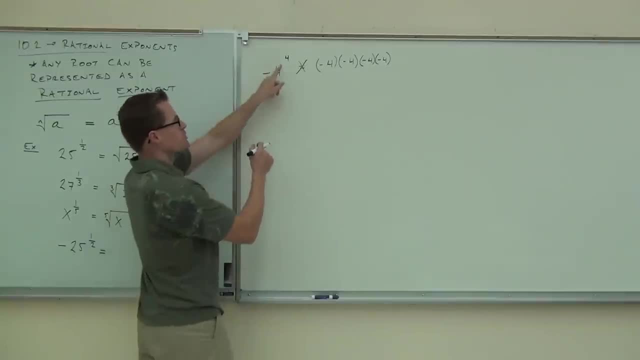 M dots. So if we have order of operations it says you're supposed to do your exponents. before you do your exponents You're supposed to do any multiplication. So what this actually can be written as: pay attention up here. 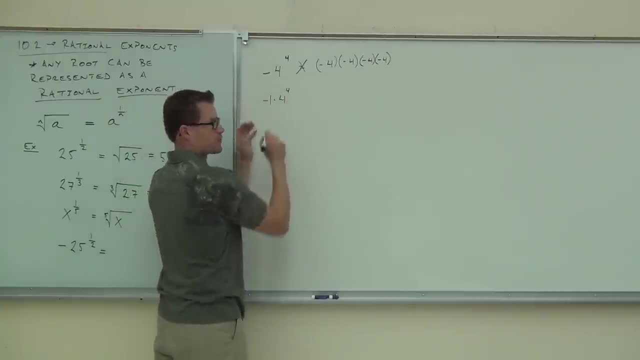 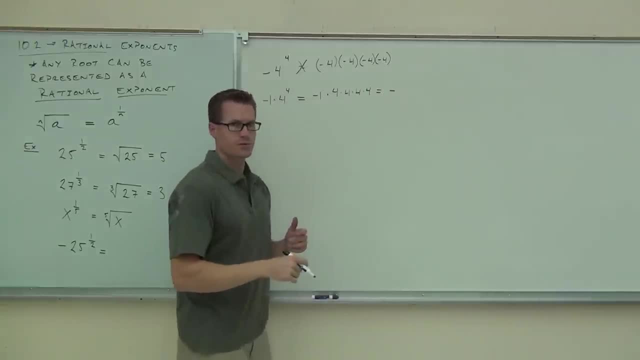 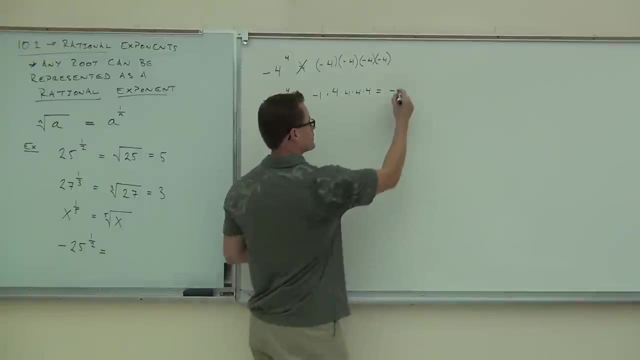 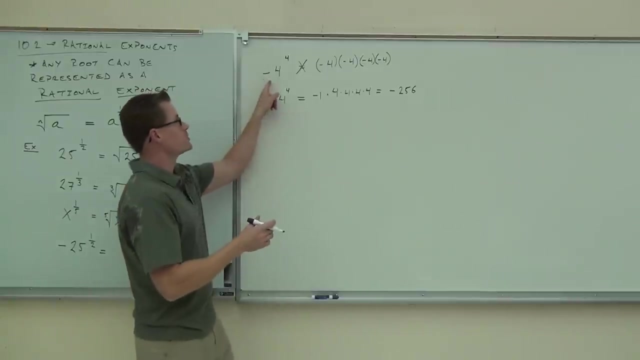 Or in other words, negative whatever. 4 times 4 times 4 times 4 is Negative. 4 to the fourth, 64 times 4.. 256? Negative 256.. So even though you have a negative 4 to the fourth power, you're still getting a negative. 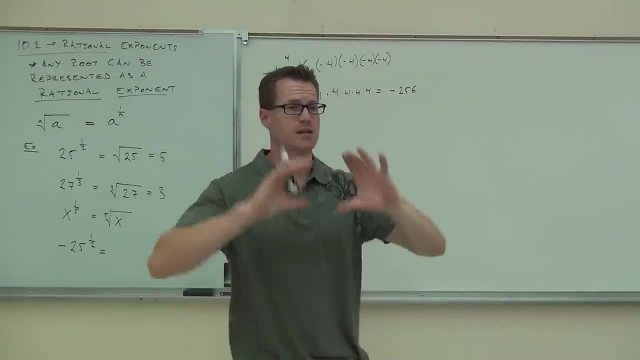 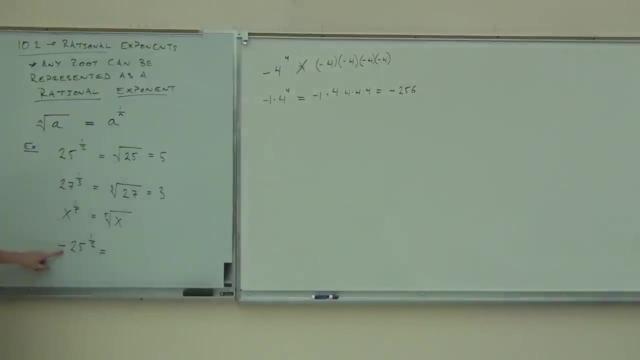 Are you guys okay with this? Here's what I'm trying to say. Unless your negative is in parentheses, it is not being applied towards that exponent. Are you with me? So in this case, is this negative 25 going to be inside of the square root or is it going to be outside of the square root? 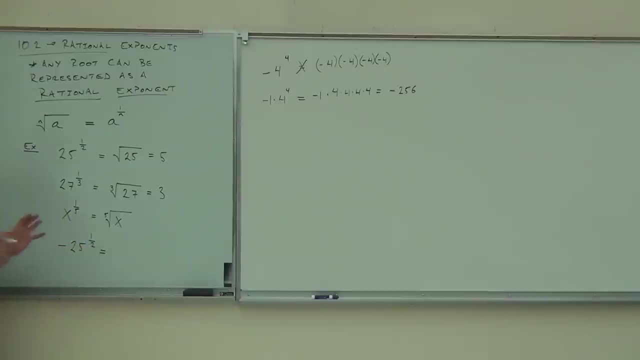 Outside. It's going to be outside. Yeah, How I would show it inside is if I had this Watch on the board. If I had that, then it would be inside the radical. Are you with me If I don't have that? 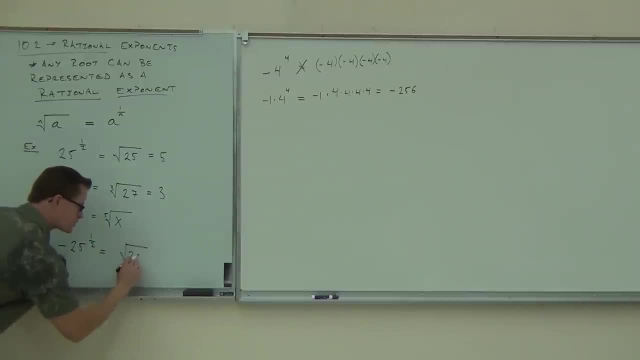 Very important that you get this, by the way. If I don't have that, this is a square root of 25.. This is the opposite of the square root of 25.. That's what that is. Is that possible? Yes, 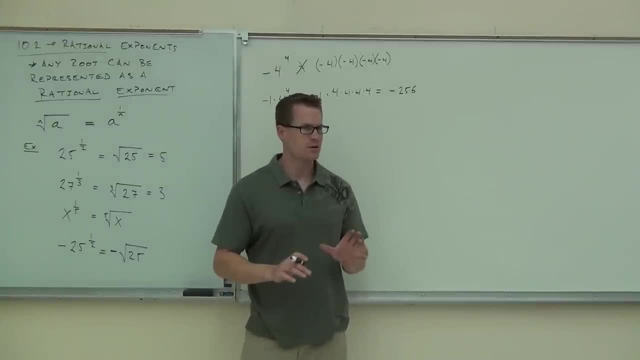 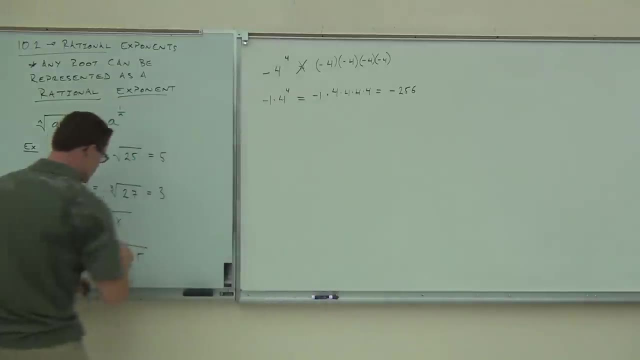 That is definitely possible. Do you see the difference here? Okay, So that negative. if it's not in parentheses, it will not be inside of the radical. If it is in parentheses, then it will be. This one is actually equal to how much? 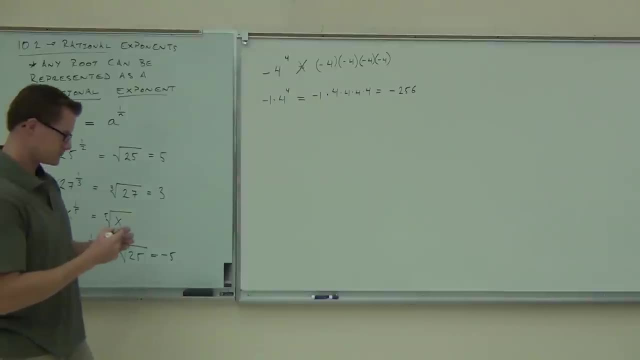 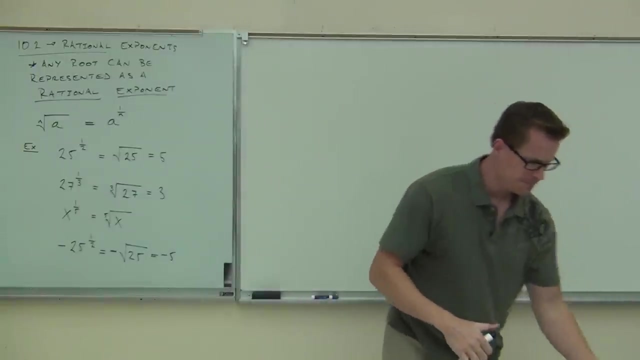 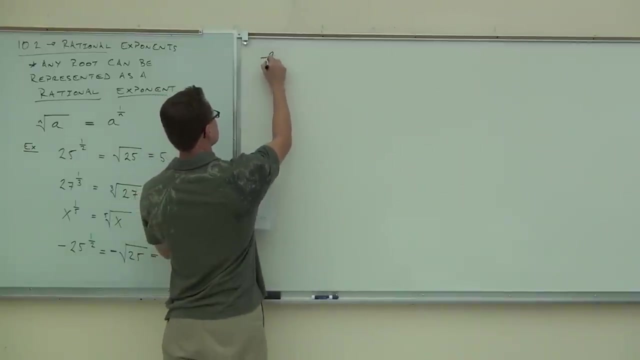 Negative 25.. Yeah, perfect. Okay, let's try a few more with that in mind. Okay, let's try a few more with that in mind. Negative 27,. y to the sixth, all to the one-third power. All to the one-third power. 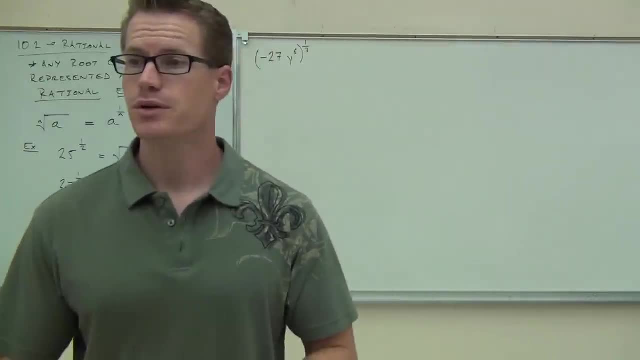 Firstly, I want you to identify if we have a root here. Do we have a root? A radical? What tells you I'm going to have a radical here? What type of exponent do we have? Fraction exponent- Okay, good. 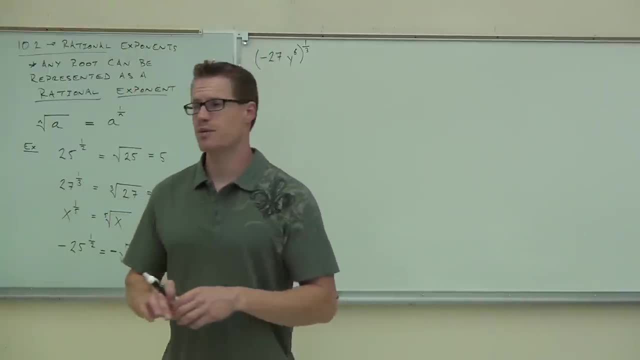 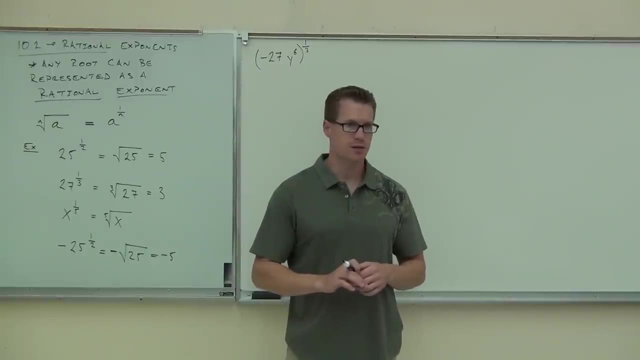 So anytime you have a fraction exponent, it means radical, for sure. What type of a radical do we have? What type of root? Cube root, all right, And is the negative going to be inside the cube root or not? Inside or not? yeah, why? 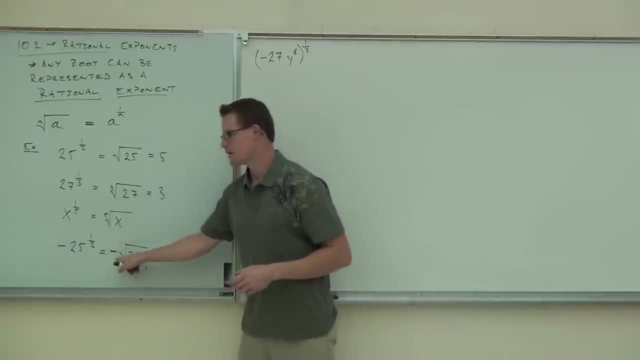 Now I want you to notice the difference. Here there's no parentheses, it's outside- Use your word- operations. that idea Exponents come before multiplication. This is being multiplied by negative 1.. Here, because it's in the parentheses. this says: oh okay, I have the cube root, sure. 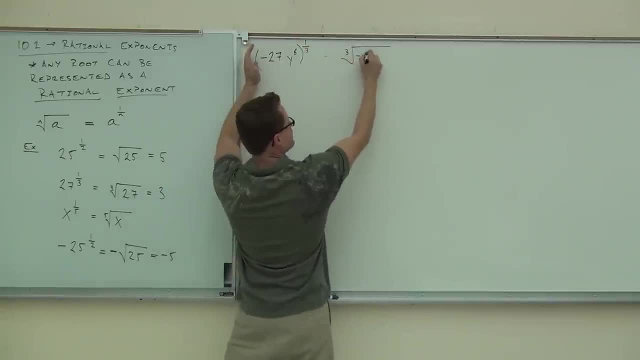 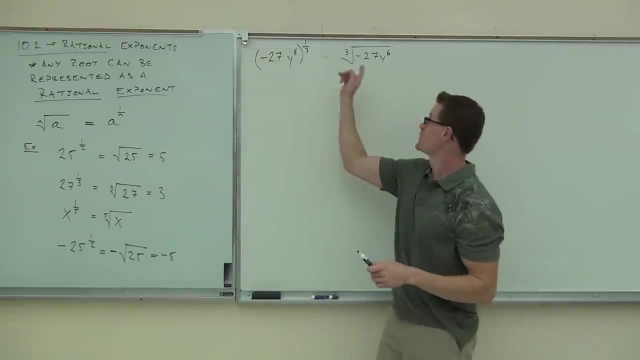 But since this is all connected with those parentheses, that's going to be inside of my radical. Raise your hand if you feel. okay with that one. Okay, I'll show you how to simplify those in a little bit. We're not going to quite go through that. 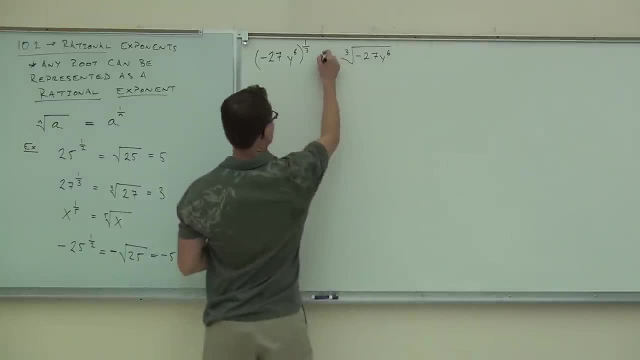 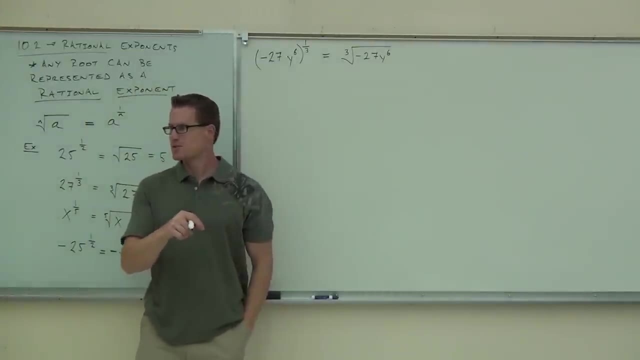 Well, I guess we could- actually We could- do that. now Let's simplify that. Do you remember how to simplify those from the very first section we did in this chapter? I hope so. Do we know how to do the cube root of negative 27?? 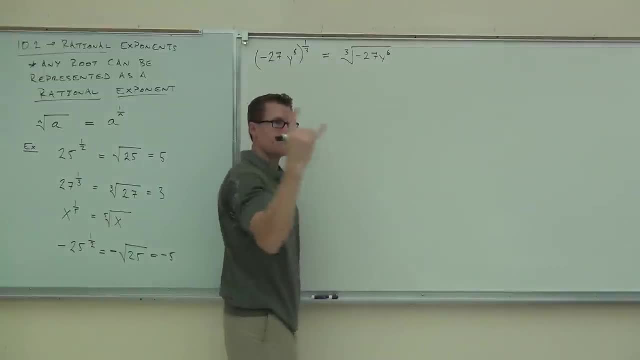 Sure, How about the cube root of y to the 7th? Remember how to do that. There's two methods. You would write this as something to the third power and cross those out, Or you'd write this as as many third powers as you can. 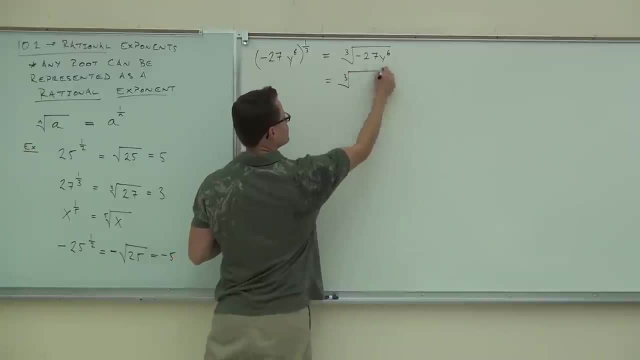 I'm going to do that method. So here you'd go. okay, cube root of negative 27,. I'm going to leave that for just a second because I know I can take that cube root And instead of y to the 6th, I'll do y to the 3rd, y to the 3rd. 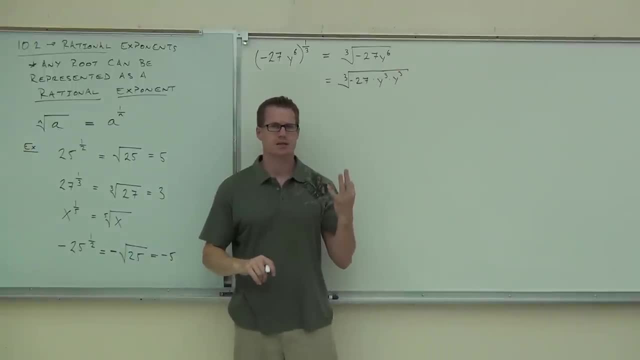 Why am I doing y to the 3rd power? Why is that Okay? so I want to match the power with the type of root that I have. So here we'll say What's the cube root of negative 27,. ladies and gentlemen, 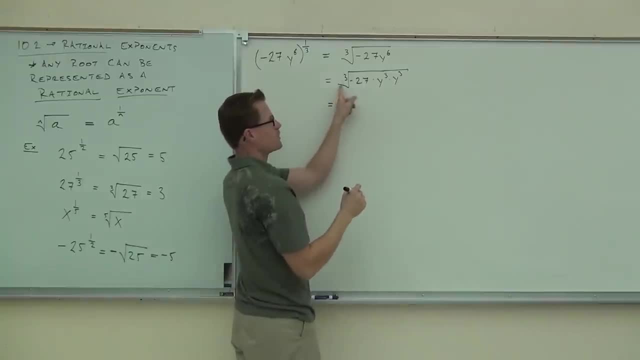 Negative: 3. Good, What's the cube root of y? cubed, Y squared. Those are gone. right, I just have what left: Y to the 2nd. Okay, so with both of them, I'm going to have y to the 2nd, absolutely. 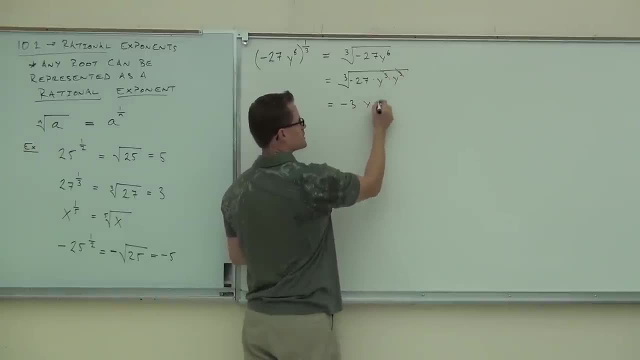 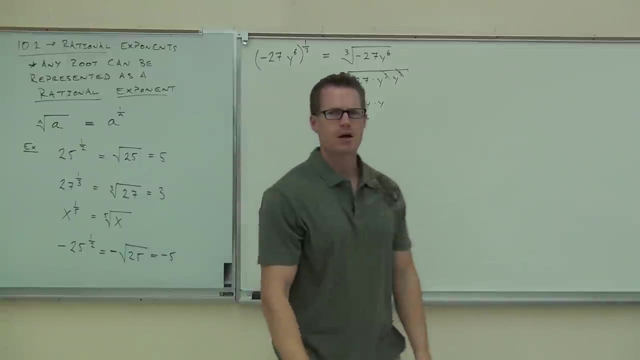 Yeah, this is going to give me a single y. This is going to give me a single y. So this all together, you guys are right: negative 3y squared, Absolutely. you guys remember that from before, actually before our test, wasn't it? 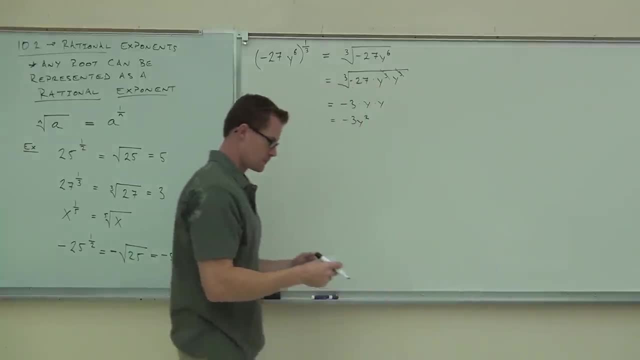 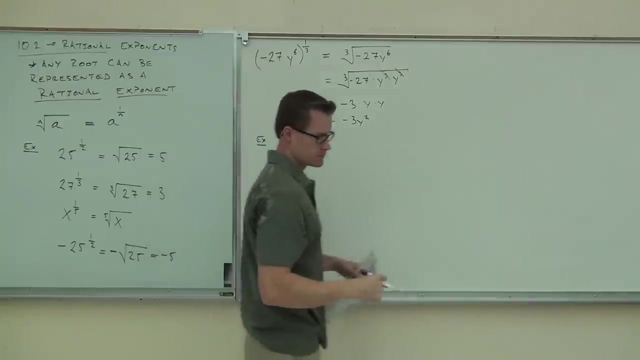 Yeah, All back. Let me show you one more thing, or you can do something on your own, then we'll move on 7x to the 1 5th. Now this one, this one, I got a lot of people on right right off the bat. 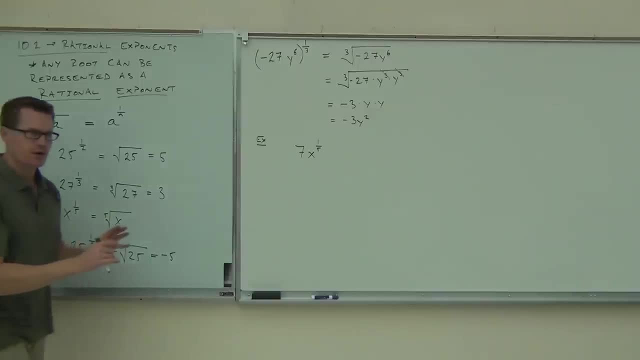 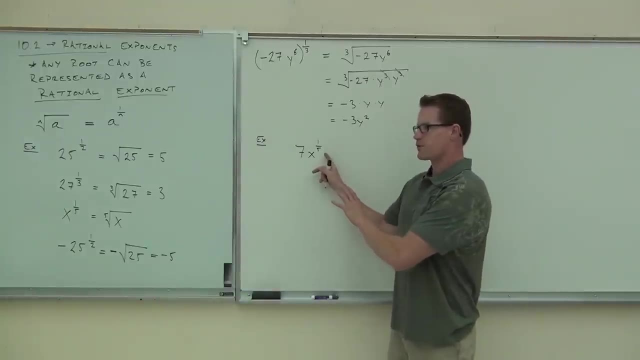 because a lot of you were thinking, oh, this isn't possible, because you thought the negative went with that exponent. I want you to look at this. I want you to look at this: real, real, careful, okay, The 1 5th. 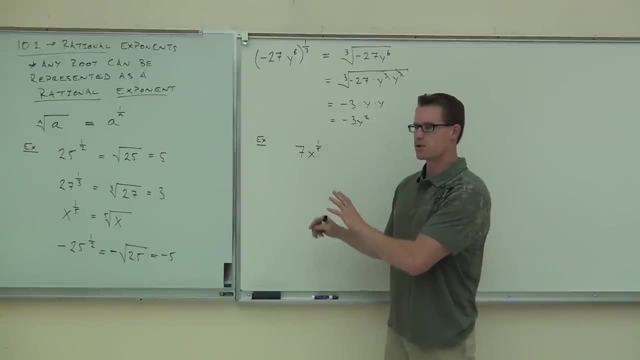 Is the 1 5th above the 7, above the x or above both of them, Just the x? Do you see how that 1 5th is just above the x? It's actually not 7 to the 1 5th. 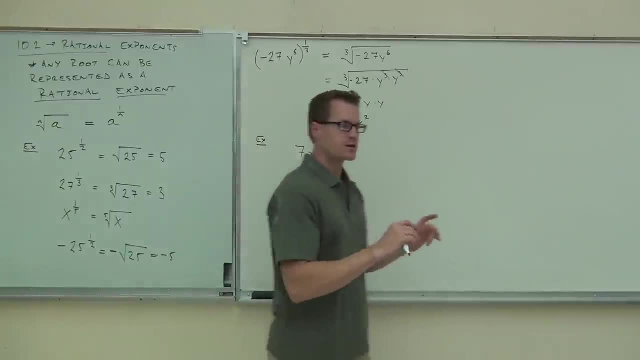 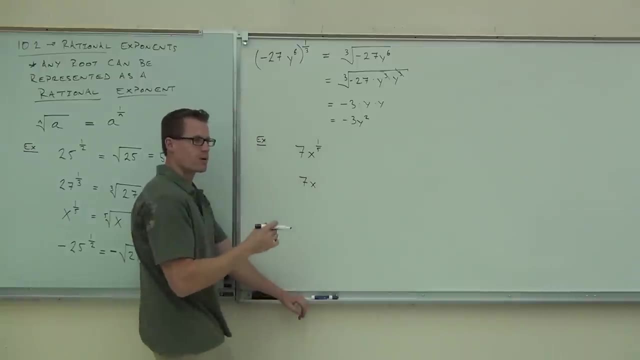 If I wanted to show 7 to the 1 5th, 7 and x to the 1 5th, here's how I'd do it. I want you to see the difference here. If I want to show both of them, what would I need to put? 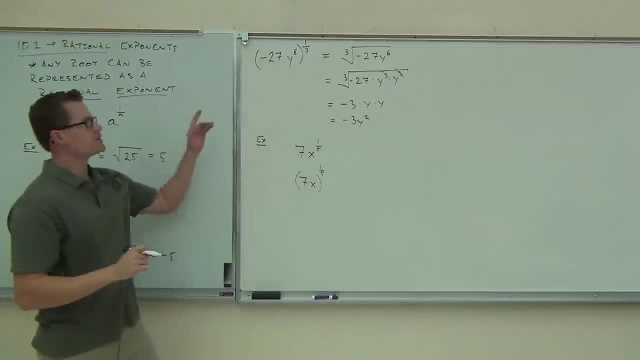 Very similar to this negative idea. Notice how, if I want to include the negative, I've got to have it in parentheses. If I don't want to include the negative, I don't have parentheses. If I want to include the number, I've got to have parentheses. 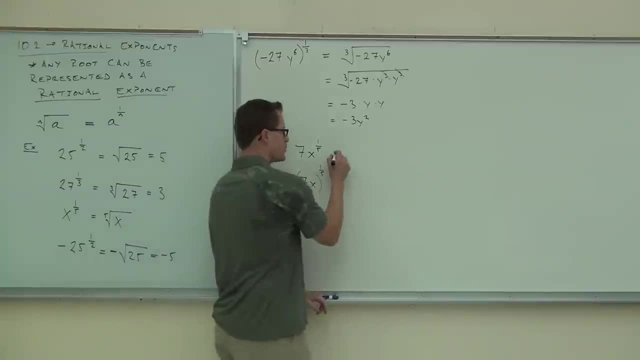 If I don't, then I don't. So, on this example, is the 7 going to be inside of our root or not? What do you think? No, it's outside. It's outside. yeah. What this says right here is 7 times x to the 1- 5th. 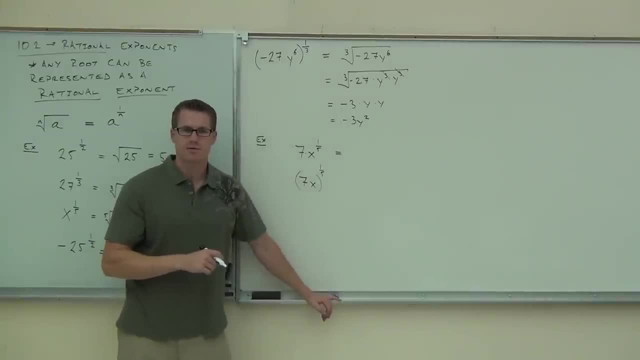 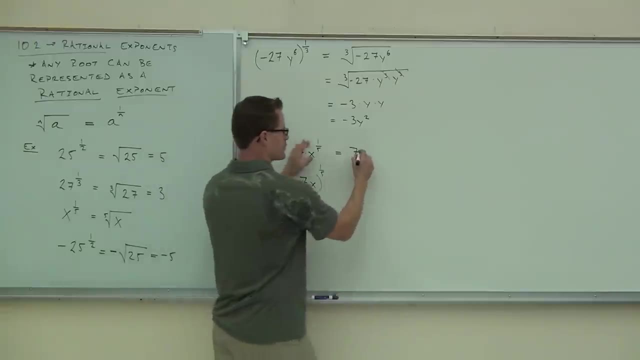 Are you with me? It's like the negative 1.. 7 times x to the 1- 5th. Use your order of operations and think about this. This says I'm doing 7 times the 5th root of x. 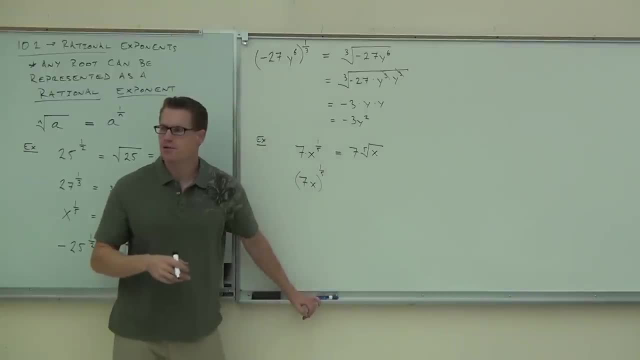 That's 7 times the 5th root of x. The 7 is not inside the radical because it's not in the parentheses. Folks, are you okay on that one, Are you sure? Yeah, Do you see the difference between this one and this one? 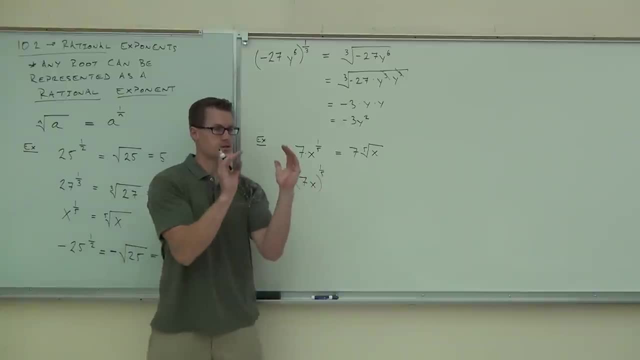 This is still 7 times x, but all of that's to the 1 5th power, So this says: all right, I do have a 5th root, and everything in the parentheses is going to be my radicand. 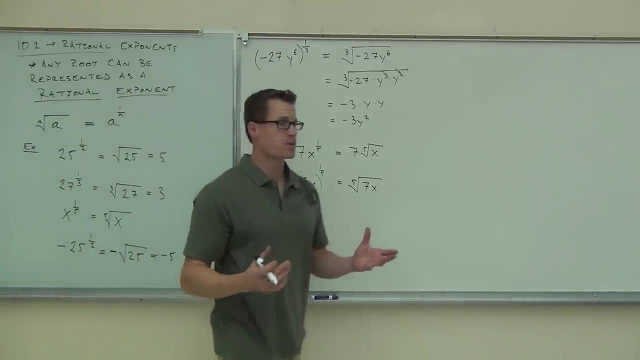 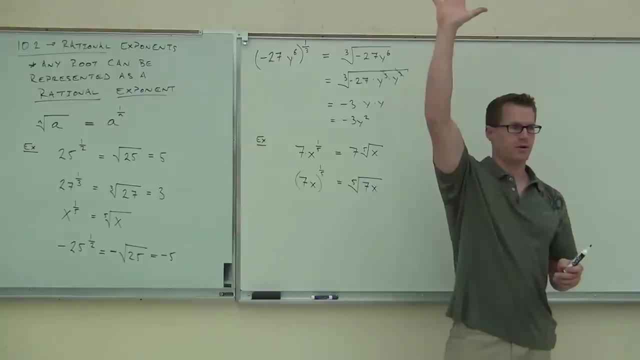 what's on the inside. So again, if it's in parentheses, yes, It goes inside of your radical. If it's not in parentheses, it doesn't. Raise your hand. if you're all right with this so far, Could you do a left side of the room, if you guys are okay with this? 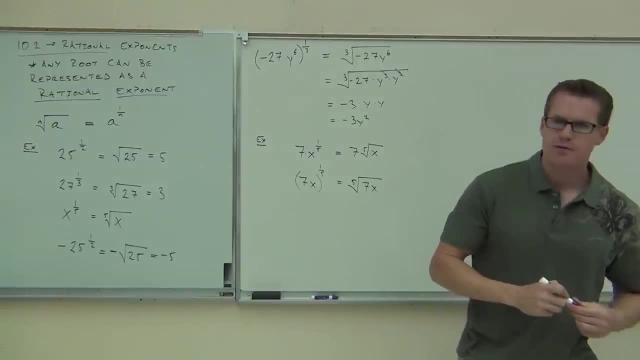 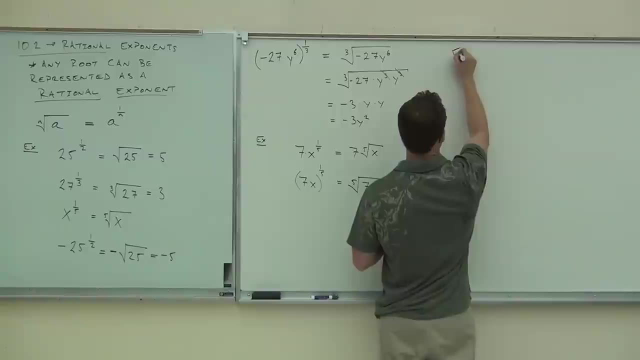 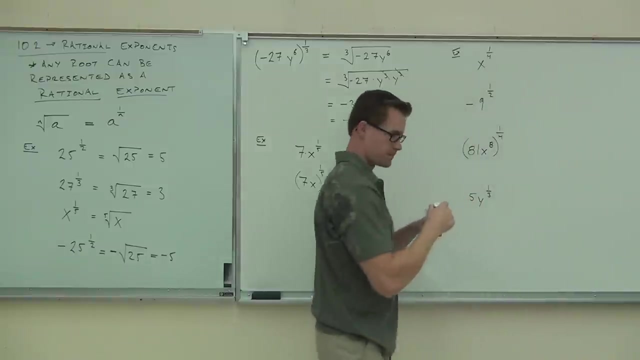 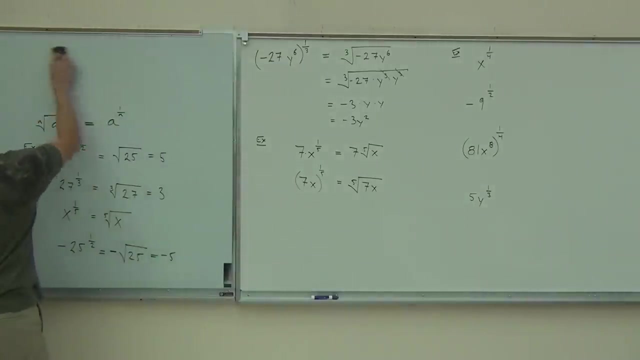 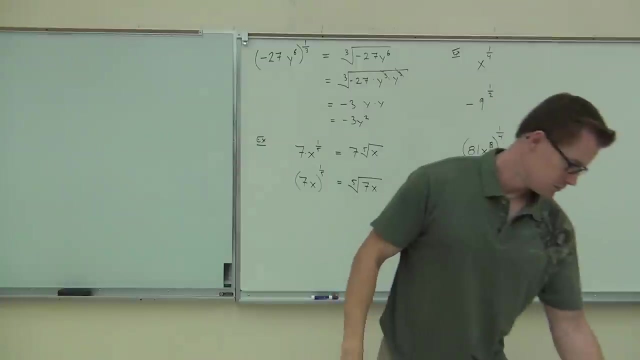 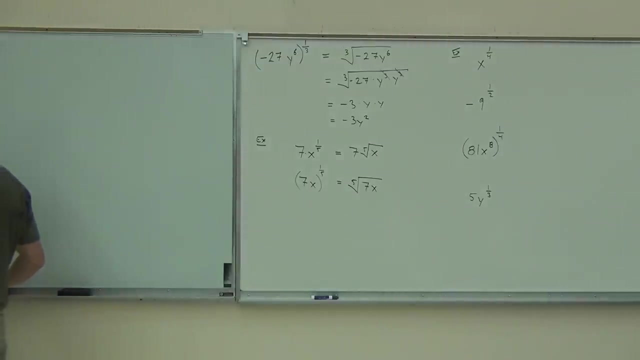 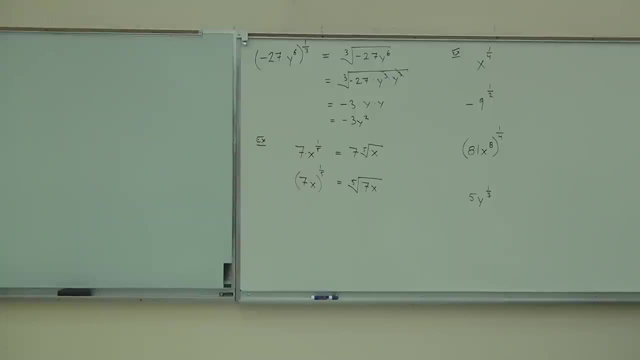 Thank you. All right, let's give these a try. So, x to the 1- 4th. we need to notice what type of roots these are, then be able to write this appropriately as the type of radical that it is. So what type of root do we have? if I have x to the 1- 4th? 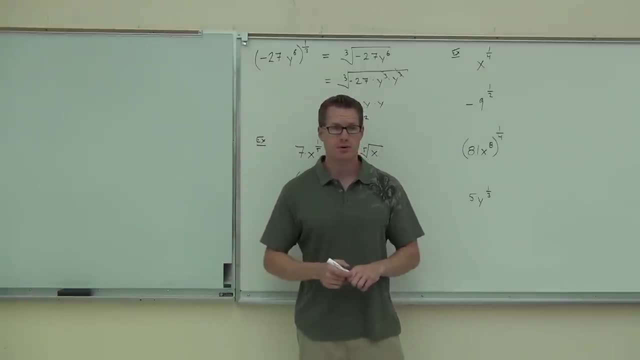 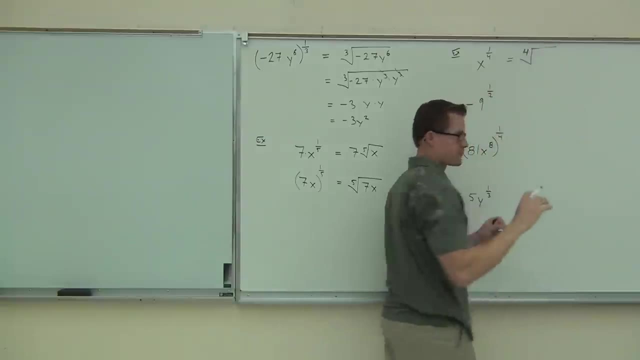 I know it is a root because I got a fraction. What type of root? Fourth root: Yeah, the denominator is going to tell you the type of root that we have. So here we have a fourth root, for sure, You can't forget about that 4.. 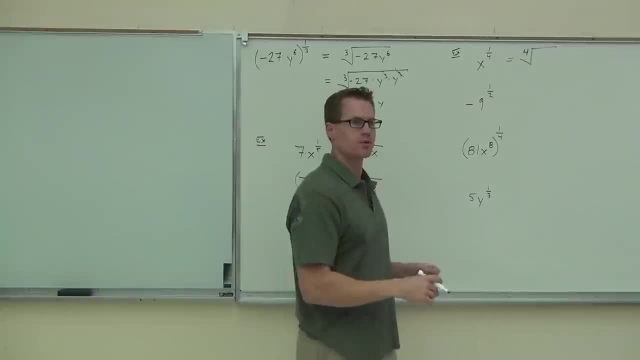 That tells you the type of root. right, We don't want to write square roots all the time. They're not all square roots. What is our radicand here? X to the what power, First power, First power, okay. 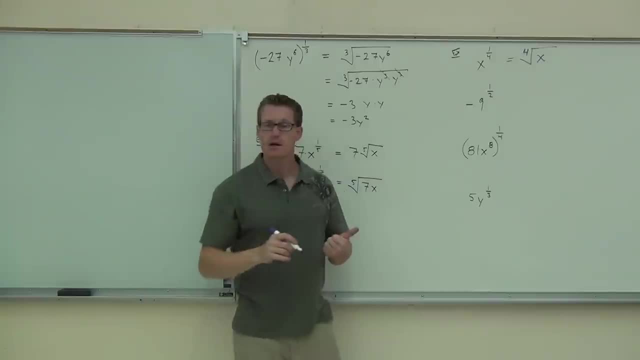 Did you all get the fourth root of x? Awesome. Next one: we got negative 9 to the 1 half. What type of root do we have? Square root. So I'm just going to write the radical without any indices, because that implies a square root. 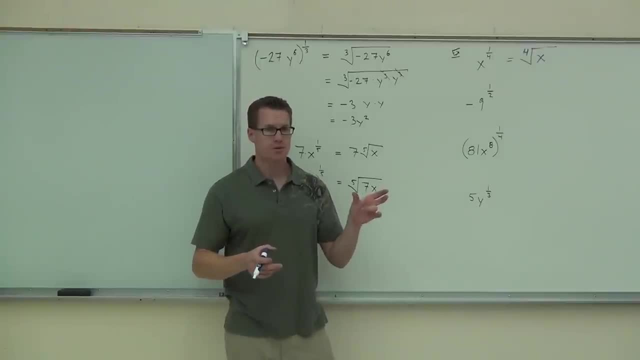 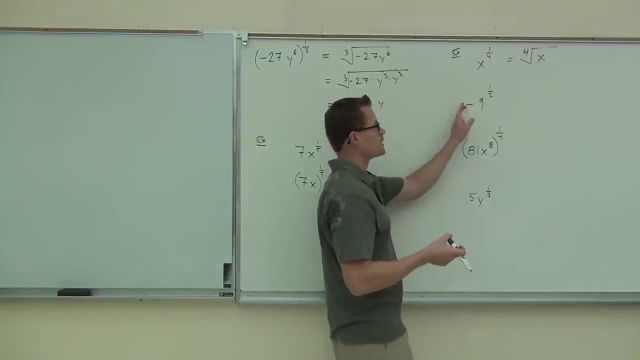 One question: is the negative going to go on the inside of our square root or the outside of our square root, Outside? Why outside? Because it's square root, Okay. so this is very much like saying this is negative 1 times 9 to the 1 half. 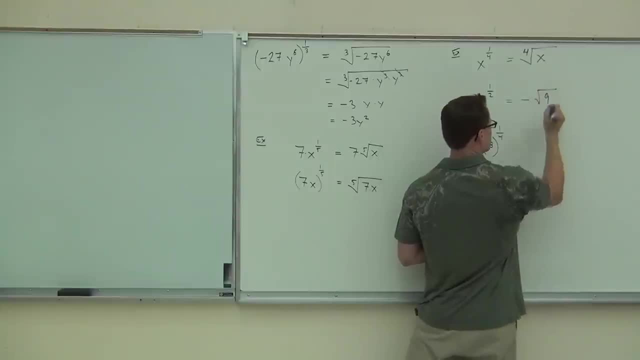 So, in other words, it's negative square root of 9.. That's something that we can do. We can do the negative square root of 9.. How much is that Negative? 3. Okay, so simplify it if you can. 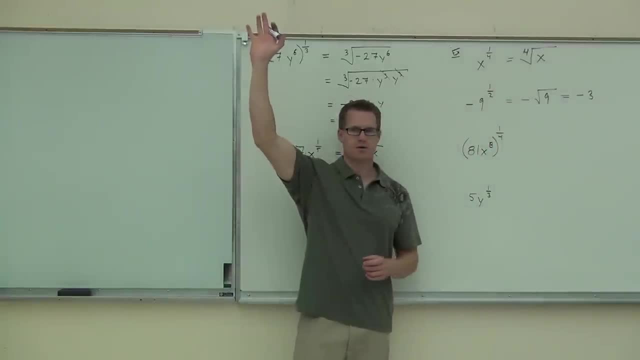 You get negative 3.. How many people are 2 for 2? so far, Good for you, That's fantastic, Okay. next up, we have 81 x to the 8th, all to the 1 fourth power. What type of root do we have here, ladies and gentlemen? 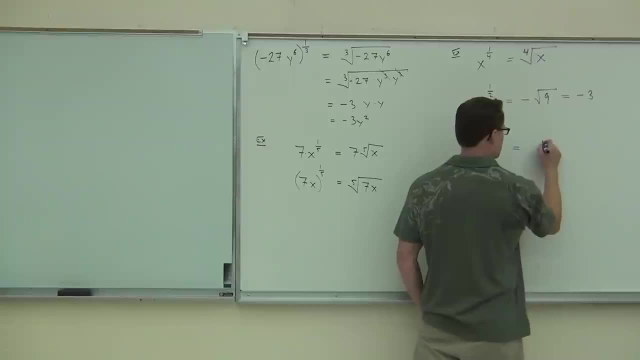 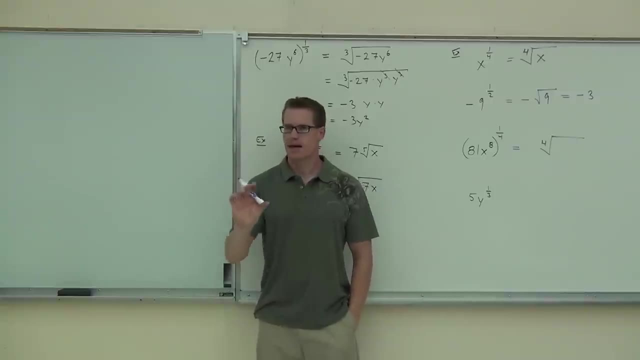 Fourth root, Fourth root: okay, so I know that I'm writing at least a 4 for the radical. Now the 81, is the 81 going to be on the inside of our radical or the outside of our radical? Inside? 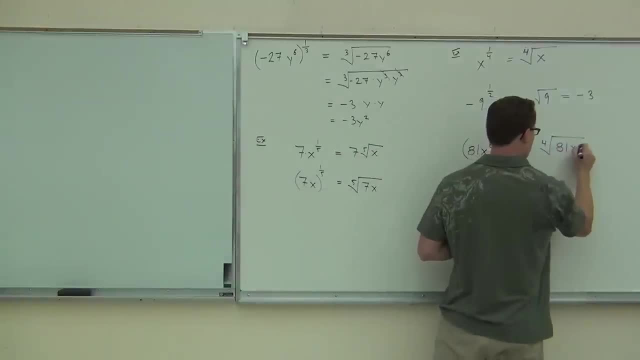 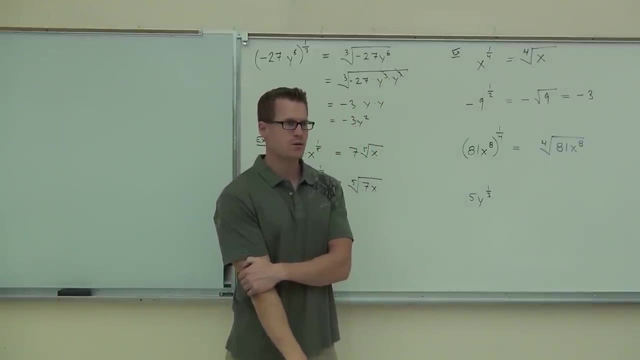 Definitely, it's in the parentheses. So we've got 81 x to the 8th. We have a fourth root of 81 x to the 8th. Let's try to simplify that. Can you think of the fourth root of 81?? 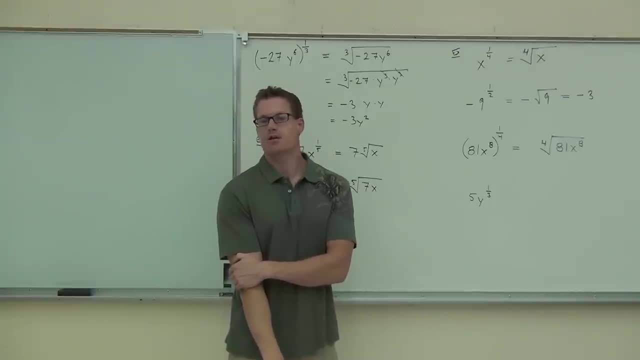 Something times itself four times, it gives you 81.. 3. Yeah, you think of maybe the square root and then do it one more time. So the square root of 81 is 9.. The fourth root: split those up, you get 3.. 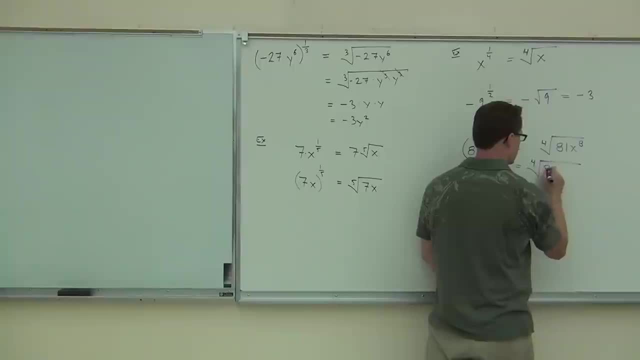 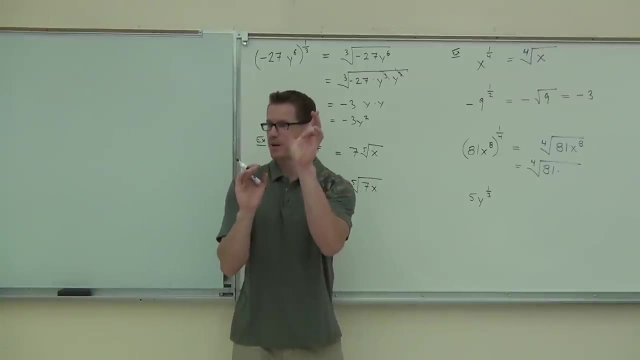 I'll leave that for just a second. We'll do the fourth root of 81 times and I'm going to write x to the 8th. You can choose to do this two ways, Either as something to the 4th power, that would be x squared to the 4th power. 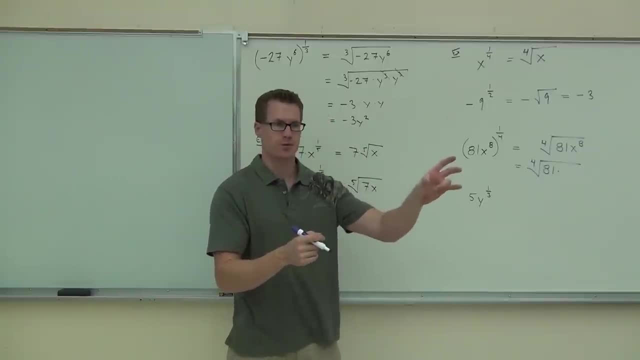 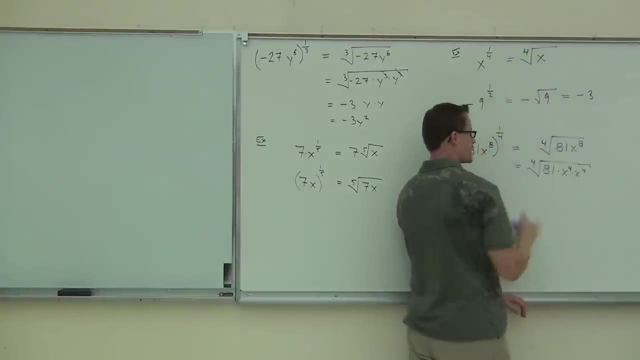 and cross out those 4ths, or you write x to the 4th times x to the 4th. Either way, you want to do that As many x to the 4ths as we can and still make up x to the 8th. 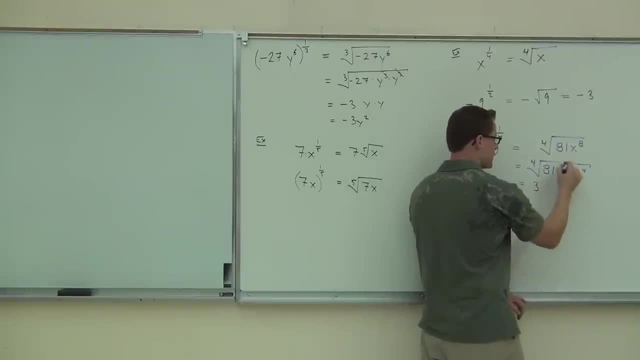 So we have the fourth root of 81, you all told me that was 3.. This gives you 1x. This gives you another x. So we have x. So we have x squared. Did you get that one? 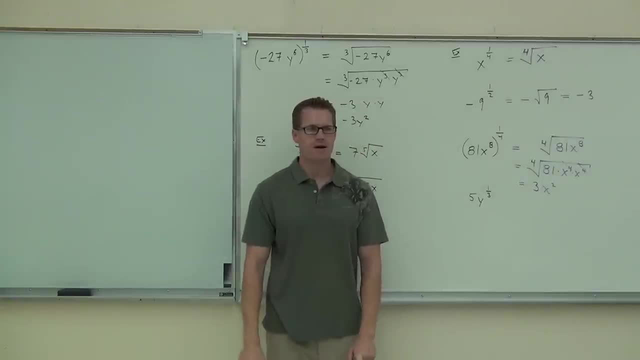 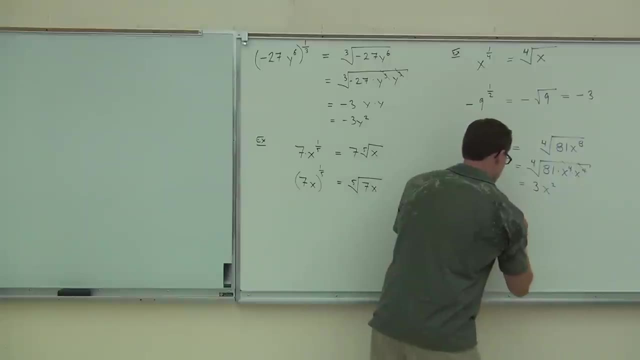 Good, Okay. Last one: We have 5y to the 1 third. What type of root? Third root, Third root, Okay, cool. So I know I'm going to be drawing a third root On the inside of our cube root. what do we have? 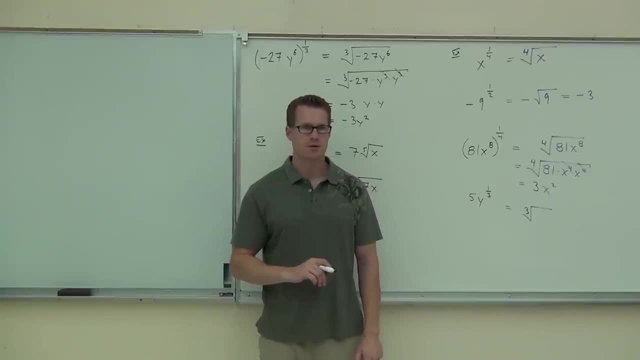 Y Well, what happened to the 5?? It's not included. Okay, So we don't have the same situation here. Here, the 81 was inside of our root because it was in the parentheses. If it's not. If it's not in the parentheses. 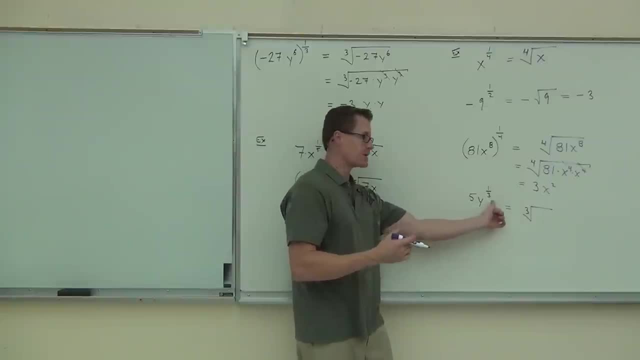 This exponent is really only being applied towards this y. It's not actually going to the 5 as well. There's no distribution of exponents like that. if there's no parentheses Here, we can, because well, it's all- to the 1 fourth power. 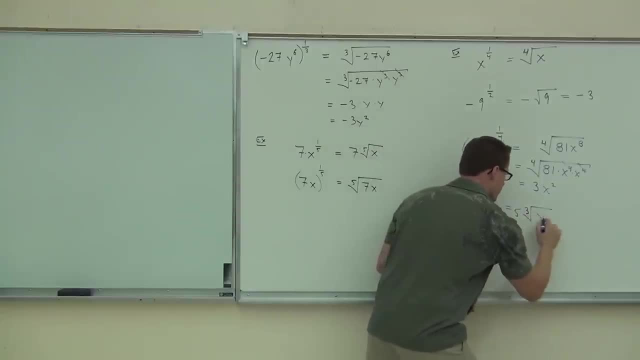 Here there's none. So we have the 5 up front, The y as our radicand, And that's our answer. We can't do anything more than that. How many people feel pretty good about this? so far, Good. 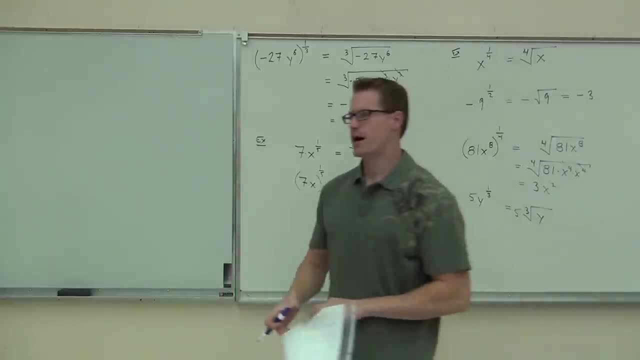 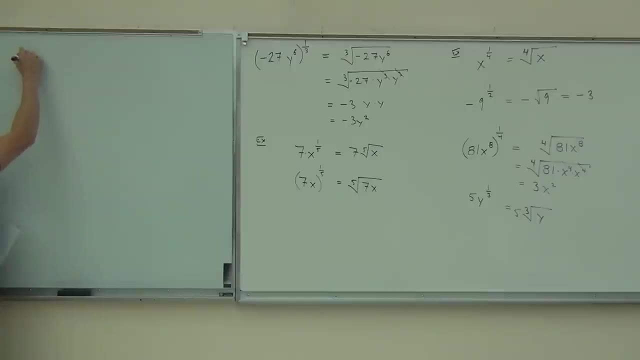 Now what would happen if, on the inside of our radical, we didn't just have a power? 1. I kind of previewed this. I previewed this a little while ago. But what if we had an nth root of a? This is exactly how we started our lesson today. 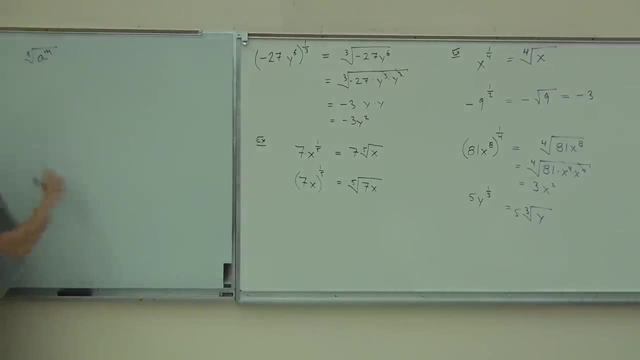 But instead of just having a little 1 here, we had another power like m. Let me draw that bigger so you can dream that a little bit better. An nth root of a to the m power now. Well, here's what we've learned so far. 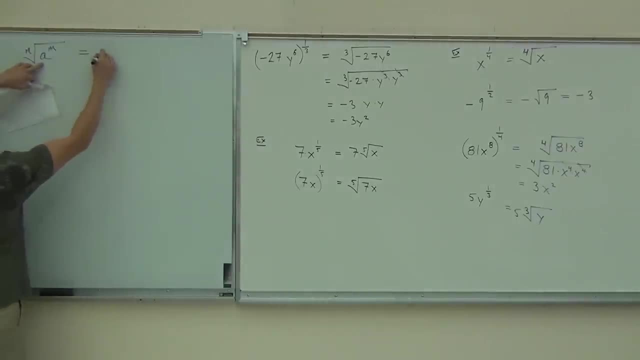 We know that whatever's on the inside of our radical is going to be our base, So we're still going to have an a. But before, when we had like x to the 1 fourth, the denominator told us the type of root that we have. 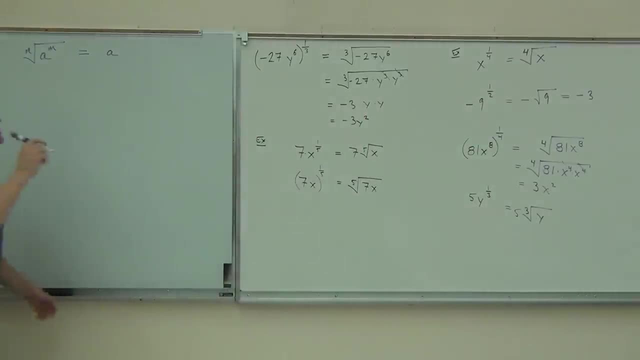 So in our case, what's our denominator here? So we're still going to have something over m. The root is always your denominator: Root, root, root, root. Every time. that told us the root. That's how we found it. 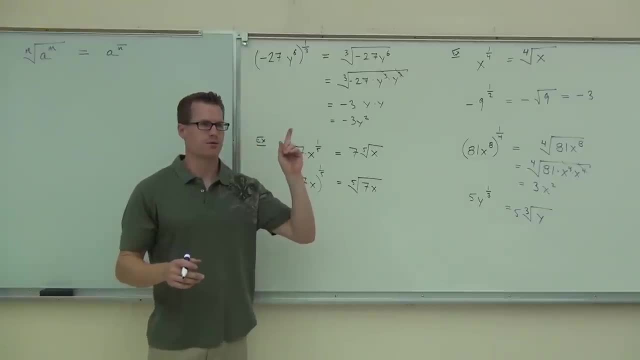 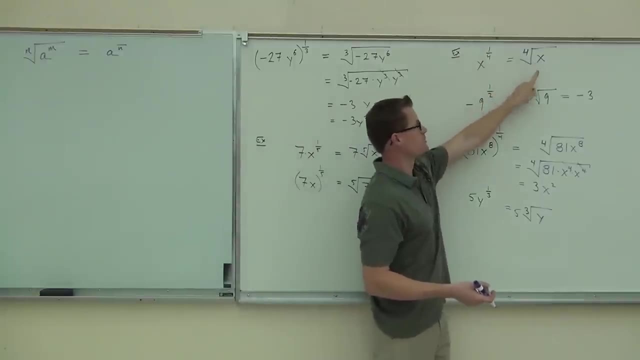 Only this time. instead of having a numerator of 1, what do you think? we're going to have? Just m. Whatever, the power is Here. in every case, our power was 1.. That's why we just wrote x to the first, 9 to the first. 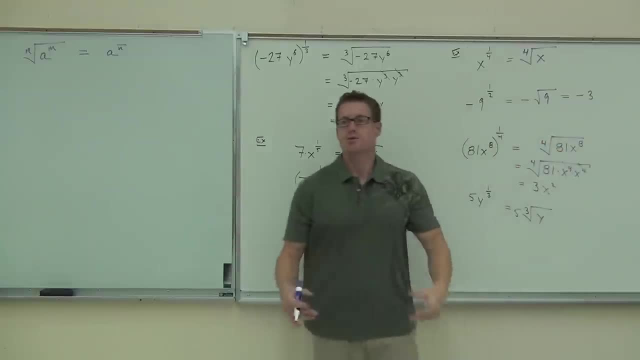 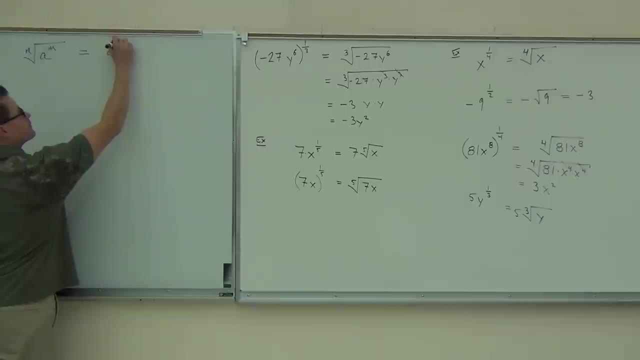 This was all to the first. Everything was to the first power. This was y to the first power. If I have another number besides a 1 up there, like an m, we just write a to the m over m. So it's power over root. 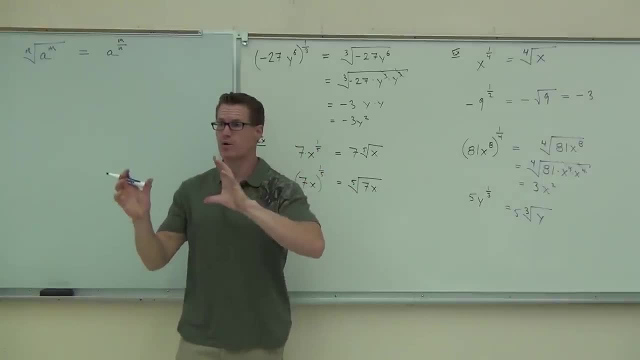 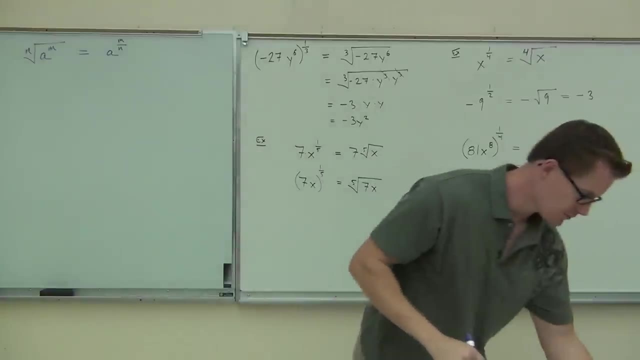 You guys got to get that in your head. How we write radicals is power over root, Power over root. Whatever the power is over, whatever the root is, None of you are going to be so okay with this, All right, Good, You want to see why? 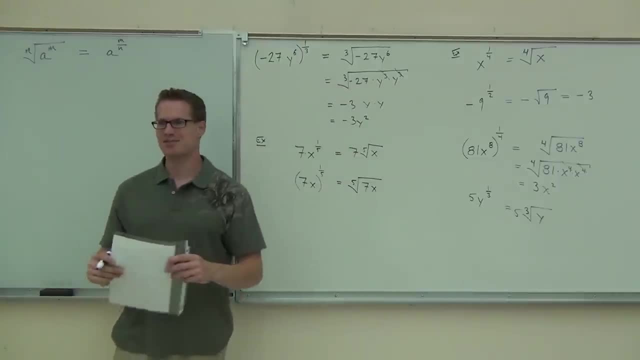 Of course you do. Answers always yes for that one. Do you want to see why? Yes, We're so excited at 725 in the morning to learn about why this is the way it is. Well, I can show you. You just have to trust me on one little piece of information. 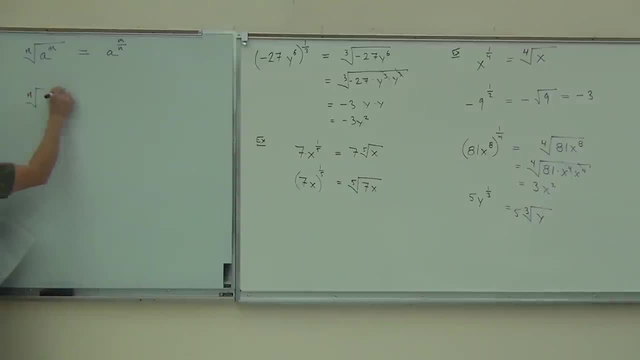 If we talk about this nth root of a to the m, you're going to have to believe me that it doesn't matter when I take this to the power. I can take it to the power and then find the root, or take the root and then find the power. 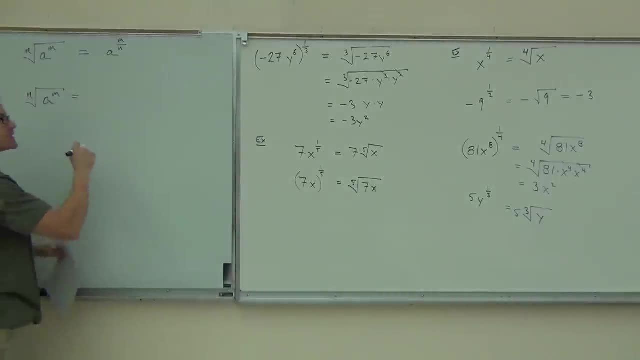 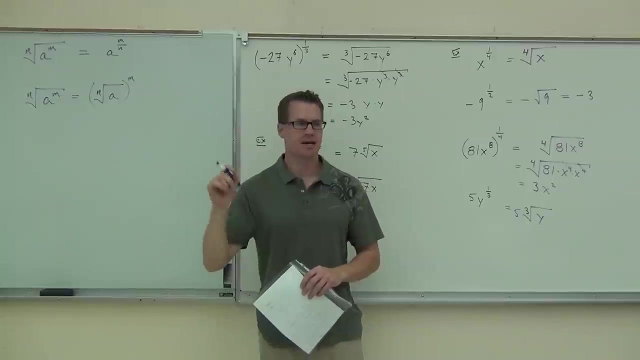 So you're going to have to trust me on this one little step, and then everything else falls into place. You need to trust me that this is the same thing as this, Do you trust me? Well, it is, And the reason why that is the way it is is because multiplication of exponents. 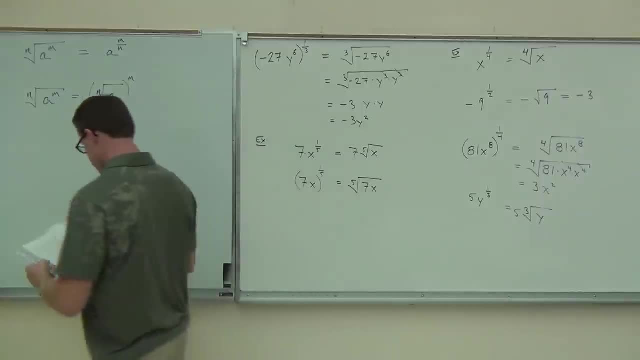 When you take a power to a power, you can do that. Well, here's the deal. We already knew how to deal with this. the nth root of a. This inside part was a to the 1 over n right. This is this. 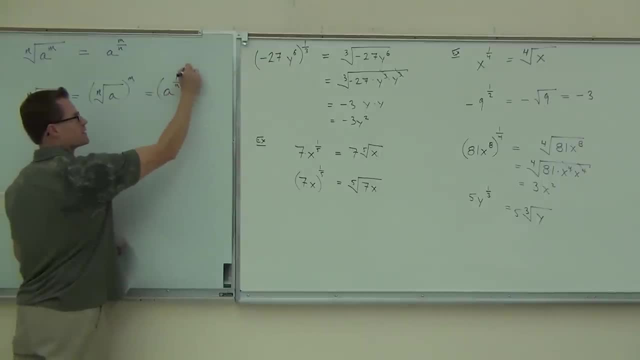 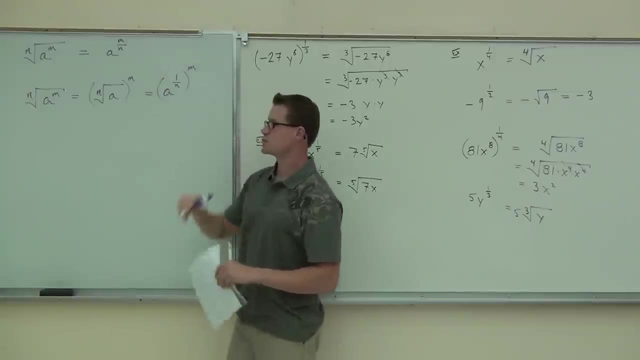 Do you guys see it? And then to the mth power. Now we kind of talked about this very briefly. But what happens when you have an exponent raised to an exponent? Do you add, Subtract, Multiply, Divide, What do you do? 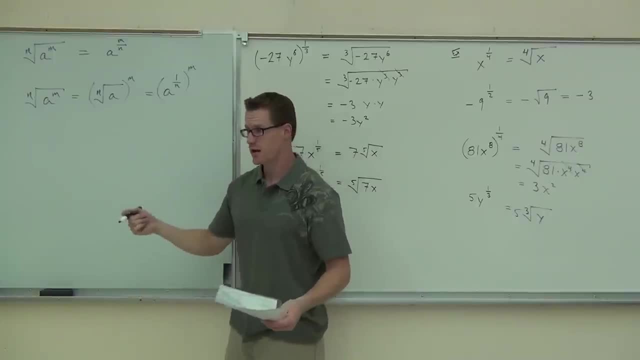 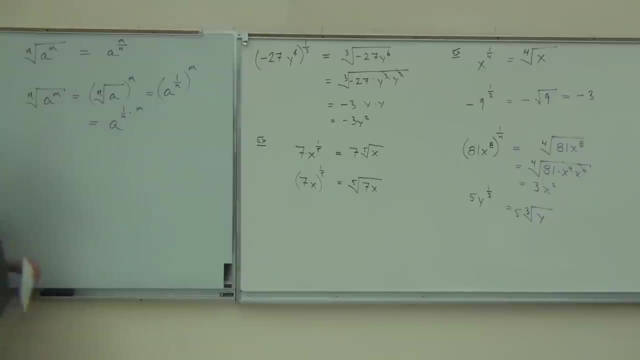 We should know those exponent rules right. When you have an exponent raised to an exponent, you multiply them, And so here we go. oh okay, Well, this is a to the 1 over n times m, Or in other words m over 1.. 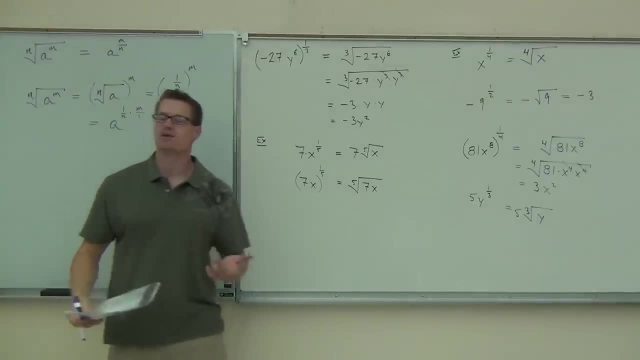 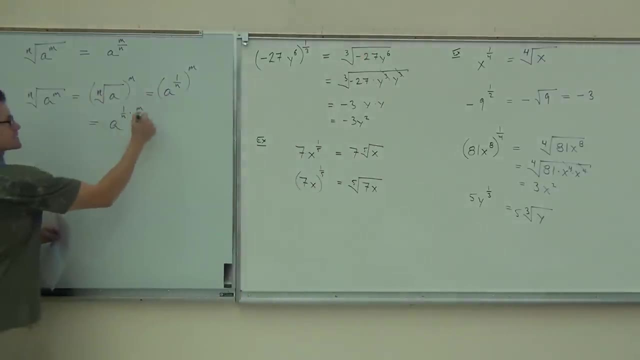 We can change m to m over 1.. And those are fractions. If you have 1 over n times m over 1, we know how to multiply fractions. We go straight across: 1 times m. 1 times m is m. 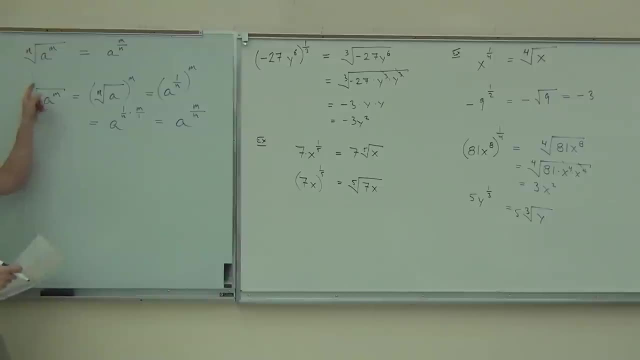 n times 1 is n, And that proves that. this equals that. Can you follow it? Yeah, Okay, So that's just a little proof. The only thing you have to believe is that step right there. Everything else kind of falls into place. 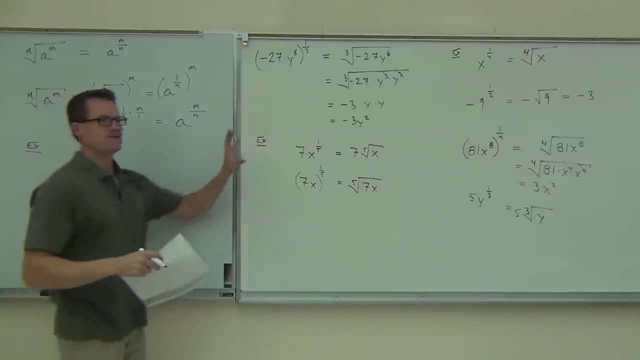 Let's see if we can do some examples. It's going to be very, very similar to what we just did over here. okay, Very similar. Let's do the cube root of 2 to the 5th. Can you write that as a fractional exponent? 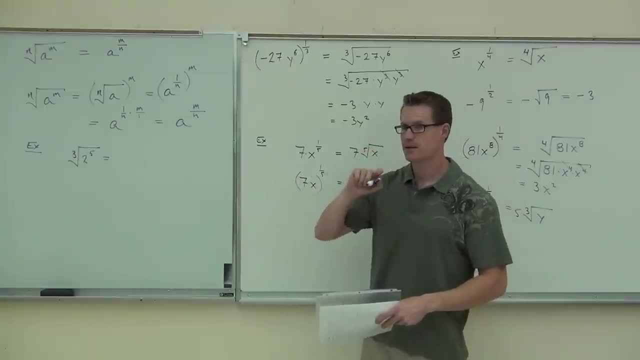 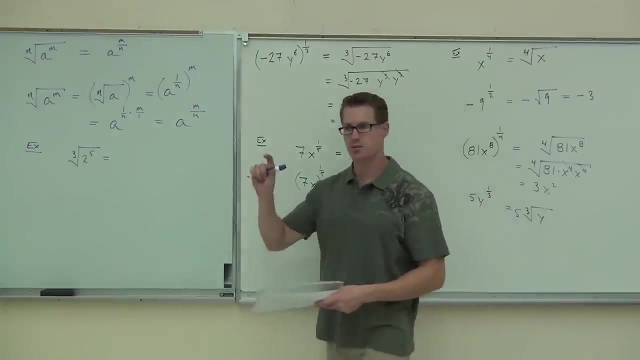 Can you write that as a fractional exponent? What is our numerator going to be in this case? 1. Good, It's going to be the powers of our numerator. What's the type of root that we have? So what's our denominator? 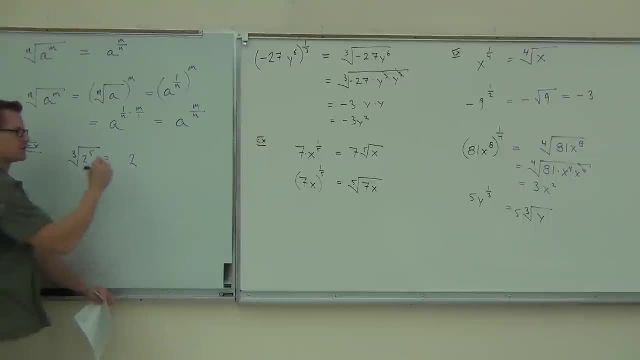 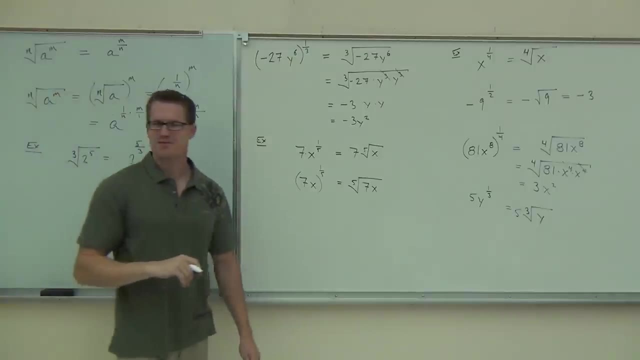 2. What power? 5th, 5th, 2 to the 5th. Do you ever think you'd see something like that? 2 to the 5th? What the heck? What does that mean? 2 to the 5th. 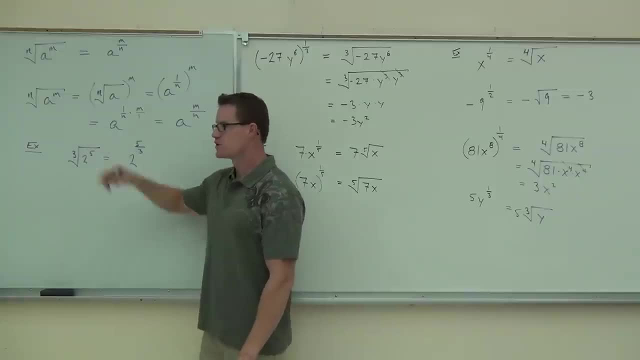 It means take a cube root after you take 2 to the 5th power. That's what that means. Can you go the other way? Can we do, Okay, 9 to the 3 halves? Can we do 9 to the 3 halves? 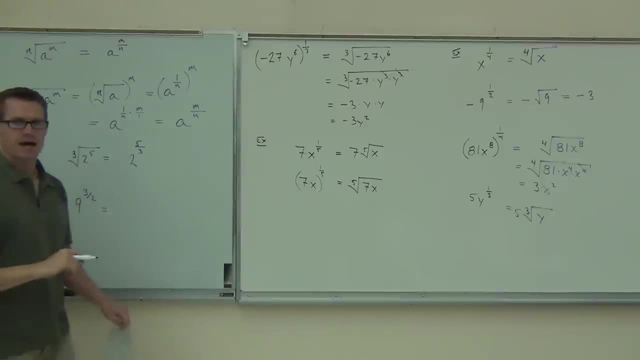 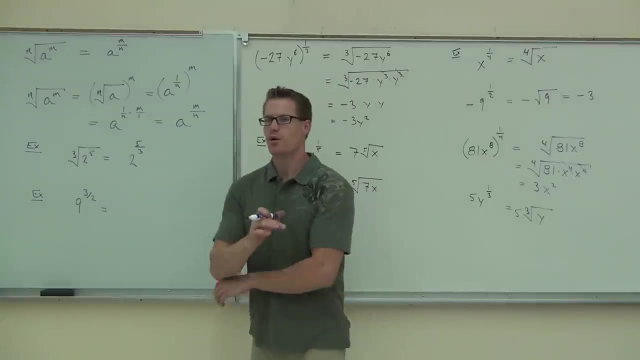 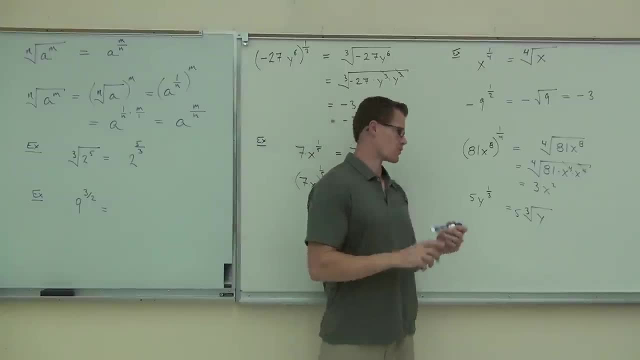 Square root, A square root. Why a square root? Because it's the denominator. Okay, So the denominator, this bottom number, that denominator is going to tell you what type of root you have every single time. So, in our case, we are going to have a square root. 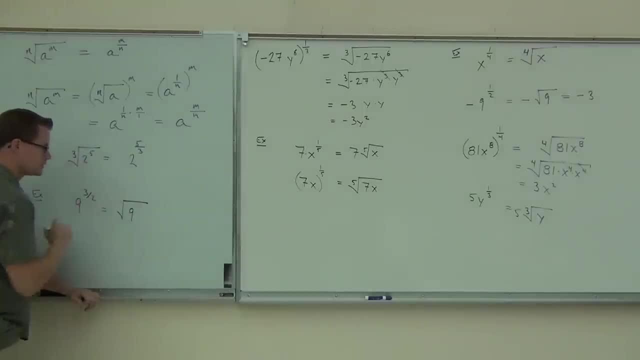 So in our case, we are going to have a 9, but that's going to be a square root. Now do we leave 9 to the first power, like I have it right here? What power is it going to be? 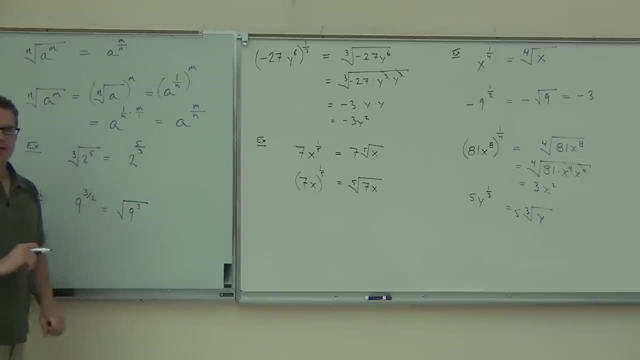 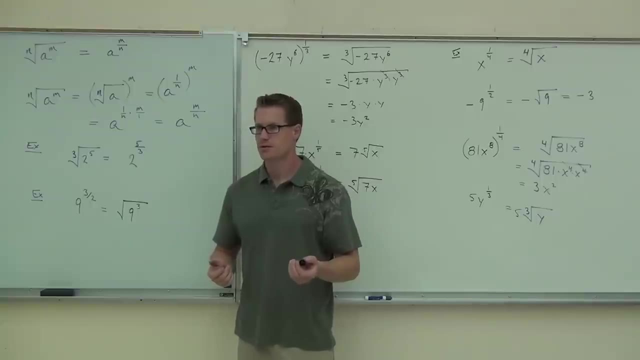 Okay, Can you simplify that? What this says is: take 9 to the third power. How much is 9 to the third power? 9 times 9 times 9, right Way more than 200.. It's going to be 81 times 9, so it should end in a 9.. 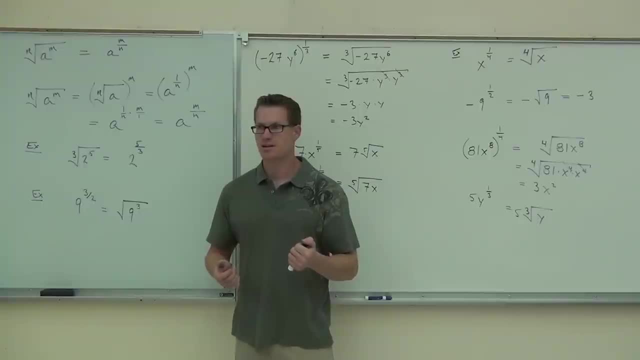 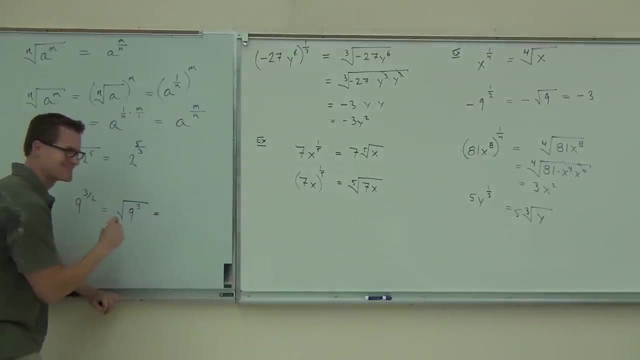 Yeah, 729.. Okay, 729.. You got it Easy. Double check that math, by the way. Is that right? Okay, and you all know the square root of 729, don't you? Of course you do. 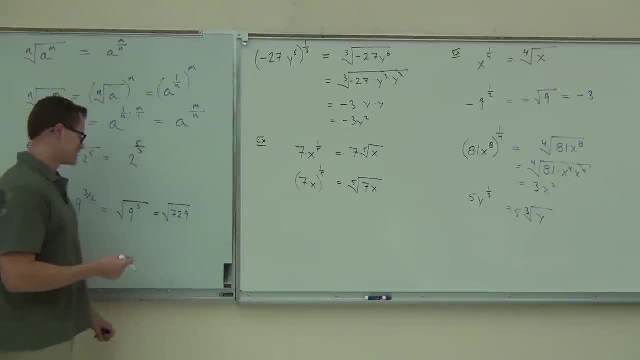 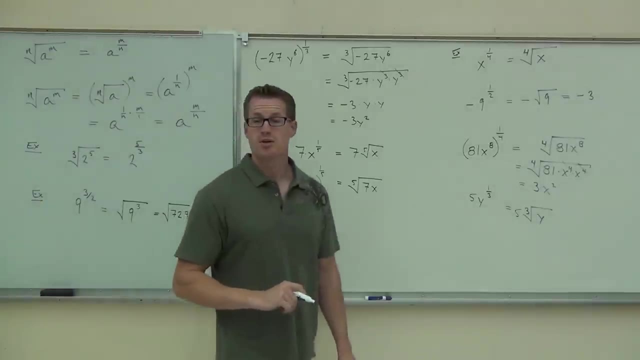 Come on, You don't know the square root of 729?? Oh my goodness, Yeah, it's 27.. How do you not know that off the top of your head? Would you like an easier way to do this? Did you believe me on this step? 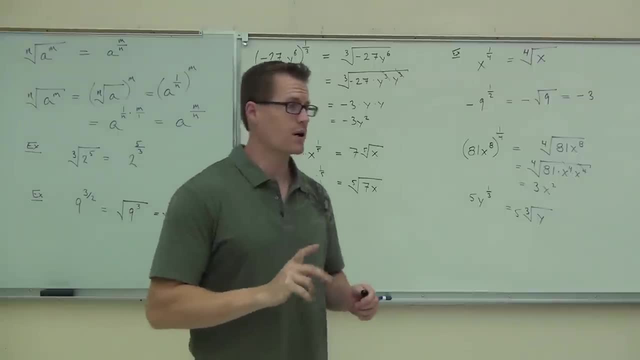 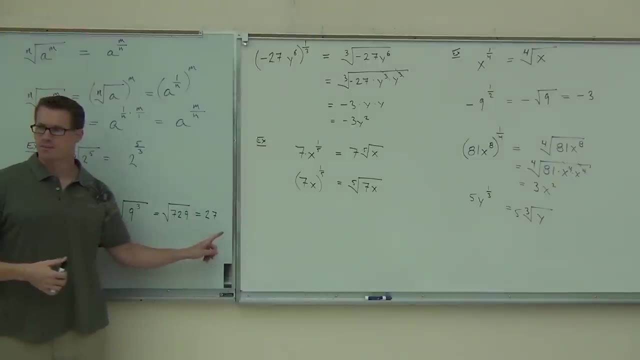 I want to show you something Right here. we did this the hard way. The hard way was make a really big number first and then try to find the square root of it. You with me, That's the hard way. Here's an easier way. 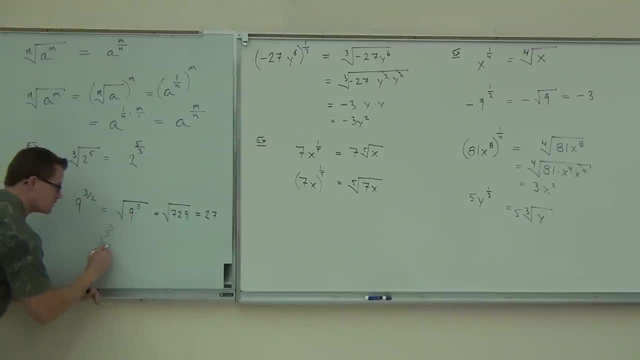 If you trusted me on On this step, watch what you could do Instead of having the square root of 9 cubed. I told you that this is the same thing as the square root of 9 cubed. Do you see that? I just moved the 3 to the outside? 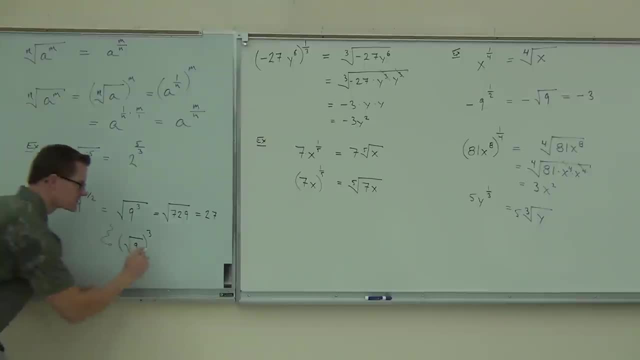 Now watch. I'll bet you all can do this problem very simply. Can you tell me what's the square root of 9?? Oh, everyone answered: This is 3.. What's 3 to the 3rd? Was that a lot easier? 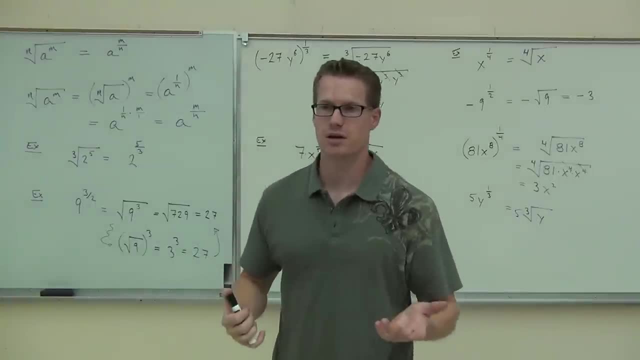 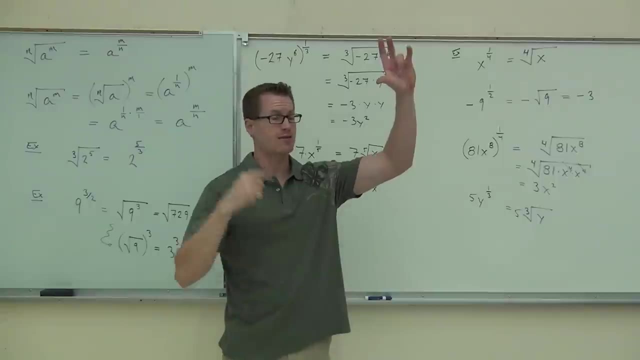 Yes, Okay, so maybe A shortcut. That's not even a shortcut. You're just doing one step. that I told you was true. If you do that step and move the power to the outside, if you have to do these in your head, 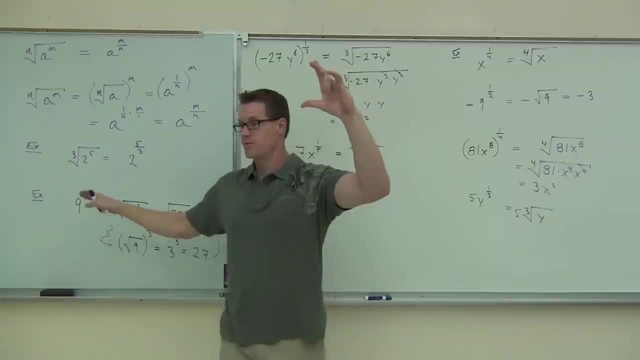 if you've got to do them in your head, the calculator will do this for you, no problem. But if you have to do it in your head, do the root before the power, if you can. You with me on that. Do you see why? 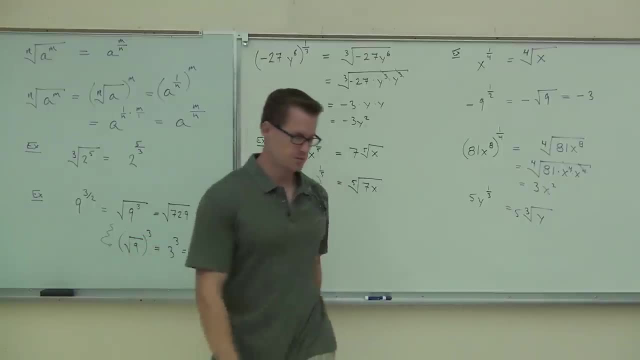 You don't want to deal with big numbers, right. Do the small numbers first. Most people don't want to do the big numbers right. They want to do the small numbers first. Most people don't want to do the big numbers right. 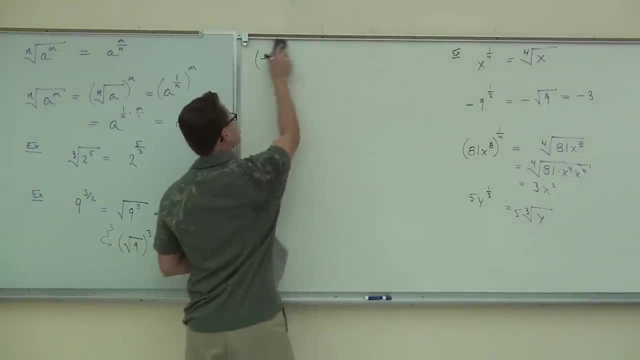 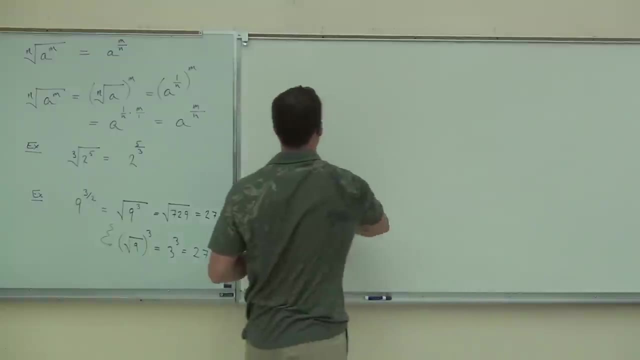 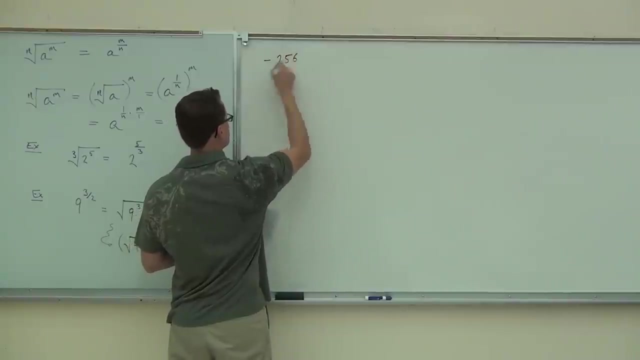 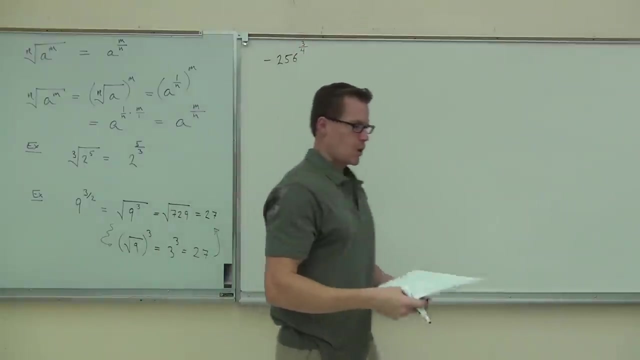 They want to do the small numbers first. Well, let's try a few more. Ultimately, I want you to be able to write the radicals very well, and then after that, I'd like to see you simplify them. But first step. 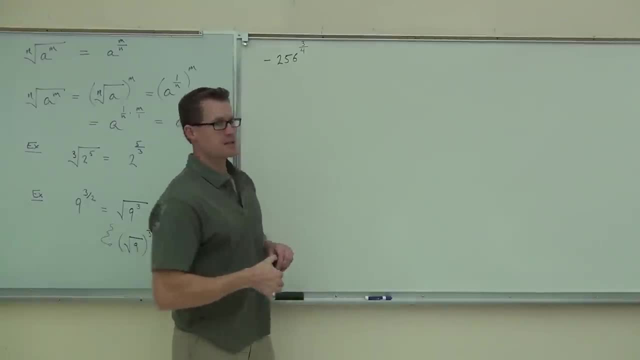 You've got to be able to write these correctly. So, everybody, what is the type of root that I have in this problem? Fourth root, Fourth root, great. Is the negative going to go inside the fourth root or outside the fourth root? 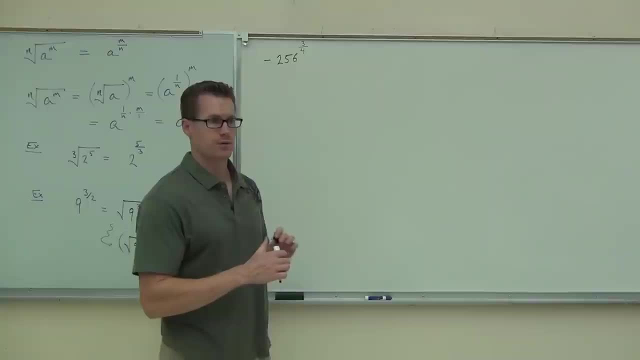 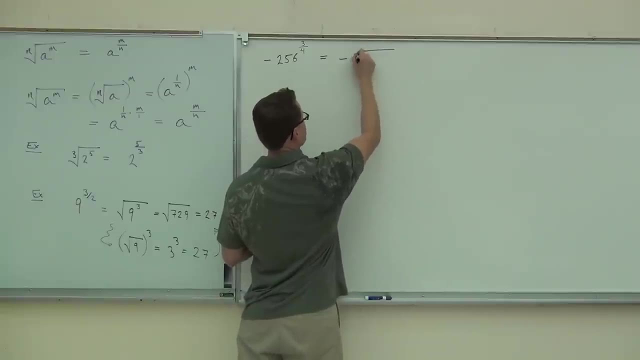 Outside Good, And do I have any power inside that root Two: Okay, So firstly, I want you to. I want to see you write it correctly like this: We definitely have a fourth root. Don't forget about that. four: 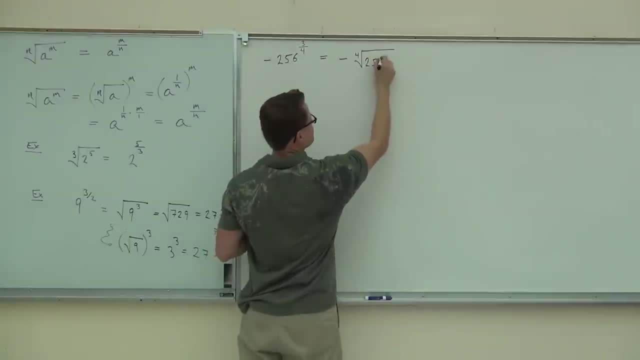 We've got a negative outside because it's not in any parenthesis. We have a 256 to the third power on the inside of the root. Not too bad. Two, You're okay on getting that far. Next, try to simplify it. 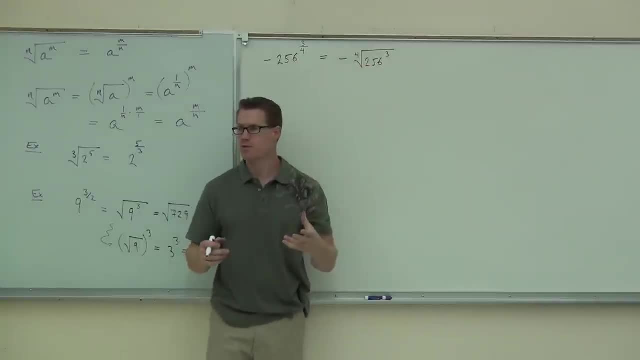 This is step one. I want to see that, that you're able to do that, because sometimes we're doing variables We can't just do. we can't do this process very well, So sometimes we're not going to be able to do that. 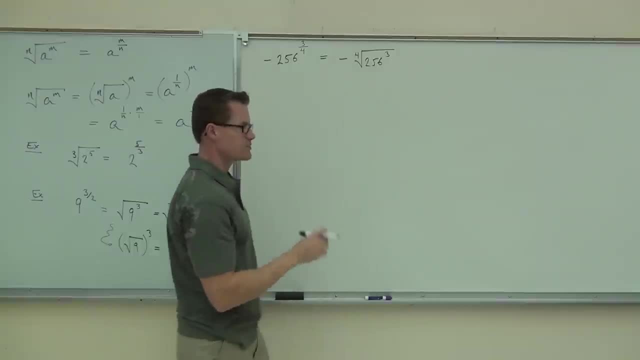 In this case we will, But firstly write it this way. Just make sure that you can. After that, do we want to take 256 to the third power first, or should we find the fourth root of 256?? You take 256 to the third power. 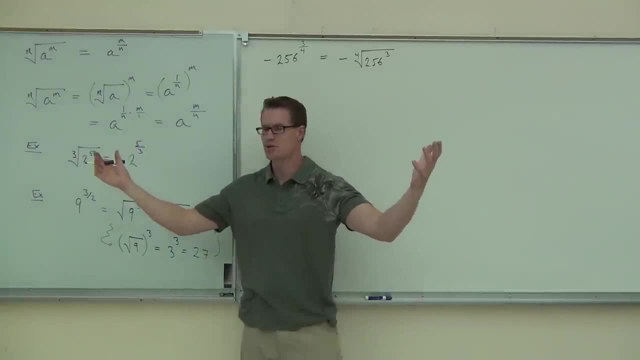 That's insane. That's a really, really big number. Right, That's huge. Instead, you could think of it as negative fourth root of 256 to the third power. like that. Do the fourth root first. Now maybe the fourth root of 256 isn't popping right into your head, but it does exist. 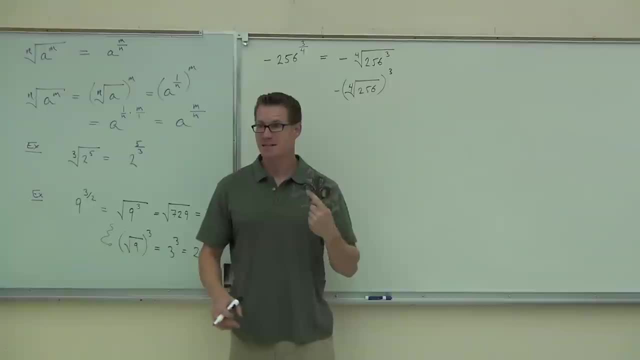 Say it now: Four. Well, it popped into your head, It popped into my head too. It did, It did. It popped right in there. I promise Whatever. Yeah it is, it's a four. So this would be negative. four to the third. 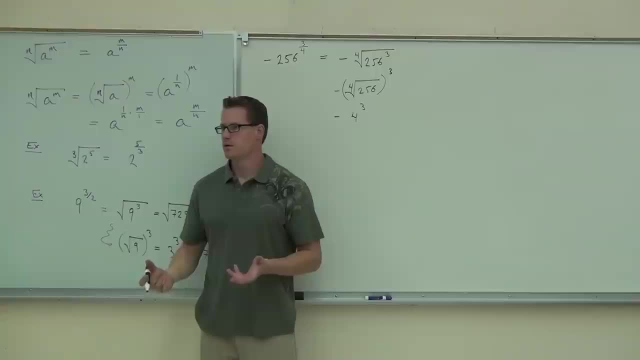 Negative. four to the third. What is negative? four to the third power? Well, we'd say negative. How much is four to the third? everybody, That's four times four times four. right, Four times four is 16 times four gives you 64.. 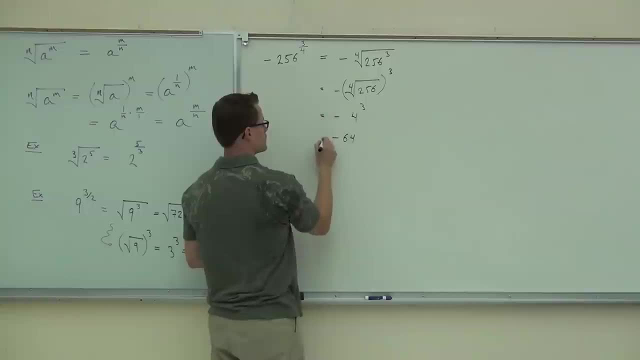 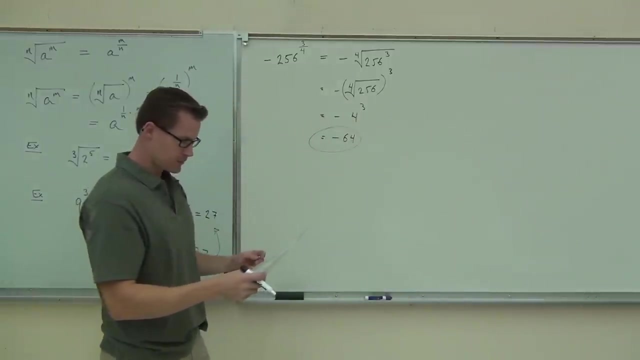 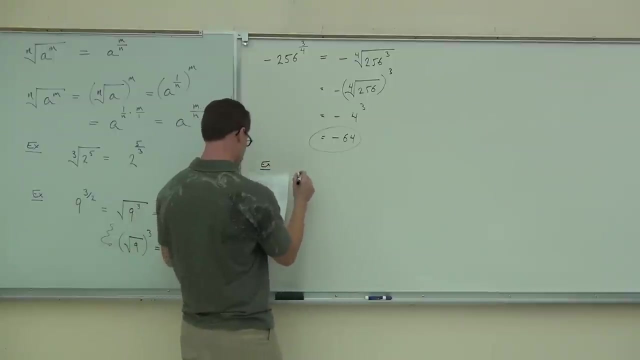 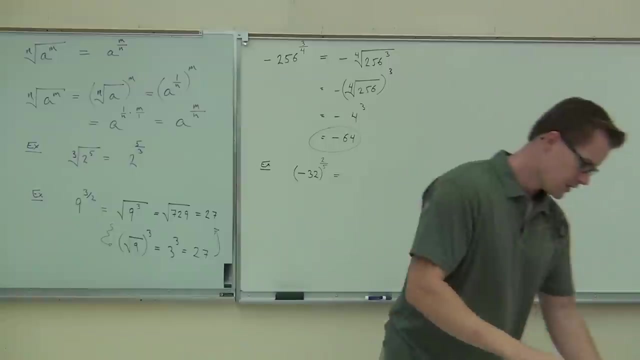 This is negative 64. So, step one: write the radical appropriately. Step two: try to simplify it. Let's do a few more of these things. Negative 32 to the two-fifths. We're going to go kind of quickly through this, because we should have the root down. 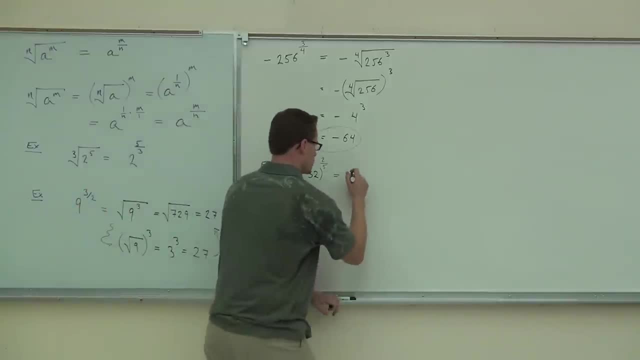 at this point. What type of root do we have, folks? Fifth, Good, So I'm going to have a fifth root. Is the negative inside or outside of the root, please? Inside, Inside, So I'll have negative 32.. 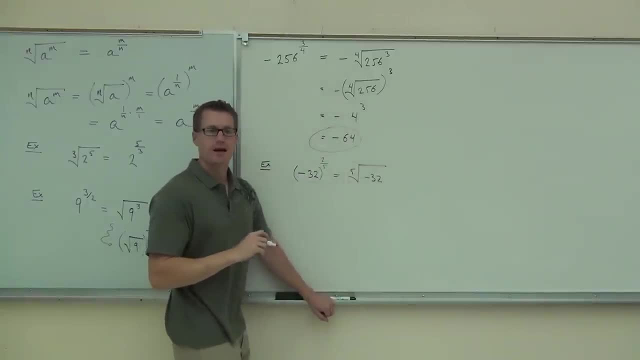 In fact, do I have a power? Second power, Second power. Now, because this was in parentheses, I want you to watch up here on the board. Please watch, I'm not just going to put a two there, Right there. that two would not be applied to negative 32.. 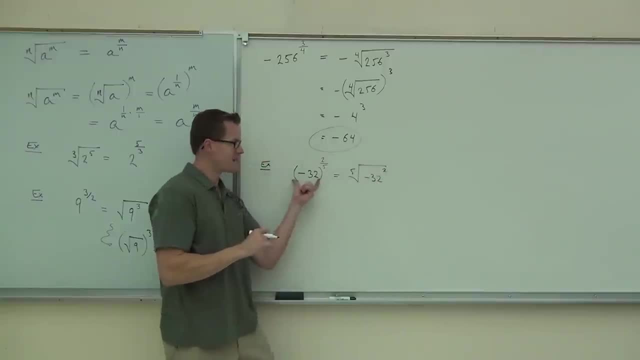 It would just be 32 and you would take the negative. Are you with me on that? Because this had a parentheses. it really is a parentheses like that. That changes, It changes. It changes the problem a little bit. This is going to make whatever you have a positive number. 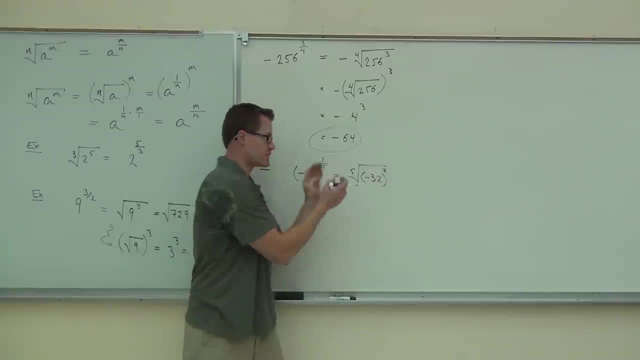 Are you with me? That's what that does, So you need that parentheses. If you have one here, you also have one there. Nod your head if you're with me. Okay, Good deal. Now we could square negative 32 and then take a fifth root, or you take a fifth root. 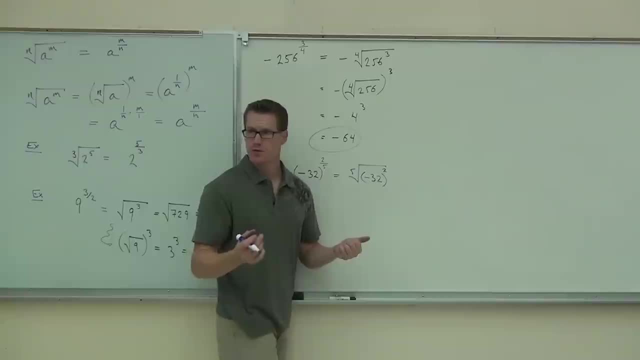 and then square. whatever you get out of that, I'm going to choose to take the root first. So if I take the root first, what I'm doing is a fifth root of negative 32 and then squaring it. Can you tell me what's the fifth root? 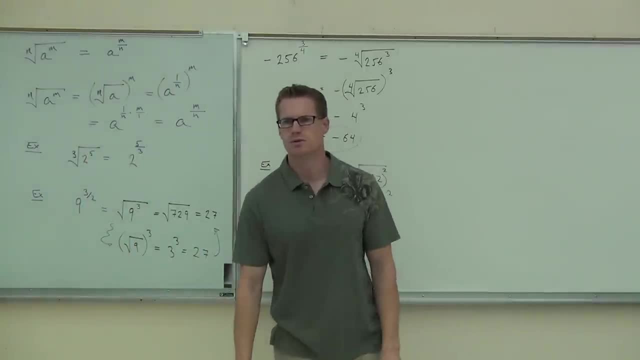 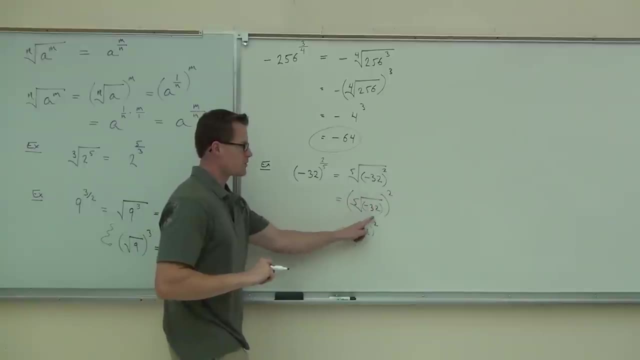 The root of negative 32.. Negative 2.. Negative 2. Okay, I have negative 2 and then I'm squaring that number. Remember, I'm doing this part first, I'm doing the fifth root first and then I'm squaring it. 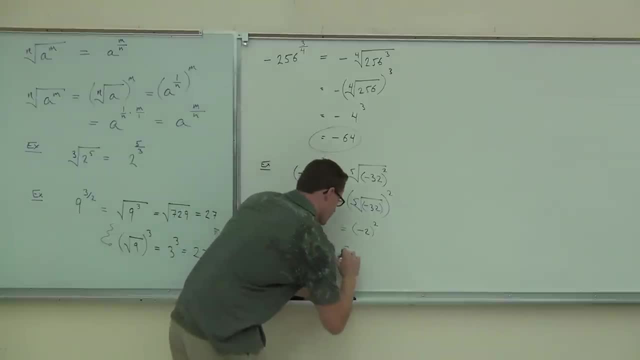 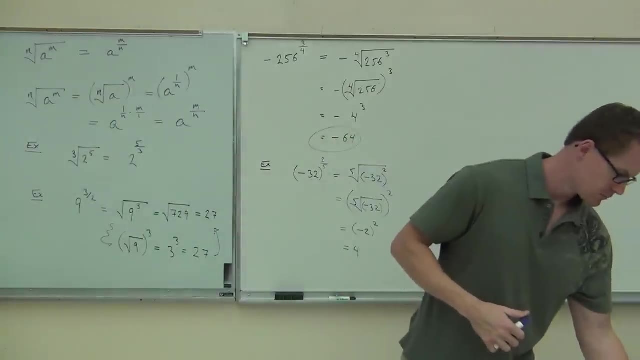 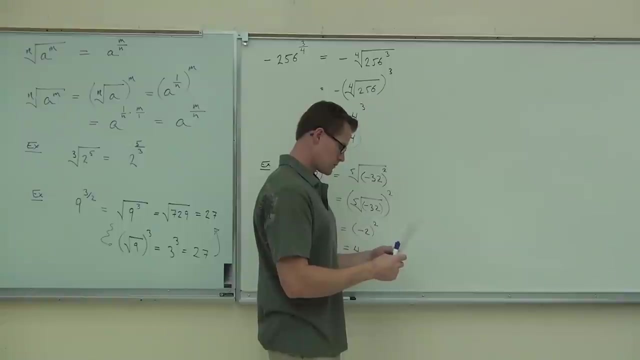 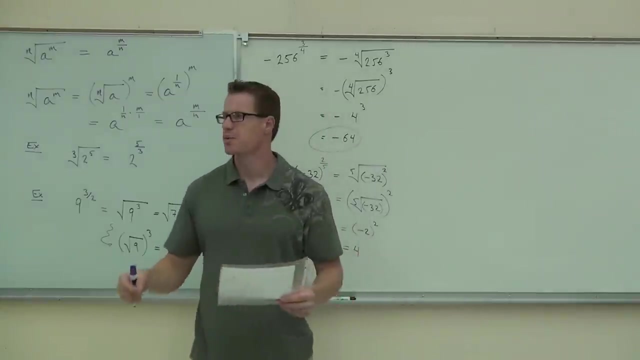 It's negative. 2 squared folks, That's 4.. That's 4.. Okay, let's try a couple more together. give you one on your own, then we'll move on to some negative exponents. look what happens there. 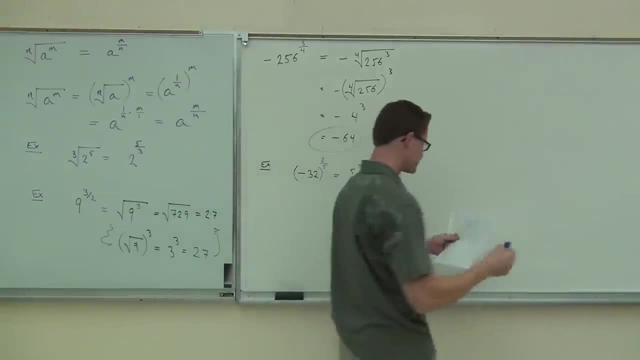 and after that we'll talk about some exponent rules to refresh your memory a little bit. Okay, you knew this was coming right. We're dealing with fractional exponents. How would a fraction to a fraction? you're crazy, Leonard, come on. 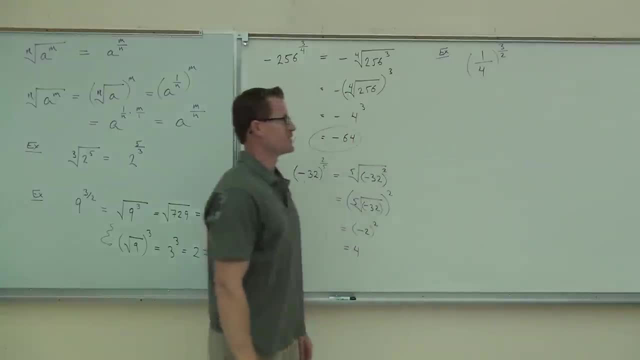 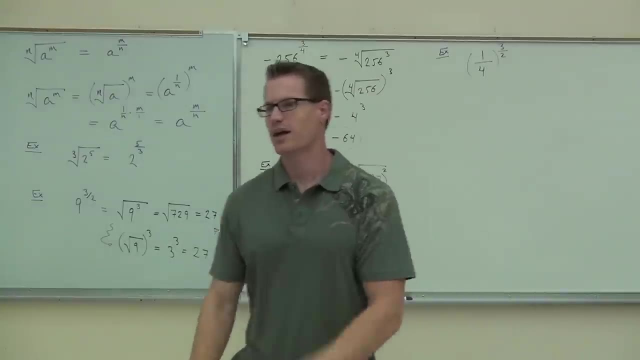 what are you doing to me? a fraction to a fractional exponent? I didn't know, this was a math class. come on, it's only 735,. my goodness Yeah, what about a fraction to a fractional exponent? My goodness gracious. well, what we know about fractions is that we take the top. 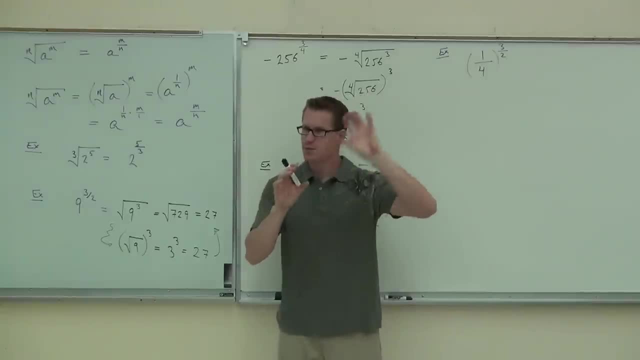 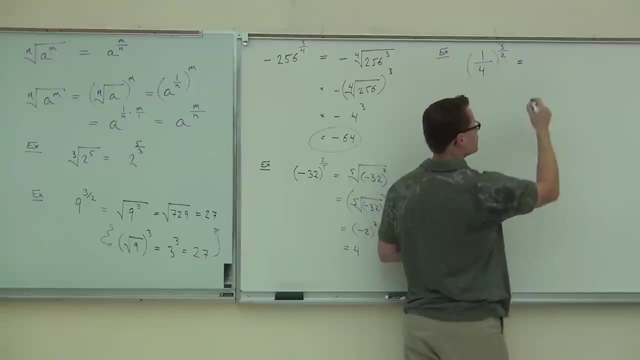 to that exponent and the bottom to the exponent, numerator to that power and the denominator to that power, and we solve the right thing. So you could go about and you could write this as: what type of root, A square root of one-fourth to the third? that's appropriate. that's appropriate. 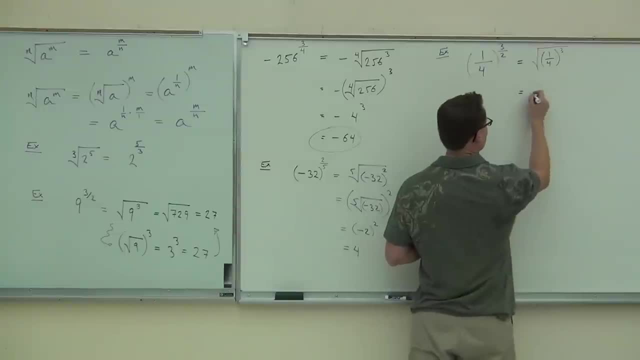 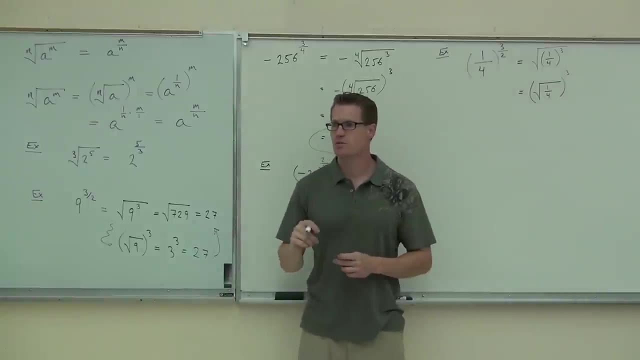 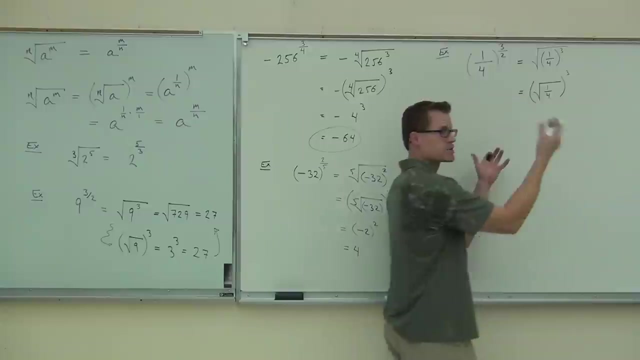 Well, what that means is that you have a square root of one-fourth to the third. that's okay too, right? Can you take the square root of one-fourth, how much is it? Okay, so this process still works with fractions. no big deal. 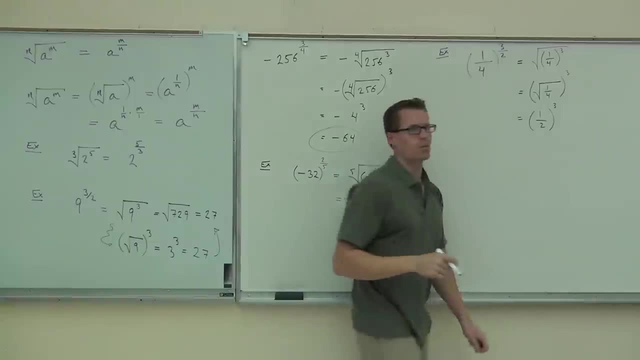 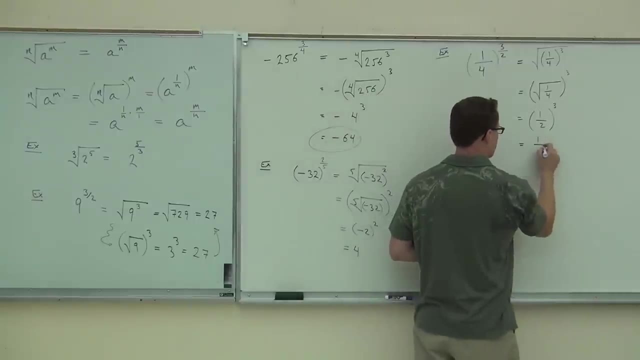 We're going to have one-half. then take that to the third power. we can do one-half to the third power. take the numerator to the third, take the denominator to the third. what's that fraction? One-eighth, that's it. so, even though we have, we have some fractions. 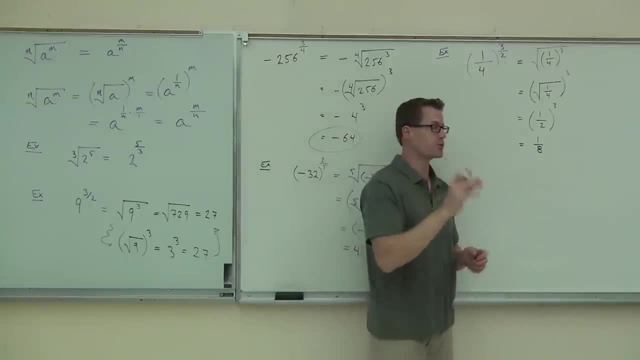 it's no big deal. the same process works. We still know it's power over root. Whatever root we have, this is going to be on the denominator. Whatever power we need is going to be on the numerator. Write it out appropriately and then use what you know to simplify it. 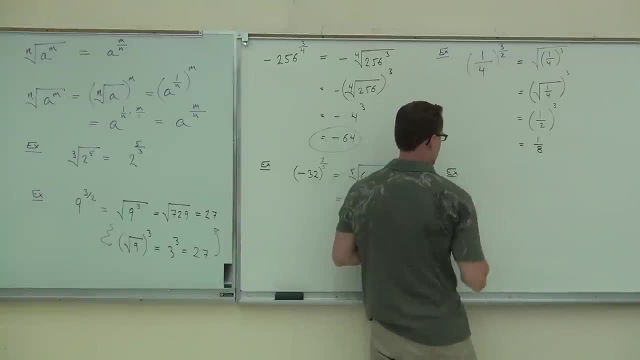 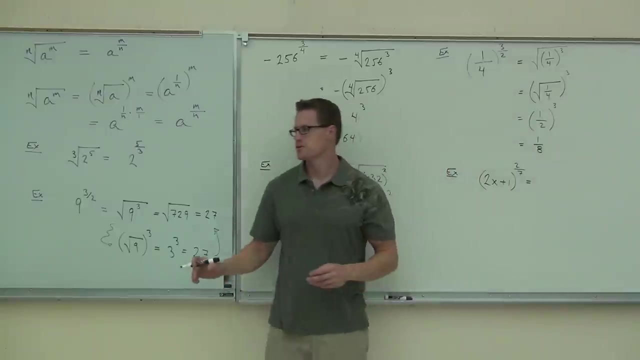 Okay, one more before I let you go and do one on your own. Let's say we have two x plus one to the two-sevenths, two x plus one to the two-sevenths power. ladies and gentlemen, what type of root do i have here? 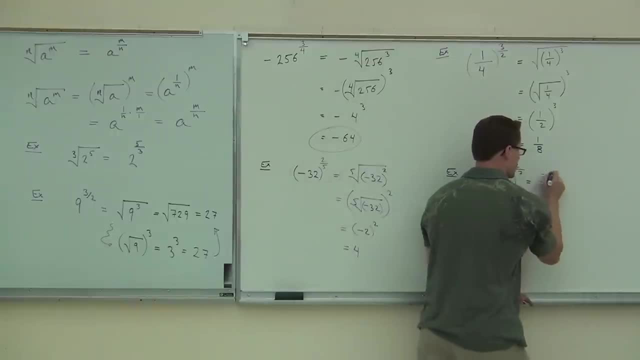 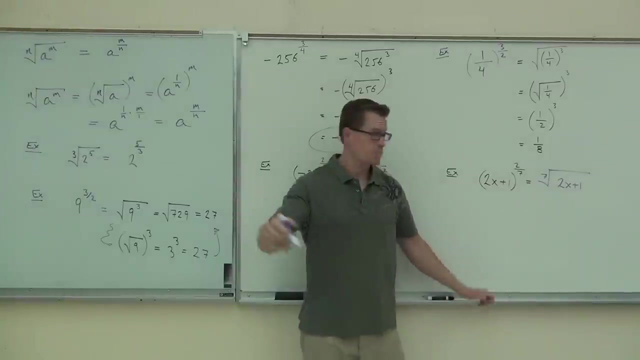 and it's all in parenthesis. so everything is going to be on the inside of that seventh root. what is going to be on the inside of that seventh root? do i have any power associated with that parenthesis? because, well, this was in parenthesis and it's being squared. 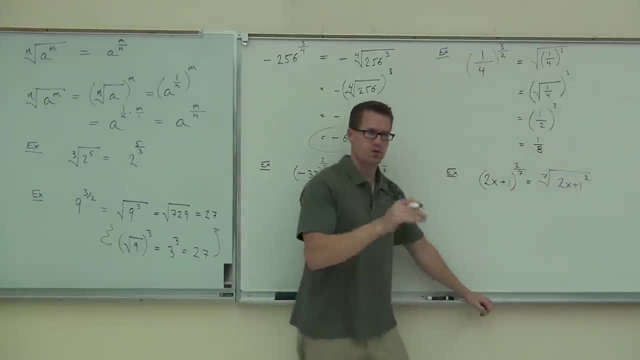 so i can't just do this. that doesn't make sense. right, that's just squaring the one. what i want to show is that the whole thing is being squared. put some parenthesis on that thing. you can't simplify this one. it's not like the other ones. i mean, if i say okay, 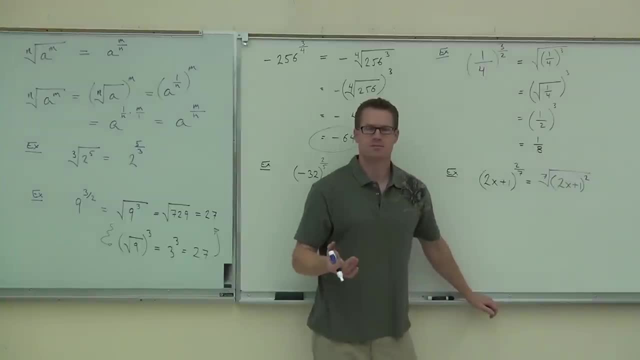 find me the seventh root of two x plus one. you're going to go: well, what's x? so we can't do anything with that? it's not like the numbers. numbers, yeah sure, we can just simplify those down once you get the variables. really, there's only a select few things we can do, which is kind of nice, i guess. 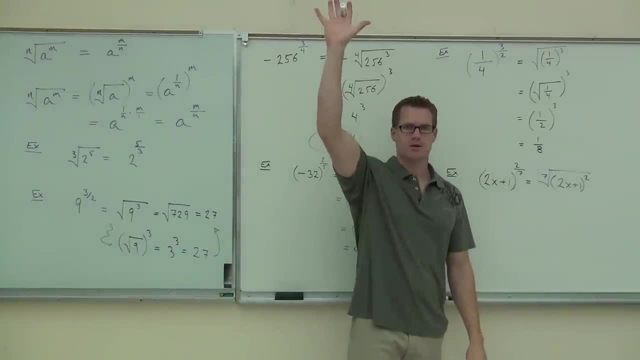 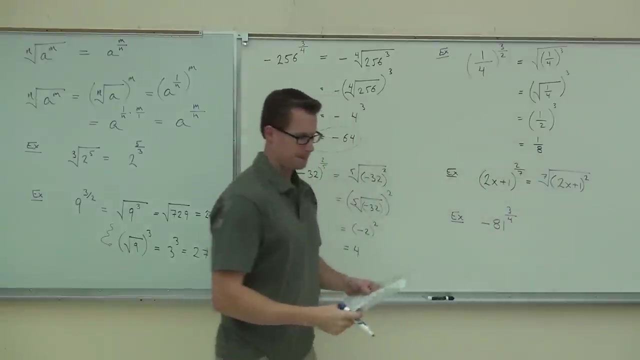 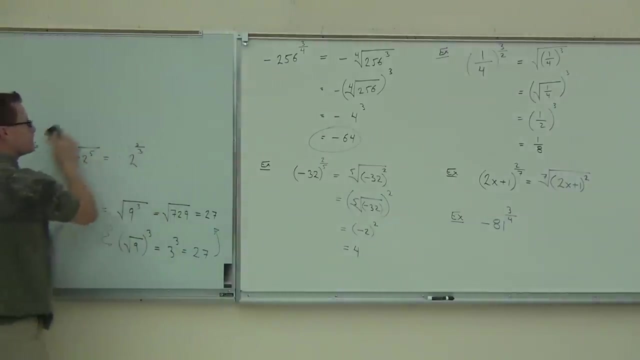 that you're done at this point. raise your hand if you feel ok with what we've talked about so far, good deal. i want you to try one of these on your own. let's do: negative eighty-one to the three-fourths. negative eighty-one to the three-fourths. 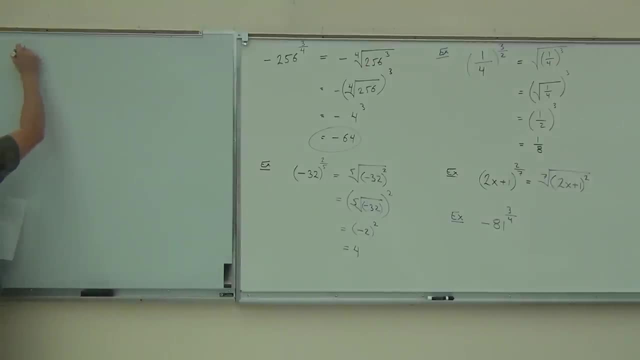 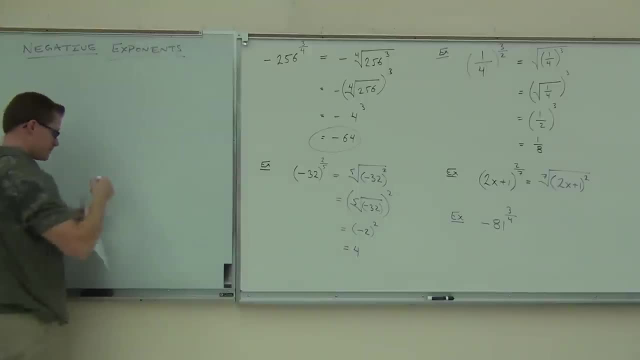 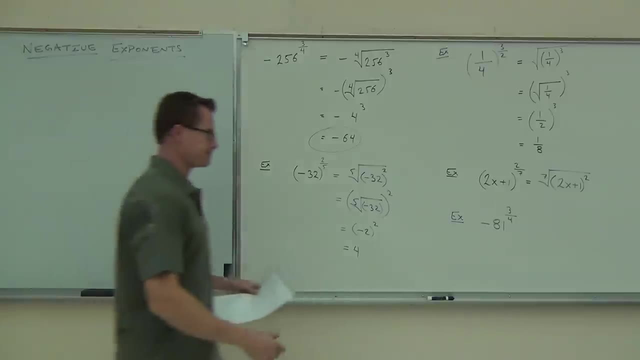 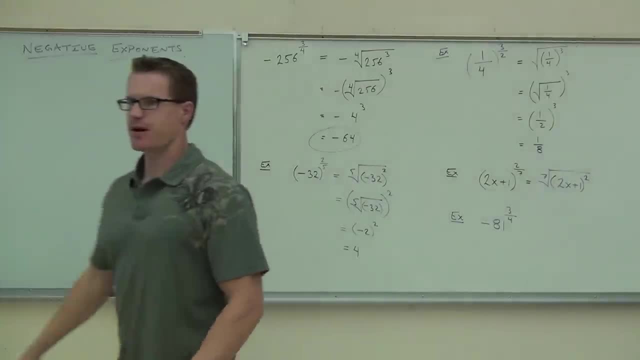 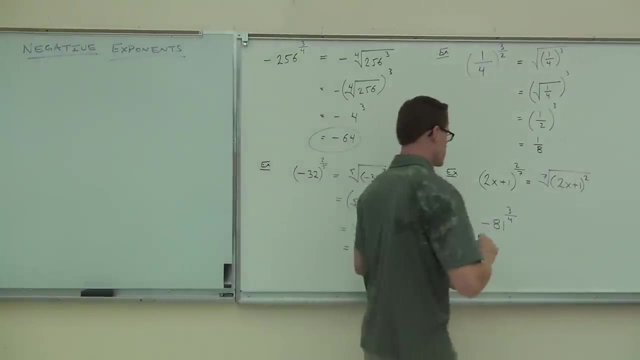 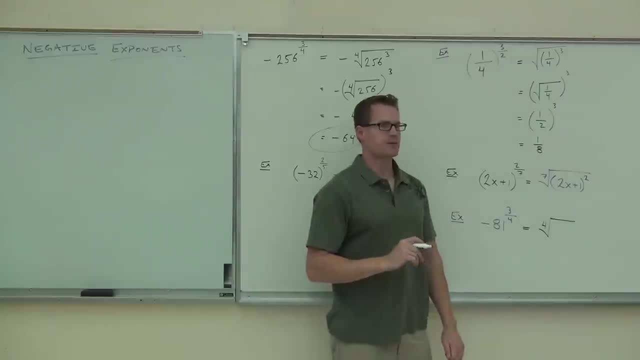 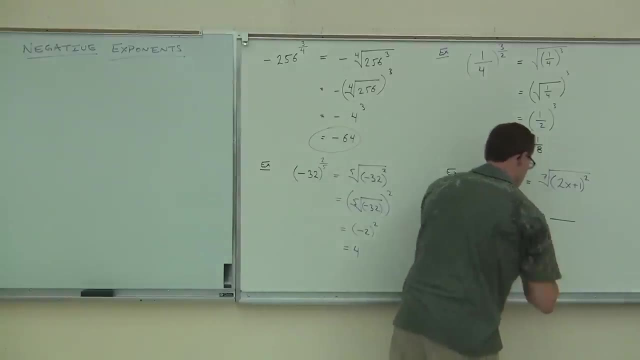 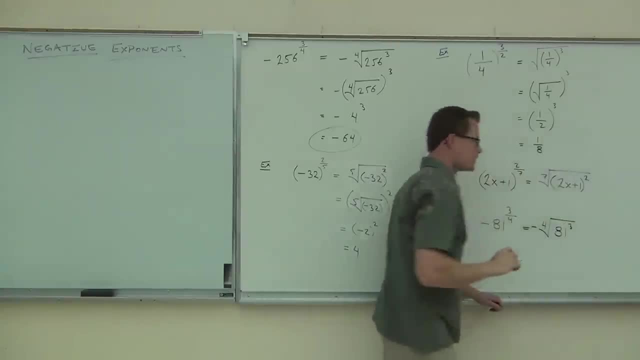 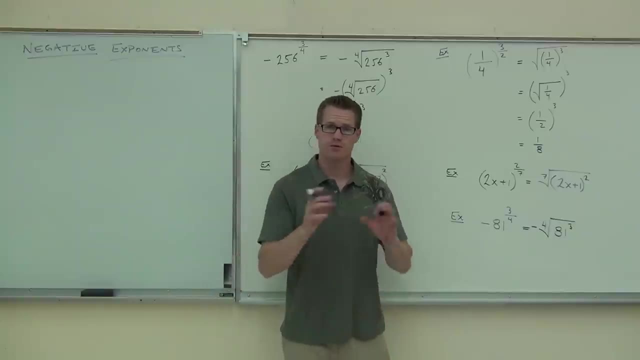 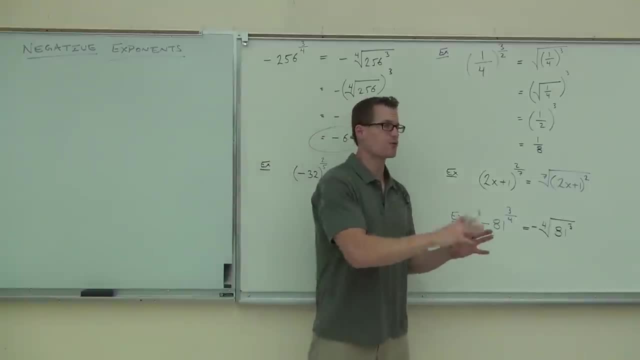 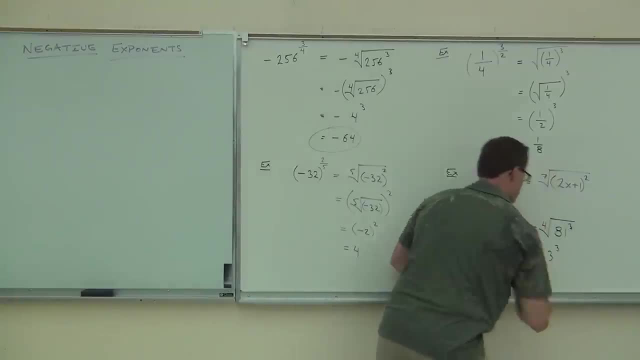 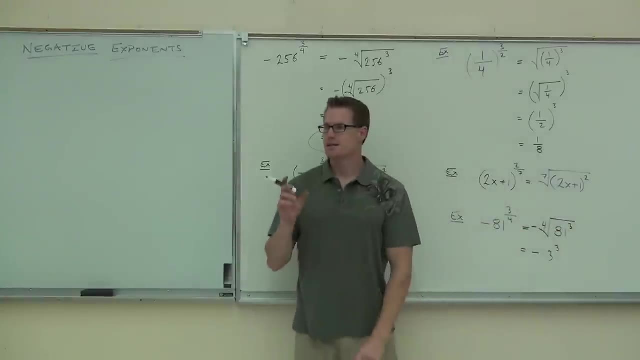 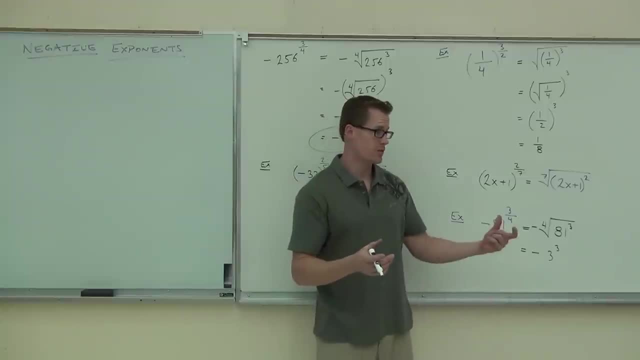 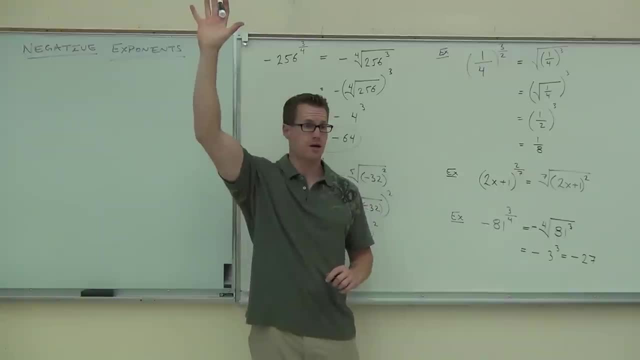 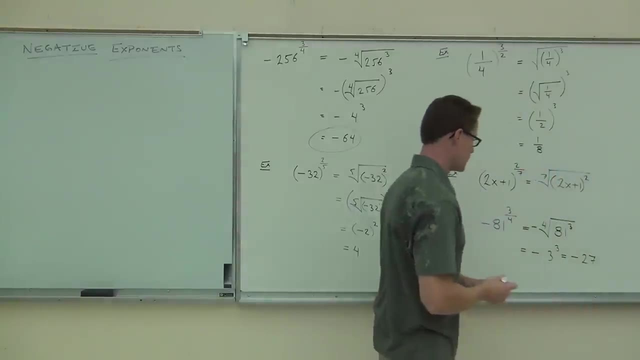 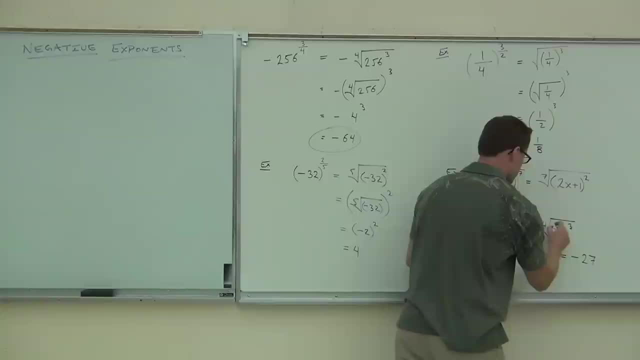 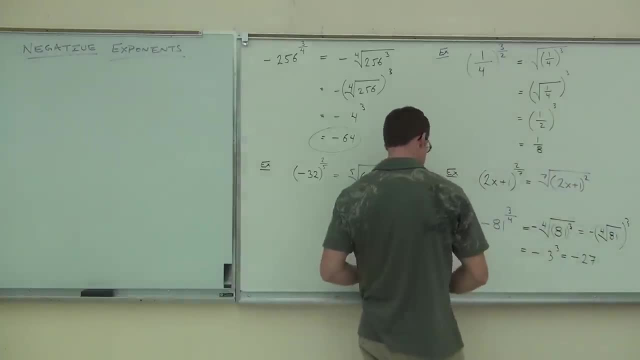 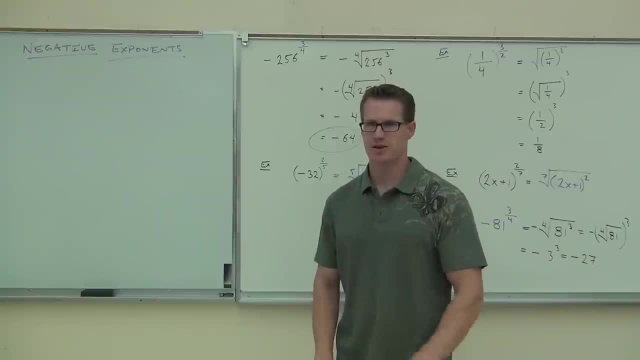 Remember I gave you those problems where it was like complex fractions. We had like x to the negative 1, and we had 3y to the negative 2, and we did some crazy stuff with it and then it was like a 10-step problem. 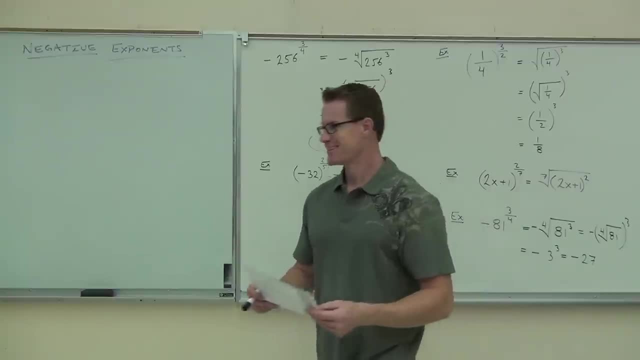 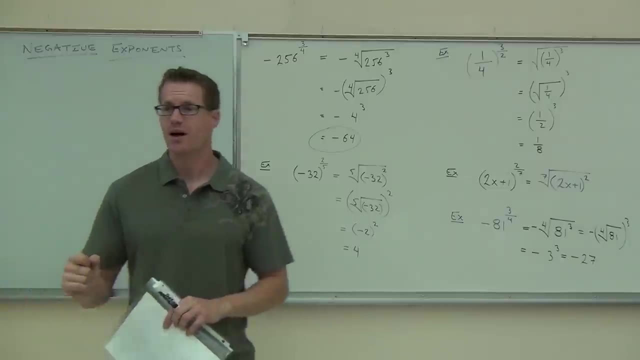 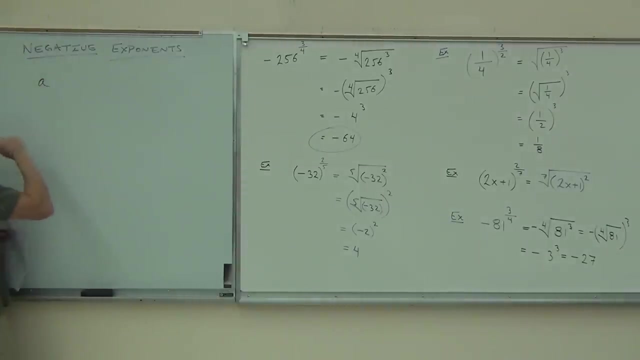 Remember those? Those are super fun, right? Obviously, Yeah, Well, we can still deal with negative exponents, even if we have some rational exponents. So negative fractional exponents, let's do it. If you remember, a to the negative 1 was the same thing. 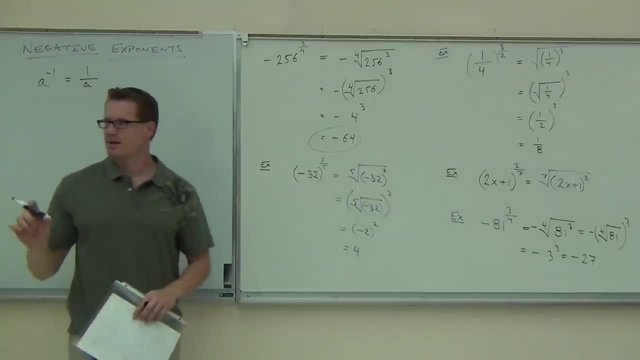 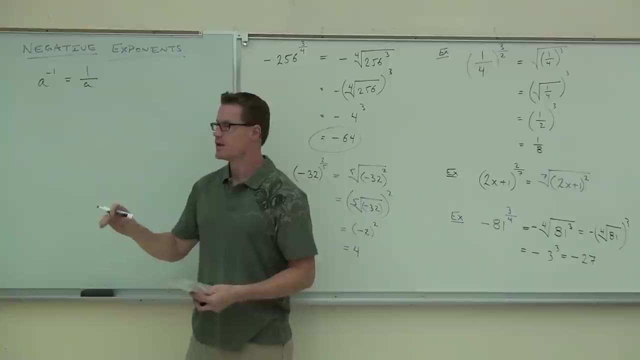 as 1 over a. Do you remember that That when we have a negative exponent, the way we change it to a positive is just put it on the denominator fraction or essentially change it? change the position where it's at, If it's negative, on the numerator which it is here? 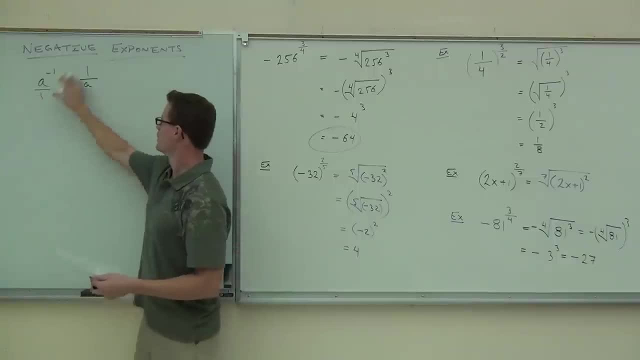 remember. this is like a to the negative 1, over 1, we move this to the denominator. That's what we would do. We would spend a lot of time doing that. The same thing happens if I have a to the negative m over n. 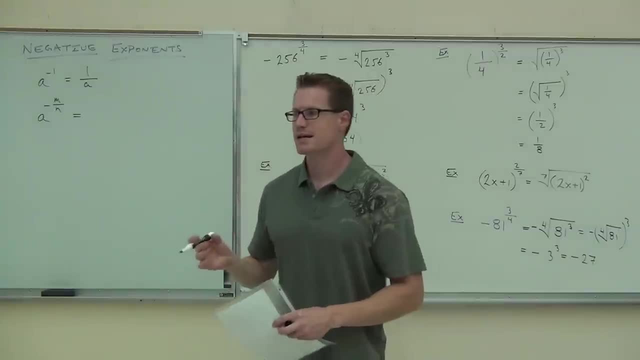 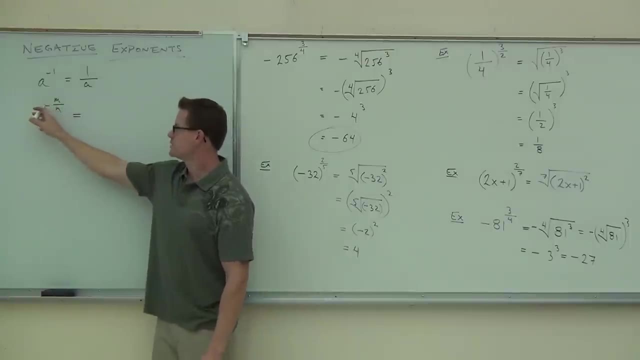 If I have negative m over n, what that says is I have a negative exponent. Let me be real clear here. This negative has nothing to do with the sign of the number. Nothing to do with that. This answer does not have to be a negative exponent. 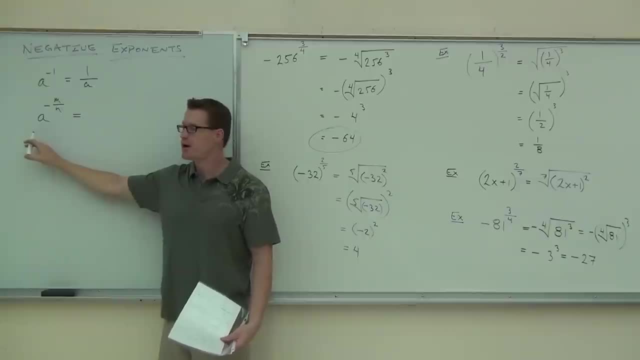 This doesn't have to be a negative when you're done, Not just going to be okay with that. This doesn't have to do with the sign of the number. This just says that this is in the incorrect position. This is on the numerator when it should be on the denominator. 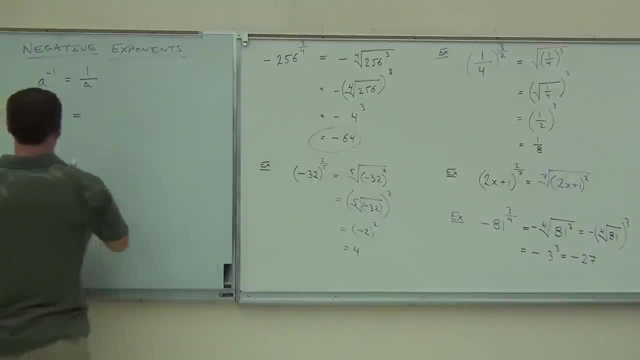 okay if you want to make it positive. So what this says is all right. if I want to change my exponent to a positive, I'm going to have to move this from the numerator like it's on to the denominator. I don't flip anything around. 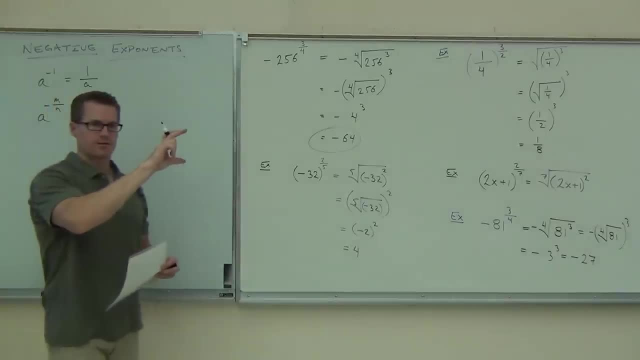 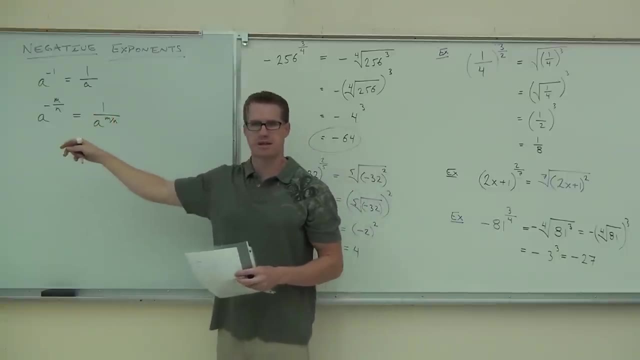 I don't change the exponent. I'm changing where that expression is. I'm changing where a to the m over m is. Don't flip the fraction around. You're not. that's not the. that's not the thing. We're just changing the sign of that exponent by moving it. 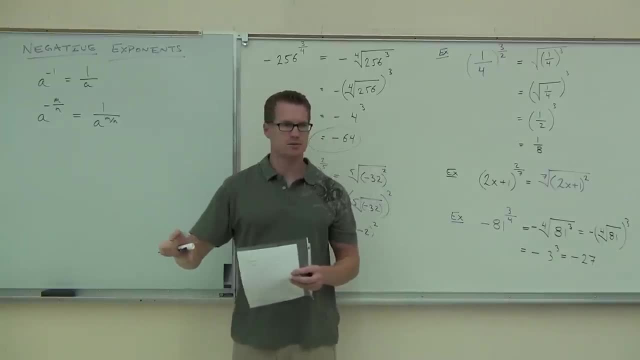 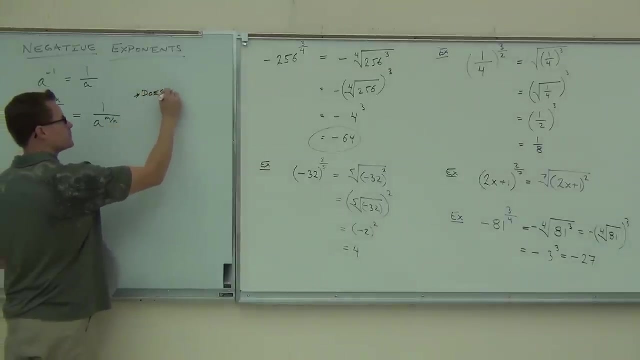 from the numerator to a denominator. You okay with that? Very, very similar to this idea. So make a little note here: This does not affect the sign of the number, It's just the sign of the exponent. Okay, let's try a few examples. 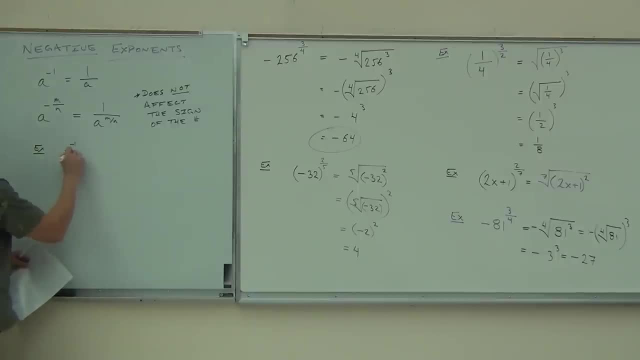 Let's do 3 to the negative 2.. If I want to change 3 to the negative 2 into a positive exponent, what do I have to do? What do I have to write? Okay, good, So I'm changing. this is like a denominator. 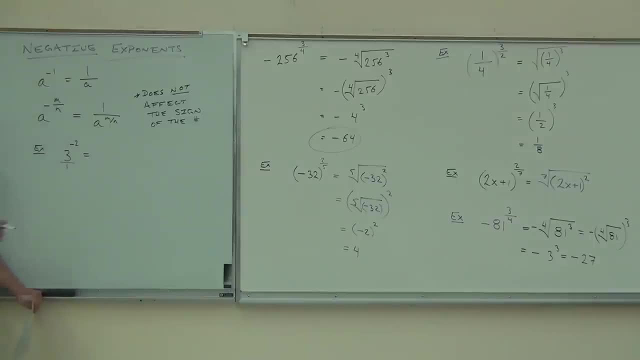 or this is like a numerator right now, Like 3 to the negative, 2 over 1.. So if I'm going to make this into a fraction where this is a positive exponent, I'm going to move this from the top our numerator to our denominator. 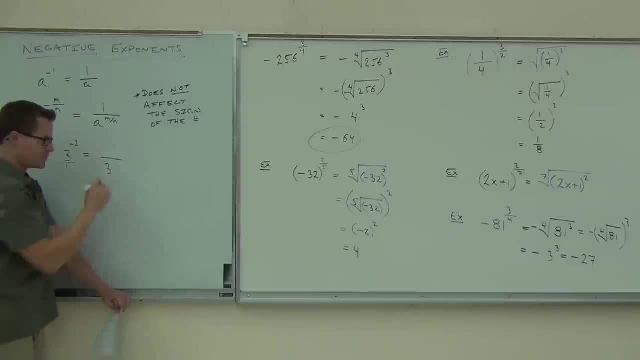 So that would be 3 to the. is it still going to be negative 2?? No, it's positive 2.. Okay, Did it change the sign of my number? No, So it's just my exponent. but what's going to be? 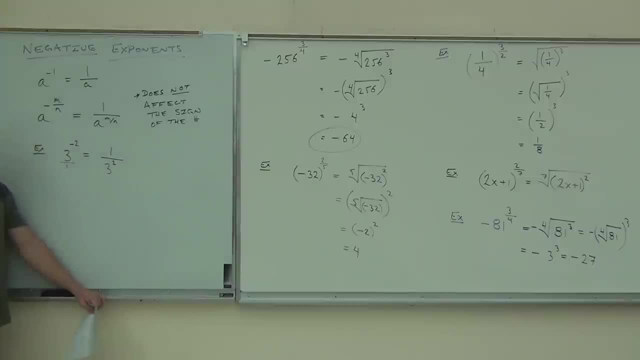 on the top of my 4? My fraction 1.. By this rule, move it to the bottom of the fraction. change the sign of your exponent. How about that? How about 9 to the negative 1 half. 9 to the negative 1 half. 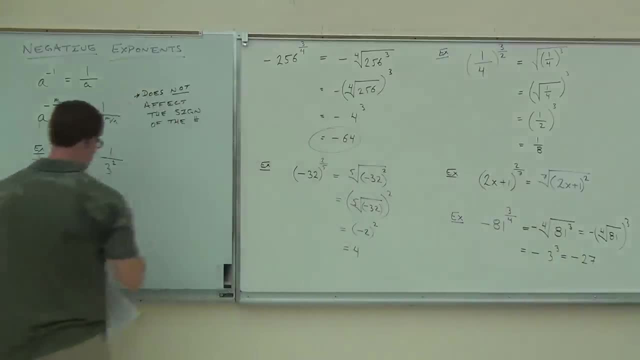 Can we write that as a positive exponent? Firstly, what's going to be on the numerator of our fraction here, ladies and gentlemen? 1. Good, Are you guys all still with me on this? Why do we have a 1 there? 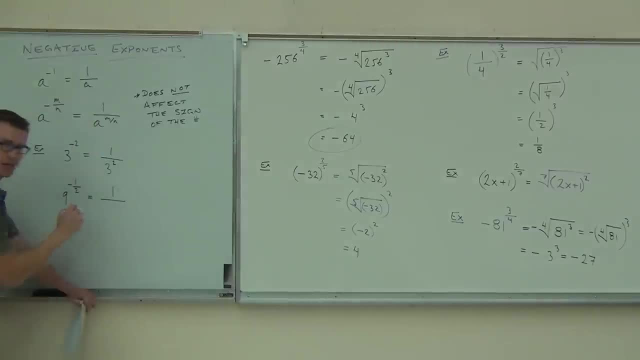 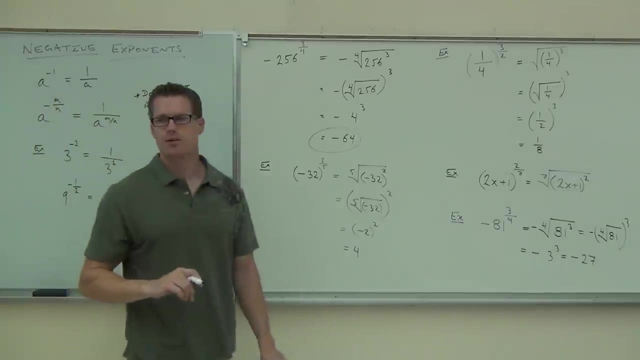 What's on the denominator of our fraction? Do we still have the 9?? Yeah, the square root of the exponent. Okay, we're going to have a positive 1 half. We're going to change the exponent to a positive. Can you deal with 9 to the 1 half? 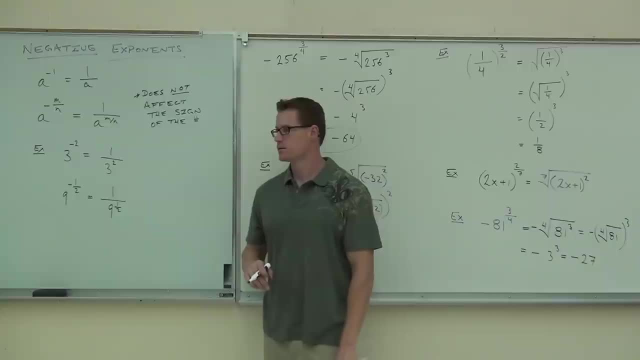 What's 9 to the 1 half mean The square root of the 1 half is 1.. Okay, So yeah, the 1 is going to be there. We're good at this, right. This says what type of root. 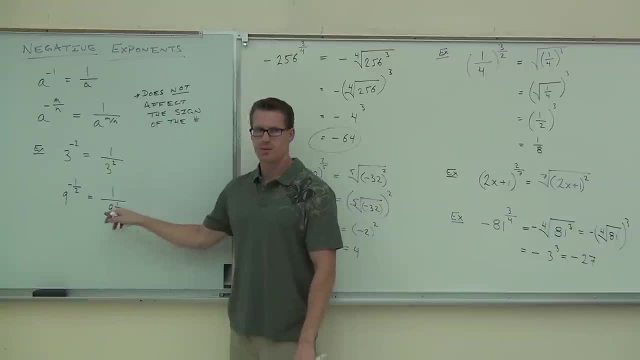 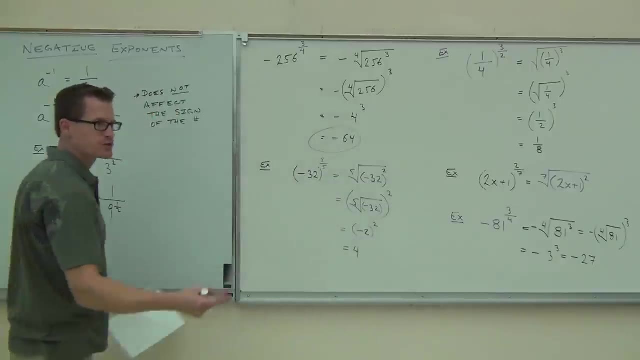 Square root of 9 to the First power. What is the square root of 9 to the 1st, 9 to the 3.. You can change it to a square root if you want to, or if you're getting good at this, just go right to 3.. 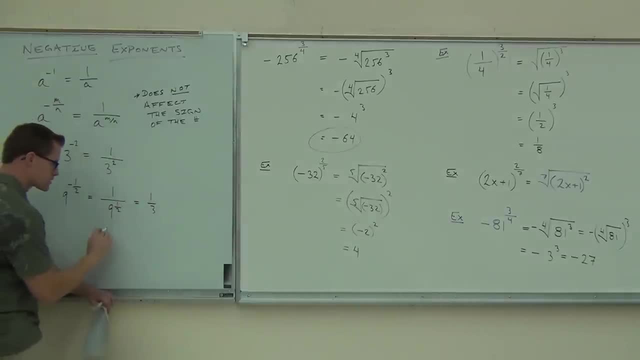 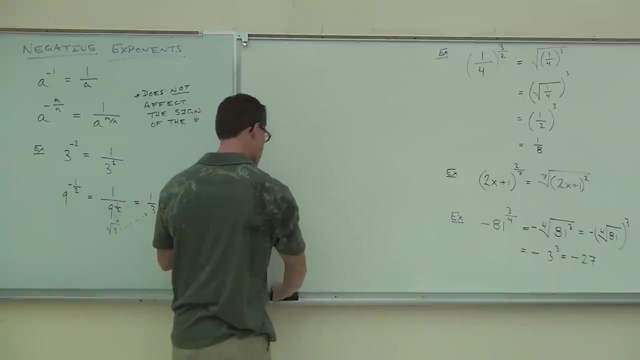 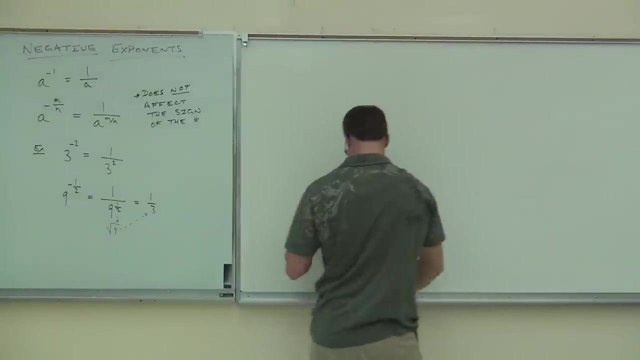 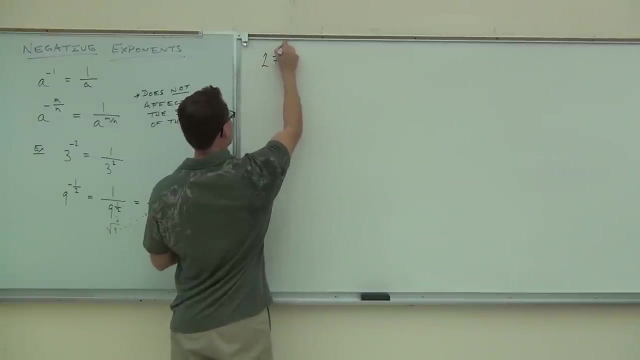 This same thing is 1 third, because this right here is the square root of 9 to the 1st. Let's do a few more examples and we'll call it a day. Okay. 27 to the negative: 2 thirds. 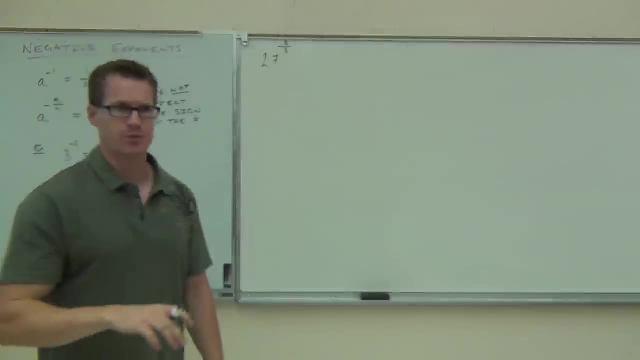 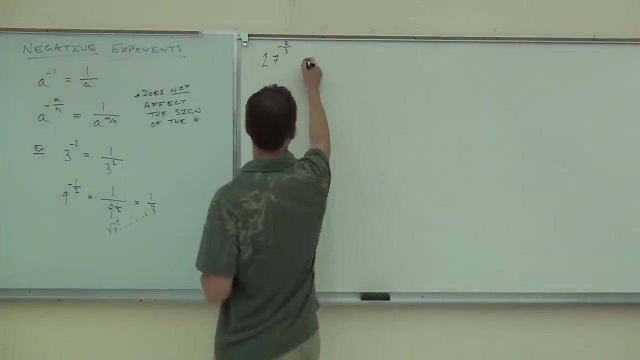 First thing we're going to do is make that exponent into a positive. I want you to do that right now on your paper. Make the exponent into a positive right. What you need to do. We should get a fraction somehow. What's on the top of our fraction, folks? 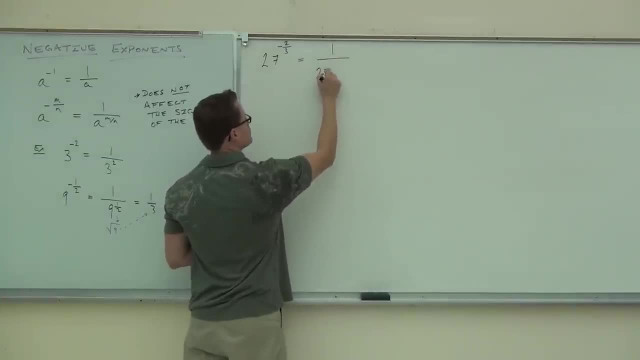 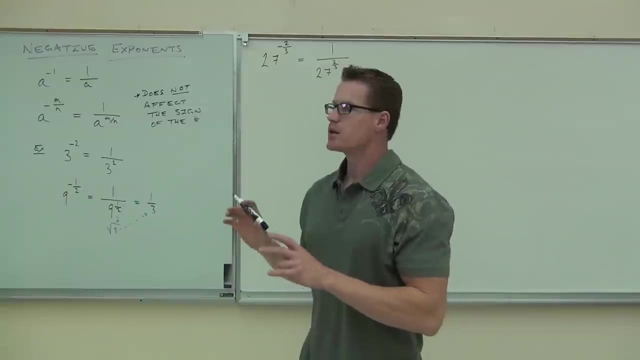 Good, What's on the bottom of our fraction, please? Good, All right, Did you make it that far? Now, once we've done that, we have the positive exponent. Now we can use what we just learned and simplify the thing. 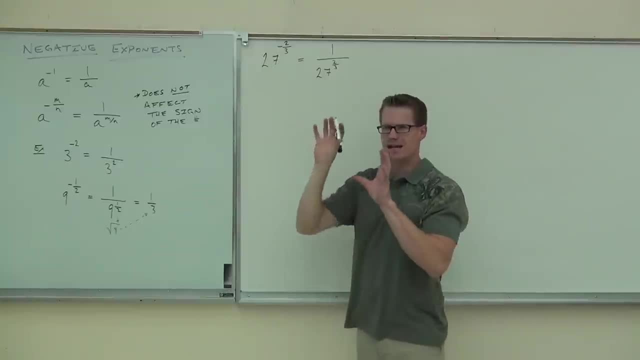 You can't really simplify here. It doesn't really work. We don't know how to deal with a negative exponent. We don't know how to do it. It's a negative version of a root. What that means is: okay, just move it to the denominator of a fraction. 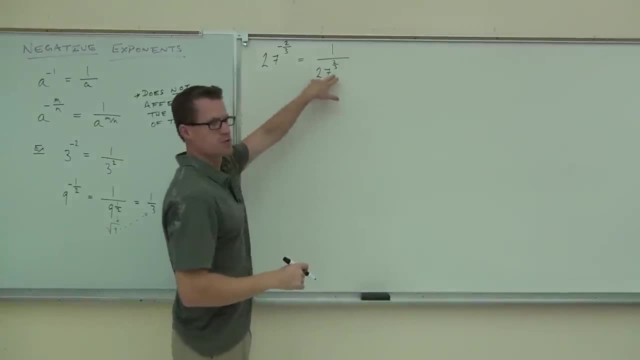 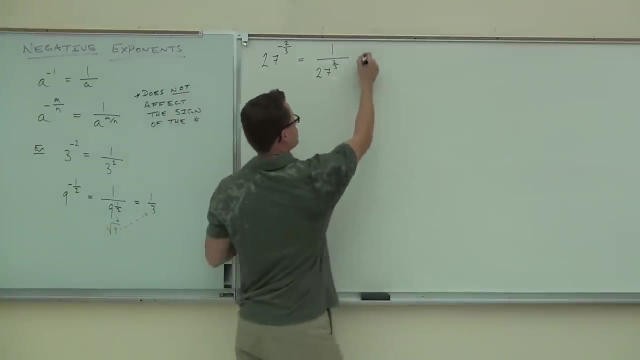 That's really what it means. So here can you simplify: 27 to the 2 thirds. What type of root do you have? Cube Cube root. What type of power do you have Second? So what this means is 1 over a cube root of 27 squared. 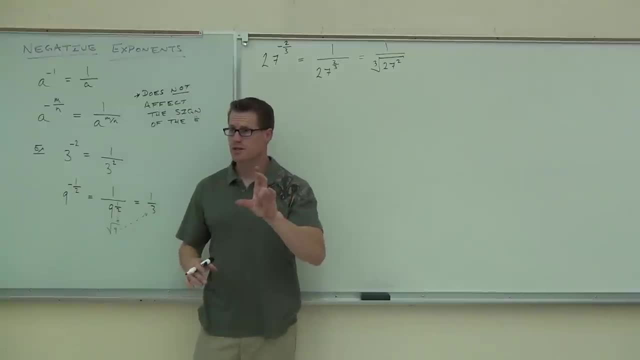 We've already done that. That's what we just learned. So you could square the 27 first, or you could cube root the 27 and then square it. I'm going to choose to do that way. Can you think of? think of on your own, don't say it out loud, just think of on your own what that's going to be. 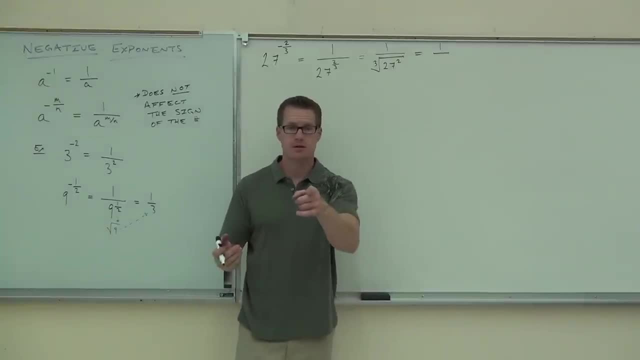 What do you think it's going to be? How much 9.. Yeah, it's going to be. the cube root of 27 is 3.. Then you square it, you get a 9.. Nigel, are you still okay with that? 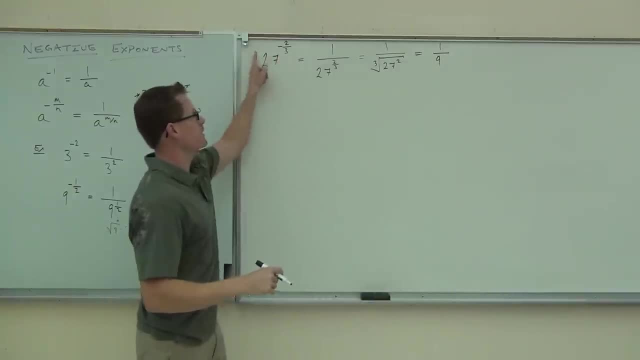 So we're going to get 1: 9.. It's kind of interesting that this whole ugly thing is actually equal to 1: 9, isn't it? It's kind of weird. Much easier to write 1: 9.. Why don't we just do that? 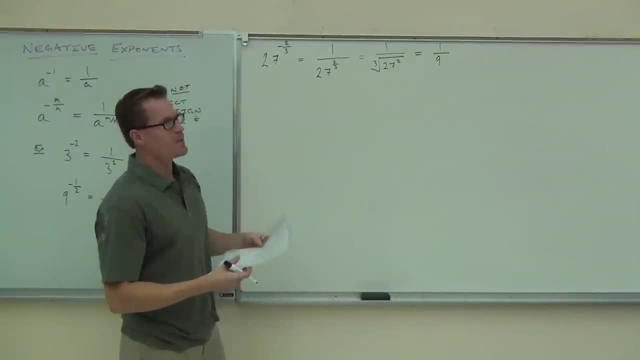 Make it that complicated. It is right, It's complicated. The problem is, you get this a lot. You get this type of stuff a lot in math. We have to know how to simplify it. All right, Let's do. let's do one more. 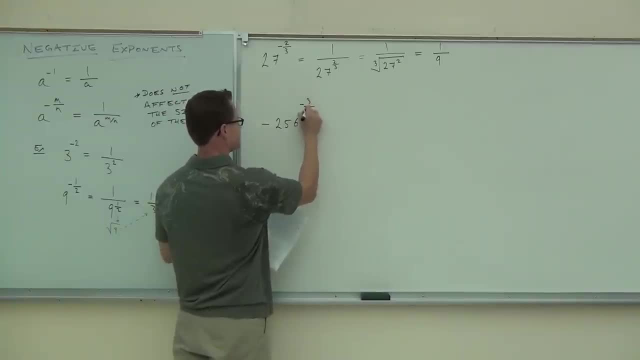 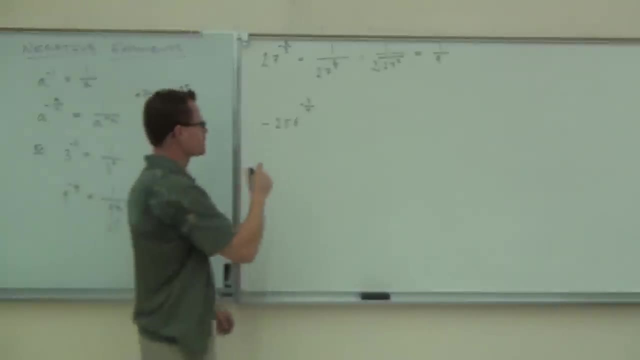 Yes, let's. Here's what I need you to know. I'm going to show you this example for one really good reason. What am I trying to change? Am I trying to change the first negative or the second negative, The second negative? 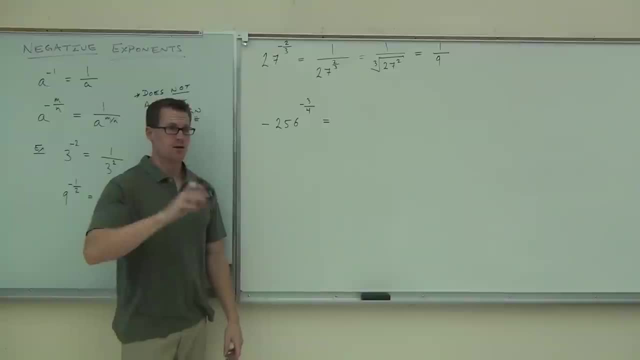 Will I ever be able to change the first negative? No, Not by moving it. So when you do this you go: okay, yeah, I have 1 or a negative 1.. I don't really care what you put there. 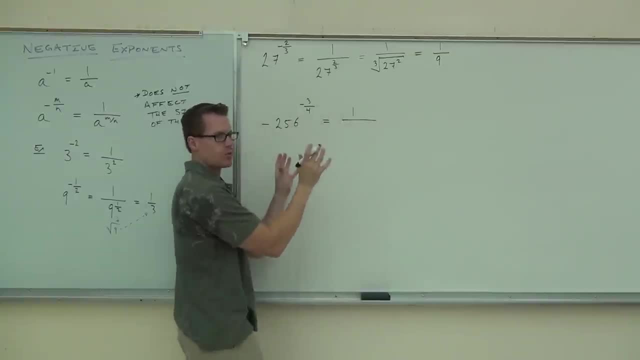 But on the denominator I have to have. I have to have that negative somewhere. I'm going to carry it with this 256.. I have negative, The negative 256 to the positive 3 fourths. I need you to notice that, yes, the sign of the exponent changed. 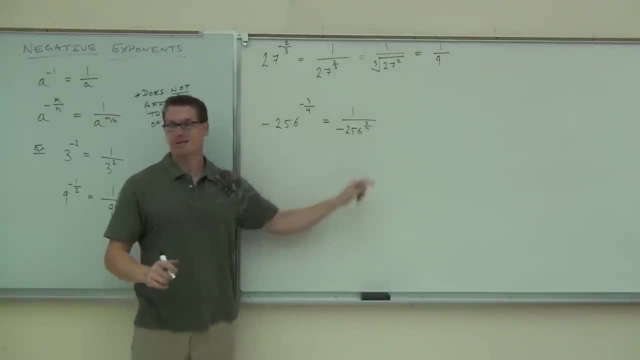 That's what we're doing. The sign of the number did not change. It doesn't affect the sign of the number. Now, we've already done this problem. In fact, it was on the board, I just erased it. Does this negative go inside of the fourth root that we're going to have? 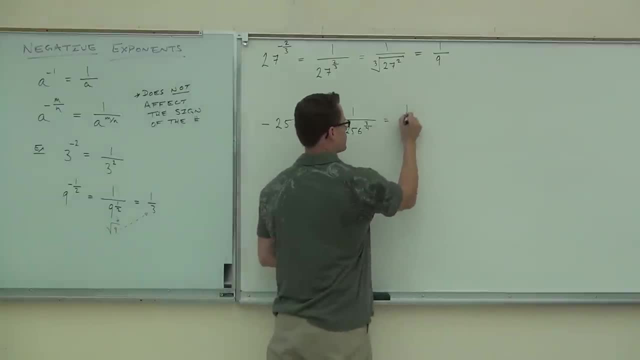 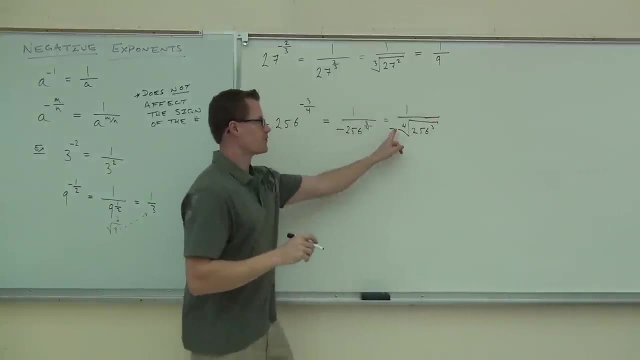 or outside of the fourth root, Outside of the fourth root. So we're going to have 1 over negative fourth root of 256 minus the negative 256.. All right To the third. we've actually already done this problem. The fourth root of 256, do you remember what it was? 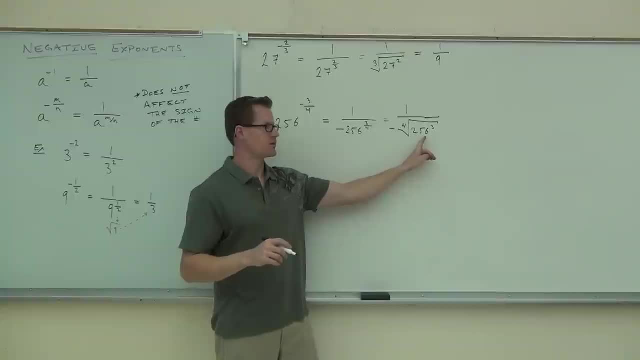 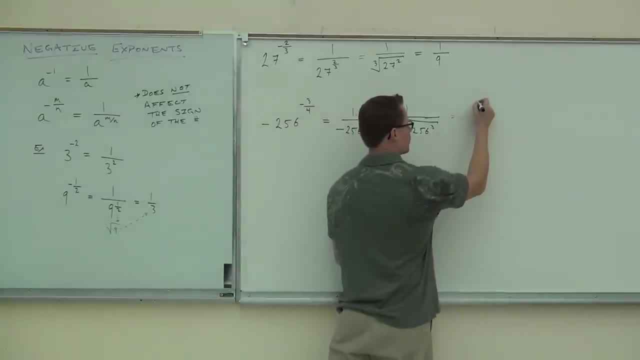 The fourth root of 256.. The fourth root of 256 should be 4.. And then we take the cube of that, We get 64. So this is 1 over negative 64. Or it doesn't really matter where you put that negative. 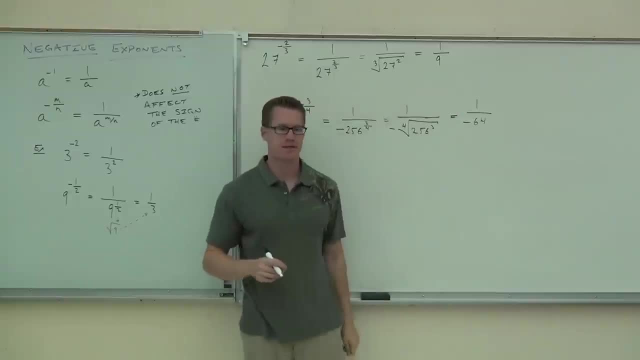 You could have negative 1 over 64 or negative 164.. That's the idea. If I did give you something like this- negative 64 to the 2, negative 2 thirds- would you be able to do it? Let's talk about it for a second. 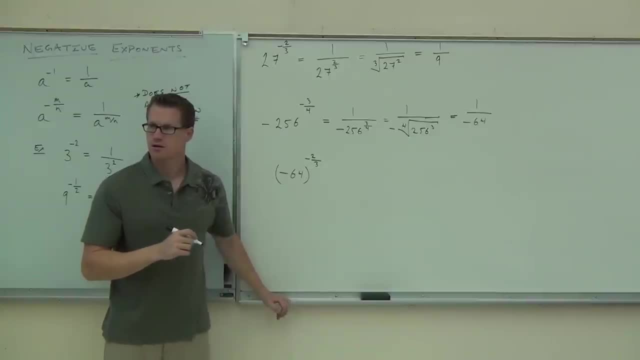 First thing you do is write this as 1 over what? 1 over 64. Would it still be negative? Is this negative ever going to change? Is this negative going to be inside the cube root that you're going to write eventually? 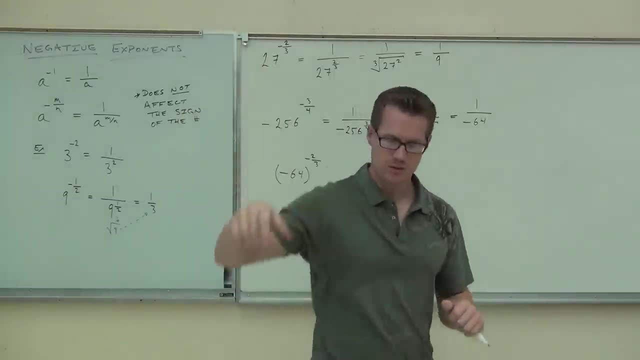 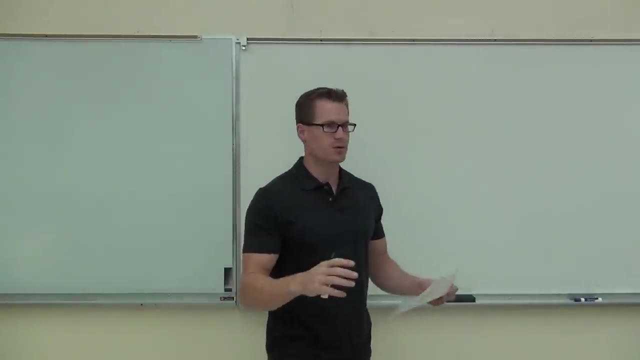 Okay, It would be inside. How many of you feel pretty good about what we've talked about so far? Good, So last time we learned that every single root that we have, the second root of our cube root, the second root of our cube root. 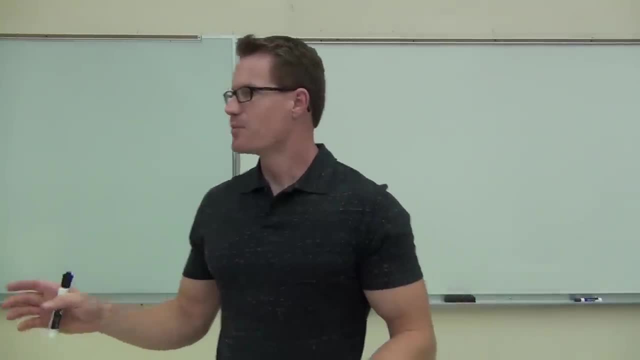 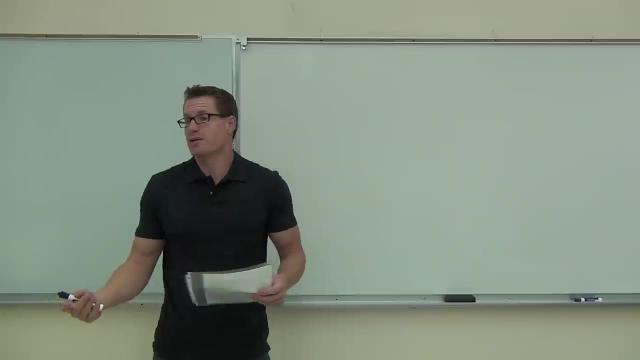 is going to be inside the cube root, Our square root. cube root, fourth root- everything about those can be written as rational or fractional exponents. We're going to learn today that those fractional or rational exponents can be used just like regular exponents. we've been dealing 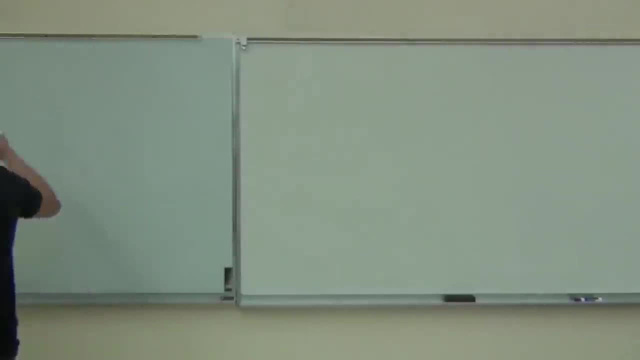 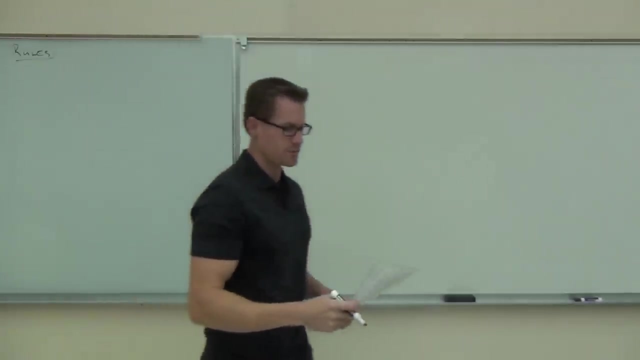 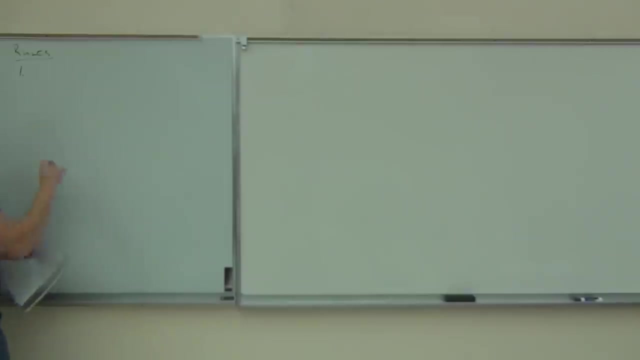 with since your pre-algebra classes. So we'll refresh your memory on some rules, Your exponent rules, and we'll apply them to those rational exponents. First one, if I give you some, and we're going to use general terms here- 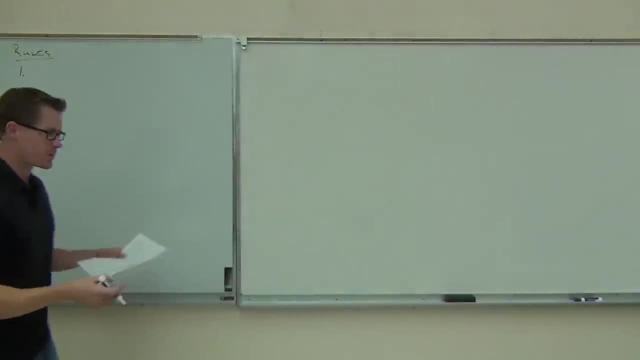 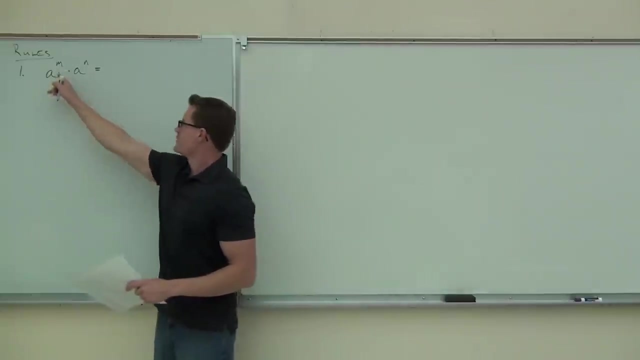 not actual specific numbers. We'll deal with those later. I just want to refresh your memory on the actual rules here. If I give you some common bases that are multiplied together, such as x squared times, x to the fourth power, well, if I have a to the nth, 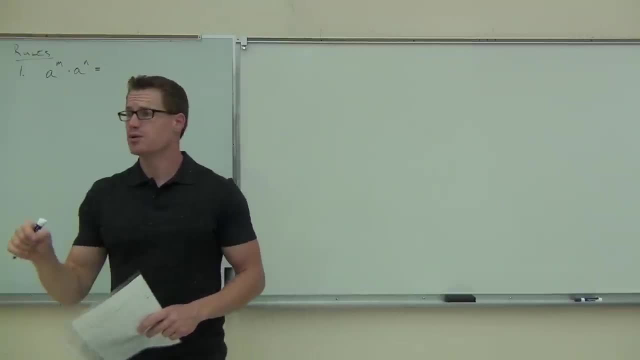 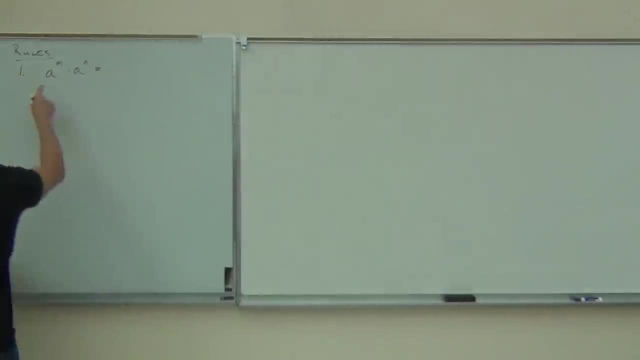 and a to the nth power. we're multiplying those things. what do I do with the exponents? Do I add them, subtract them, multiply them or divide them? We add them, Yeah, that's right. So if I have a to the m? 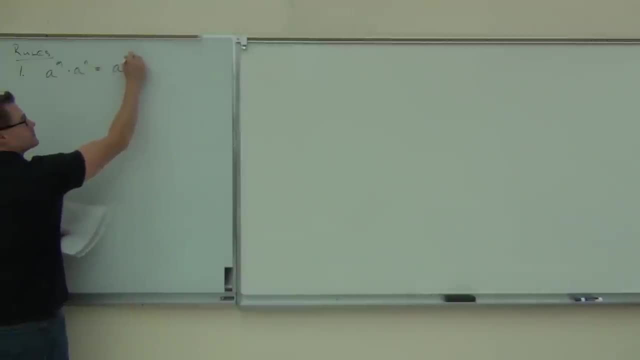 Times: a to the n. we know that's a to the m plus n. I just add those exponents. This should be a little bit of a review for us. Second one: if I have, and you know what, maybe I'll do an example over here. 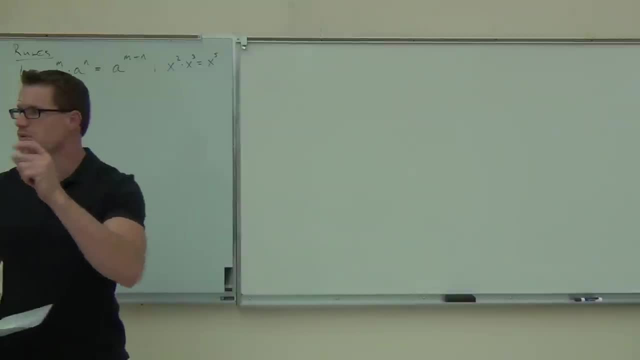 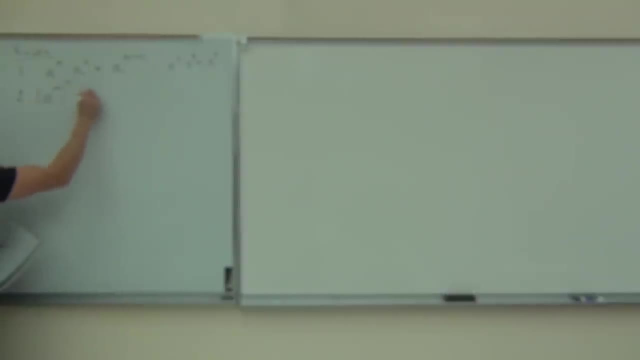 X squared times, x to the third is well, x to the fifth. We just add those exponents together If we have An expression that has an exponent in it being raised to another exponent, such as a to the m power, and then we take all of that to the n power. 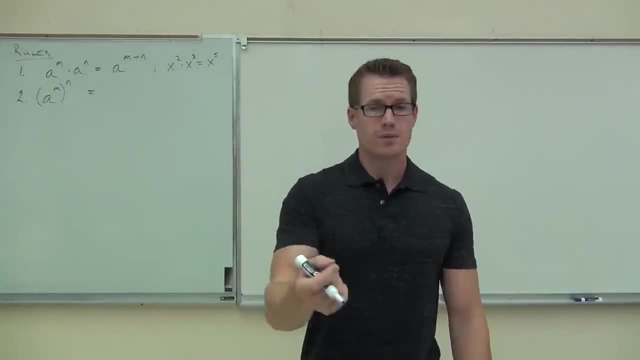 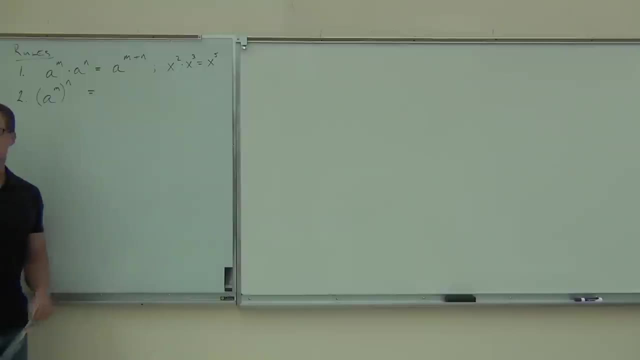 Do we still add those exponents together? No, No, we do multiply. That's right, because what this says is: I have a to the m times, a to the m times, a to the m times, a to the m? n times, and every one of those, we would add those m's together. 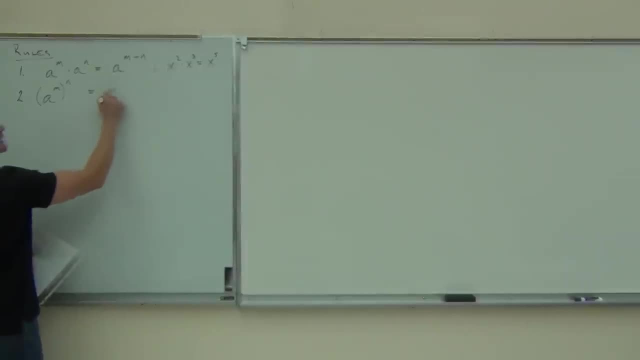 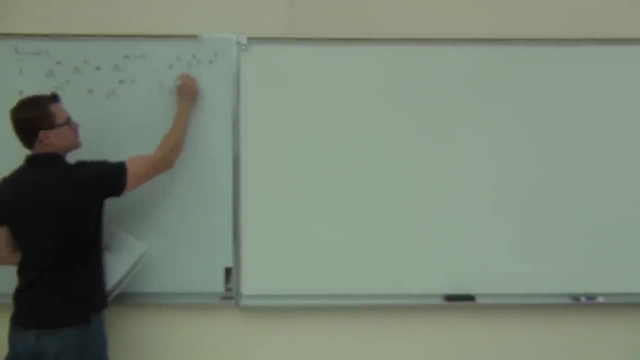 So that's repeated addition. That means multiplication. So here we'd have a to the m times n, For instance, if we had Y to the fourth to the third, that's going to give us y to the twelfth. This is kind of an important one for us. 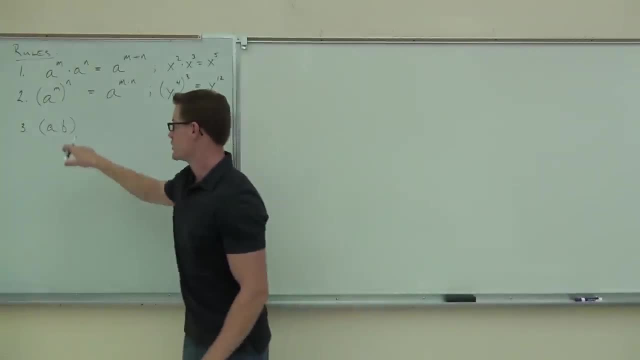 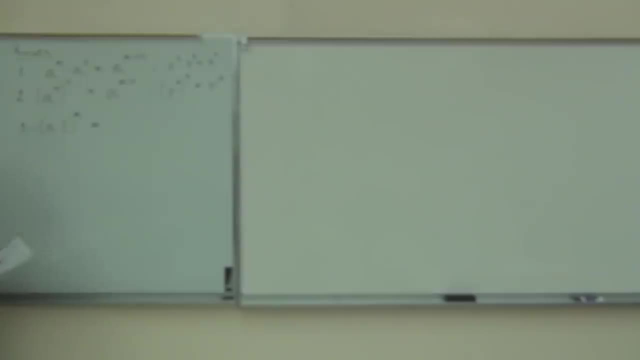 This is going to work a lot well for us. it's going to happen a lot. this situation, If I have a times b and I raise all of that to some power, Raise all of that to some power. What you need to know is that. 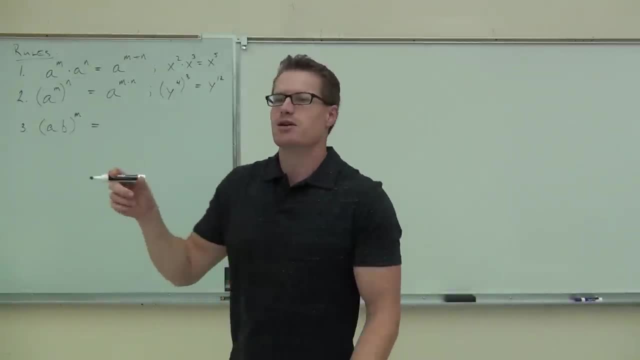 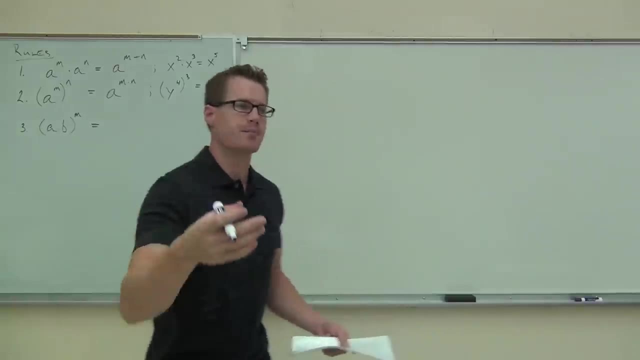 By cross multiplication We can. it's not like you're distributing, you're not actually multiplying these things, but you're raising every single factor in there to that exponent. So if I have a times b all to the m power, Then I know this is equivalent to a to the m, times b to the m. 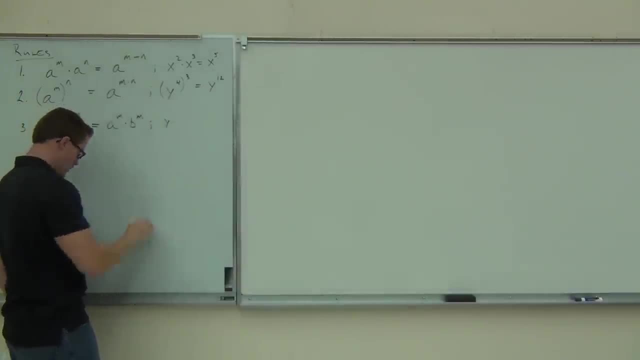 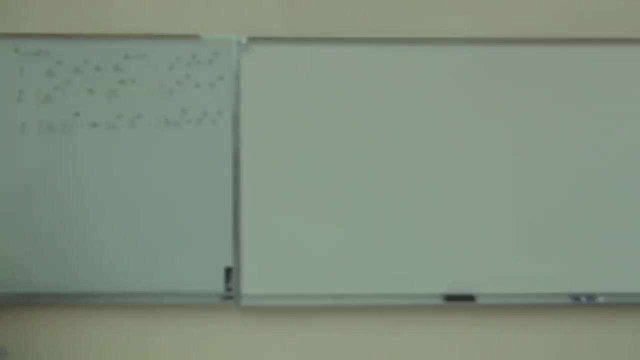 For instance, if I have y, Sorry, let's make it x- y. If I have x, y to the third, that means I'm going to have x to the third times, y to the third, It goes to both of them. 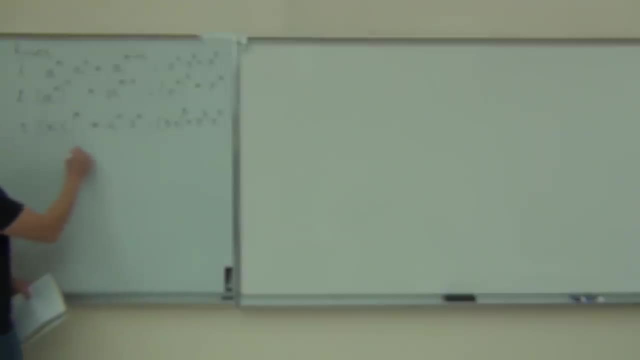 Hey, by the way, is this true? for addition, For instance, if I do a plus b to the n, is that the same as a to the n plus b to the n? Is that okay? Do you think so? Okay? 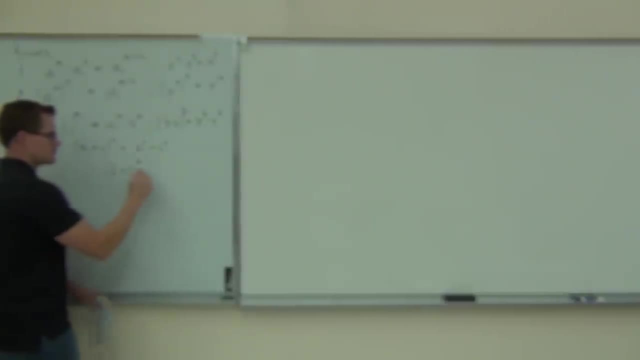 Let's make it even easier. How much is this? 5 by 5. 5 squared, How much is this? How much is this? Is it the same? Does this work? Does this work? Never do that, Never do that. 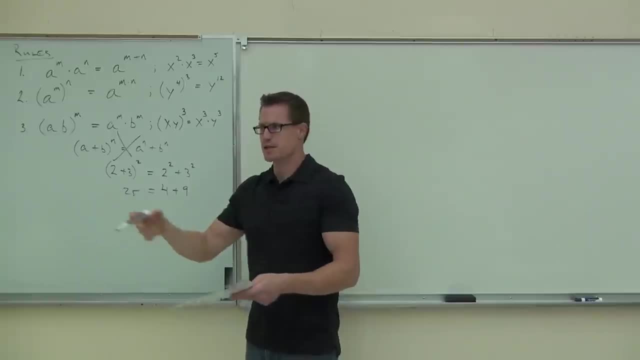 You can't distribute. or if you want to say distribute, you can't take an exponent across addition. It doesn't work. I just proved it to you. right, There's one example. It does not work, So this does not work. 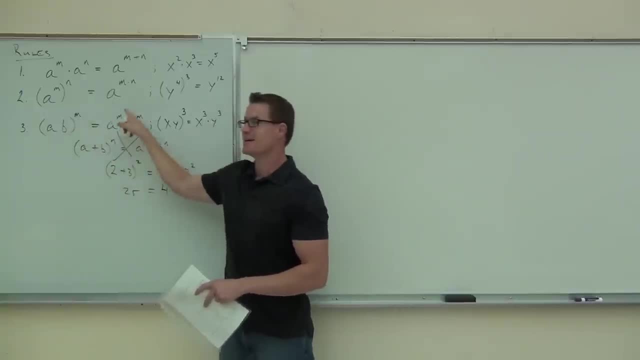 So are you ever going to do this? No, No, Can you do this? Yes, Yes, It's a different story. Okay, So when you have this product in here, that's fine. Both those factors get raised to the same exponent. 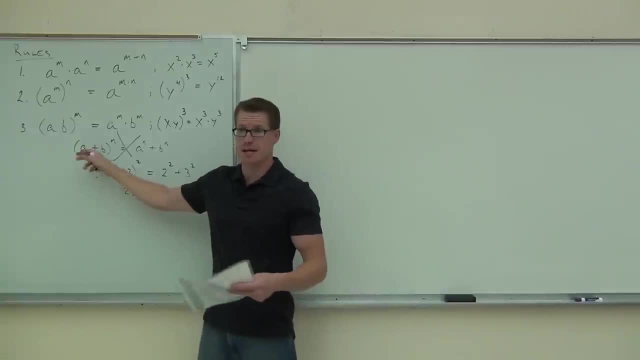 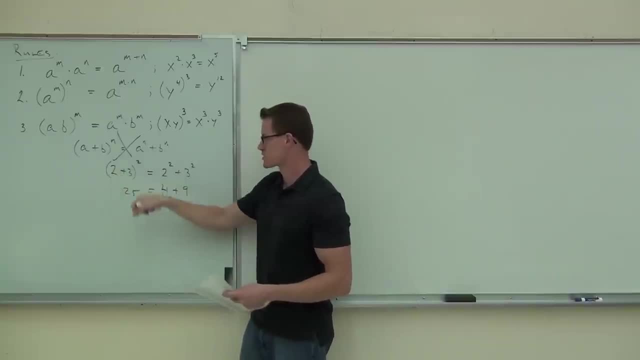 break that down Right. For instance, right here we have the 2 plus 3 squared. There's no way this equals 2 squared plus 3 squared, This is 25.. This is only 13.. There's no way that it's the same. 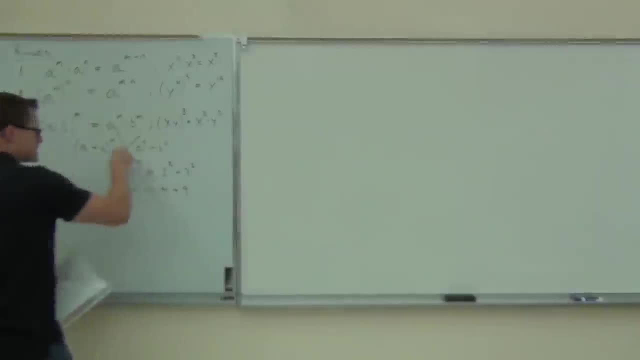 I'm not sure. if you're okay on that, All right, So make sure you have that down. I'm going to erase this just so we're sticking with our rules, but if you want to write that down, this is just one instance where you cannot do that. 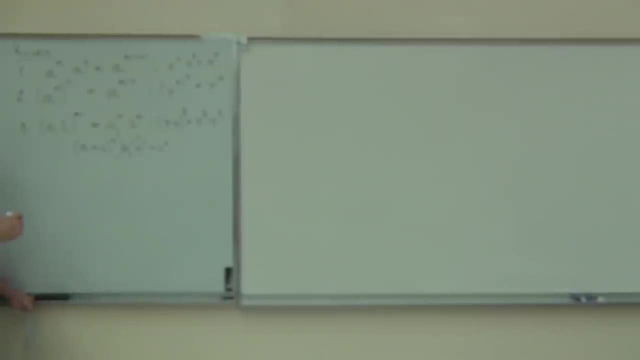 So that's just like a FOIL method, though right, If it was just a plus b plus a and a plus b, it would sort of work. If that was a square, If that was a square, sure, Oh, okay. 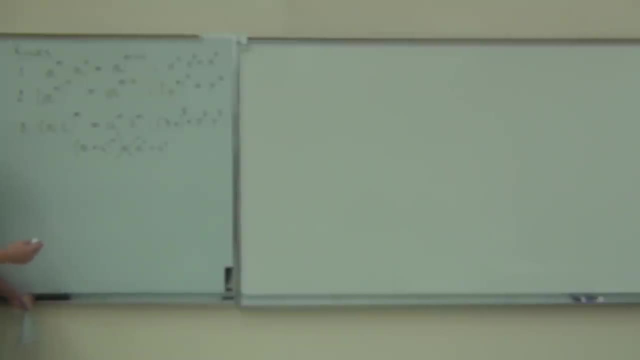 Yeah, yeah, yeah, If that was a fourth power, Then it would be four times. Yeah, That would be messy, right? You don't want to do that. Yeah, But you could, You, could. You just can't do that. 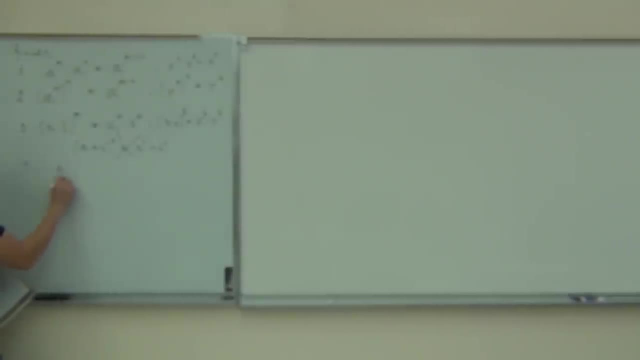 Okay, Back to our rules here. If I have some fraction to an exponent, what we need to know is that, just like here, where we had the product and you have your product raised to the n power, if I have a fraction raised to the n power, both the numerator and the denominator are going to be equal. 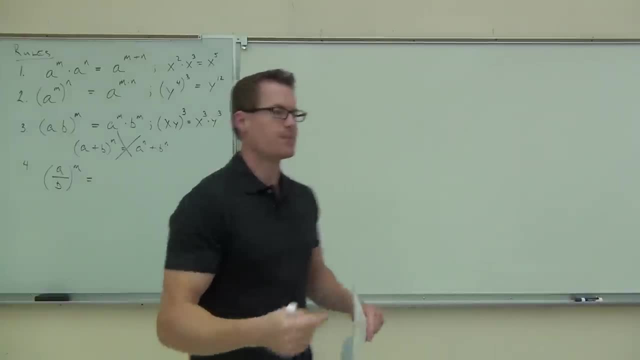 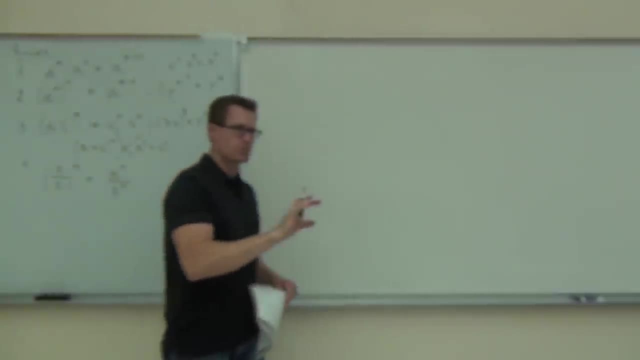 Right, The denominator and the denominator get raised to that power as well. We've talked about that before in this class, so we're just going to write a to the m over b to the m. It just goes to both the numerator and denominator. 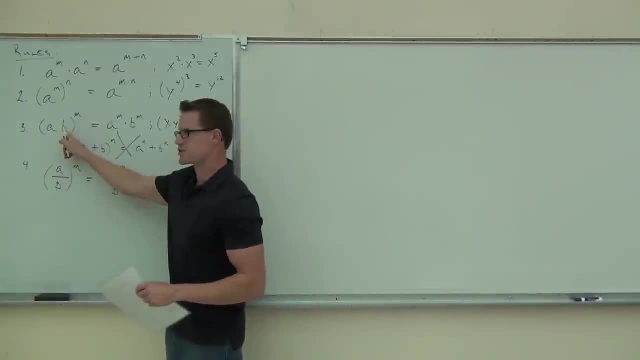 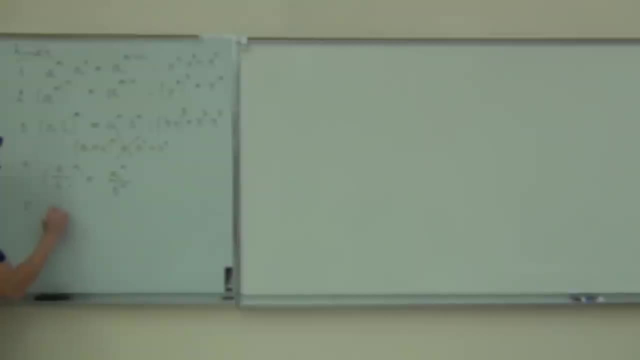 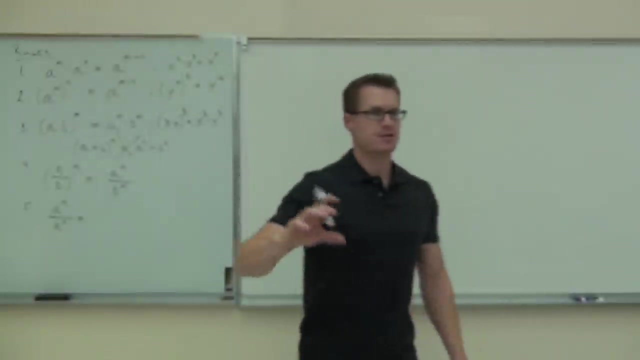 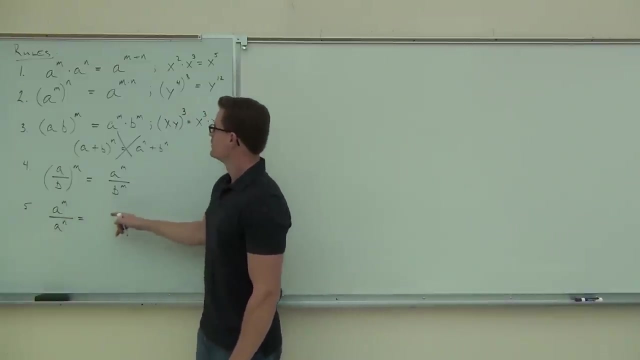 Very, very similar to this one is just you're dealing with a quotient instead of a product. If I have a quotient where I have the common base there, a, I have a to the m plus a and a to the n power over a to the n power. if I multiply common bases and got to add exponents. 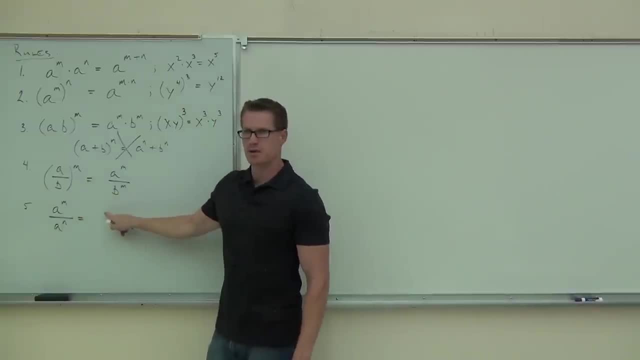 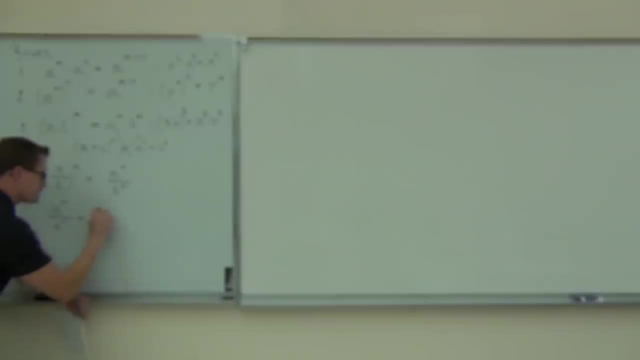 when I divide common bases, what am I going to do to those exponents? Add them, And multiplication means you're going to add those exponents. Division means you're going to subtract those exponents. And we do it like this: We do the a to the m power minus n power. 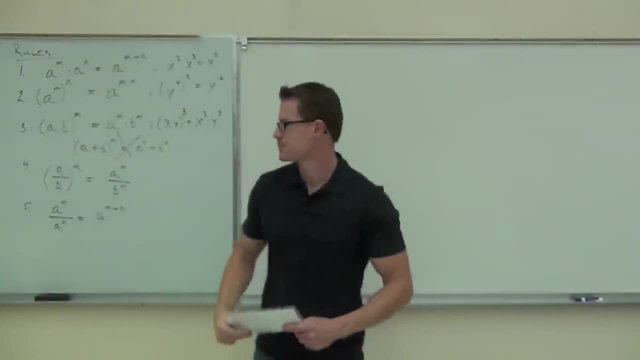 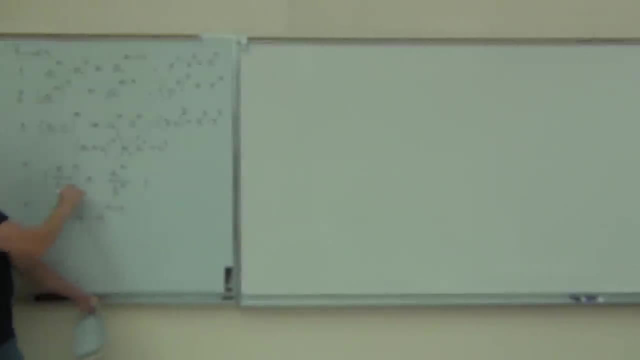 M minus n, The top power minus the bottom power. Okay, Okay, Well, I guess I could give you some examples here. huh, So for this one, if I did 3 over x to the second, that'd be the same thing as 3 to the. 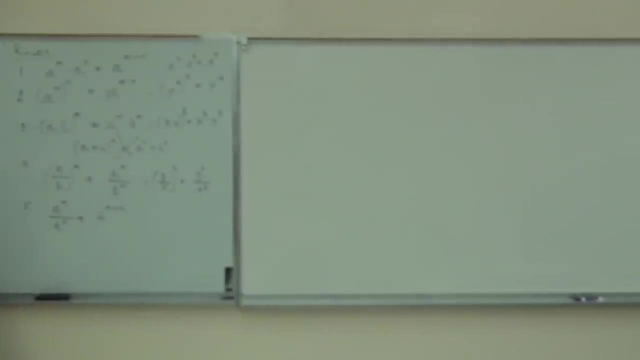 second over x to the second or 9 over x squared. If we wanted to do common bases, we'd do something like y to the second over y to the fifth. Okay, If I did y to the second over y to the fifth, we have common bases. 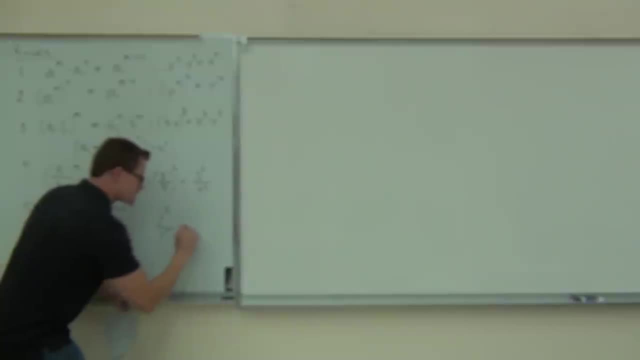 We have y to the second, y to the fifth. What we do here is we'd say: this is the same thing as y to the what comes first, 5 or the 2, if I'm going to subtract the 2?. 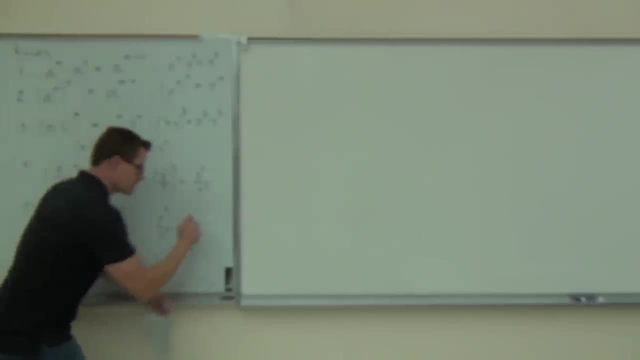 It makes a difference, doesn't it? The 2 would have to come first. it comes on the numerator there: 2 minus 5, what's our answer going to be Y to the negative 3.. Y to the negative 3.. 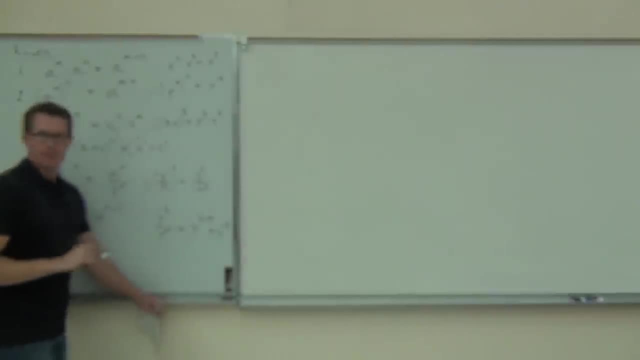 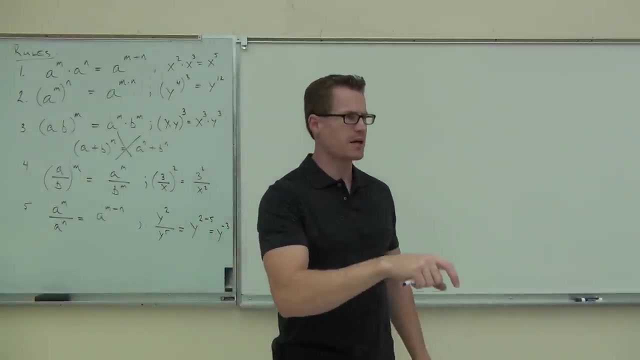 Okay, You still have to do the first half. Yeah, It's a 1 over y to the third. Say that again: 1 over y to the third. That's right. So if I write that as a positive exponent, you remember doing that last part of class. 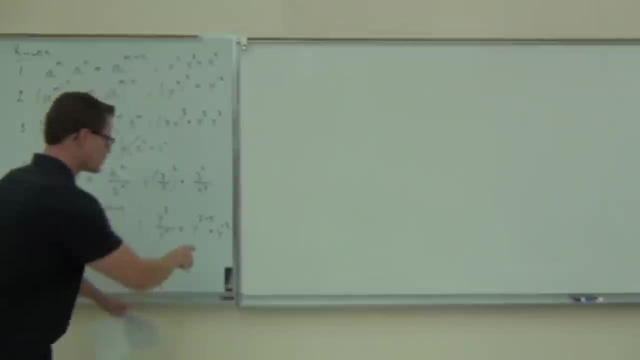 last time for those negative exponents, we changed those back to a positive. You go, okay. instead of y to the negative 3, I don't like that so much. I want to do 1 over y. cubed, I'm going to move over here with the rest of our rules so you all can see them. 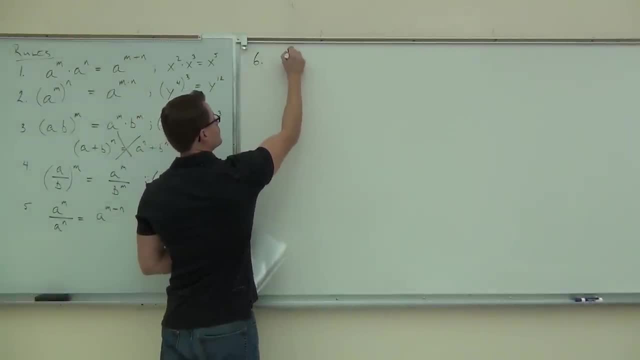 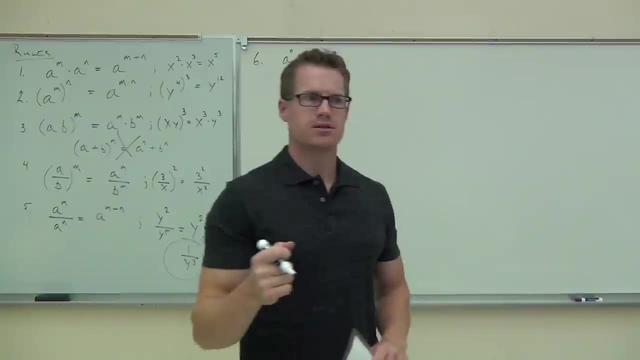 There's only two more. Next one: What's anything to the 0 power? How much is that? Some people say 0, some people say 1.. What is it? It's not itself, It's 1.. Yeah, it's 1.. 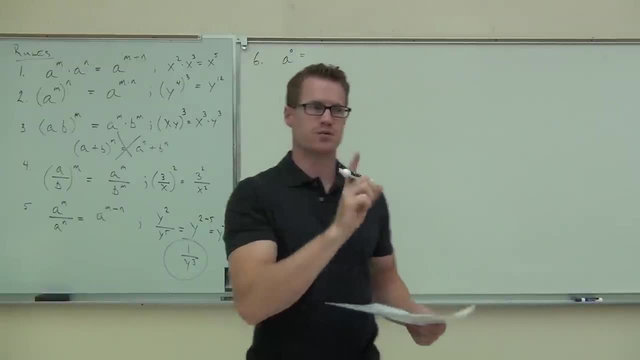 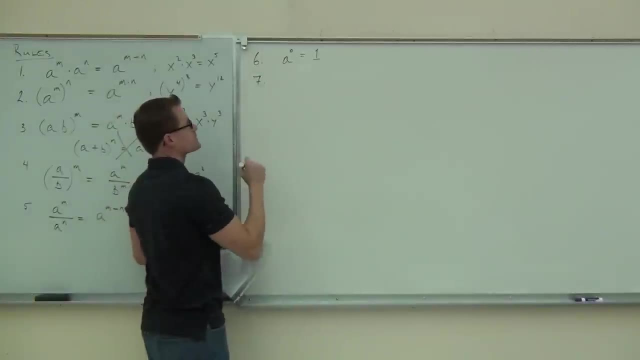 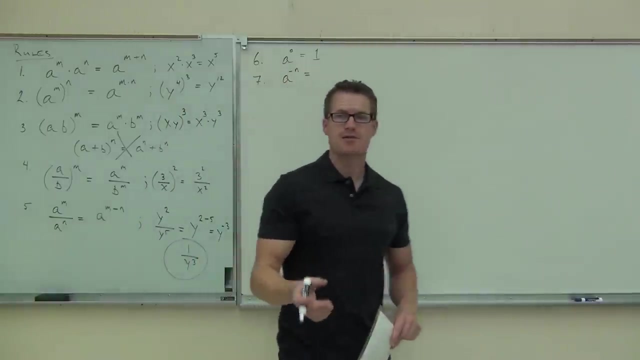 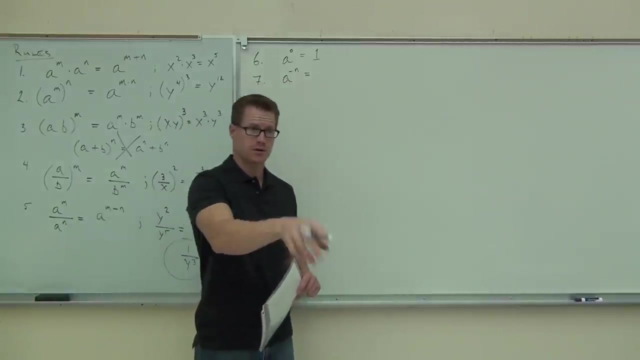 Anything to the 0 power is defined as 1.. And lastly, a refresher. We did this last time. just a good little note to have Anything to the negative exponent, You can always change it to a positive exponent by doing what? 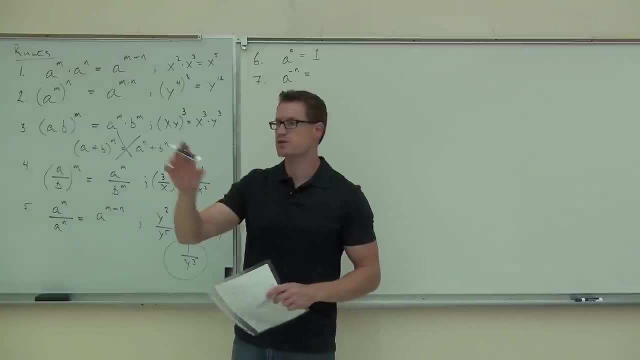 So, wherever it is, we change the part of the fraction that's on it. It's on the numerator and it's negative, We move it to the denominator, Because on the denominator we can make it positive by moving it to the numerator. 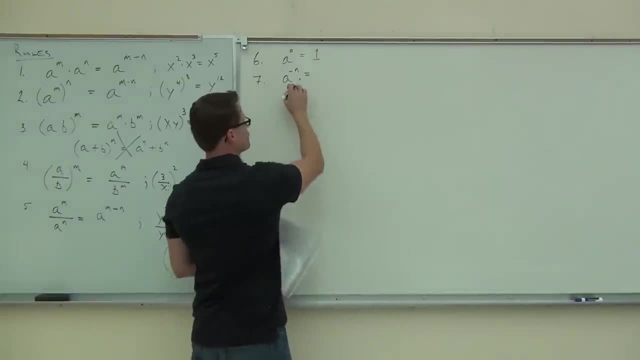 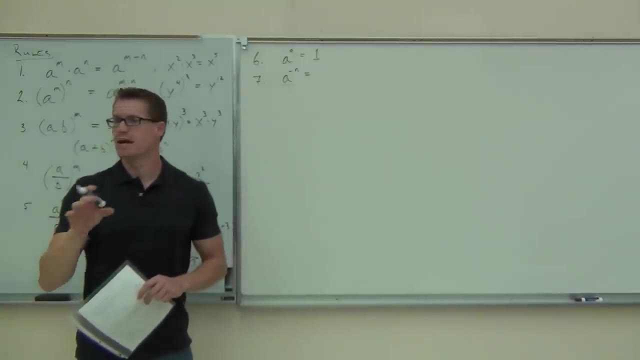 We just change the spot of the fraction where it is. So, for instance, right here, we consider this to be on a numerator, because you can write that over 1.. If we want to change the a to the negative n to a to the positive n, what we have to 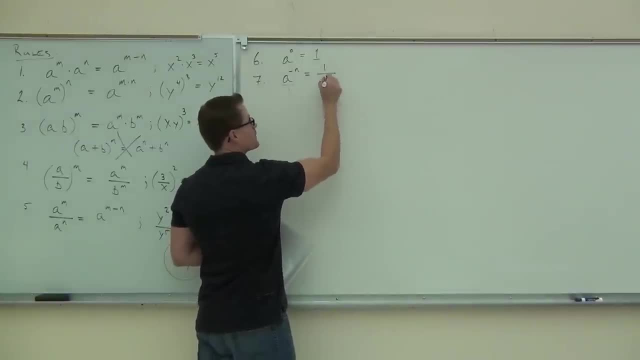 do? is we have to write this? What do we do? We have to write this on the denominator of the fraction. Remember, recall from last time, that it doesn't change the sign of the number, It just changes the sign of the exponent. 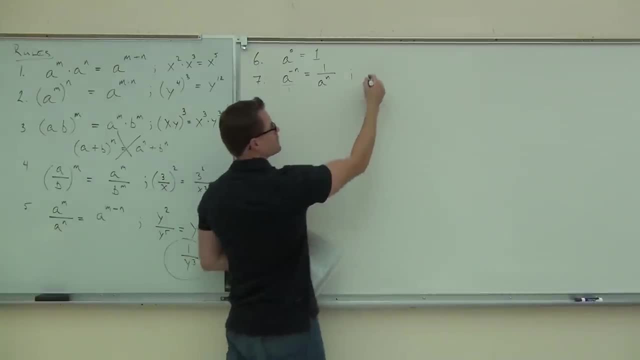 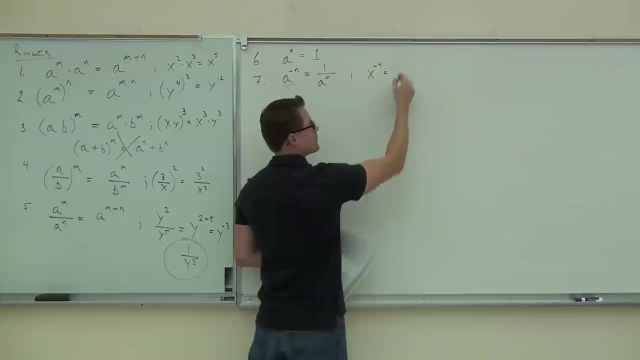 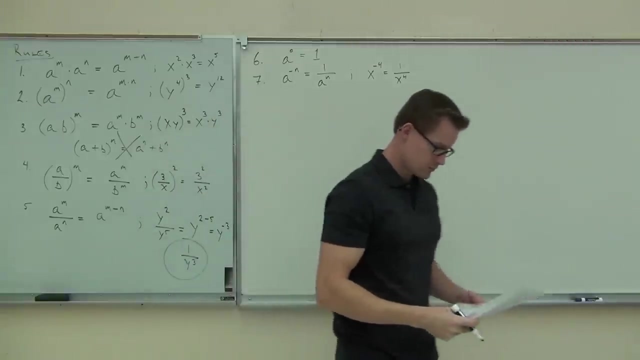 And we did several examples, but I'll give you another one over here. Let's see X to the negative 4, we could write that as 1 over x to the 4.. Hey, would you raise your hand if you feel OK with this? 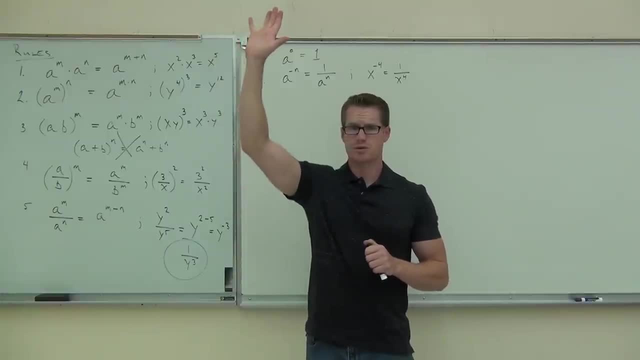 Yeah, Yeah. Yeah, That's right, It should be a refresher for you, right, It should be a refresher for you. Now, what we're going to do is we're going to take these rules that we just kind of reviewed. 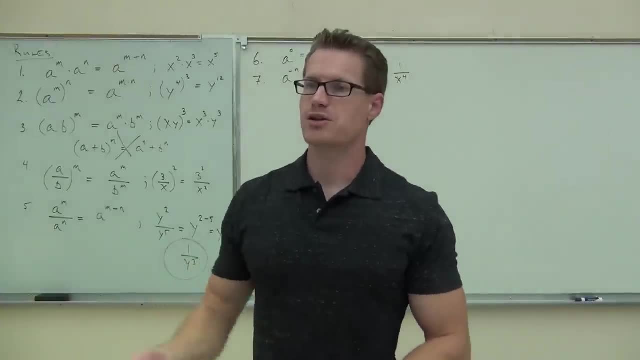 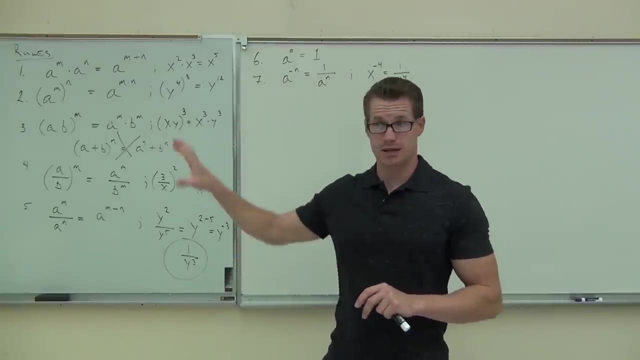 and we're going to apply them to our rational exponents. What you need to know is that every one of these rules works exactly the same way for rational exponents as it does for whole numbers. Now I gave you some whole-number or integer exponents, but right now I'm going to give 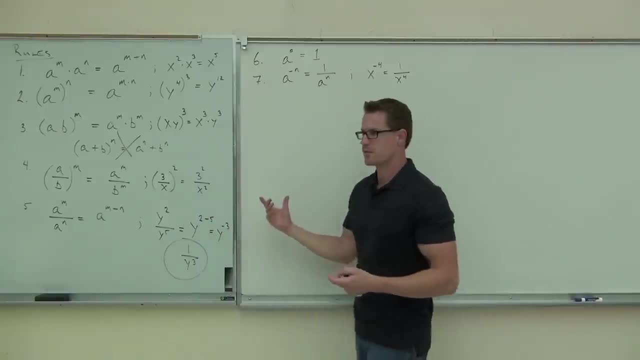 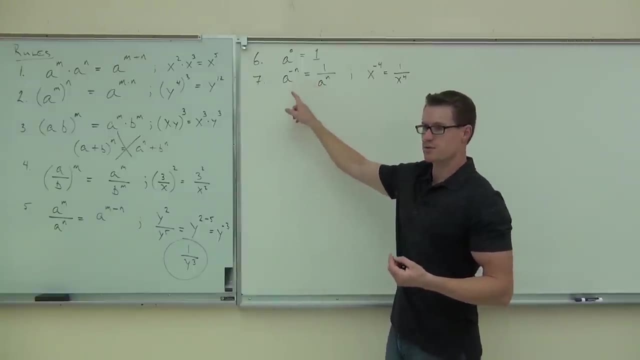 you those fraction exponents. They work the same As long as you stick with these rules. there's only 7 of them. Most of them are very refresher. The only one that really might be a little new for you is using this with those fractions. 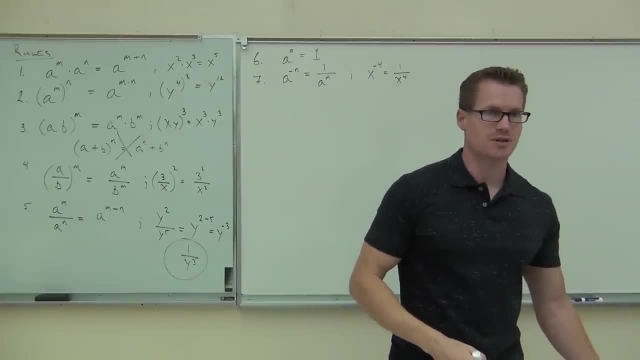 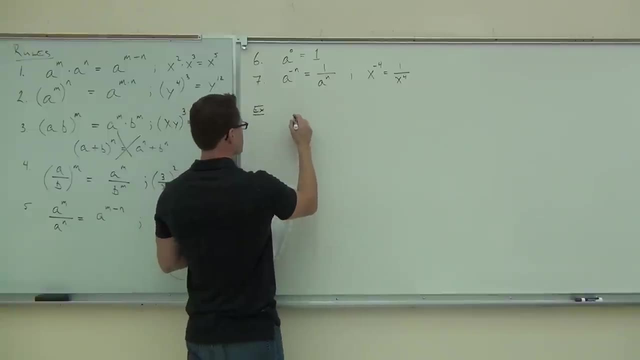 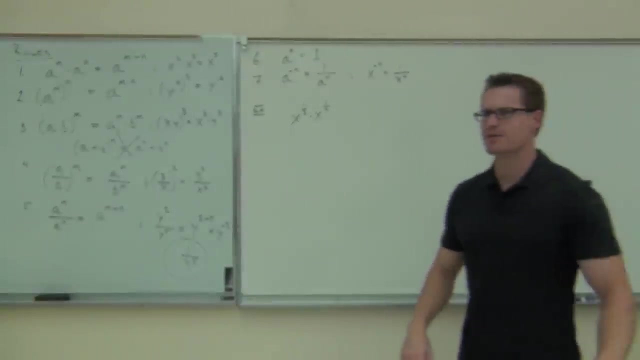 but it's the same ideas. Are you guys ready to try some examples here? Let's do that. Okay, we got x to the one-third times, x to the one-fourth. Ladies and gentlemen, do we have a common base there? 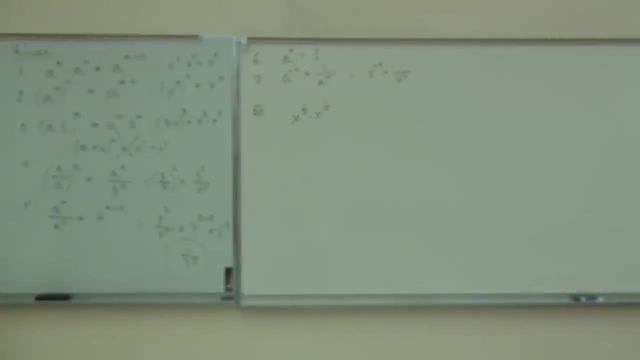 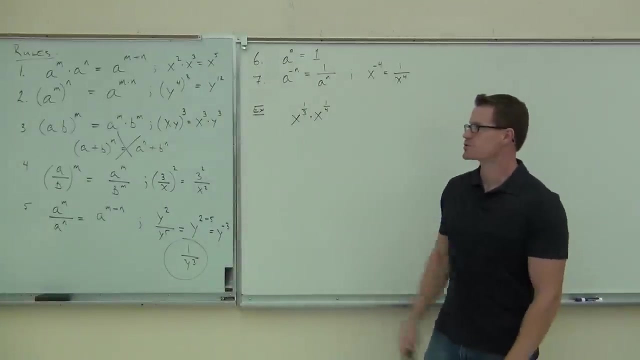 Do we have a common base And they're being multiplied. So when we look at this, we're multiplying them. What situation are we most like? Rule one through seven: Which one are we most like? do you think Rule number one? 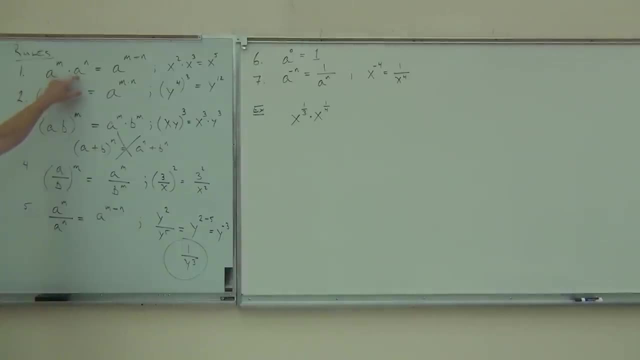 I've got two things with a common base that are multiplied together, and I have some exponents up there. So what am I going to do to those exponents? Am I going to add them, subtract them, multiply them or divide them? 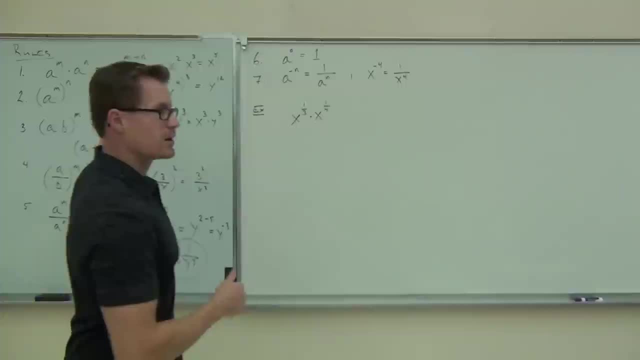 What do you think? Add them For sure, I'm going to add them. That's what this says, right? You know what a lot of people do. A lot of people do this. They make the mistake and they're doing this really quickly because they get the handle. 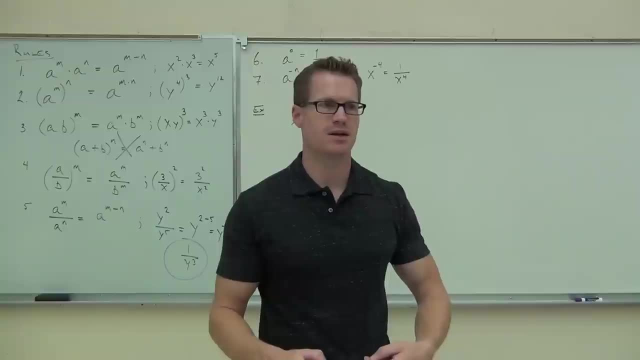 on it right. but then they're really not reviewing it enough and they get to the test and they go: oh, that's x to the one-twelfth. Do you see how easy that is to do? If you're just thinking multiplication, your head's thinking multiplication, right. 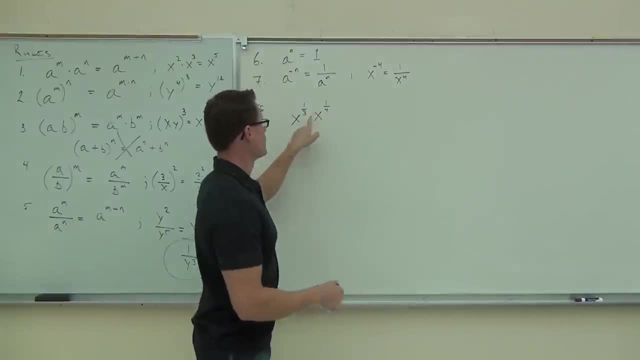 You're not thinking really. the exponent rules if you're just seeing this. If you just see this, you go: oh, one-twelfth, yay, I'm done. Well, if we do that, we're kind of missing the big picture here, right? 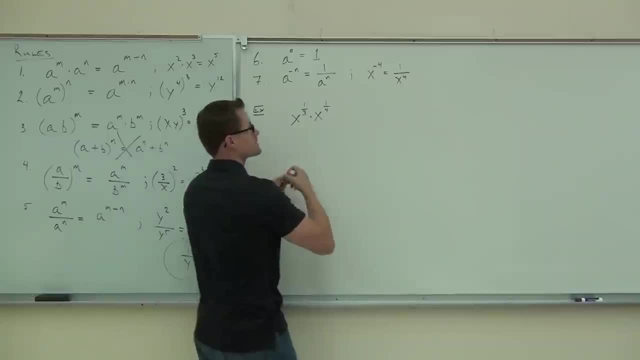 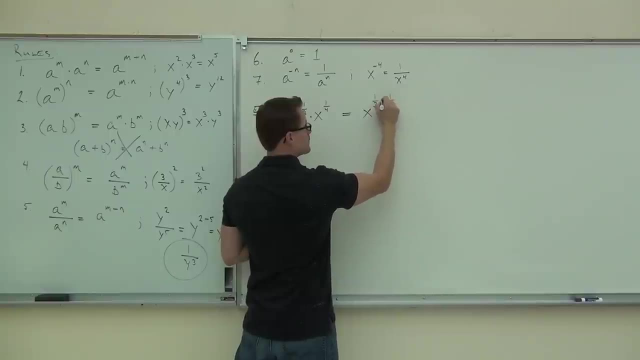 These are exponents, And exponent rules say: if I multiply on a common basis, what I'm really doing is I'm adding those exponents together. That's what I'm really doing Now. can you add one-third plus one-fourth? You do. 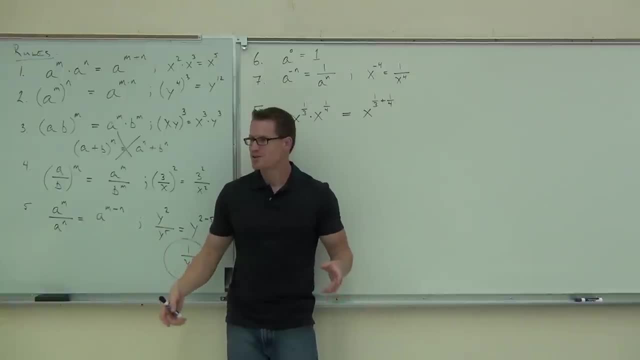 We know how to add fractions. right, This is a fraction class. We're past fraction class, It's great. So we use your calculator. I don't care if we use your calculator or do it off to the side. I would personally do this off to the side and just say: okay, I know I need to do this. 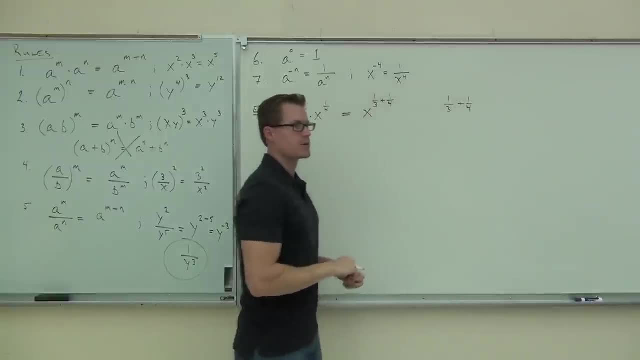 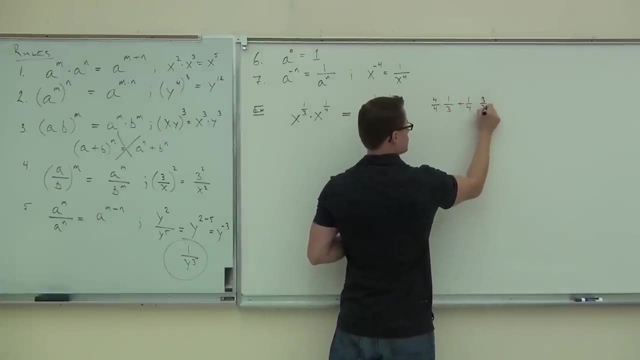 to add one-third plus one-fourth. That means the common denominator is going to be what? So we're going to multiply this by four over four, This by three over three. we'll get four-twelfths. We'll get three-twelfths. 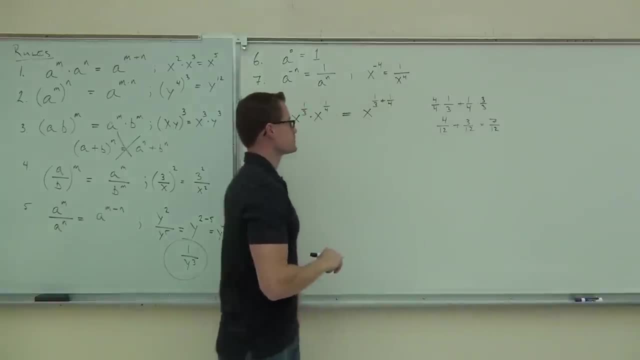 That's going to give us seven-twelfths. So instead of x to the one-third times x to the one-fourth or x to the one-third plus one-fourth, We actually added those and we got x to the seven-twelfths. 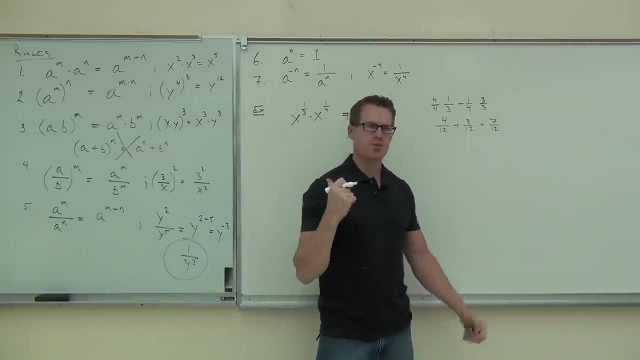 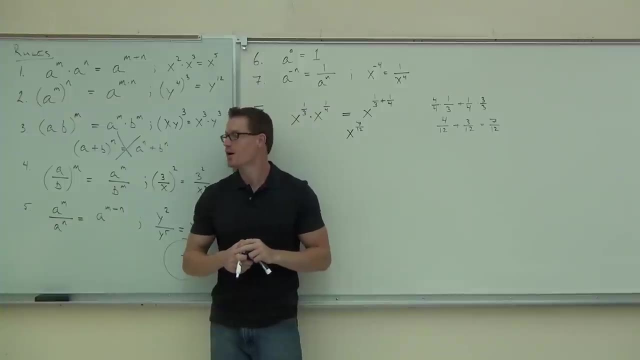 Are you okay with that one? Yeah, Hey, by the way, could you write this as a root? No, Could you write that as a root? What type of root do we have? Twelfth root- Twelfth root of what? 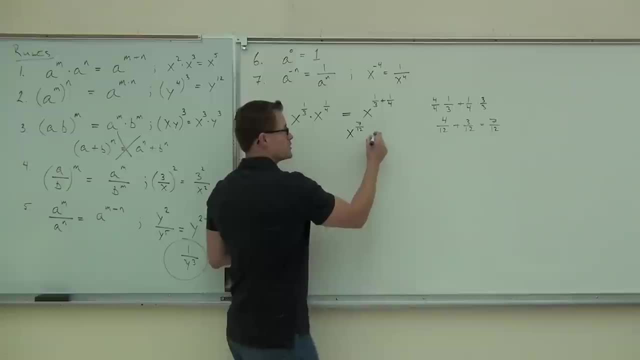 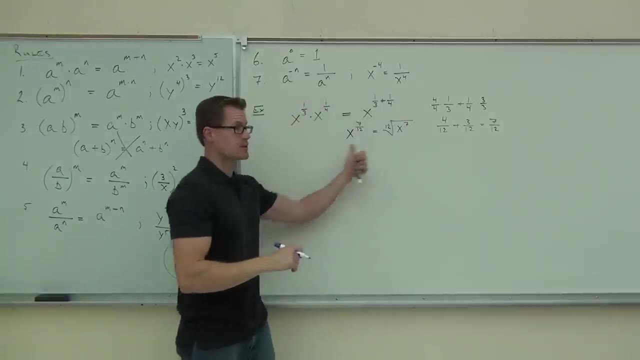 X to the seven-twelfth. So, if you wanted to, if the problem asks for it, that's that root. These things are the same thing. So this actually makes that. I want you to see how this stuff actually works here. Notice that the common denominator. the common denominator is the root, isn't it? 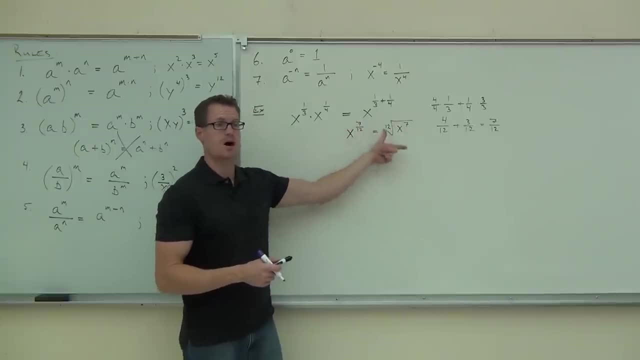 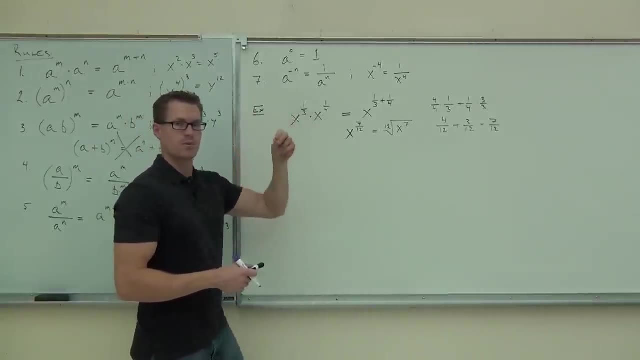 That is the root, Because we know that the denominator makes the root up. So when we find the common denominator, that's making a common root, This you could have written as a cube root of x. right, This you could have written as a fourth root of x. 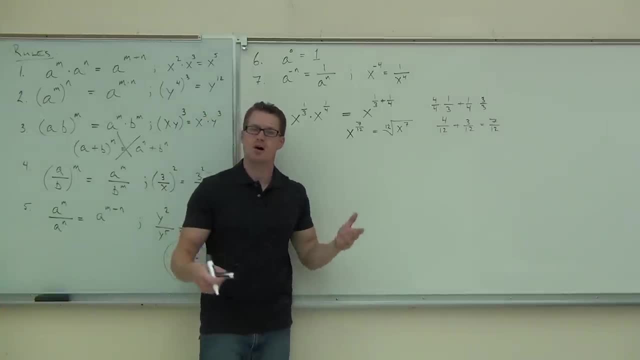 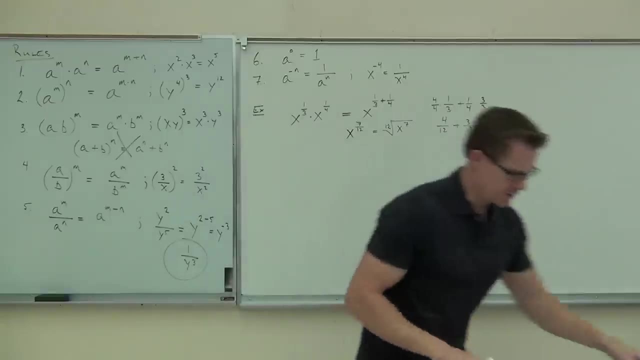 Multiply those two things together. you have to find a common root. In that case it means a common denominator. That's why all this stuff is intertwined. It works like that. All right, Let's move on here Before I do. are there any questions on that example? 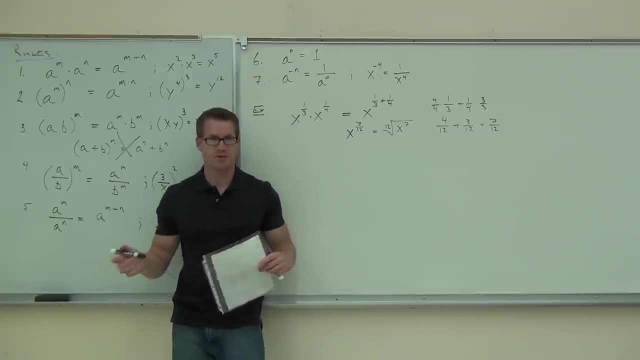 Because this is just our start off point. Are you guys all right with that one? So the final answer is the square root. If it asks for the root, then yeah, that's the final answer. If it doesn't, you can definitely leave it. x to the seven-twelfth. 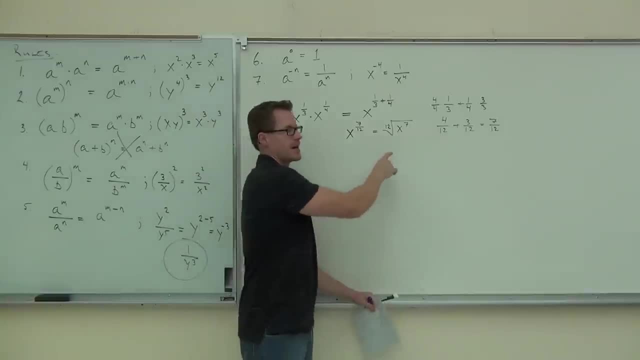 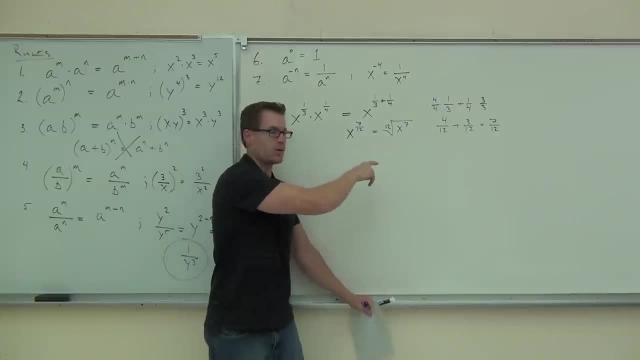 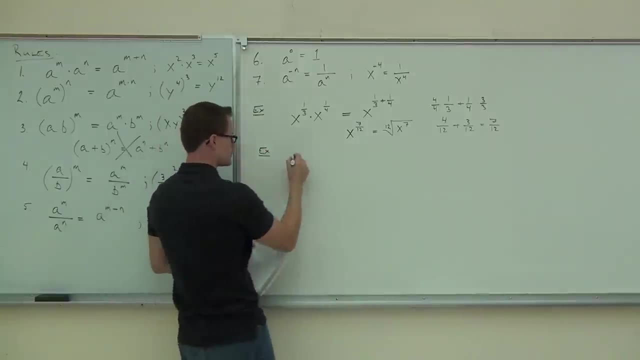 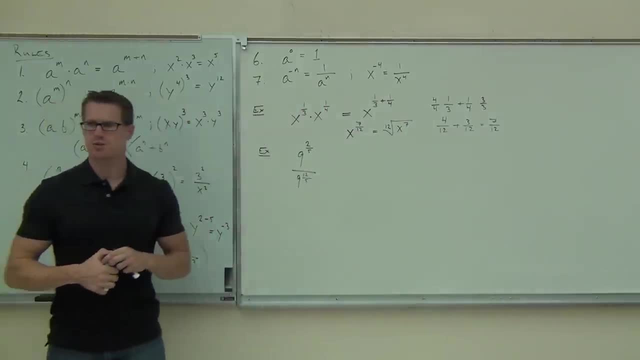 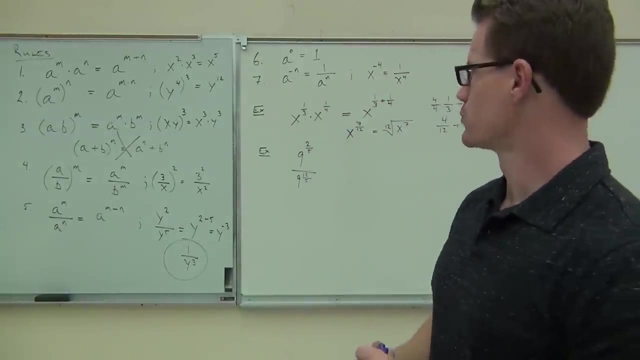 All right, 9 to the two-fifths over 9 to the twelve-fifths. Hey, let's look back at our rules. Can you tell me what rule we're most like? One through 7.. There's only two that have fractions, right? 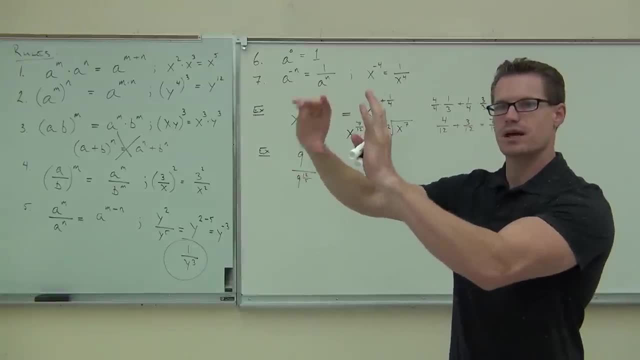 There's four and there's five. The four would be everything raised to a power. We're not there. We're actually on number five, where we have something raised to a power and something raised to a power. We have the common base there. 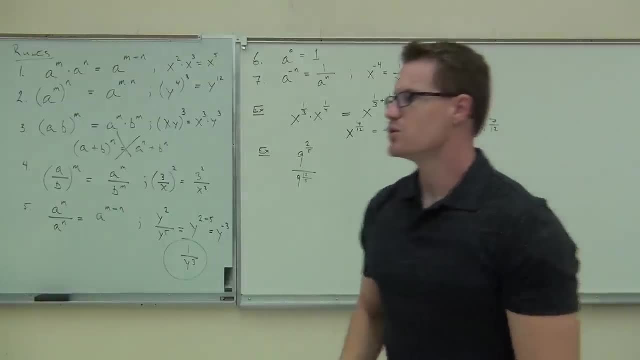 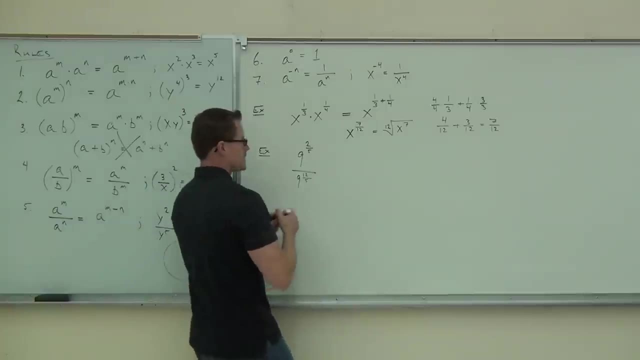 You with me on that? that's 5?. Okay, so what are we going to do with those exponents? Add, subtract, multiply, divide, What do you think Definitely subtract? What we do in this case is we take our 9.. 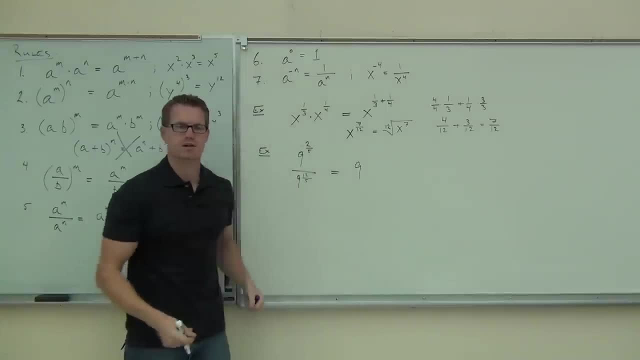 We write only one, 9, because we're combining the exponents. We're combining these two things by subtracting exponents. Are we going to have 12 fifths minus 2 fifths, or 2 fifths minus 12 fifths? 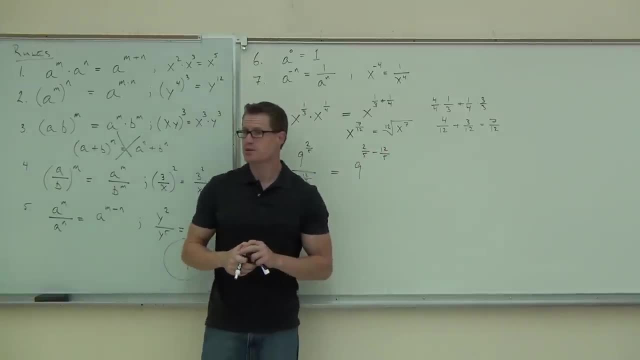 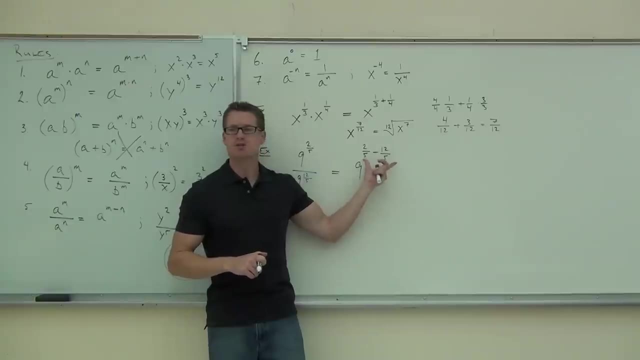 Can you do 2 fifths minus 12 fifths? That's kind of better than that problem, right? You don't even need a common denominator, It's already there for you. That's great. How much are you going to get? 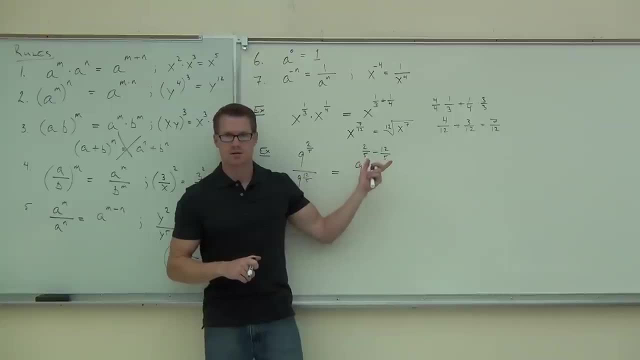 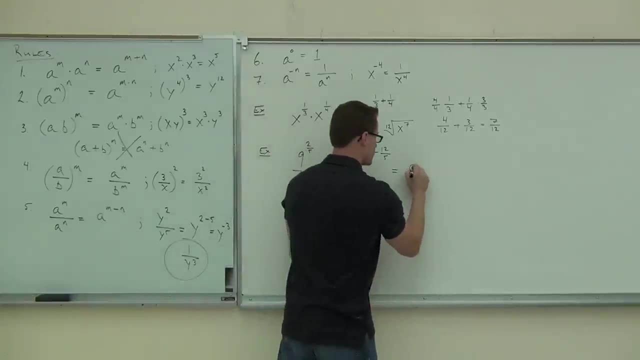 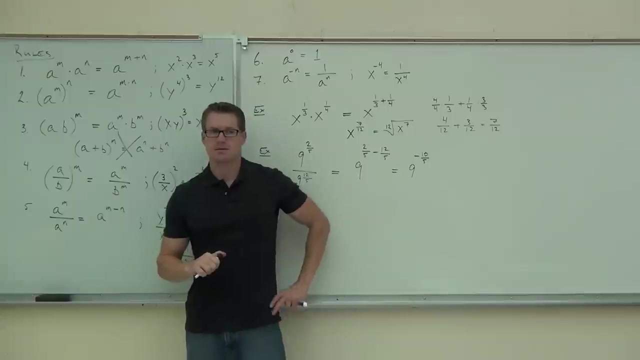 2 fifths minus 12 fifths, It's negative. Okay, Is the number negative or just an exponent Negative: 10 fifths. Are we done? What do we need to do? This is a fraction. Even though it's an exponent, it's still a fraction. 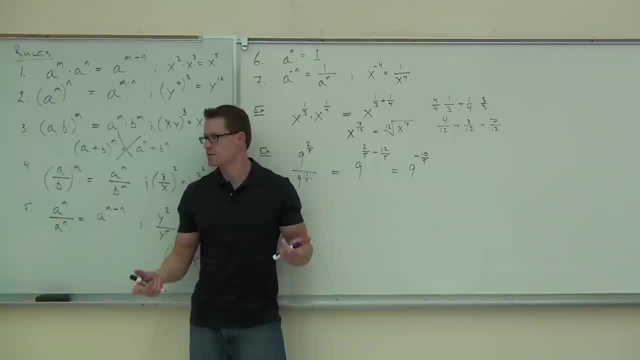 which means that you can simplify it just like you would any other fraction. So negative 10 over 5, we didn't know that's negative 2.. I'm not going to give you negative 10 fifths. I don't want that. 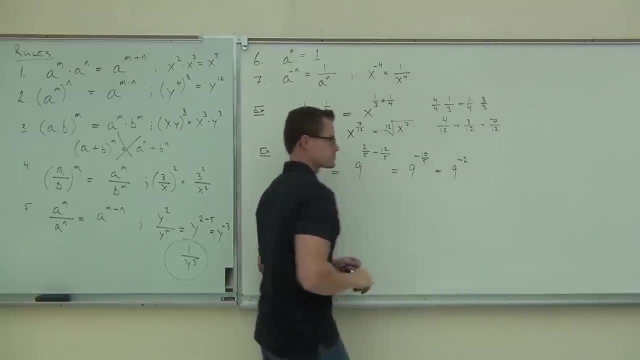 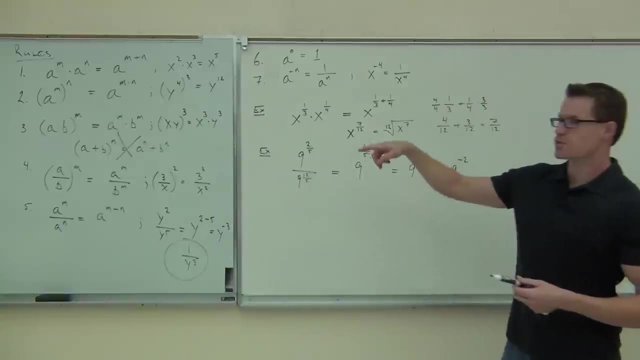 We say: oh okay, that's 9 to the negative 2.. Tell me another thing we can do with that. This is another rule. What rule is this Now? that's number 7.. It says okay anything. 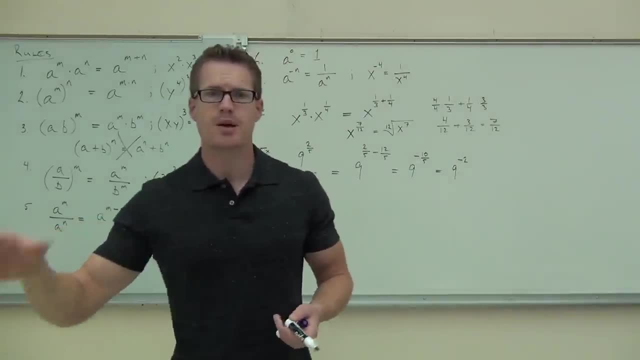 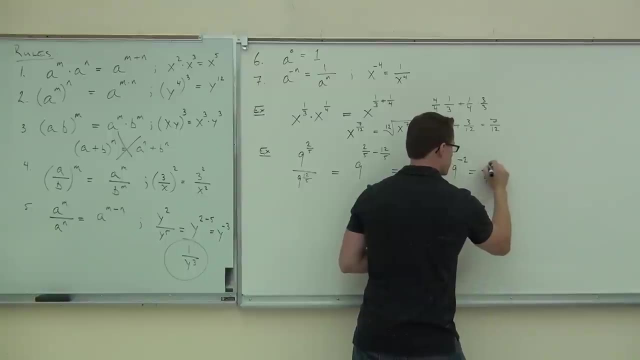 that's raised to a negative exponent, we can make that a positive exponent by putting that on the denominator of a fraction. So right here we're going to go. all right, I want 1 over 9 squared. 1 over 9 squared. 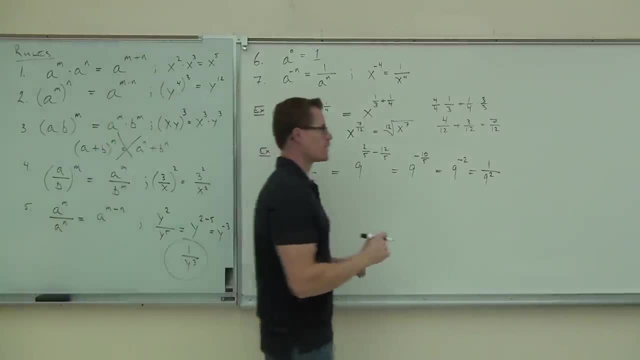 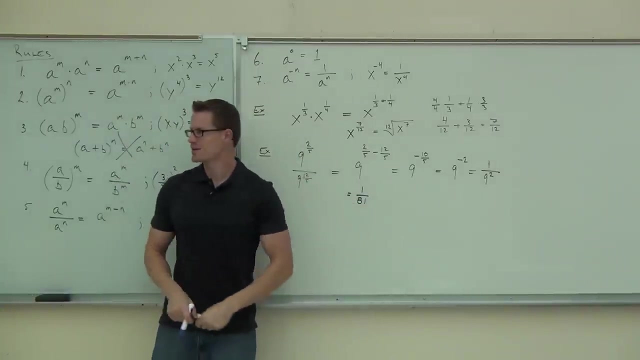 Ladies and gentlemen, how much is 9 squared 81.. So this is 1 over 81.. Gee, So we worked this all the way down. We only got 1 out of 81.. Isn't that kind of interesting that this means the same thing. 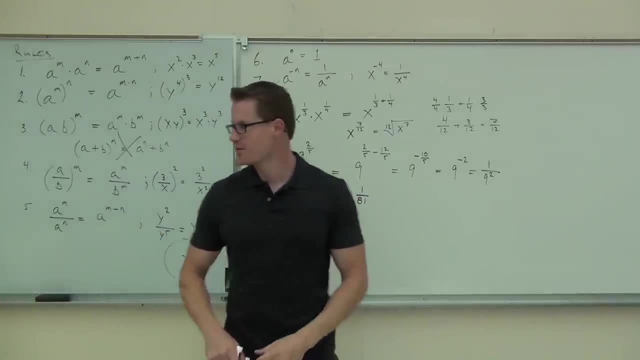 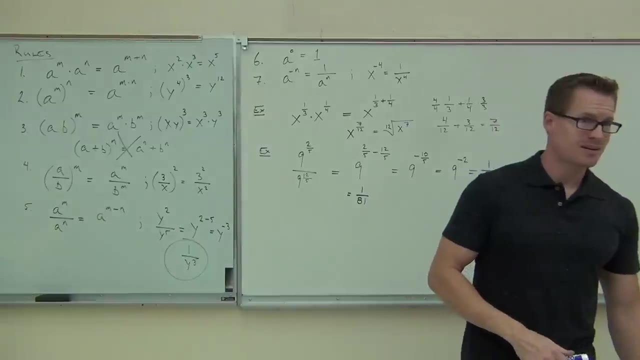 as that, just by using our rules and manipulating that, We get that down to 1 over 81. It's kind of cool, right? That's a whole lot easier to think about than that. Can you go back to the original problem? 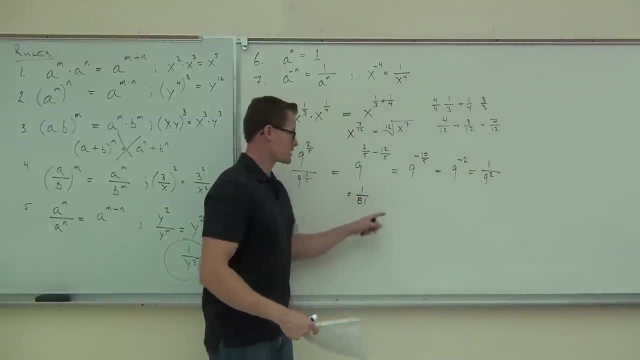 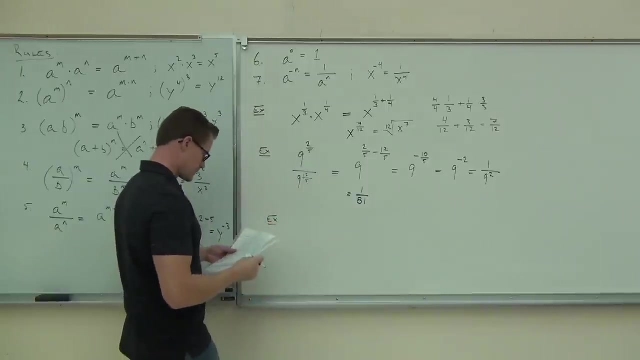 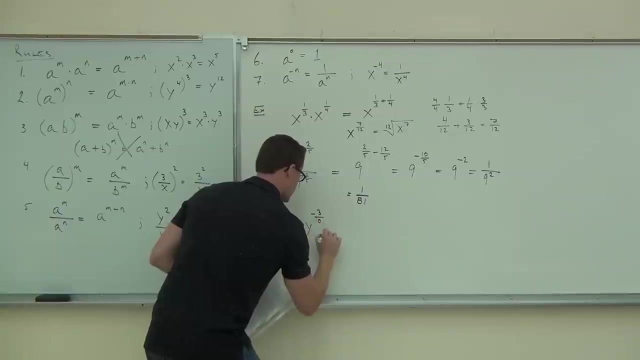 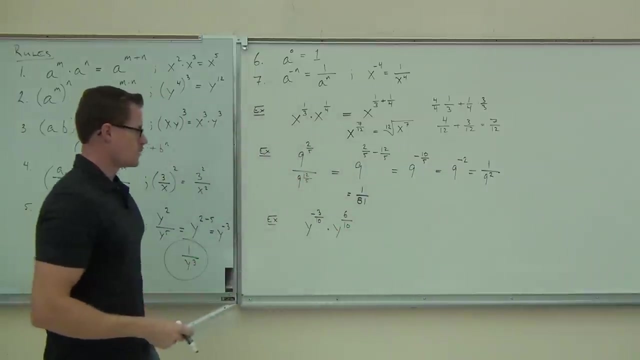 You can, but I mean it's after you do all this. if you just looked at this, there's no way to tell that that's what you started with. Okay, Y to the negative 3 tenths times. y to the 6 tenths. 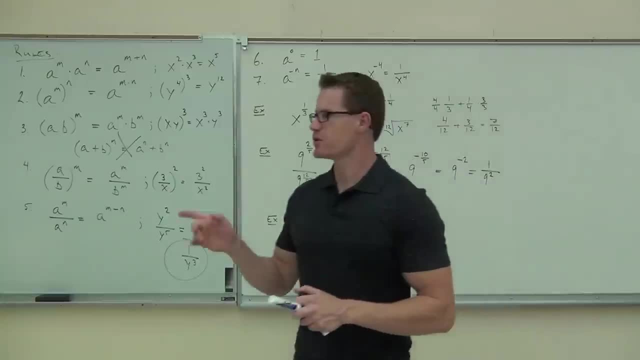 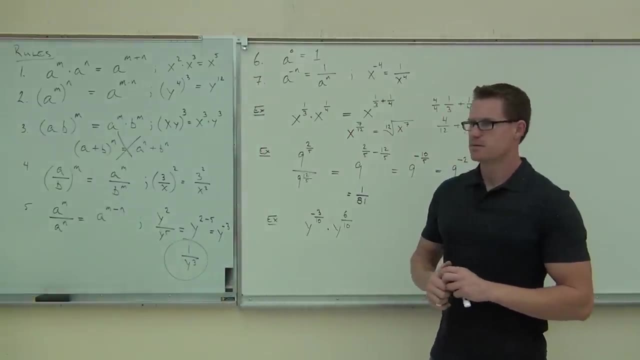 Hey again, what situation are we? Let's look closely at the board. What one are we? What are we looking at? What are we looking at? Oh, like here, We're still at number one. We've got common basis, We're multiplying, That's. 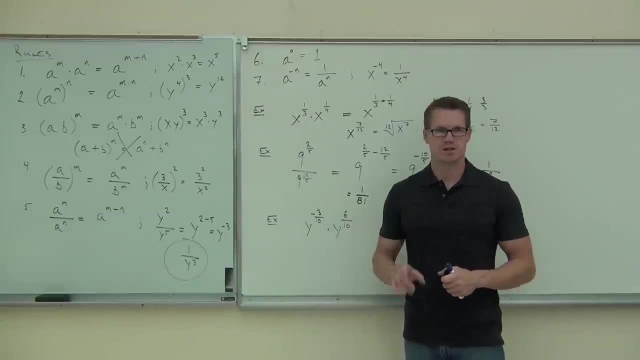 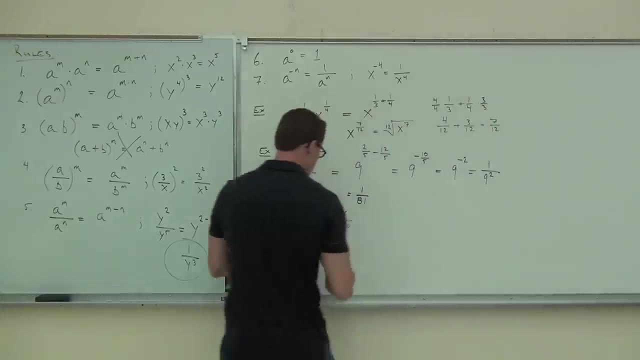 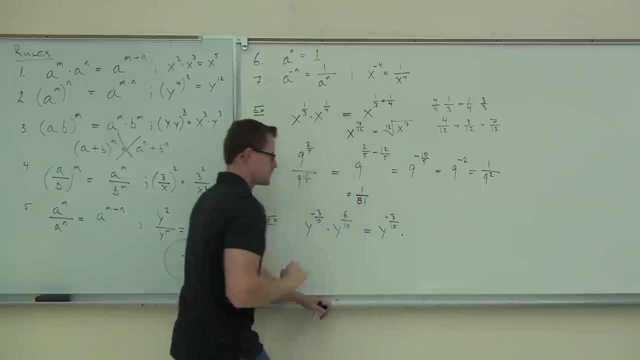 definitely number one. What are you going to do with these exponents folks? You can add them. Even though one's negative, that's okay. You can still add them together, That's fine. So we know we're going to have y to the negative three-tenths times y to the six-tenths. 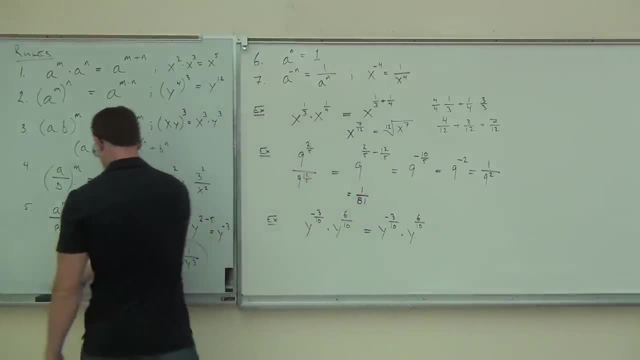 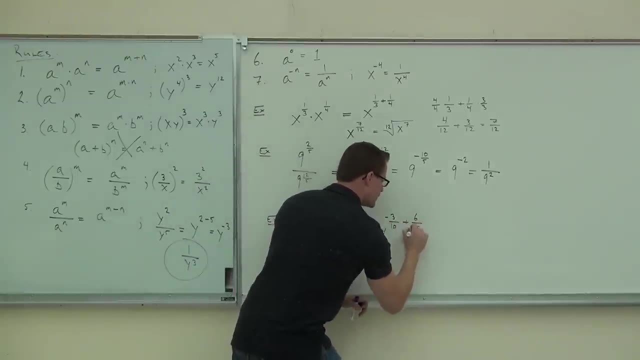 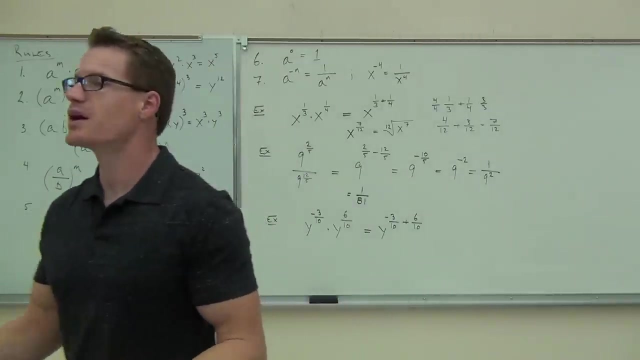 times y I just wrote the same thing twice. Since we have this common basis, we're multiplying. we know we're going to add the negative three-tenths and the six-tenths. What's great is we already have a common denominator. If you don't have a common denominator, you've got to find one. 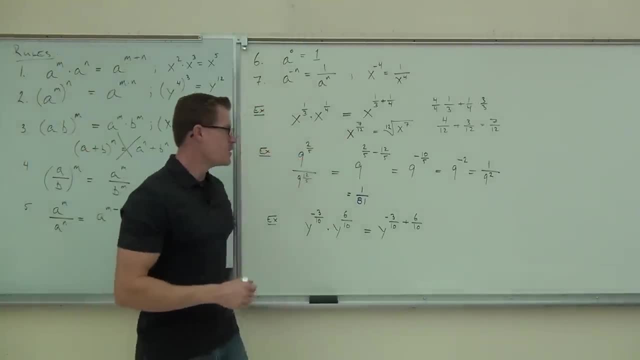 if you're adding fractions. That's what we did in this first example. But now that we have negative three-tenths plus six-tenths, how much are we going to have Positive three-tenths? Okay, very good. 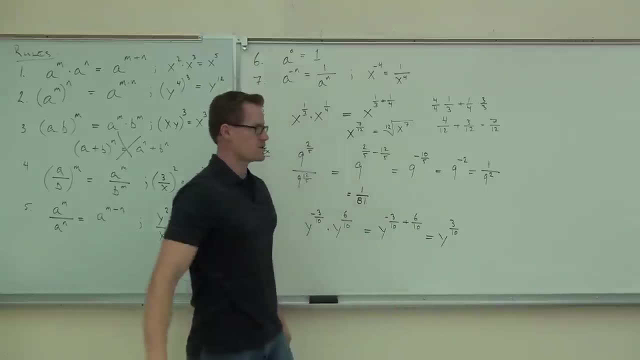 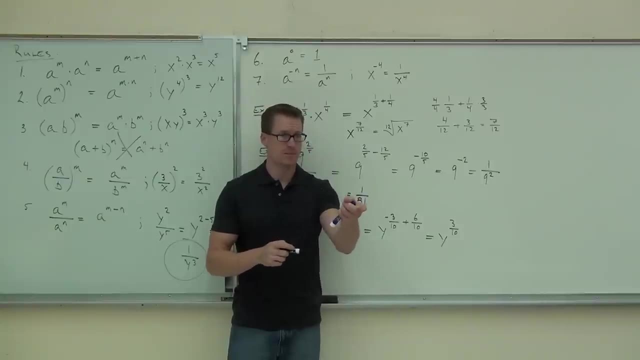 Add those together, you get three-tenths. Could you write this as a root? Yes, Tenth root of y to the third: Good, yeah, tenth root, because that's our denominator and the power is the numerator. so we would have that exact root. 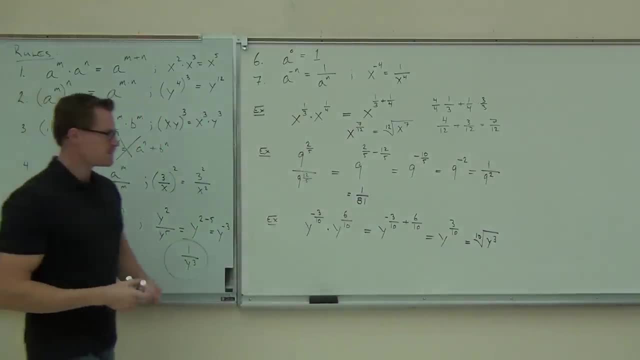 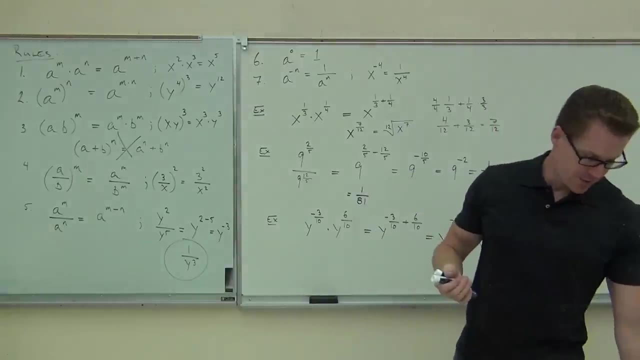 That's as far as we could go. Would you really feel okay with these ones so far? All right, We're going to try a couple more together. I'll give you several to do on your own and I'll make sure that you guys can do this. Then I'll move on and I'll show you how we 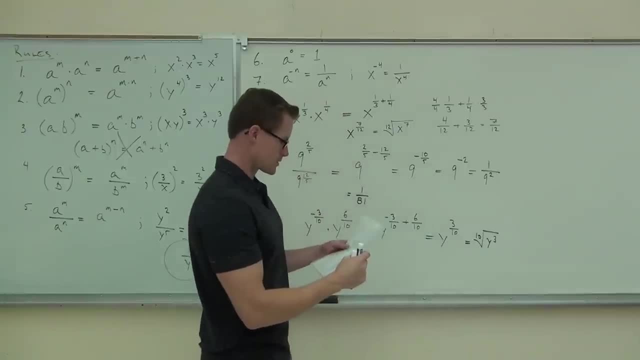 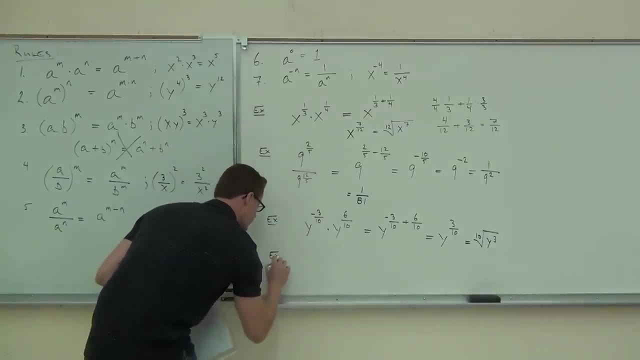 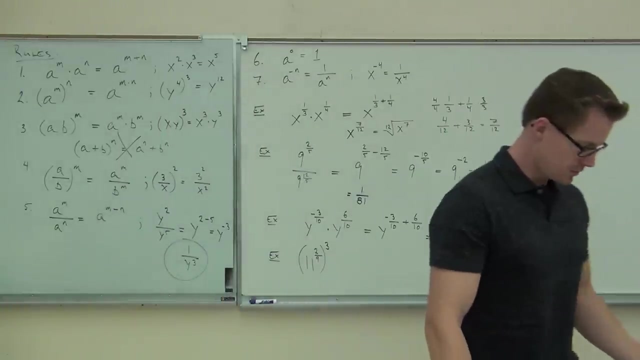 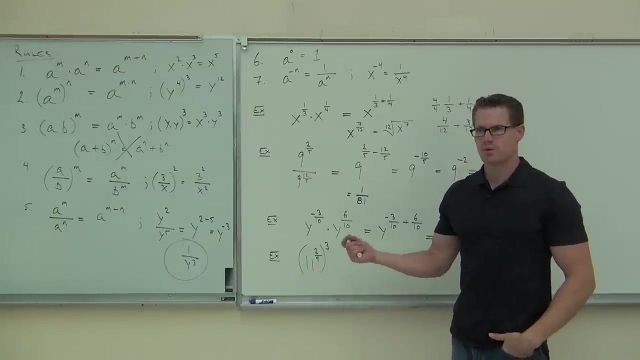 can really apply this stuff. some unique ideas Here. it is: Eleven to the two-ninths, Eleven to the third power, Eleven to the two-ninths, all raised to the third power. What do you think about this one? What rule are we for that? 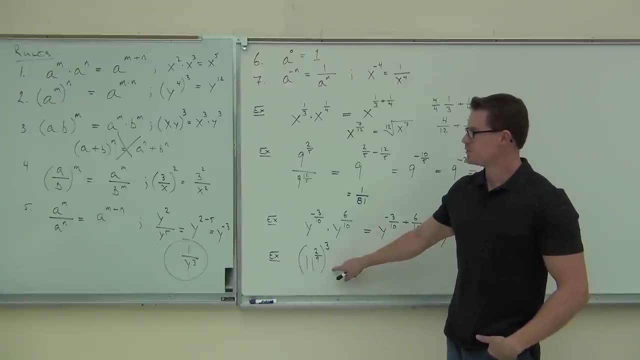 Number four. Number four would be a fraction raised to an exponent. We don't really have a fraction, We have. that's an exponent, right, And that's an exponent Which one is that Two? That's number two, That's right. 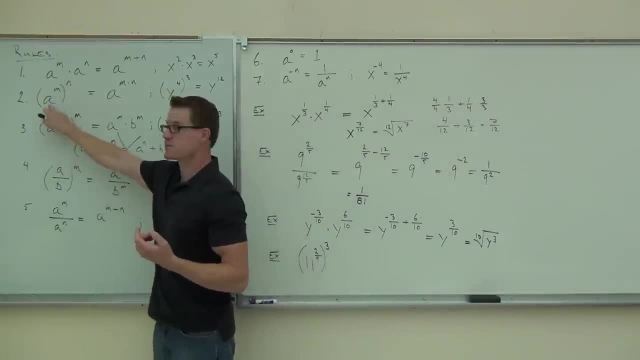 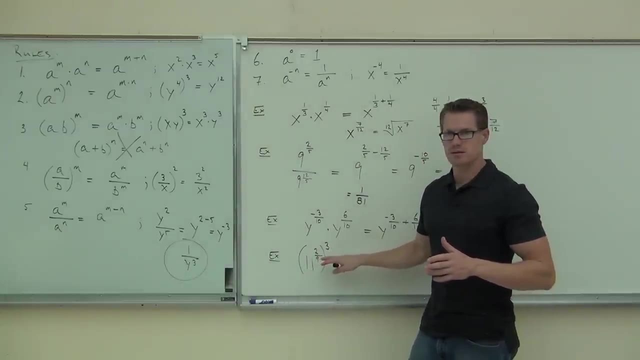 This says an exponent raised to an exponent with some number or some value. We have some value. We have an exponent raised to an exponent. Do you guys see it? I have a question. Yeah, How come you don't know? the third power to the base? 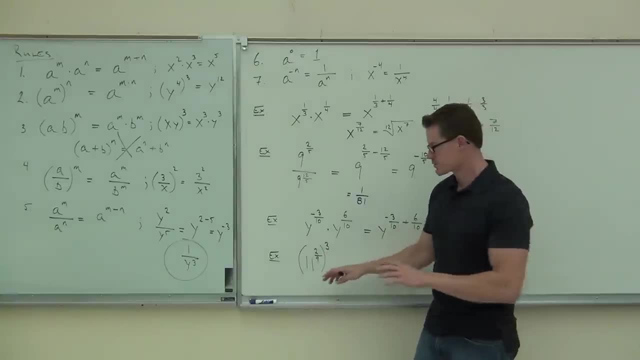 This one to this one. Yeah, You are. You are, because what you're doing here is this means 11 to the two-ninths. This would be 11 to the two-ninths times 11 to the two-ninths times 11 to the two-ninths. 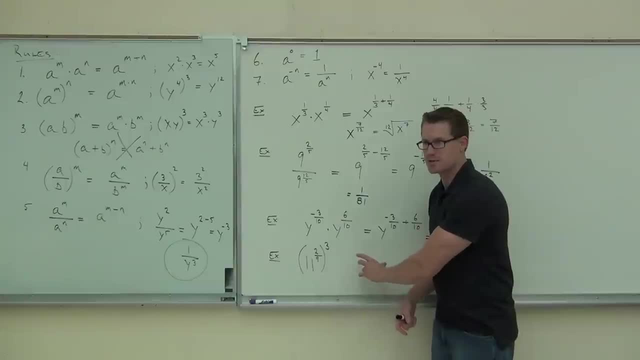 Oh, Does that make sense? Yeah, And when you do that, you don't multiply the 11's, they're already being multiplied. You're taking those exponents and you're making it so that you don't really have to deal with. 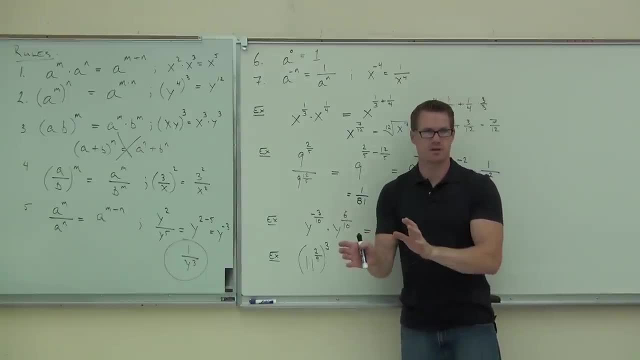 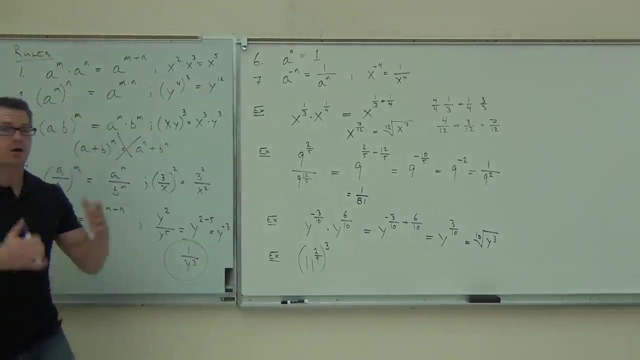 the 11's. you're dealing only with the exponents. Indirectly, you are dealing with the 11.. Does that make sense? Yeah, You are doing that. Okay, 11 to the two-ninths, to the third power. What are we going to do with those exponents? 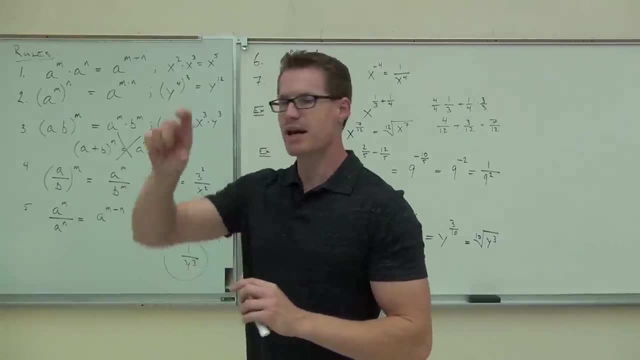 folks. Multiply them. Definitely multiply them. Yeah, we have an exponent raised to an exponent there, Exponents raised to an exponent. So we're going to have sure 11 is still our base, Yeah, Okay, So you have 11 to the two-ninths, to the third power. What are we going to do? 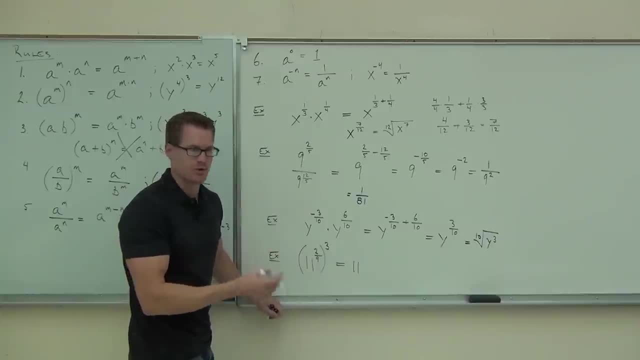 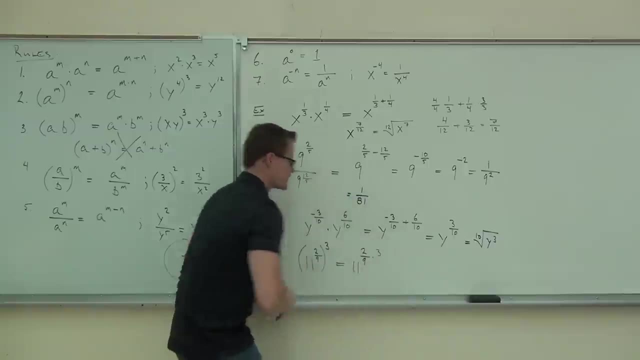 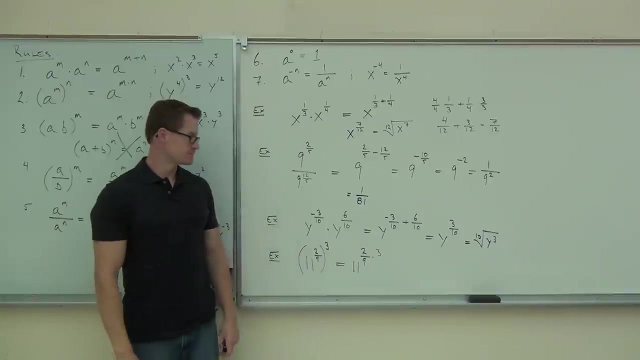 The base doesn't really change when you're dealing with exponents. but up here for our new exponent, we'll have 2, 9ths times 3.. We're multiplying those exponents, Yes, no, Yeah, Okay, How, What are we going to get? 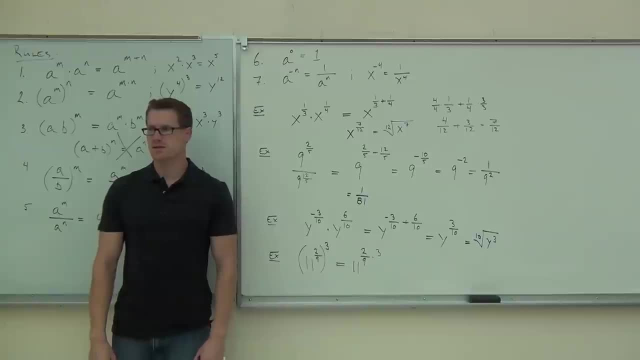 6- 9ths. Okay, 6, 9ths, sure. Can you simplify this like you would any other fraction? For instance, this is 3 over 1.. Could you simplify that? Sure, What simplifies out of that thing? 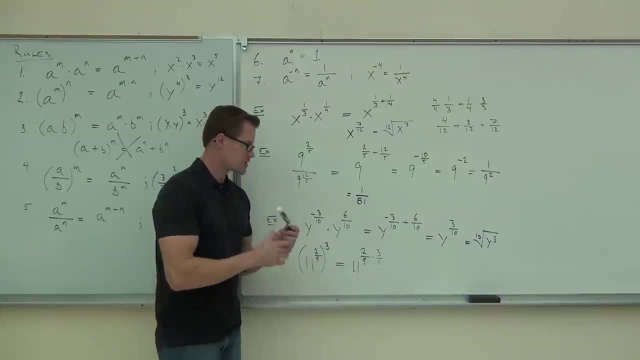 Okay, you could get 6 9ths, but then you'd have to reduce that. If you simplify this, you know 3 goes into 3 one time, 3 goes into 9 three times and there that's going to give you the 2 3rds that you would reduce that 6 9ths into. 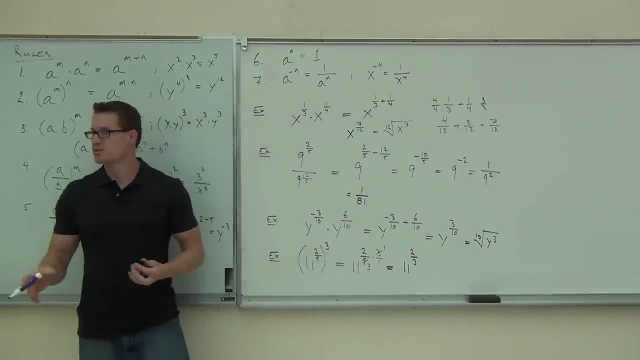 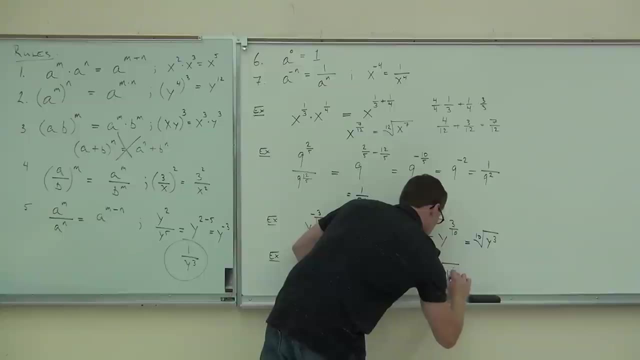 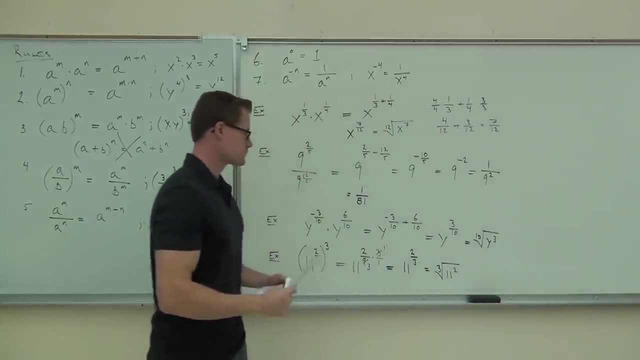 11 to the 2, 3rds power And again we could write that as a root. This is a what type of root, folks? Cube root of 11 squared. You could do a cube root of 121, but you can't go any further with that. 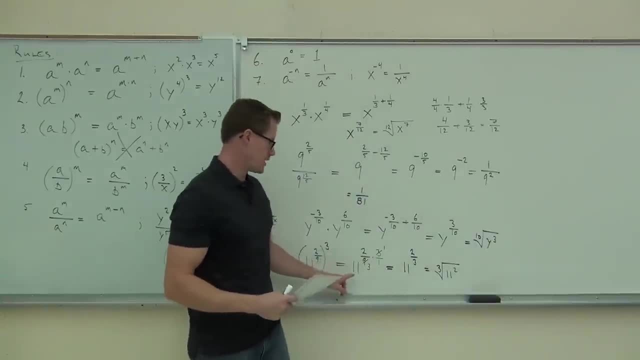 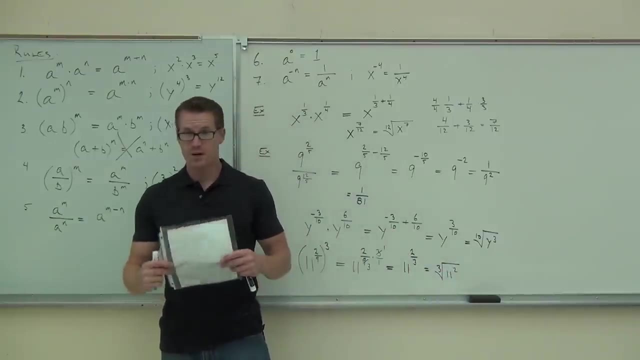 So, either way, I don't really care. I just want to make sure you're okay on getting at least this far and understanding that this can be written like that. That's really what I care about. Are you ready to move on? Okay, we're going to start combining some of these rules together so that we're not just doing one. 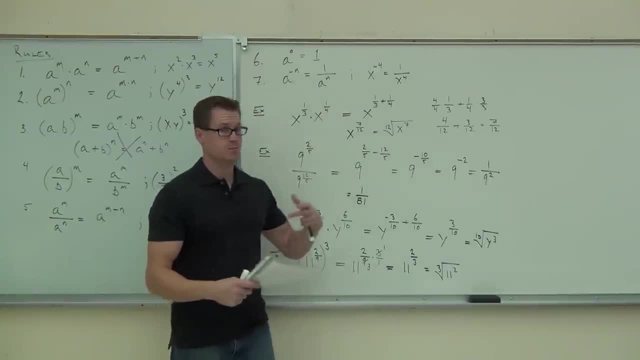 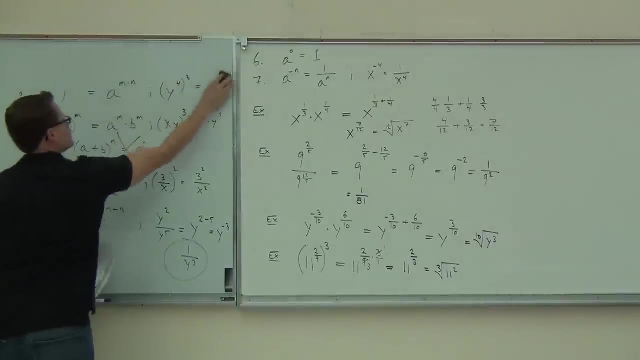 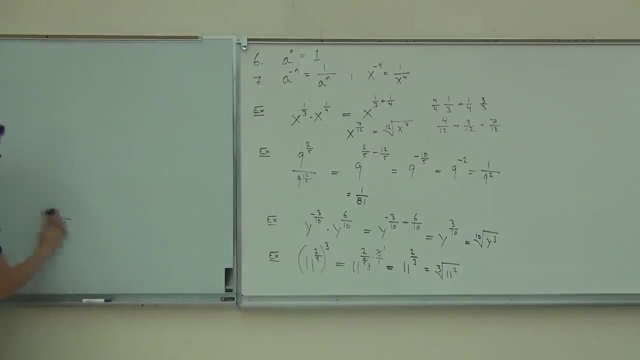 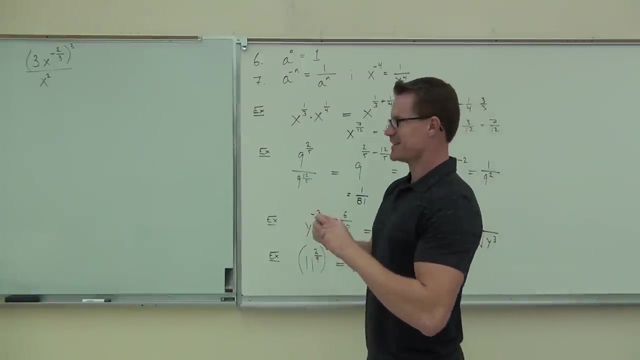 Here. we've just done one rule four times. Now we're going to start putting this all together. We're going to do one rule five times. That was a nice looking one. huh Yeah, That's what you like to wake up to in the morning. 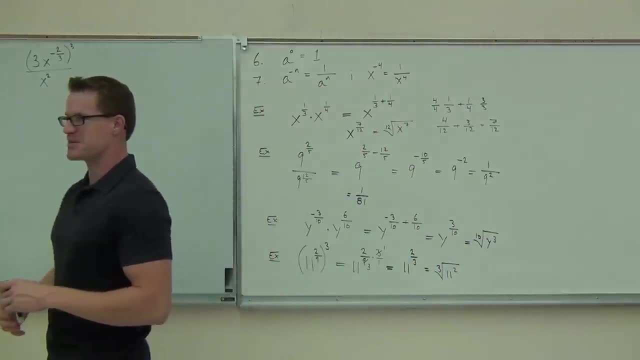 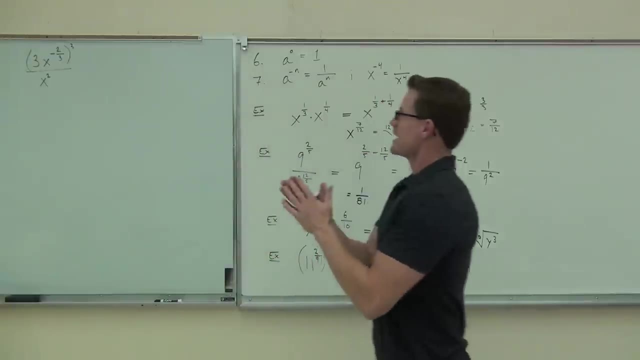 That's it right there. Nice cup of coffee and some math. Best day- That's what you're going to do tomorrow. I bet I don't think I'm going to do that tomorrow. So we have three x to the negative, two-thirds two to the third power and then x squared. 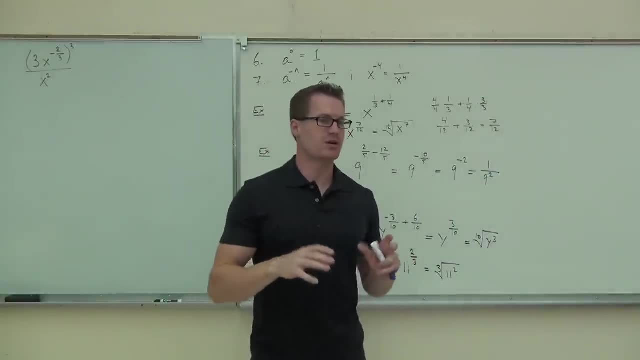 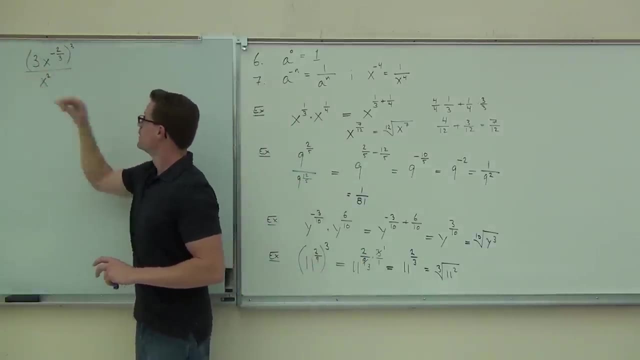 First thing we're going to deal with is very much like order of operations. You're going to get rid of any parentheses that you see, So we're not going to deal with this x squared until we do all this stuff up here. You with me on that. 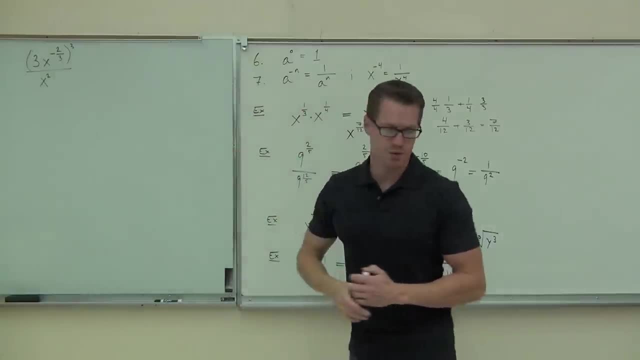 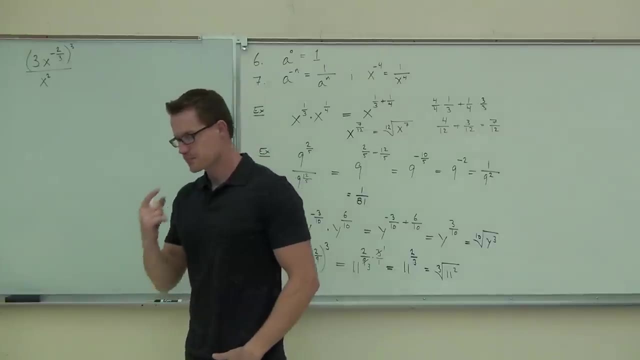 So let's deal with all that stuff up there. Now, going back to your rules, I want you to look at rule number three. So look at rule number three. On rule number three, it says: if I have some things, some terms, some factors being multiplied together, 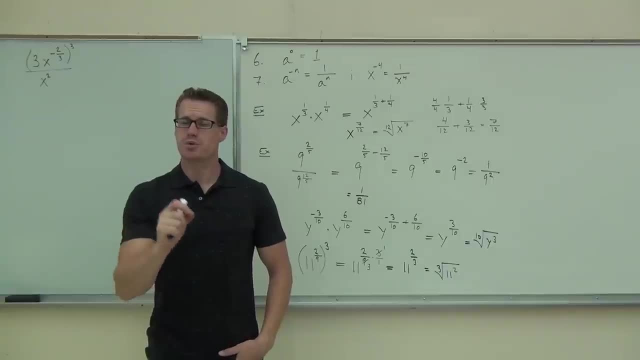 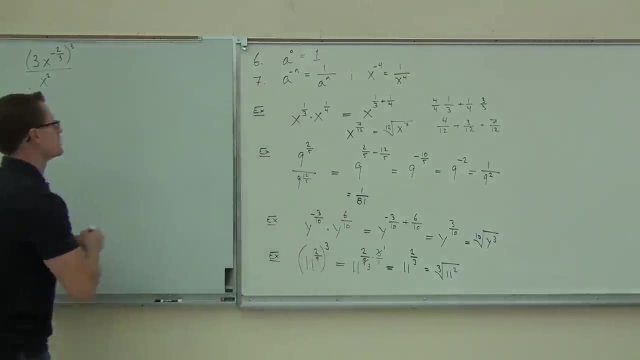 and set in my parentheses, and it's being raised to an exponent. each one of those factors gets raised to that exponent. Are you with me? I want you to look at what I have. What I have here is a product that's three times x to the negative two-thirds. 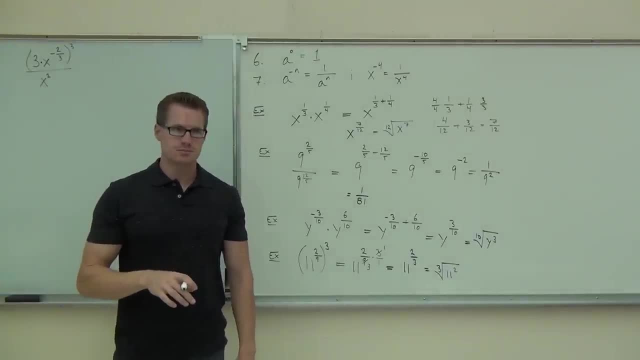 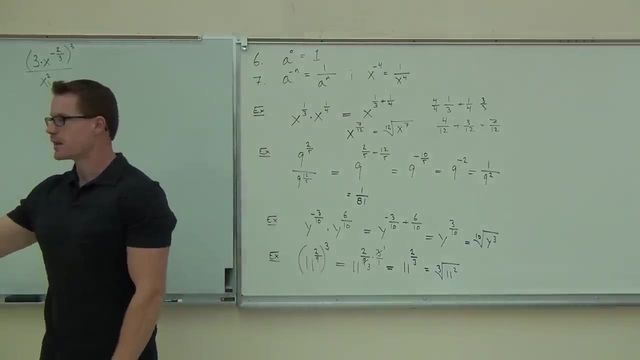 Are you with me, Mm-hmm? So what this says to you is that each of those factors- since three is a factor and x to the negative two-thirds is a factor- gets raised to that power. So what happens here is: we don't just get a three back. 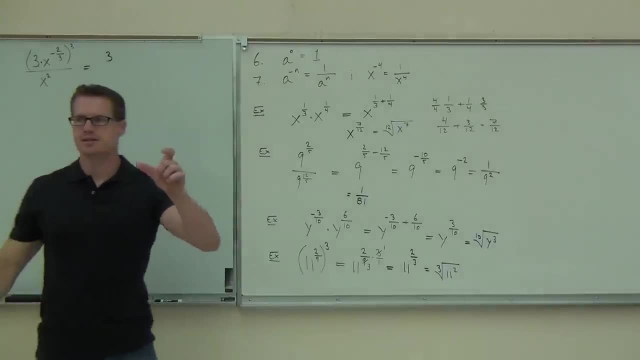 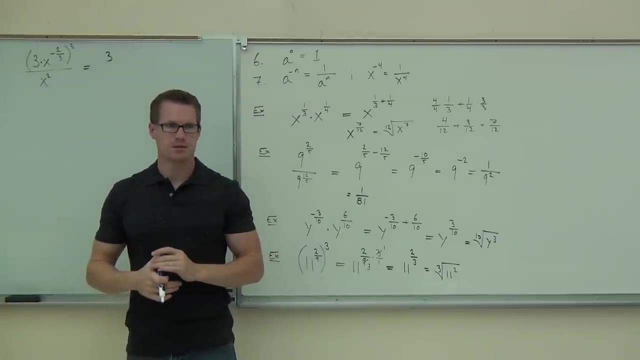 We don't just get a three. Since it's being multiplied there, it says that the three is also getting raised to the third power. Are you with me on that? So what am I going to have? instead of three, I'm going to have 27,, or three to the third. 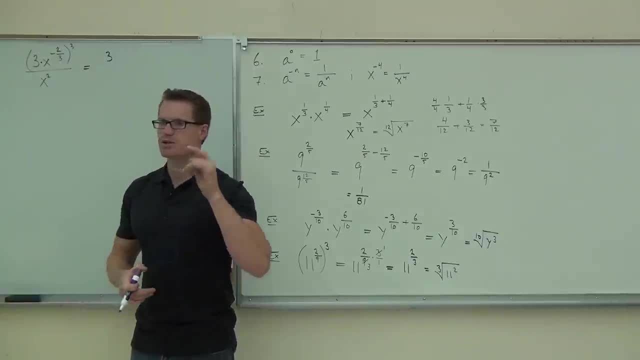 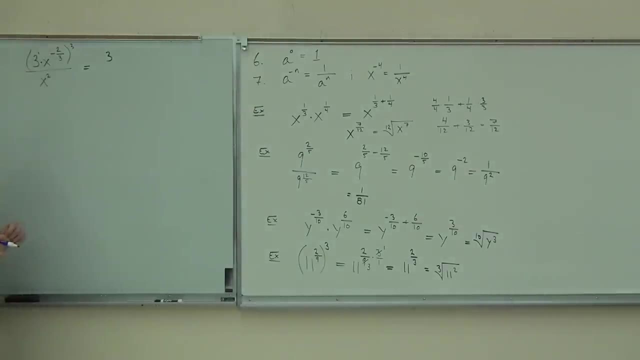 Now, how do we do three to the third? I want you to think about this. We're not just arbitrarily raising a number to a third power. Please watch carefully on the board. This is three to the first power. Are you with me? 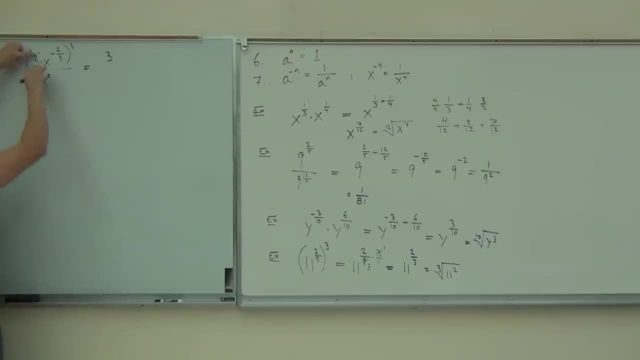 So, really, what you're doing? you're saying, oh, I have three to the first, two to the third, What's one times three? That's how we're getting three to the third. That's how we're doing it. We don't just say, oh, we're taking it to the third power. 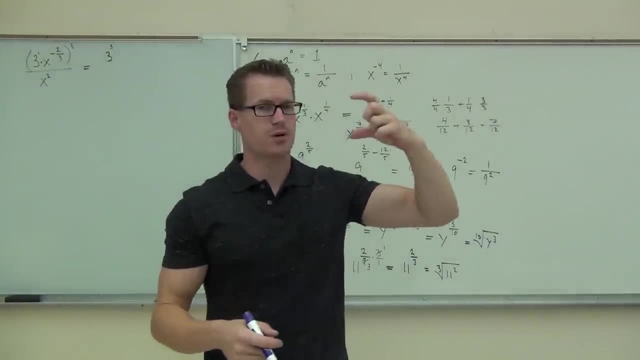 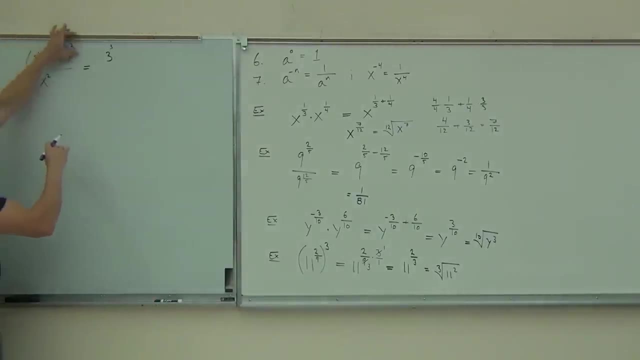 The product of those exponents still works for us. When you have an exponent raised to an exponent, we do multiply every single time. You just need to know that this three to the first power is also being raised to the exponent. That's how we're getting three to the third. 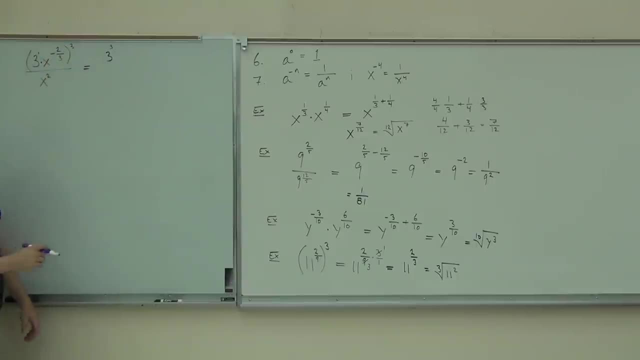 Not sure if you're okay with that. Okay, that's good. Now we do have something else in there that's being raised to the exponent. We have x to the negative, two-thirds to the third power. What are we going to do? 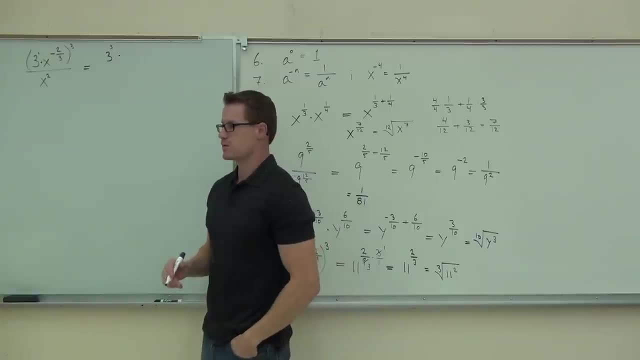 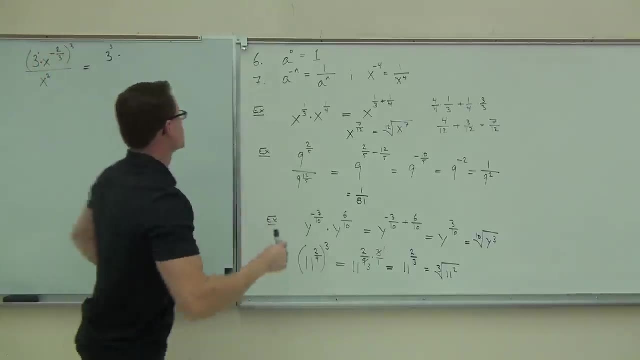 Add, subtract, multiply or divide those. What do you think? What do you think? We're definitely not going to add them right. There's no common basis. We have an exponent raised to an exponent that says we're going to multiply those things. 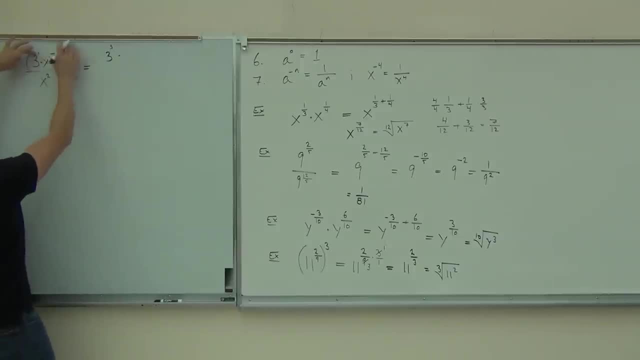 So here we multiply the one times three. That's just the first power. We add three to the third. Now we're going to add x to the negative two-thirds times three, And of course we're not even going to worry about that. x squared so far. 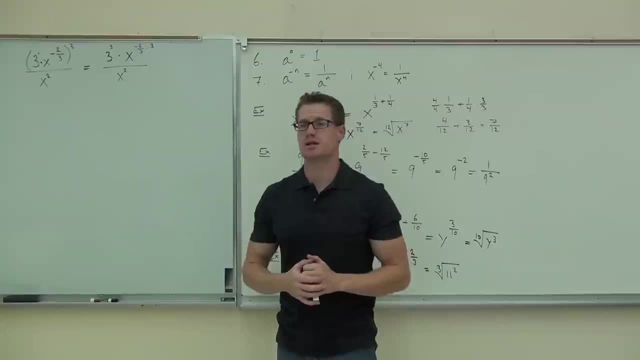 Okay, that's kind of a big step for a lot of people. I want you to really take a look at it. If there's questions, you need to let me know right now. Are you okay that we're going to have three to the third power, not just three? 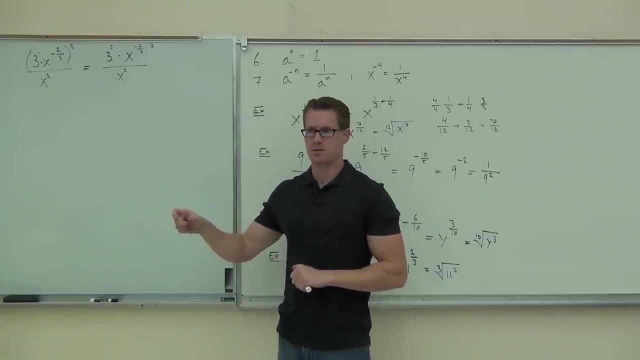 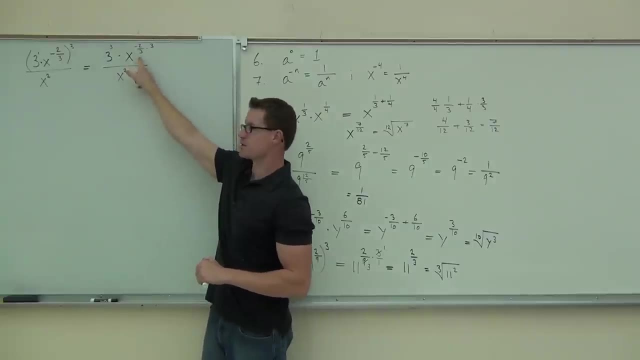 Are you okay why we have three to the third power? Because x squared is one. We're multiplying that times a three. That's how we get three to the third. Are you okay that these two things need to be multiplied and that's what we're getting? 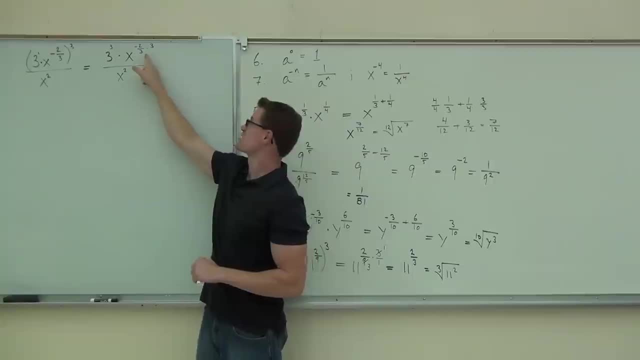 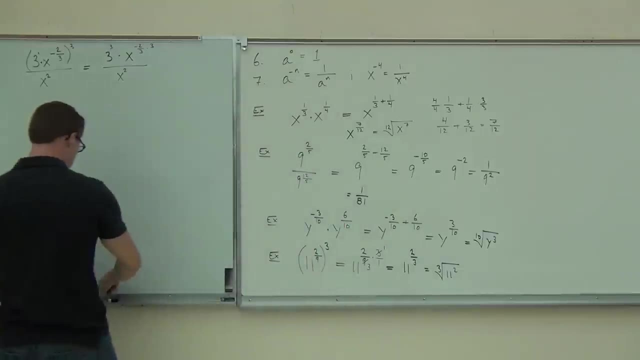 here. Yes, no, All right, Does this simplify? Yeah, How much are we going to have out of that? Yeah, those threes, Those are gone. This is like three over one. We can simplify fractions like you were taught a long time ago. 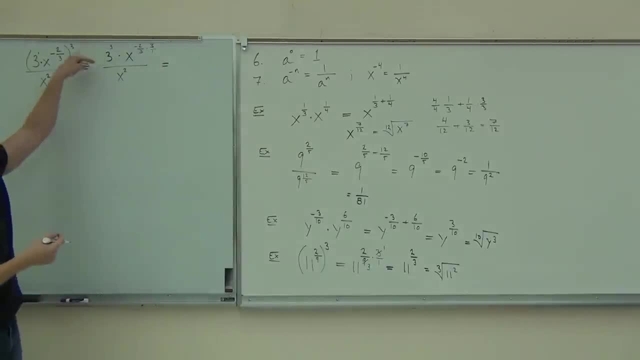 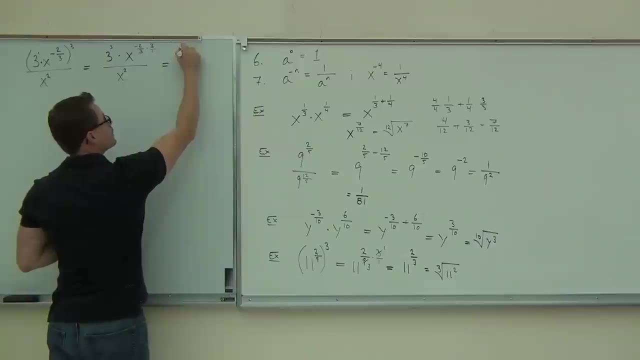 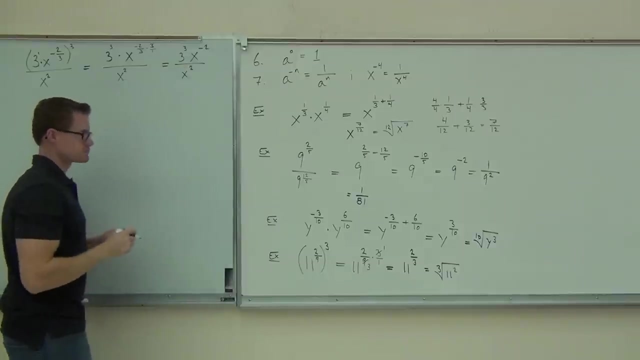 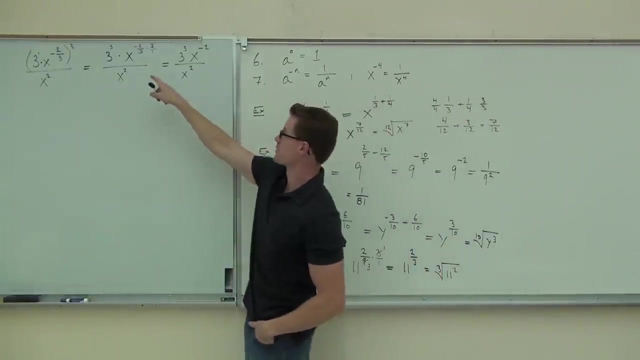 By the way, I'm going to leave this in terms of the power, just so you can see this all the way down. You can write 27 if you want to. I'm just going to leave it three to the third for now, Just so you can see for that one step of that. three to the third, it's still there. 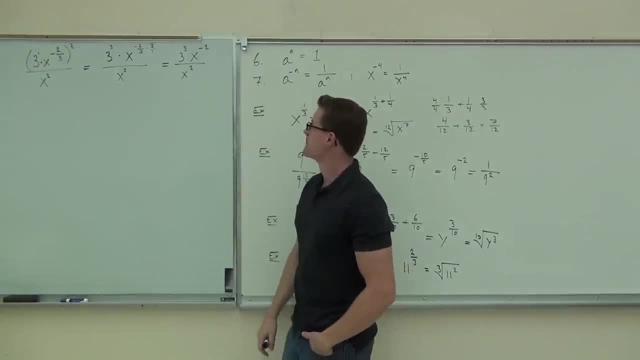 I'm going to change it to 27 in the next step. Hey, is there anything else that I can do? I could. There's actually options here for you. You can do two things. You can do two things: Watch on the board. 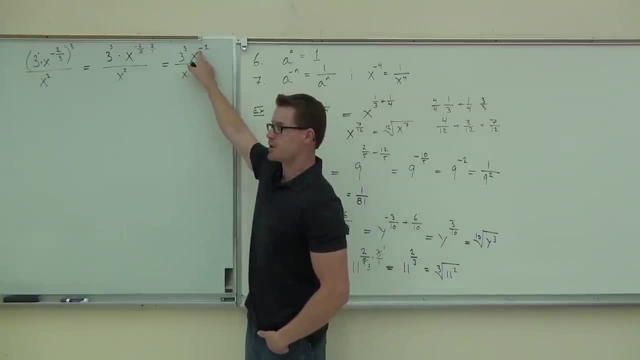 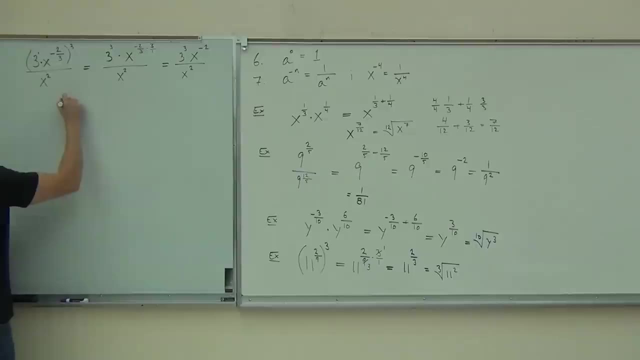 Since that's a negative exponent, you could move this to the denominator of the fraction. If you did that, what you would get is three cubed over x squared times x squared. Do you see where that x squared is coming from? That's this one. 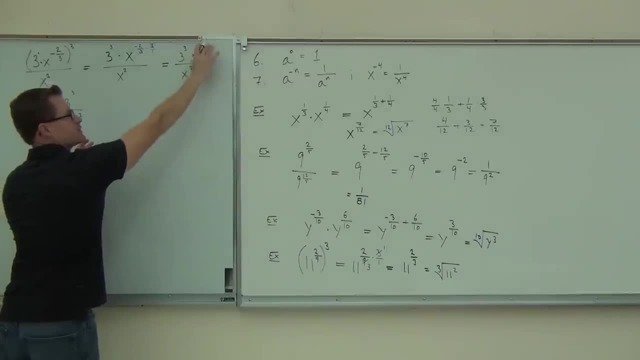 That's moving to the bottom. Remember this is multiplied and we moved that to the denominator. It's still going to be multiplied right here. If we move that to the bottom, it becomes a positive exponent. Are you with me on that? 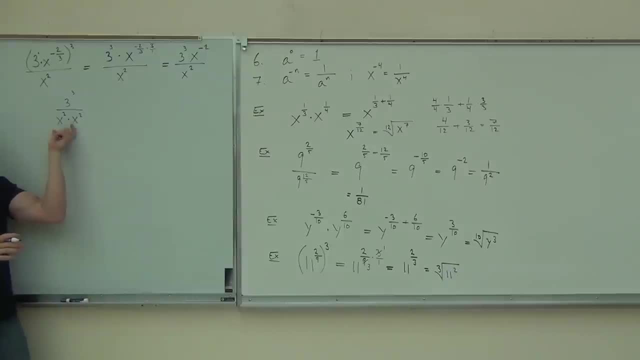 Then could you combine these. That's going to be x to the. what Good? We add exponents for that. That's x to the fourth. Or you could think of it like this: You have three to the third To combine these exponents. ignore that for a second. 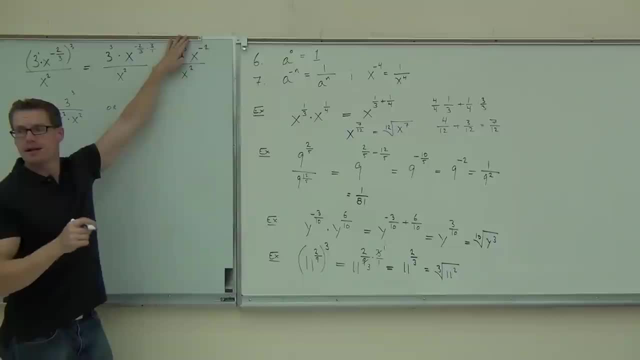 That's x to the negative, two over x to the two. How do you combine exponents when you're dividing common bases? Subtract: You'd have x to the negative, two minus two. Do you see where the minus two is coming from? What was that rule? 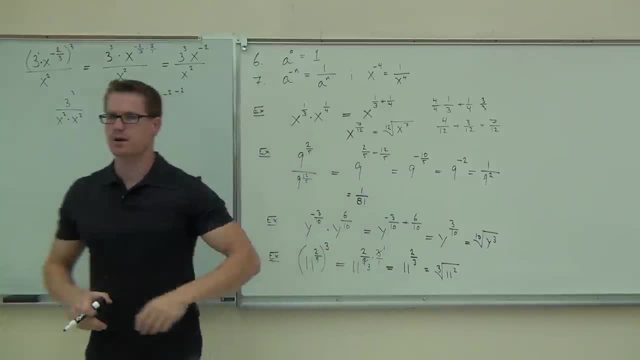 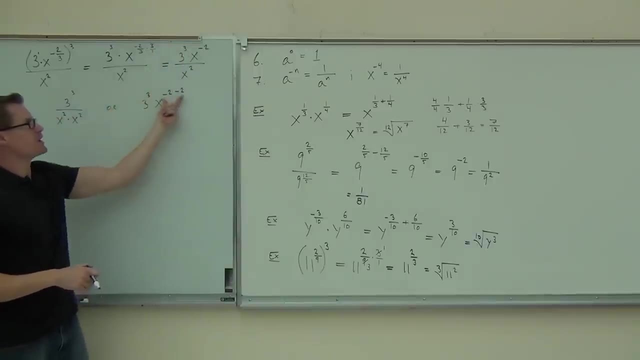 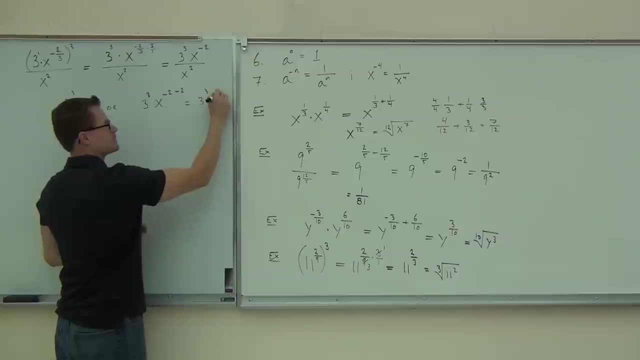 Rule number? That's rule number five. You're right, That would be rule number five. It said you have common bases being divided. You subtract top exponent minus bottom exponent. How much is negative? two minus two? Three, cubed x to the negative four? 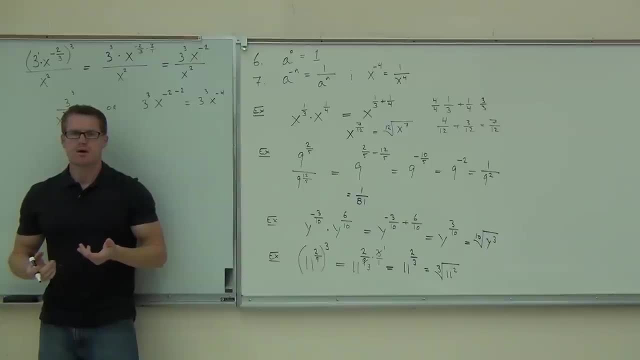 Is it going to work out the same? Which one do we move to the denominator? Do we have to move the three to the third? That's a positive exponent. Leave it. This is x to the negative four. That one would move to the denominator. 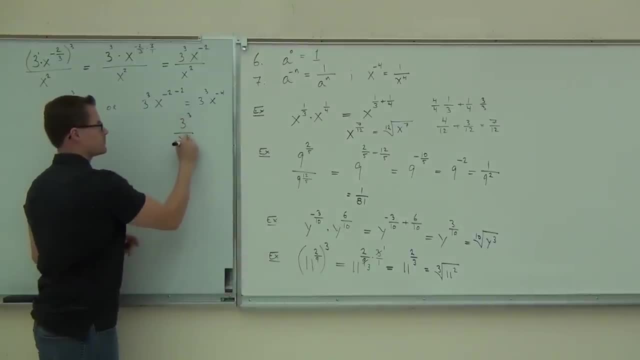 This would be three cubed over x to the fourth. This one would be three cubed over x to the fourth. Either way you'd get the same answer on that. We have options on this stuff. There's not one right way to do it. 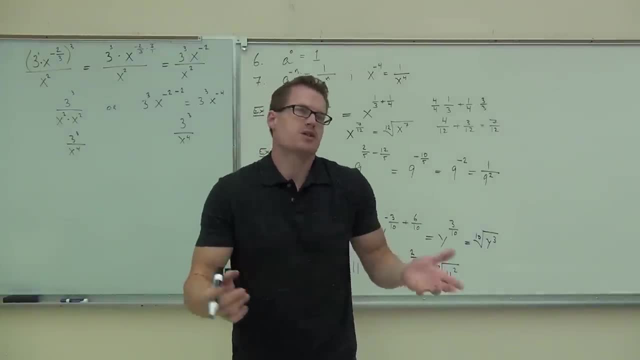 These rules. you can do them in different orders. provided you stick with the exponent rules, They're fine. It's fine. You get rid of your parentheses first and then we combine whatever we can. When you move the x to the negative, two down. 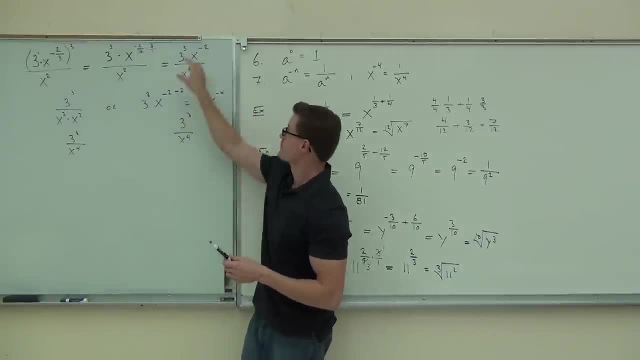 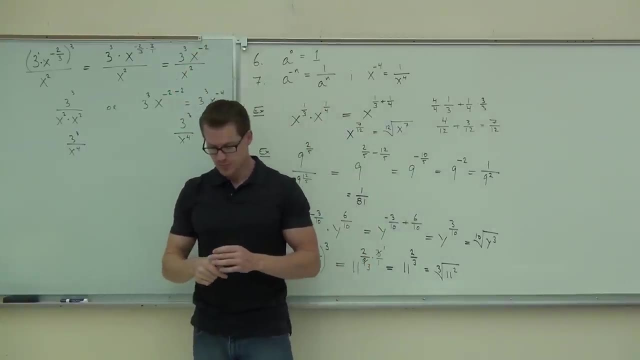 do you remove the sine two? The sine of the exponent will change if you change it from a numerator to a denominator. That's the whole idea for rule number seven. Make sure you're okay with this example. Good, I'm going to give you some to try. 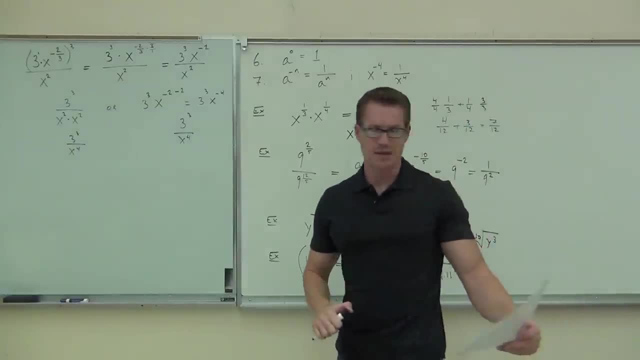 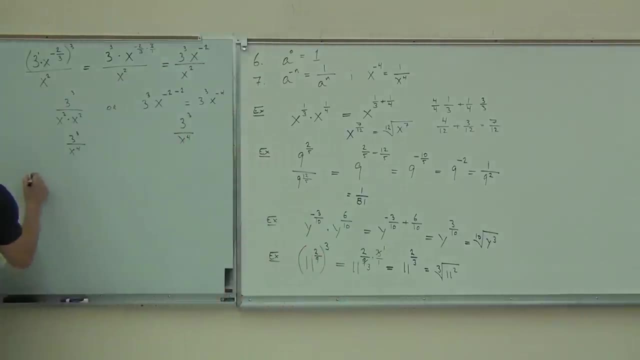 I'm going to give you some simple ones to start with, and then the last one I give you is going to be pretty nasty. You ready for it? There's one. There's two. Three, Two, One. There are two. 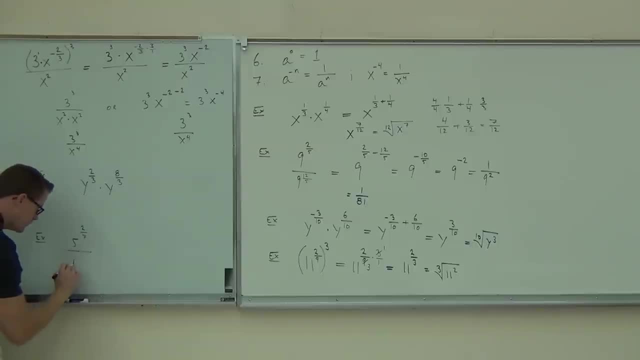 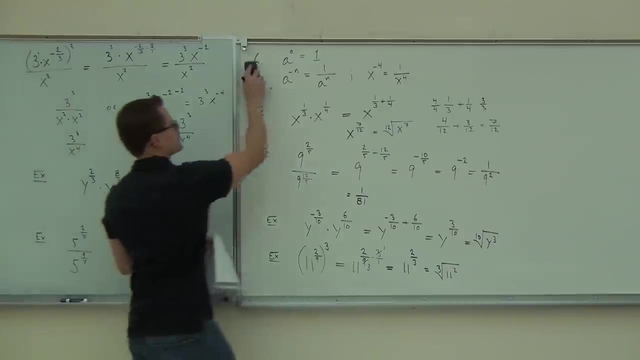 Three, Two. What's the number of things you're gonna go for? That's the number of things you're gonna go for. Yeah, there's some Three, Three, Three All the way across the left-hand corner. One. 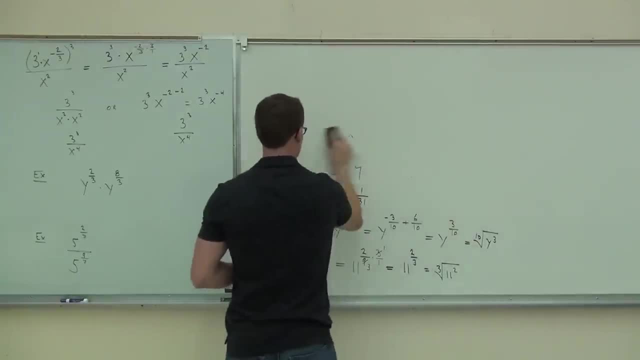 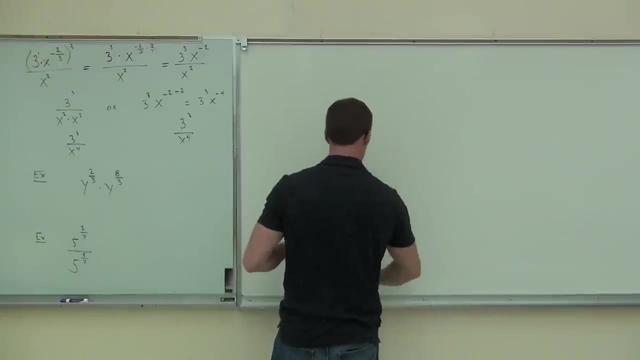 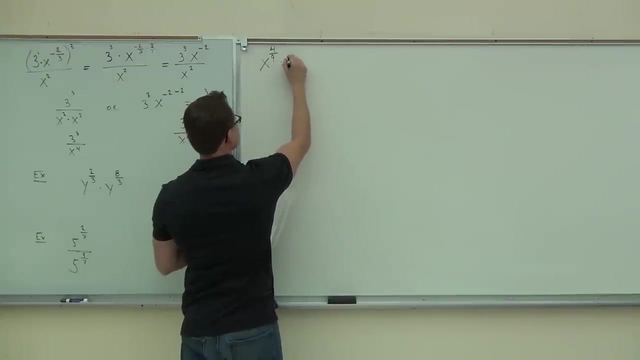 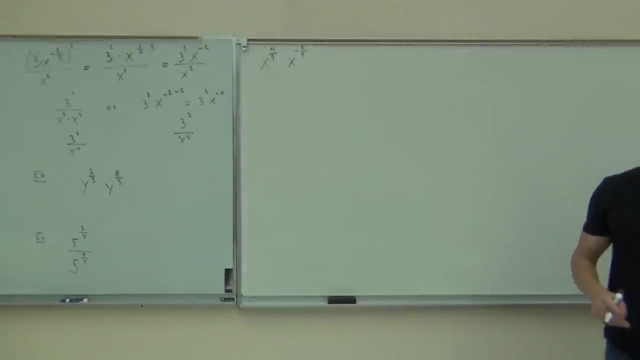 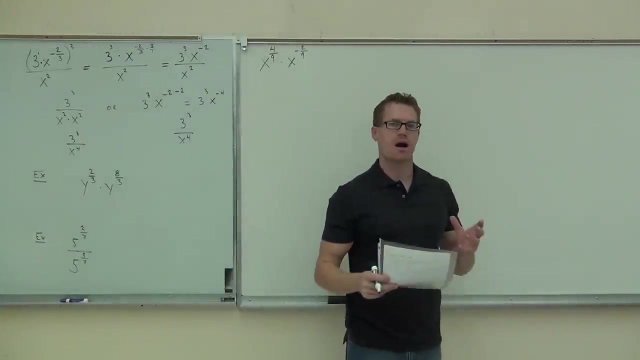 Three Two One Two, Three, Two, Three, Two, Three One, One, Two. I definitely want you to be able to do those three with no problems. These are just the basic rules for us. This next one is going to take you some time. 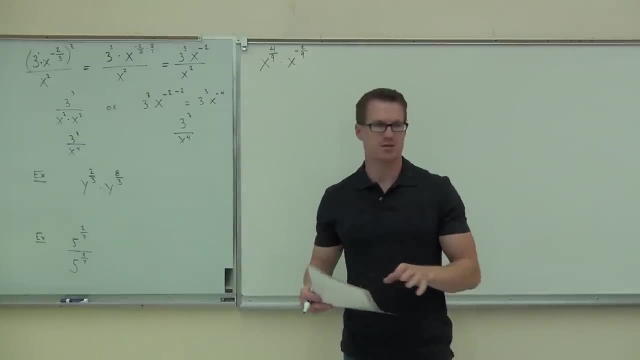 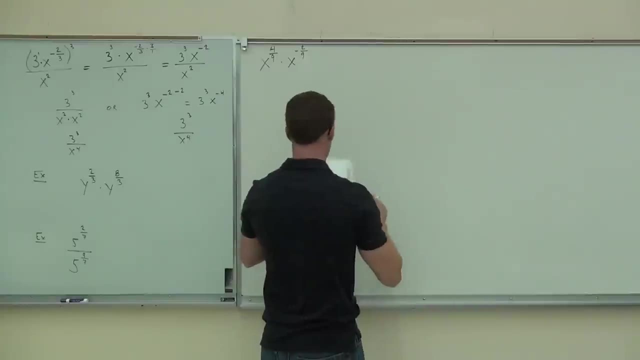 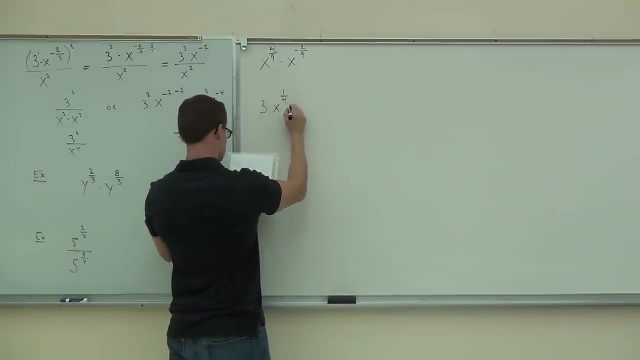 This is the one where I need you to get to. ultimately, You can do this last one I'm about to give you- You're set already as far as the test goes- on- this idea. This is where I need you to be the problem I'm about to put on the board. 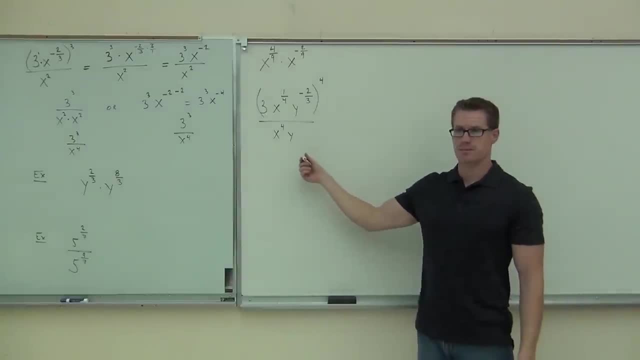 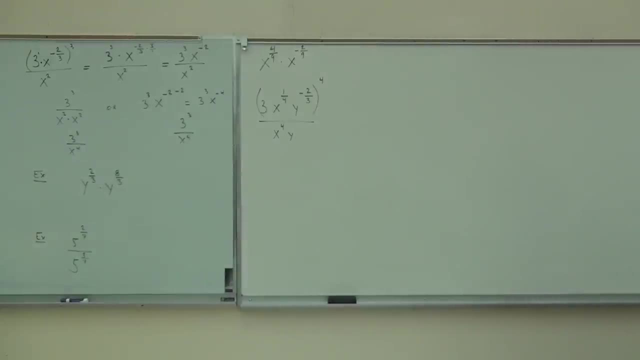 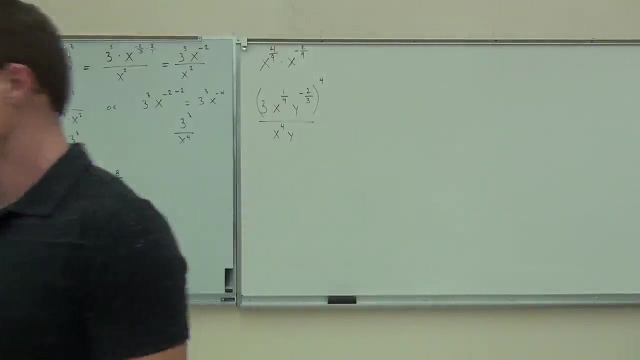 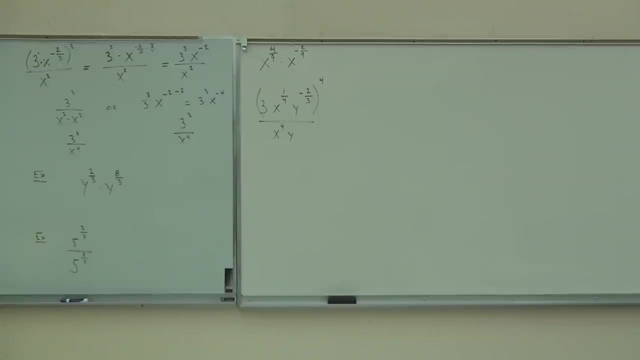 You will have a problem like this one on your test. Okay, Okay, Okay. So work them out, Work them out. So first three: no big deal, just kind of reviewing the excellent rules. Last one: big deal, Big deal. 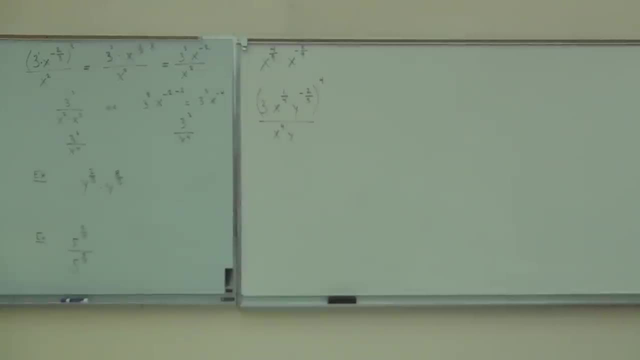 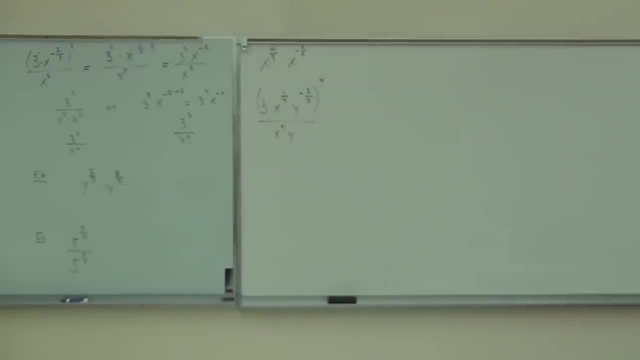 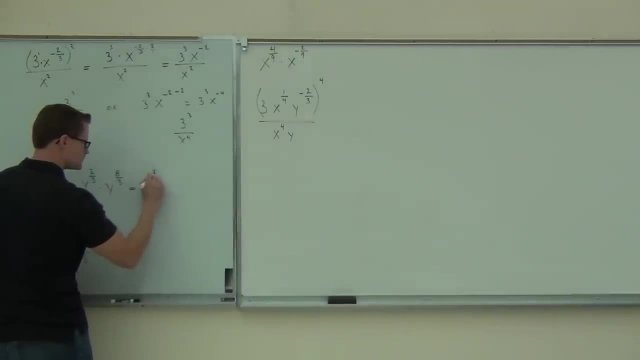 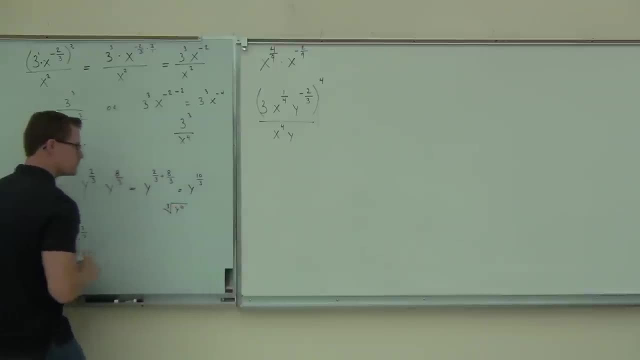 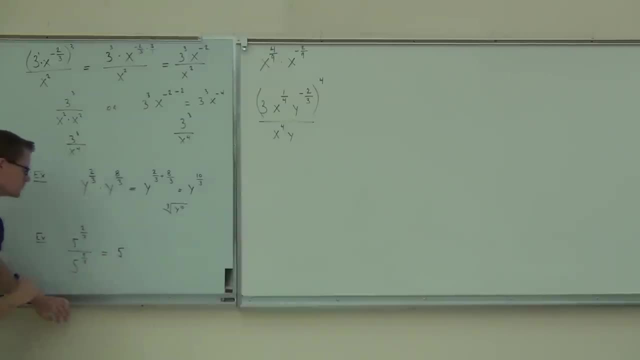 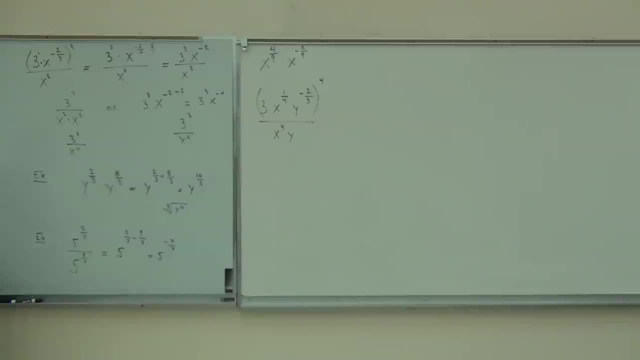 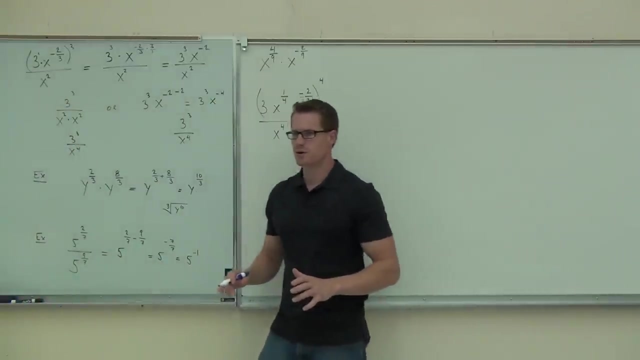 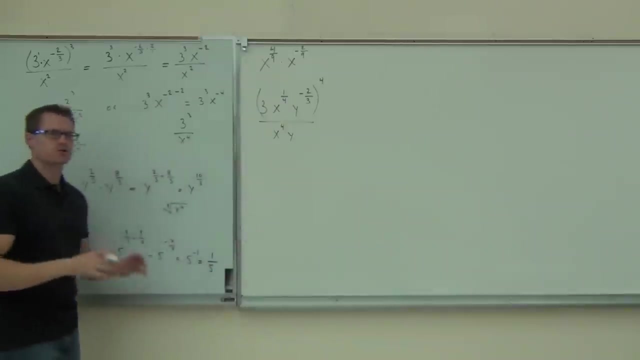 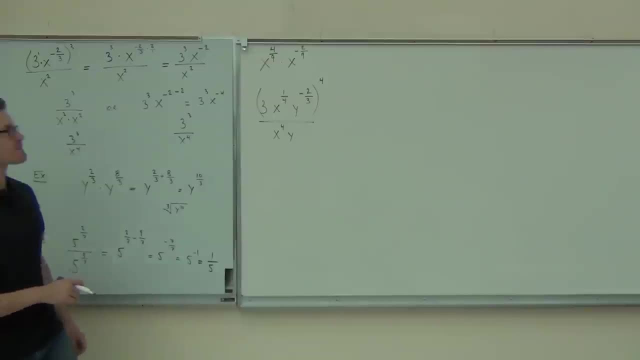 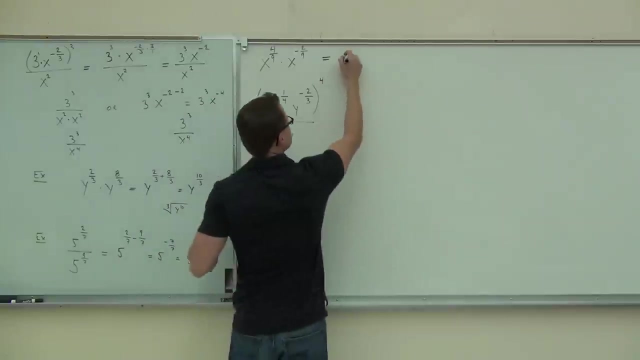 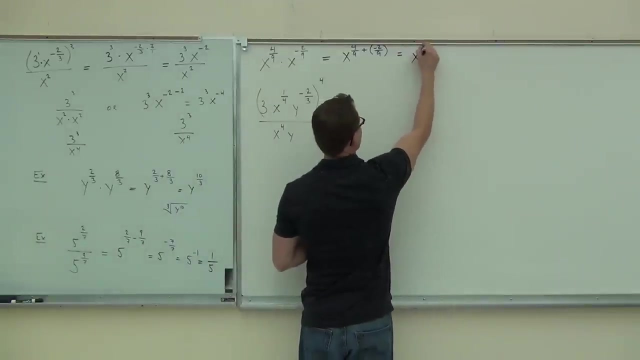 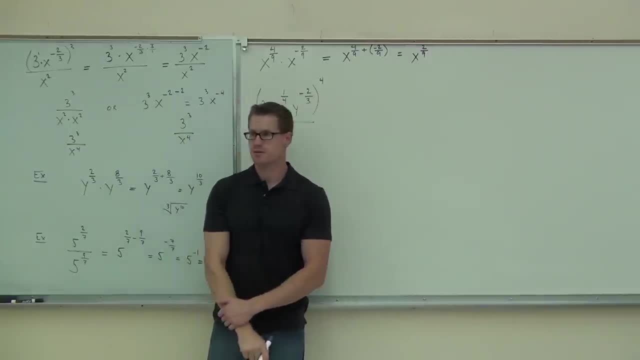 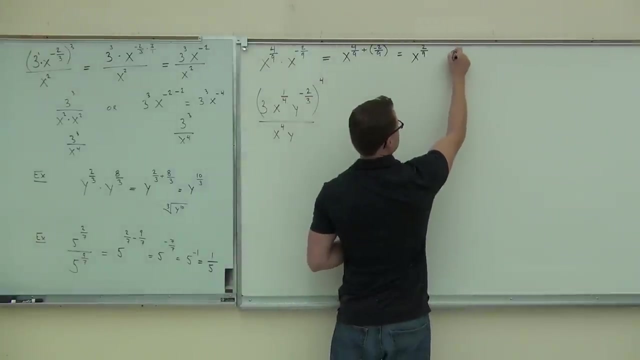 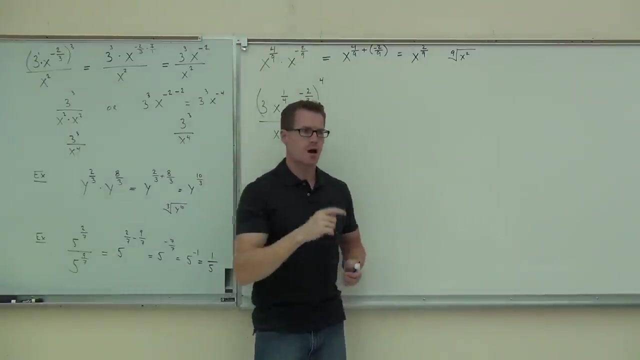 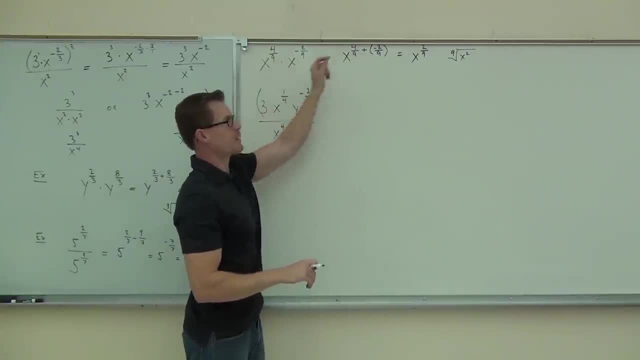 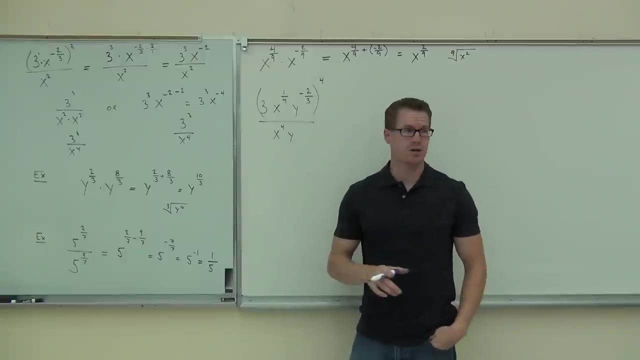 Was it a sign error? was it subtract or was it multiplying instead of adding? Those are the big ones right there looking for those. Are you okay on the first three folks? Are there any questions on the first three? Okay, now the last one. 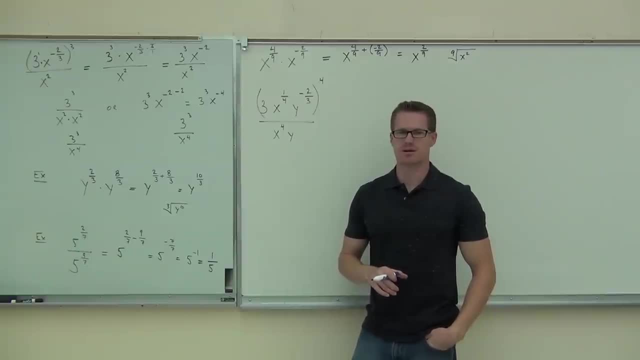 Last one's kind of fun, right. Lots going on here, lots going on. We've got big fraction, we've got huge parentheses, all raised to an exponent. What we're gonna do is break this down little by little. We're gonna completely ignore the denominator four now. 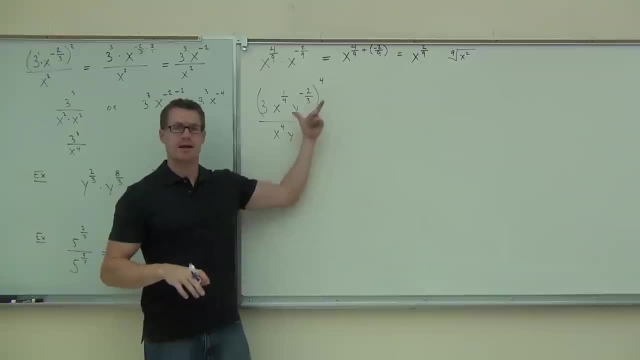 We're gonna wait until we get all of this stuff simplified as much as we can, and then we're going to include the denominator there. You with me, Let's do it. So we have this: large parentheses all raised to the fourth power. 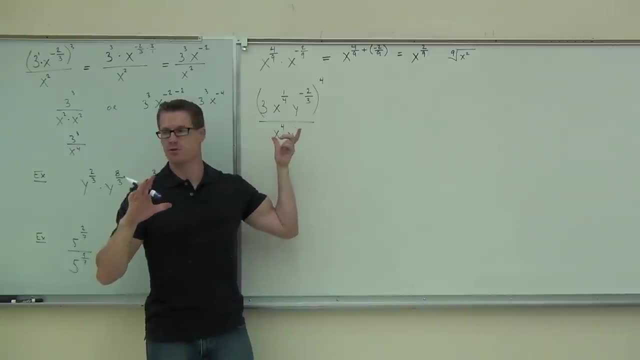 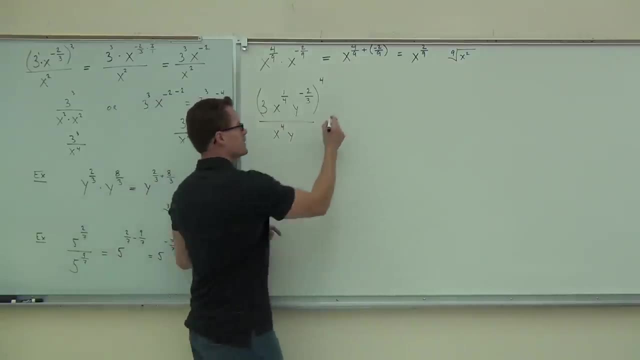 Can you tell me how many things inside of my parentheses are being raised to the fourth power or need to be Three? How many Three? So not just these two, we also have that number three, Don't forget about that. three. 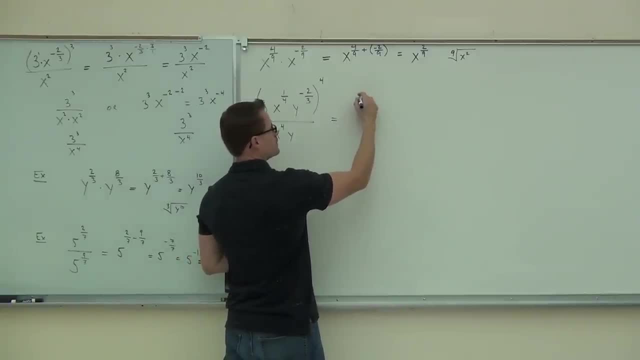 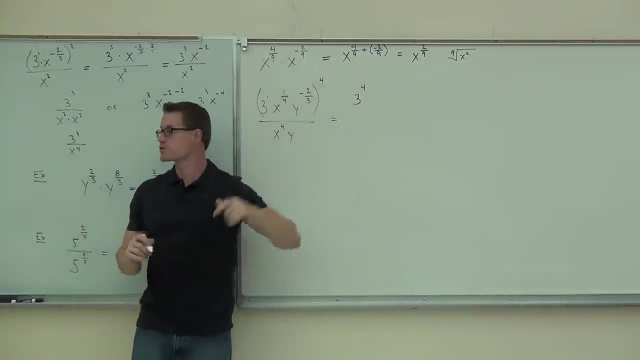 So we know that this is gonna give me what? Three over four. Good reason why that is is because I have three to the first power. I take an exponent to an exponent. an exponent means multiply one times four is four. 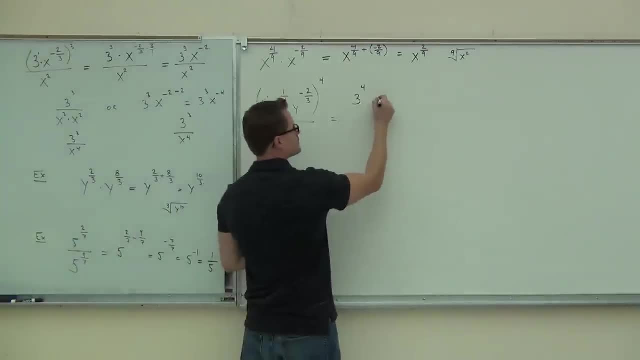 and that's why we get three to the fourth. Now here we have x. this is a one fourth power to the fourth power. we're taking an exponent to an exponent. you need to multiply that, So it's gonna be one fourth times four. 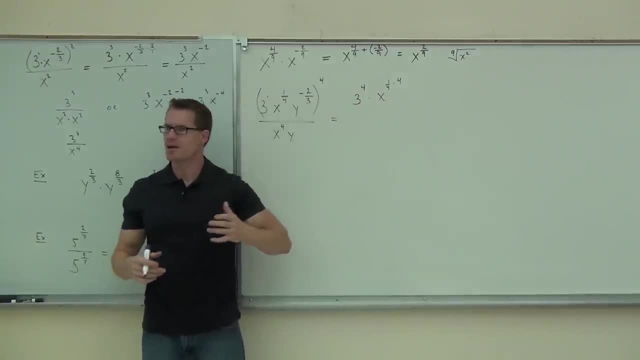 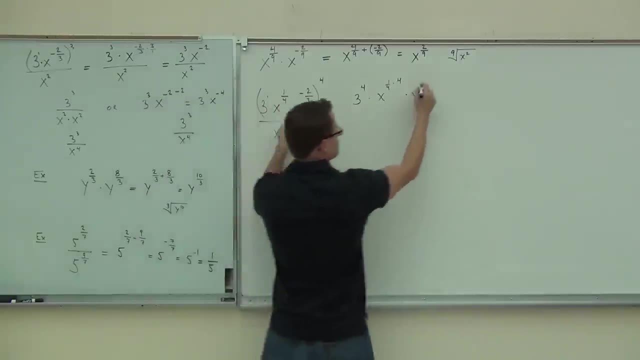 It helps to write this stuff out, Don't just do it all in your head. sometimes that's more tricky. Next time we get the y, we got all three things: y to the negative, two thirds. we're taking an exponent to an exponent again. 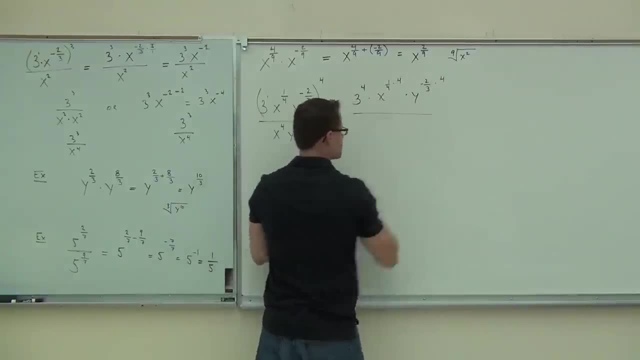 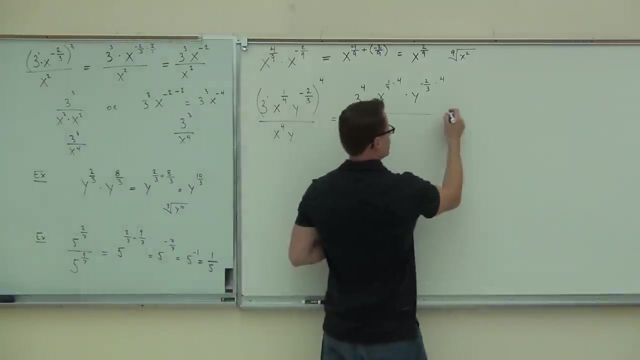 which means we need to multiply, And I'm just gonna put that denominator up there because we need to keep track of it. Did you make it that far? Good, all right, Let's see about those fractions. now I'm gonna leave three to the fourth. 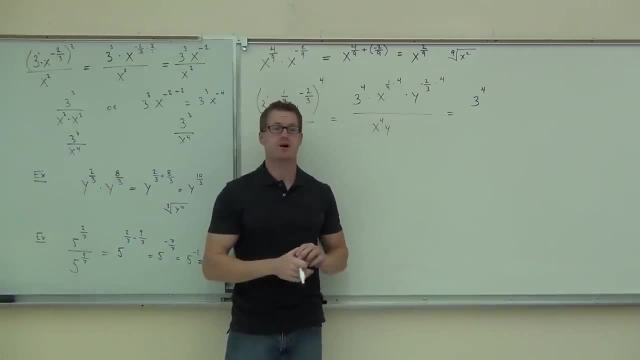 and you can put whatever that is 81 if you'd really like to, that's fine. In fact, on your final answer, it's probably gonna be 81.. Let's go ahead and simplify whatever fractions we can. We have one fourth times four. how much is that? 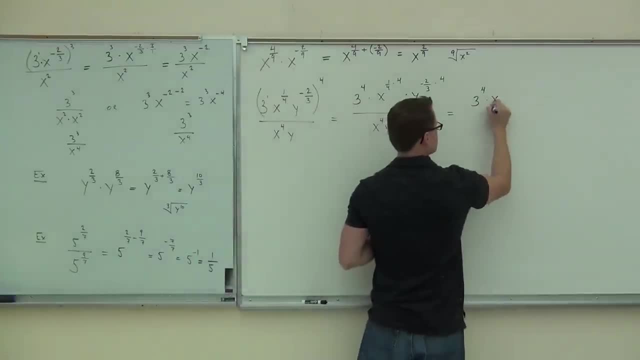 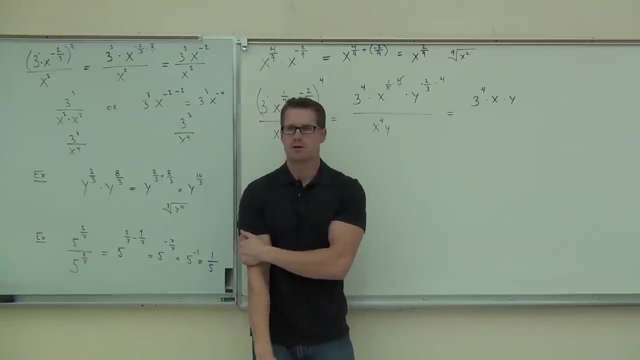 So we're gonna have just x to the one, X to the first power. we have four over four. those simplify to give us a one Times y. how about negative- two thirds times four. Negative. two thirds times four Negative- how much. 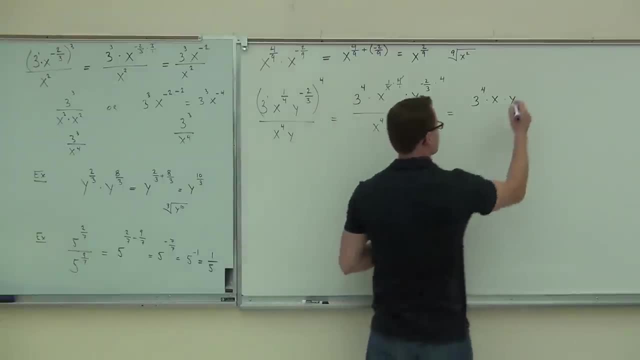 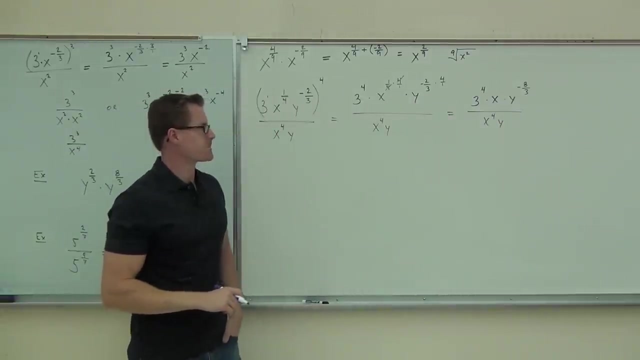 Negative eight thirds. okay, Nothing simplifies there. Negative eight thirds times four. Negative eight thirds times four. Negative eight thirds times four. Remember, this is over one And we still have this denominator X to the fourth y. Okay, all right. 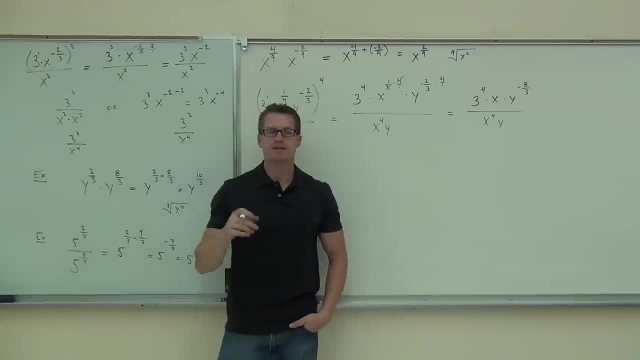 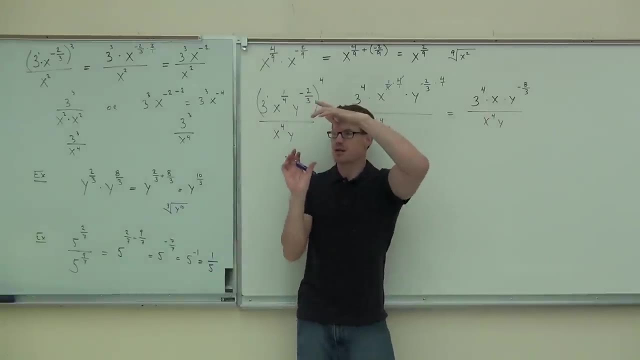 Are we done? No, We still have common bases on the numerator to denominator. You need it so that if you ever have a fraction, everything's being multiplied. If you have the same bases, you need to combine them. You can't leave it like this. 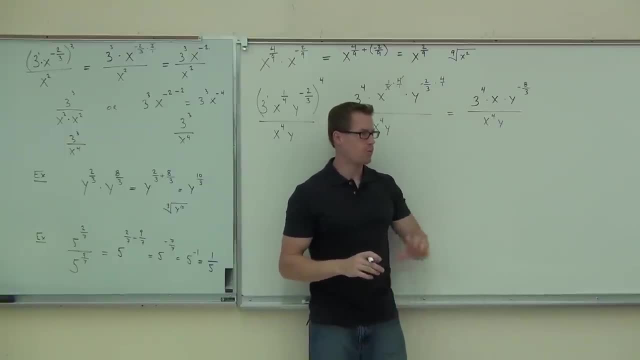 This isn't good enough. This is about halfway done. One more big step to do: We're going to look for anywhere we have common bases, For instance our x's and our y's, and we're going to combine those with our rule number. 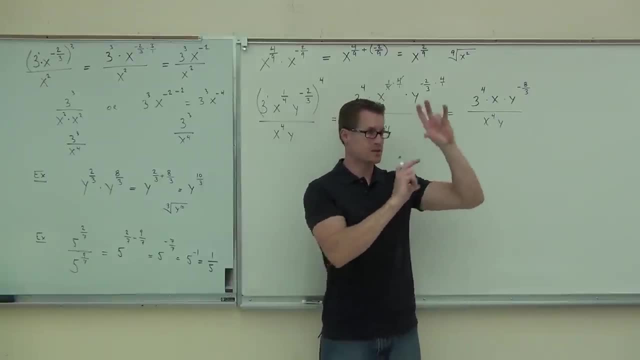 five, taking our exponents and subtracting them. So if I have common bases over each other, I subtract those exponents. Are you with me on that? Now you could move this one to the denominator first and add those together. I gave you that option over there. 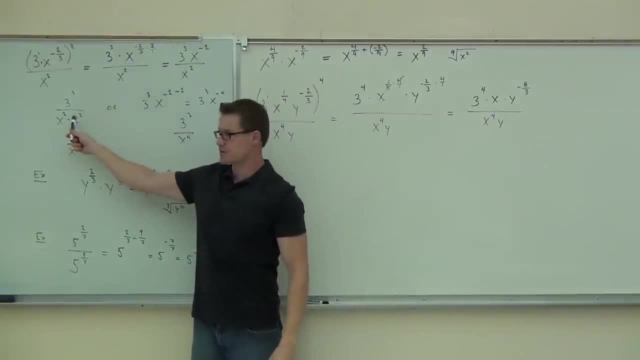 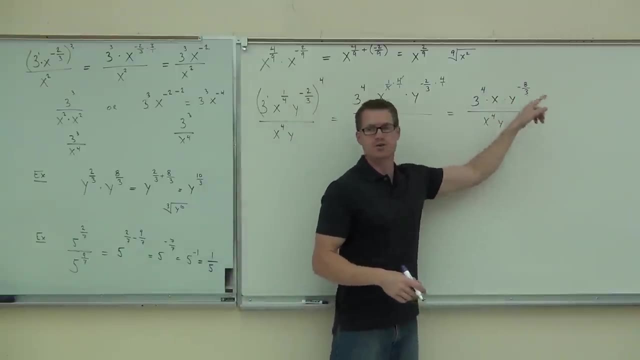 Remember that one. You could do it this way, That's okay. However, for this one, they're both positive. You need to use that subtraction And in fact, I'm going to use the subtraction here as well, just to make everything using. 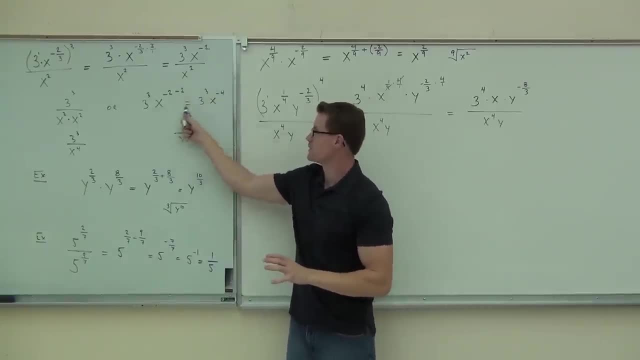 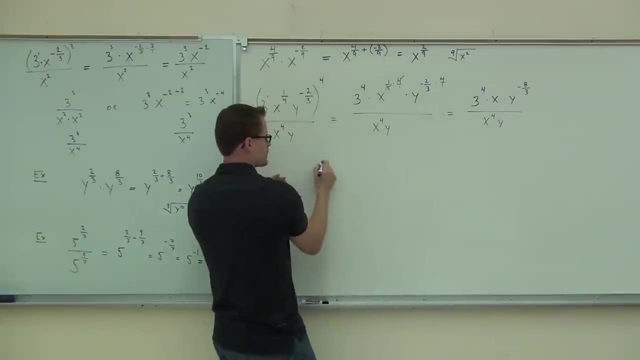 the same rules. I'm going to do it this way. Are you all right with that? Okay, so we're going to keep going on that way. So the first thing I know is that three to the fourth. that's as good as I'm going to. 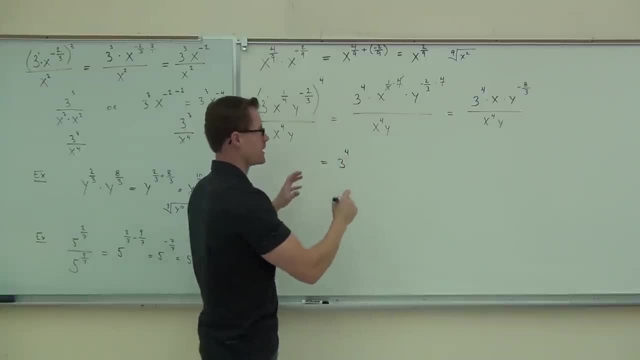 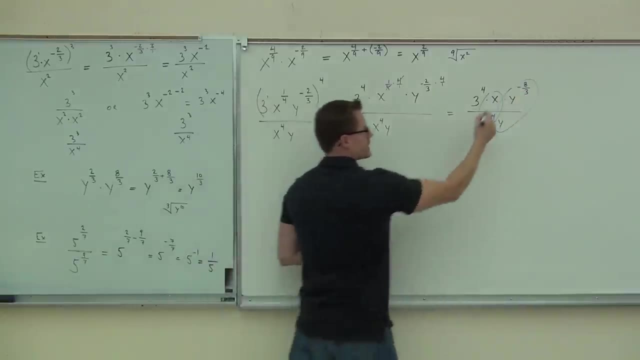 get out of all of them. There's only one, three. We can't combine anything else with that. But I do have those x's and those y's. This is x to the first power over x to the fourth power. So what I'm going to do here, I'm going to take x to the first. 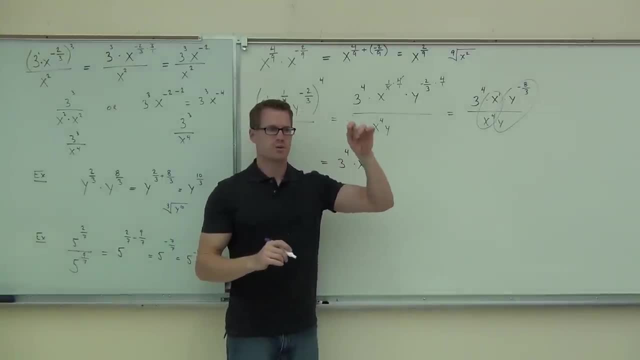 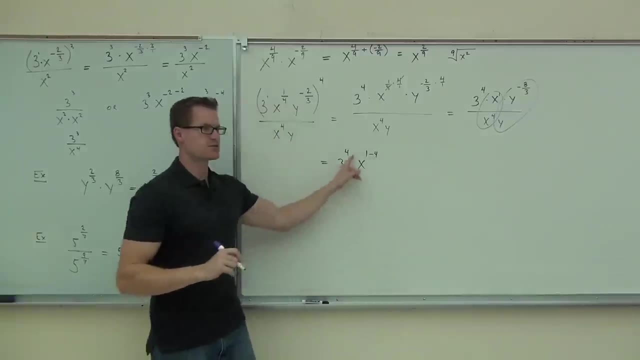 What is it? Are we going to add them or subtract them? Subtract them: Four minus one, or one minus four. One minus four, One The top one minus the bottom one. Whatever this gives me, that's going to be my final answer for my x's. 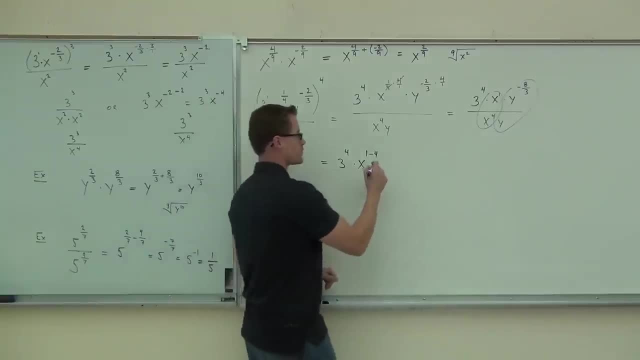 Right there, That's my exponent there. One minus four times y. Okay, we have negative eight thirds over y. to what power is that one? First One, Is it just going to be negative eight thirds? Does that one do anything? 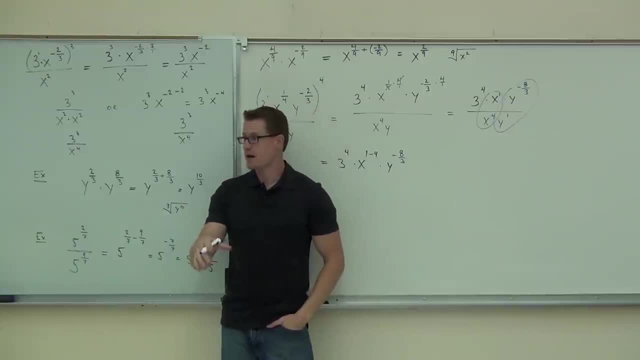 It subtracts, We're subtracting it. Yeah, So it's y to the first power. So when you're doing this, you go. okay, I know that my column bases are: one's a numerator, one's a denominator. 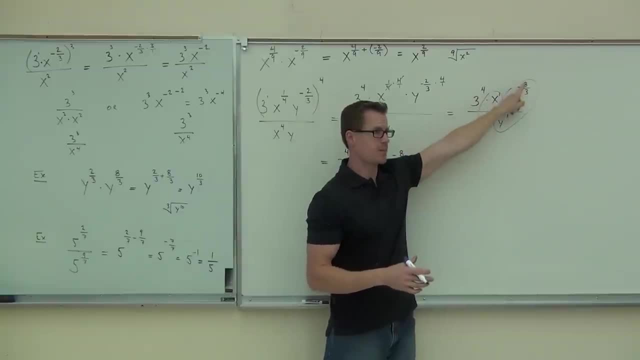 I know to combine those, I subtract exponents: Top exponent minus the bottom exponent, So it's not just negative eight thirds, It's negative eight thirds minus one. Alright, so what's your answer? What's your answer for that? So you're going to raise your hand if you're okay seeing all that stuff? 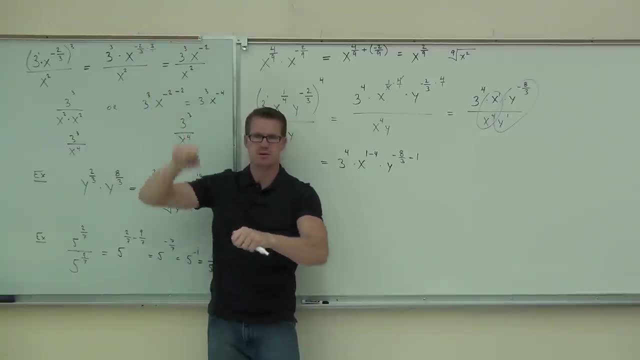 You're guys in the middle, you're not with that, Yeah, okay, Let's keep going. Three to the fourth. I'm going to leave it X to the one minus four. How much should we get out of that One minus two? 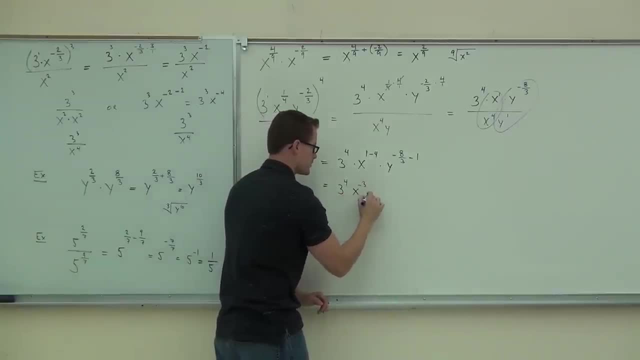 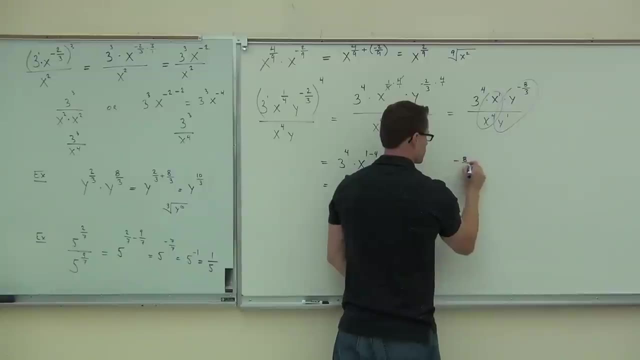 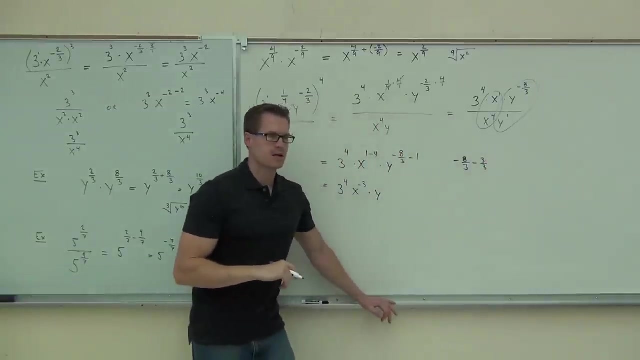 Times y to Oh. negative: eight thirds minus one. Negative eight thirds minus one is the same thing as negative. eight thirds minus three. Three thirds find the common denominator: Negative. eight thirds minus three thirds is the same thing as negative. 11 over three. 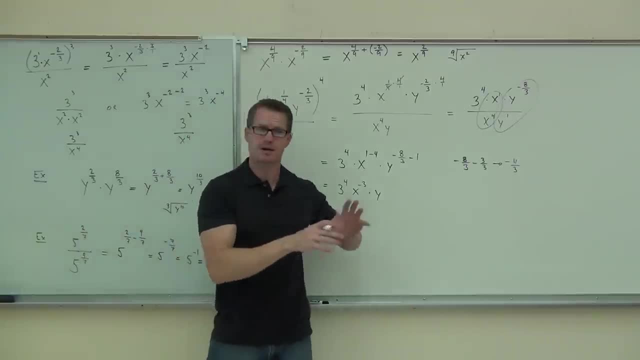 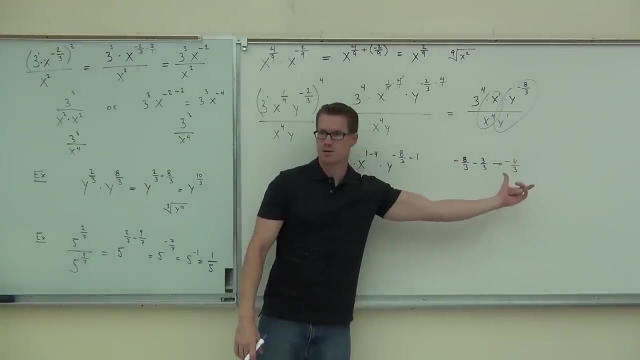 Negative 11 thirds. this is a fraction class right, We're beyond this, so I'm not gonna really spend a whole lot of time doing these basic fractions. You need to be able to do that part on your own. yeah, You need to be able to do that part. 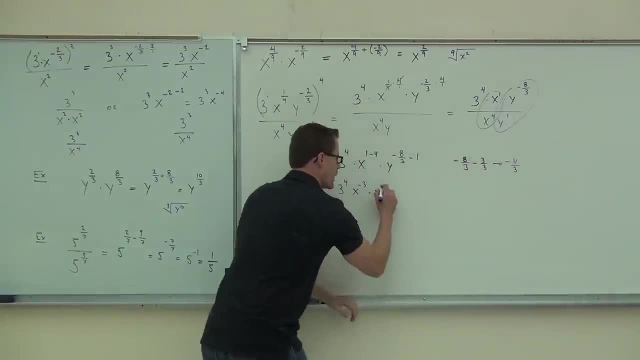 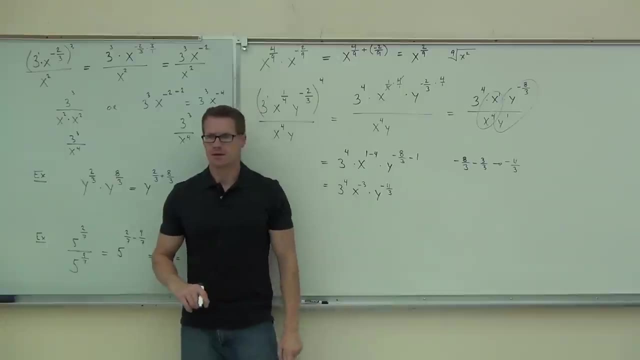 So take our fractions common denominator, subtract them. We get y to the negative 11 thirds. Are we gonna leave it like that? Nope, You said we dropped the negative seven. Yep, rule number seven says I'm not gonna leave any negative exponents. 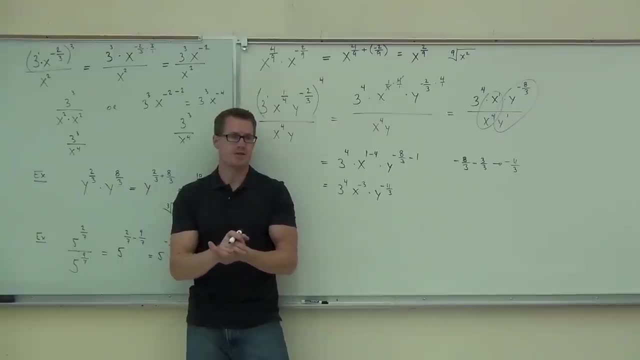 Negative numbers, sure, but negative exponents, no. So how many things do we need to move down to the denominator? One, two or three, Three, The three to the third. we're gonna leave that, I'm sorry. three to the fourth. 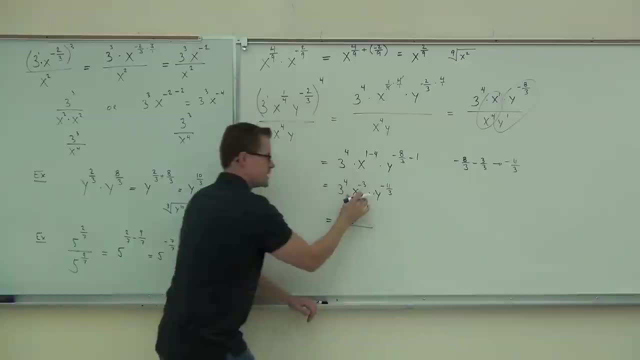 We're gonna leave the three to the fourth, But the negative exponent. we're gonna drop that to the denominator, thereby changing that to a positive. The y to the negative 11 thirds: we're gonna drop that to the denominator and making that a positive exponent. 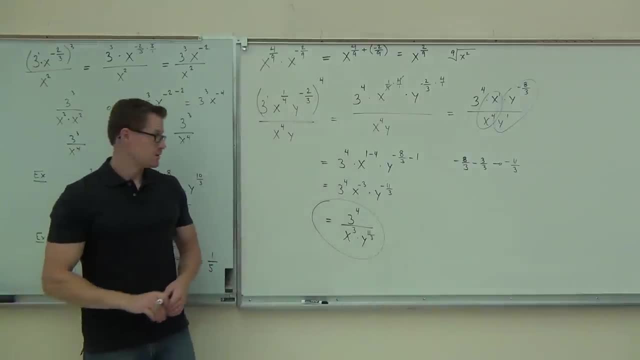 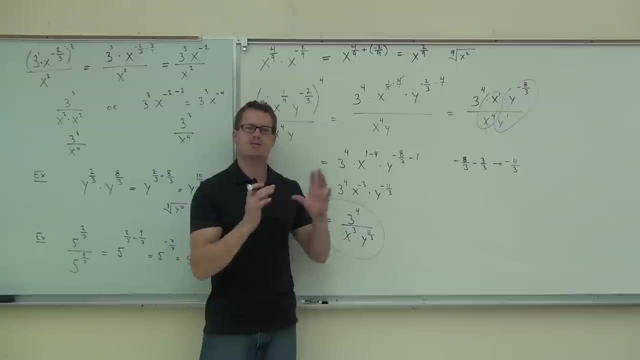 And that, folks, is as good as we can get Three to the fourth over, x to the third, y to the 11 thirds, Positive exponents all in the right places. We've combined everything we possibly can. You're done. 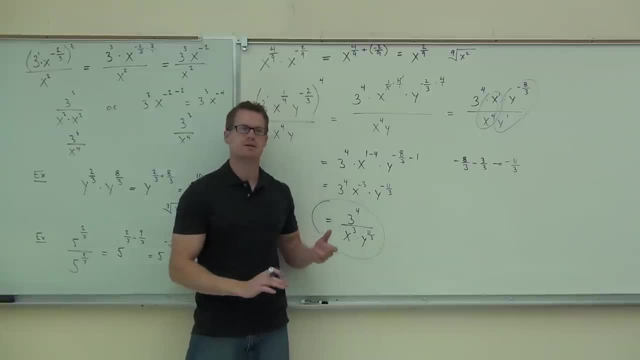 I don't need to see the radicals, I just wanted to make sure before that you knew they existed still. but that's as good as we can get. How many people enjoyed that problem? Don't raise your hands. You're a lion in the eat and you don't even know. 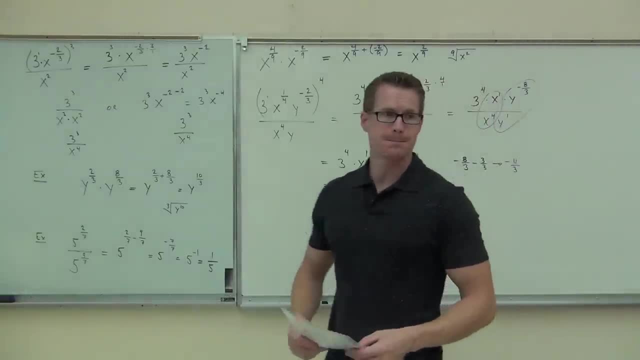 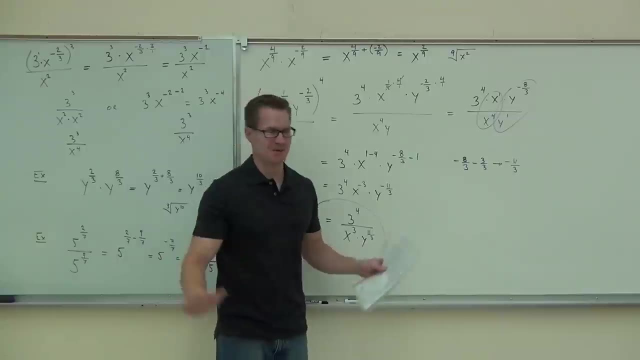 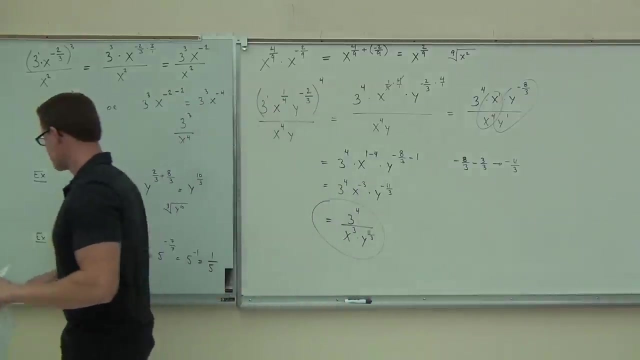 Takes a lot of steps. but did you understand it? How many of these kind of problems are gonna be on the test? Oh, no, more than 16.. 17 of them passed. I don't know one or two. There's a lot more material that we have to cover. 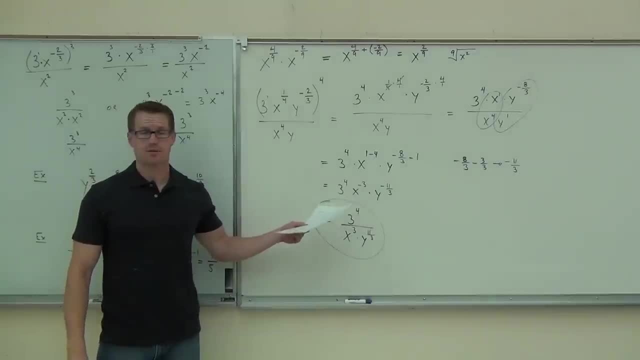 besides just this, Can you follow it though? Yeah, Of course, that took us a while, but when you get the handle on these rules, stick with them. have them in front of you when you're doing your homework. but another thing: when you're doing your homework, 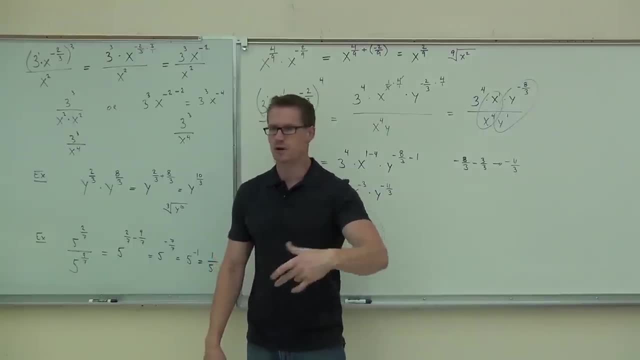 you need to progress past looking at notes doing a problem. looking at notes doing a problem. looking at notes doing a problem. If you're doing that, when you get to the test you don't know well enough. Okay, if you're having to refer to your notes. 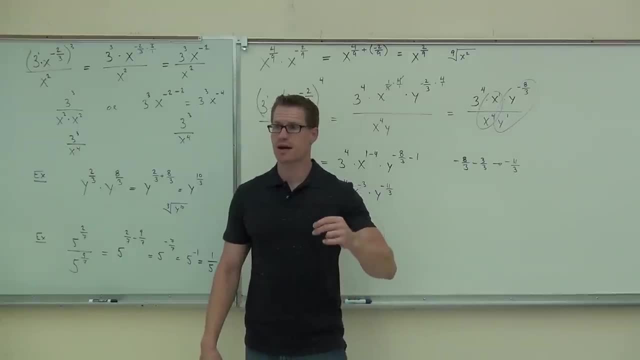 every time you do a math problem, you don't know it well enough. Okay, so you need to go back and make sure that you can do a couple with your notes. That's great. Look at the book for a couple examples. That's fine. 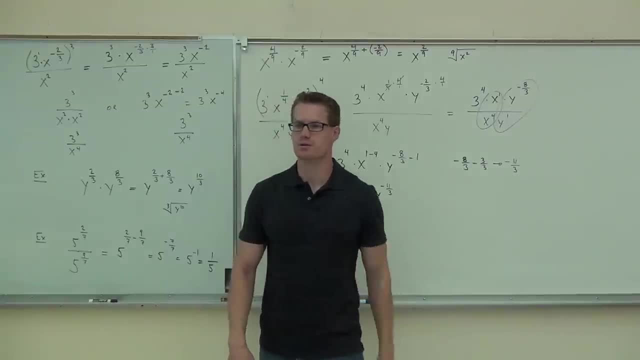 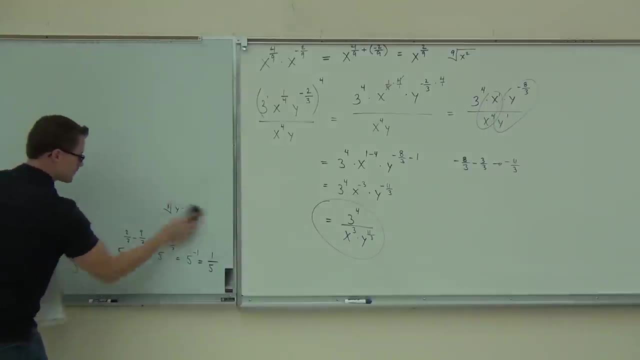 Then put them away and see if you can do the problems by yourself. Okay, That's the way you know that you knew these problems, So make sure you're trying that on your homework. Now let's extend the concept just a little bit further. 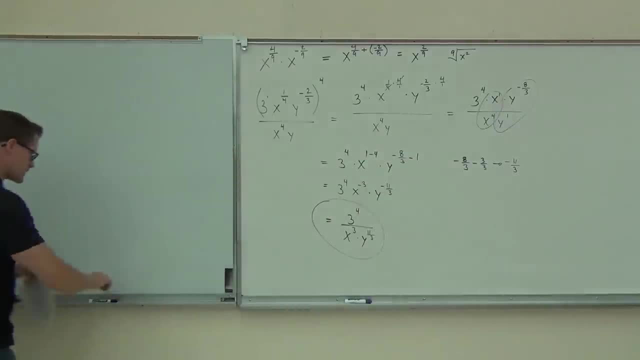 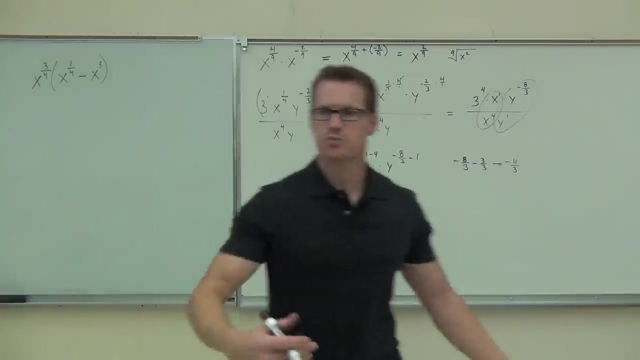 We should be okay on all this stuff. However, there's a couple more things that we need to be able to do with this, namely: What can I do with that thing? Oh my gosh, It's not just multiply anymore. 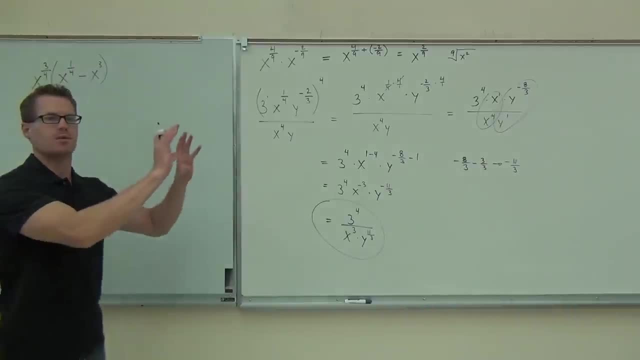 I have some subtraction. Well, I'm going to make this kind of a similar problem over here. Essentially, I've just dropped the denominators. I've made this similar problem. Now I want you to ignore this for a second. Just ignore this one. 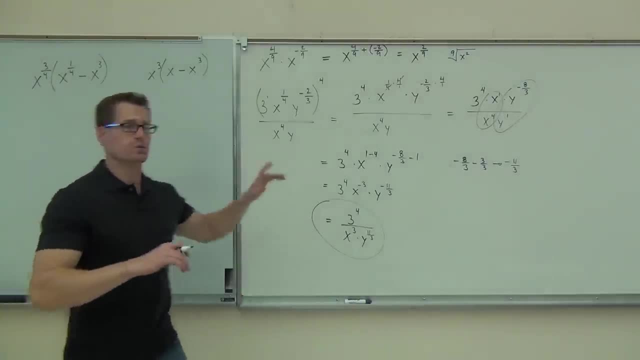 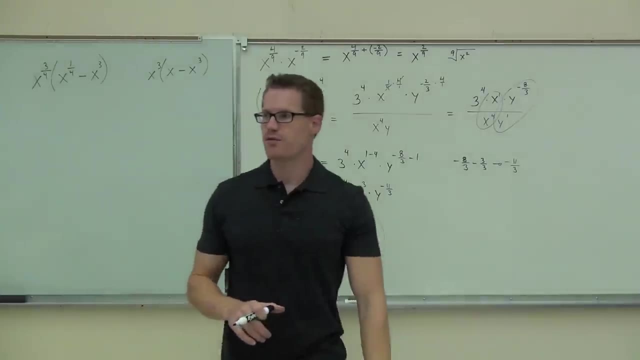 Look at this one. Could you do that? How would you do this? What's that called when you multiply each one? Factor of units, Not factor. Factor is the opposite of what we're about to do: Distribution. We're going to distribute. 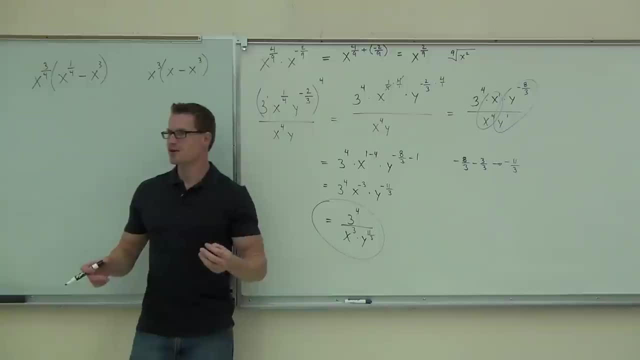 Remember how to distribute. I hope you do Well, you should. If you're in this class you know it. I mean, you've done this a long time. Distribute says you take this outside one and you multiply it times each inside one right. 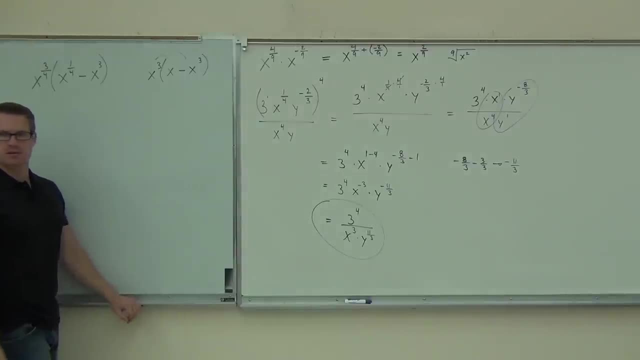 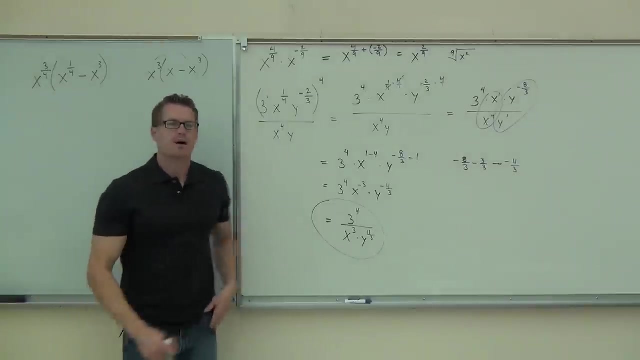 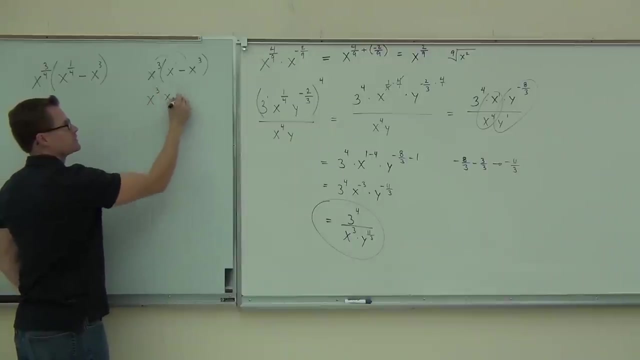 So can you tell me what is x to the third times x, X to the third, X to the Fourth? How do you get an x to the fourth That way? OK, this is x to the first power. So how I do this? I do, oh, x cubed times x minus x cubed. 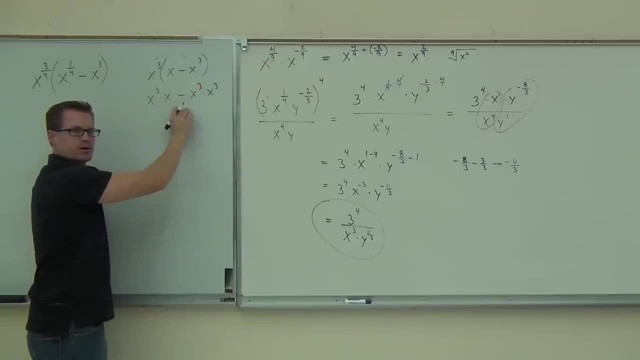 times x cubed. Are you seeing where all these things are coming from? Let your head if you do. This is distribution. You need to know distribution, at least to be here. You need to know that Now, if we have x to the third and x to the first. 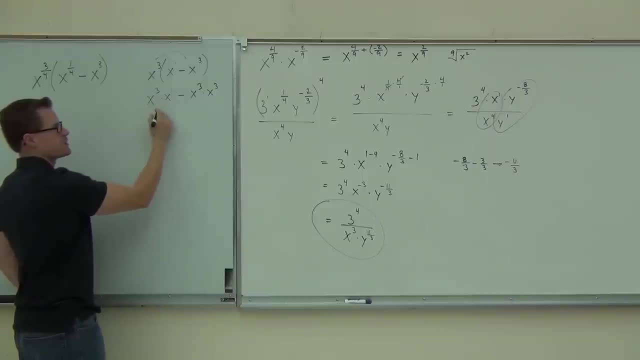 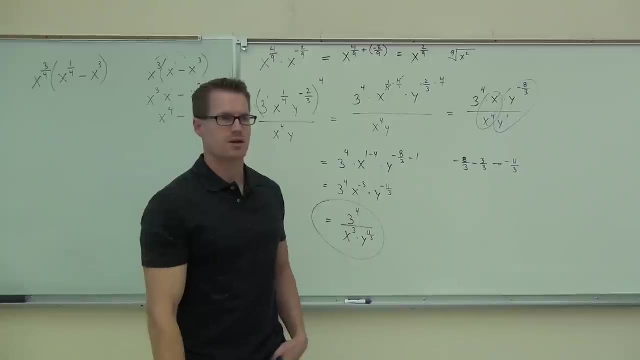 we know that we add those common bases, The exponents of those common bases. we get x to the fourth minus what is that? x to the sixth or x to the ninth, Ninth? x to the sixth or x to the ninth? 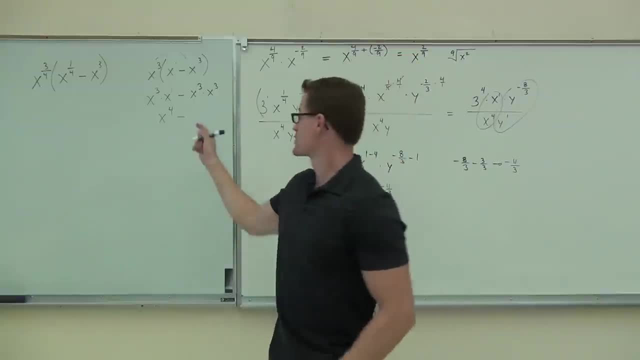 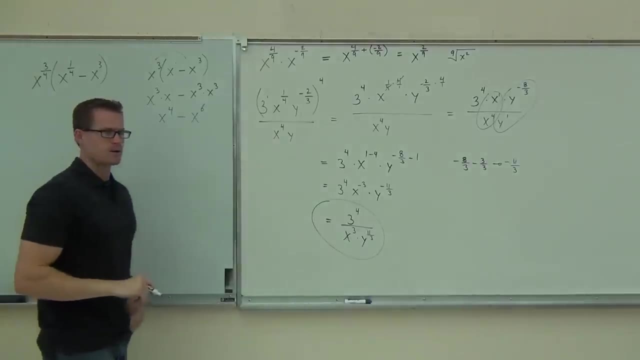 We're multiplying common bases. Don't let your mind trick you and go: oh, this is nine Common bases. what do you do with those exponents folks Add up? You're going to get x to the sixth. You OK with that? 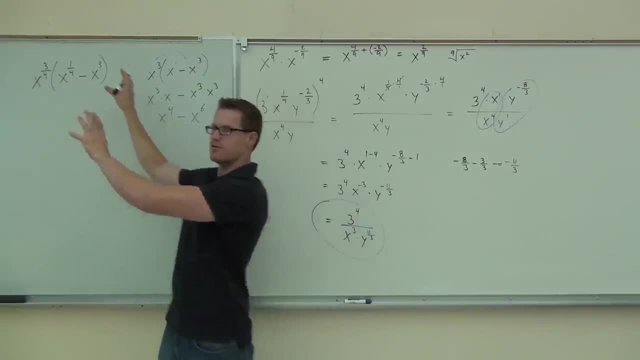 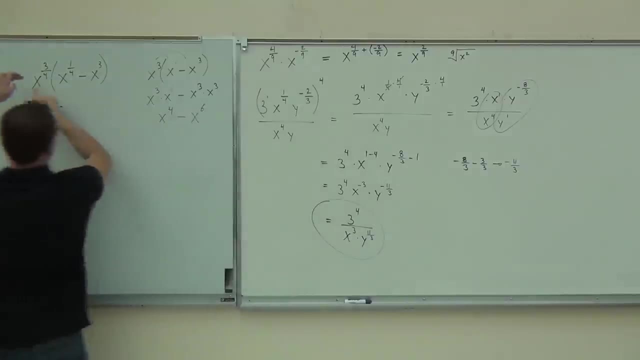 We can use this idea of distribution even when we have rational exponents. It's fine. It's the same exact thing when we took x to the third times x to the third times each of these two. We're going to take x to the 3 fourths times each of these two. 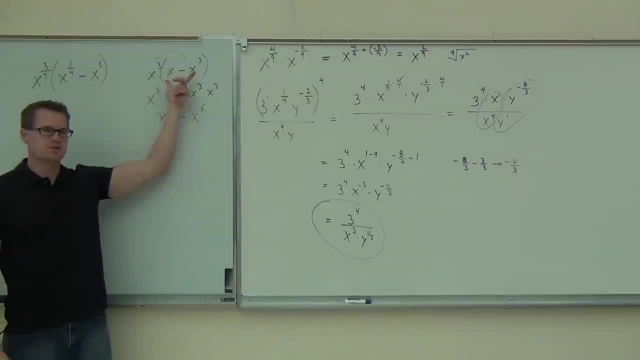 However, instead of just doing this in your head, you could probably- most of you could probably- just go from here to here, right, I hope so. I mean you just x to the fourth, x to the sixth, No problem. 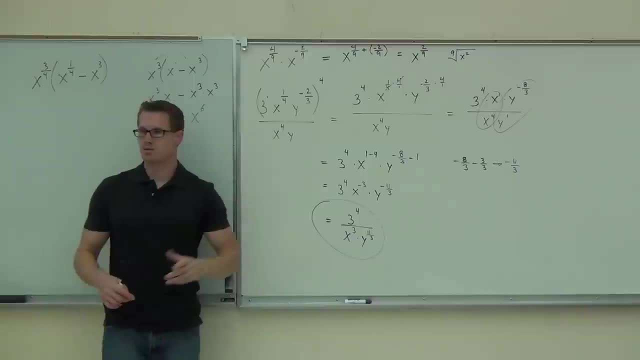 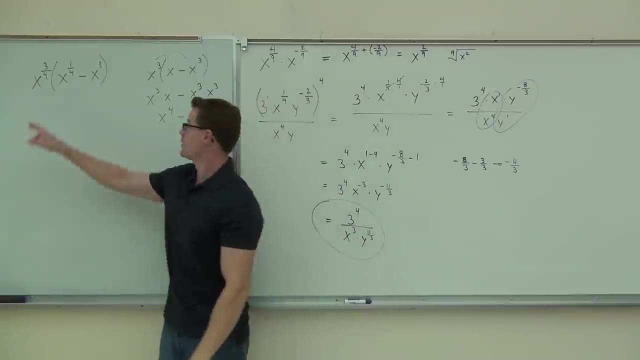 I'm going to have you write these ones out like this so that you can see the rules. You see, the problem with distribution, with rationals, is people. a lot of the time they love to do this, They love to go oh x to the 3 sixteenths. 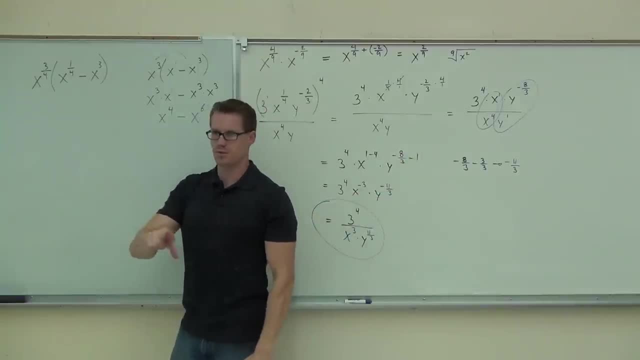 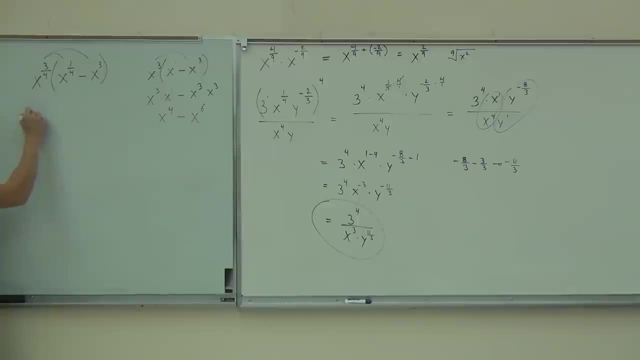 I'm done Because you think multiplication, we're not multiplying, We're adding those x's because we're multiplying common bases. So what I'd like to see from you, sure, we're doing x to the 3 fourths times x to the 1 fourth. 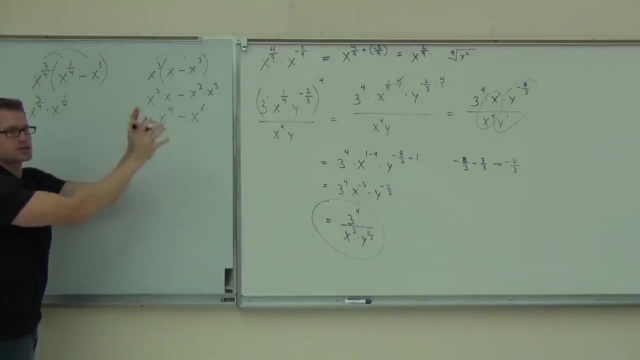 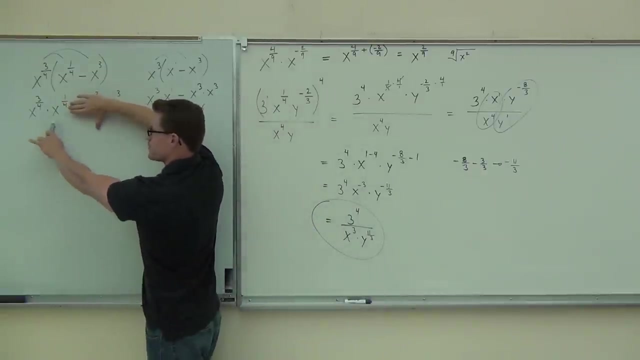 We're taking the first outside factor times each inside term. Are you seeing where this is coming from? Then we're going to have a minus and we're going to do x to the 3 fourths times x to the third. Can you tell me if you ignore this? does that make sense? 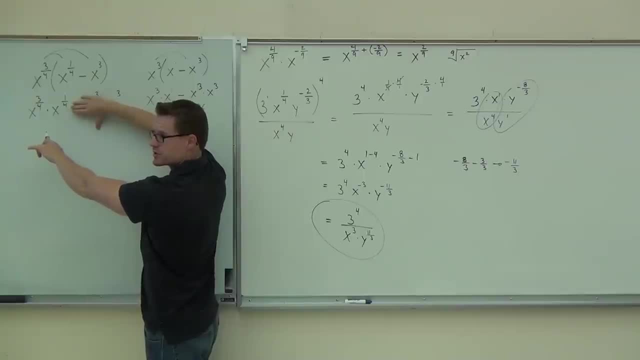 Are you familiar? We started the section off this right Today. off of that, You can do that. What are you going to do to combine those exponents x to the 4 to the 4 to the 6th? Yes, exactly. 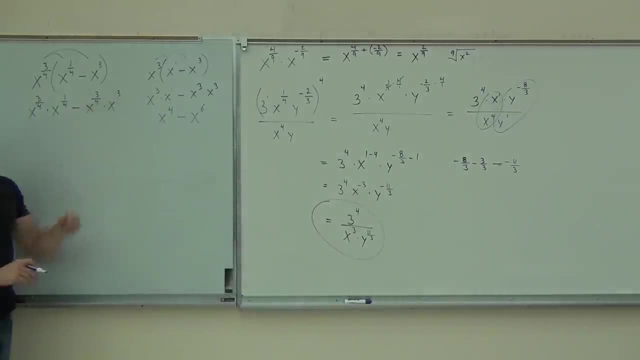 You're going to add those together. You're going to add these together. I think you're going to add these to the 4, to the 4, to the 6th. Yes, Don't rush through this stuff, otherwise you might make a mistake. 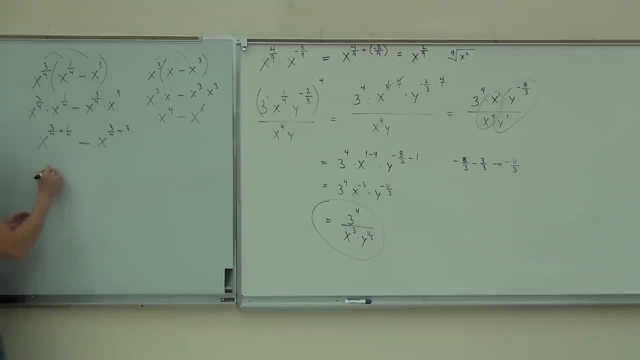 Go slowly. think about the rules, do them deliberately. You have x to the 4 fourths, or x to the first minus x to the 3 fourths plus 3, that's 3 fourths plus 12 fourths. that's going to be 15 fourths. 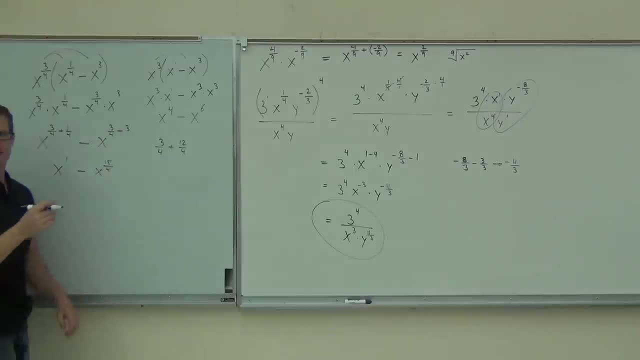 Add those together, you'll get 15 fourths out of that. Check my math and make sure I did that right, by the way. So x to the first, x to the 15 fourths. By the way, can you combine x to the first and x to the? this is where we'll stop today. 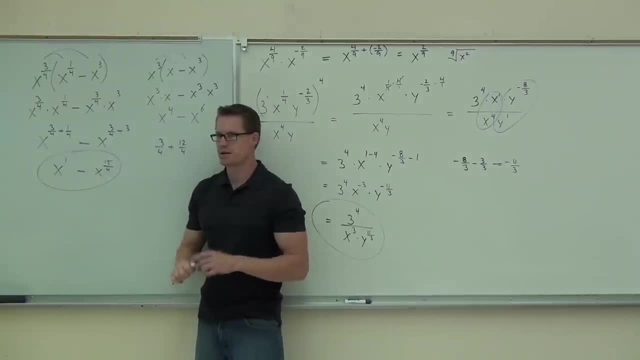 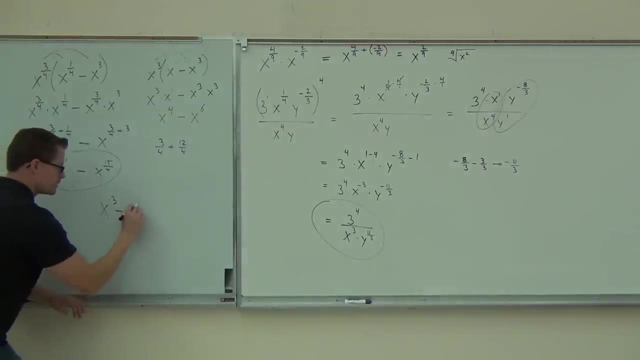 can you combine x to the first minus x to the 15 fourths? Can I subtract those? Let me ask you a different question, a similar question: Does that equal x? Does that equal x? Does that equal x? Let me ask you the first. 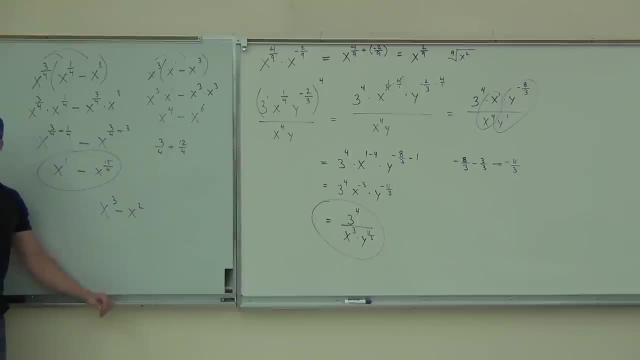 I need to know that. What do you think? Wow, I have some stumped looks out there. It's a good thing. I asked about this. Can you combine this? No, Why not? Can you combine this? Can you combine this? 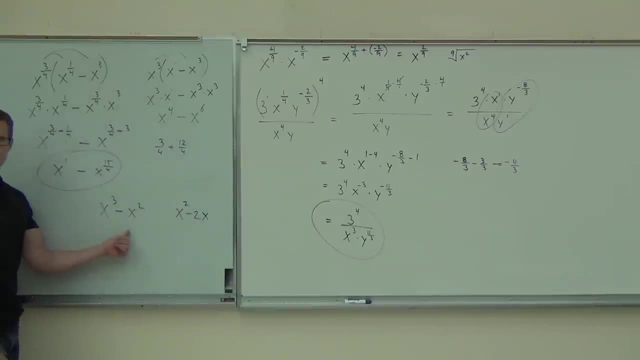 No. Can you combine that? No, Can you combine that? No, No, Like terms have the same variable, the same exponent. If you do not have like terms, you cannot combine them. Do you have like terms here? Are they the same variable? yes to the same exponent. 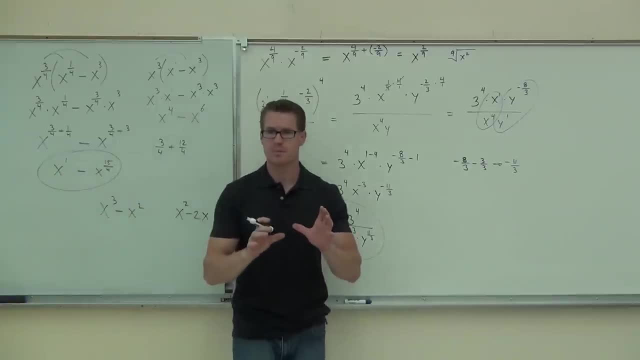 No, No, You cannot combine that unless you have exactly the same variable, the same exponent. You can't add or subtract, Multiply, divide, sure, because you know you can multiply x cubed times, x squared right, That's fine. 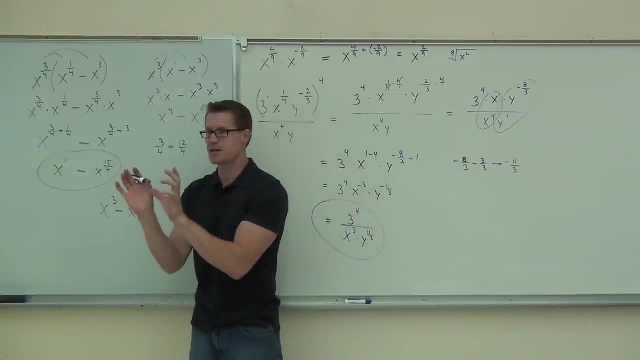 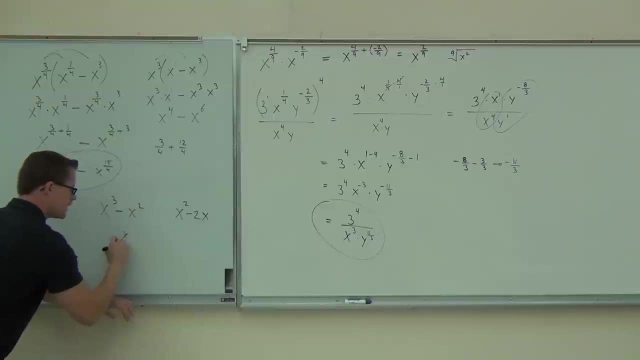 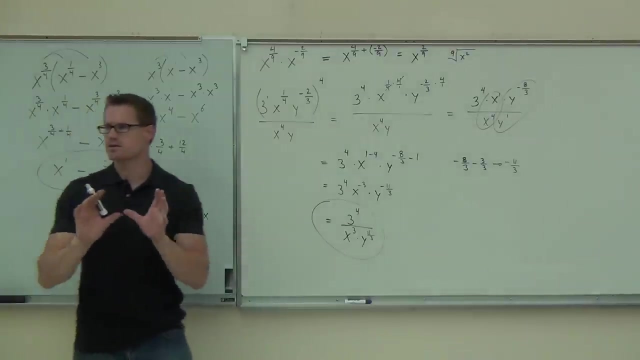 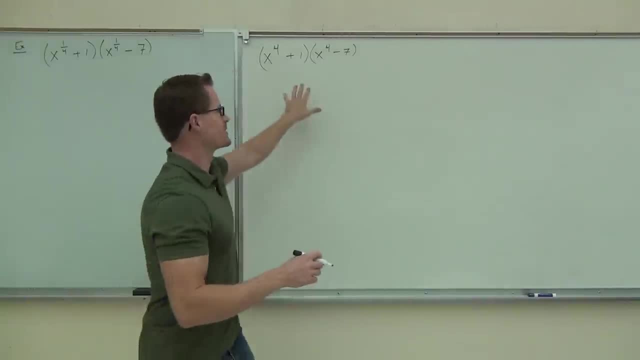 Now, in this process, when you distribute stuff like this, you'd probably do it in your head, right? You just go x to the fourth times, x to the fourth, and you're gonna give me x to the 16th, right. 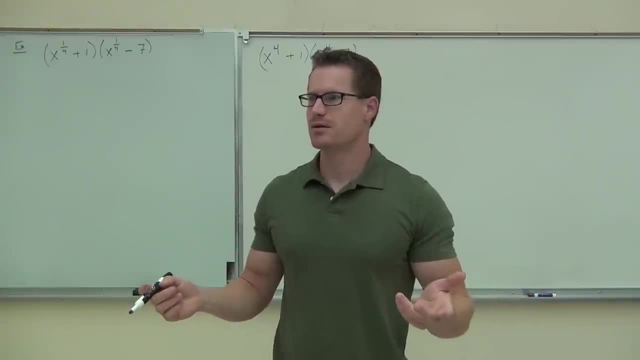 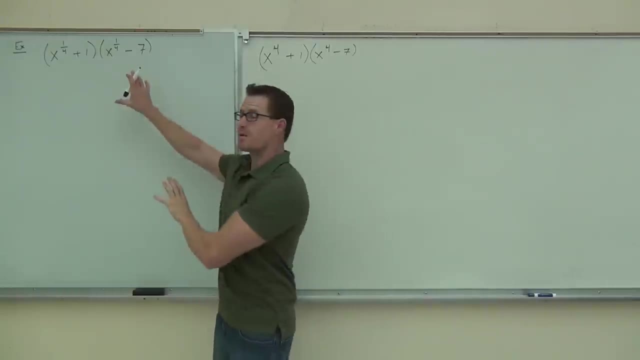 Really Well, why not x to the 16th? Okay, now, we catch that in our heads usually when we do our distribution, but really in this problem a lot of people don't catch that and a lot of people would give me. 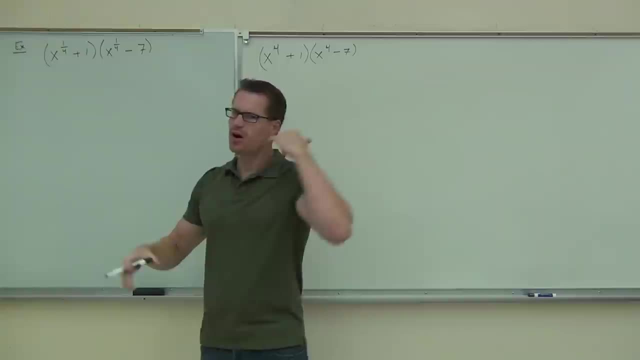 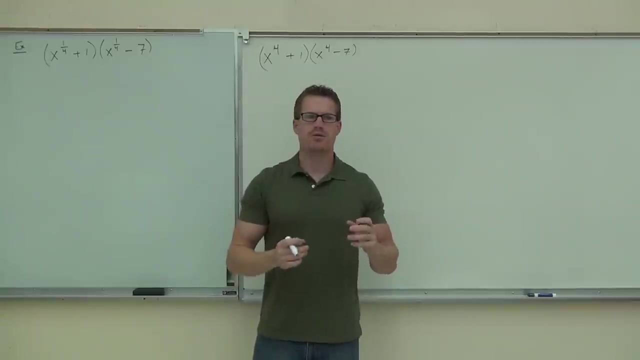 1- 16th out of that thing, because they're multiplying and they're thinking, oh, we multiply. What I'd like you to do is, instead of doing these problems completely in your head, take the extra five seconds and write out one extra step. 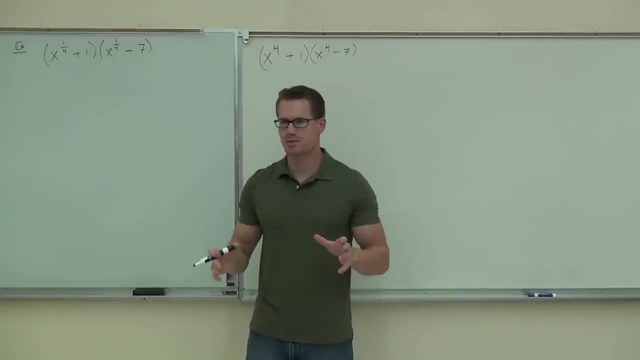 This is gonna let you see the excellent rules that we've been practicing. last time, Trust me on this one: If you try to do a lot of this stuff in your head, sometimes you're gonna make some mistakes. If you write it out a lot of times, 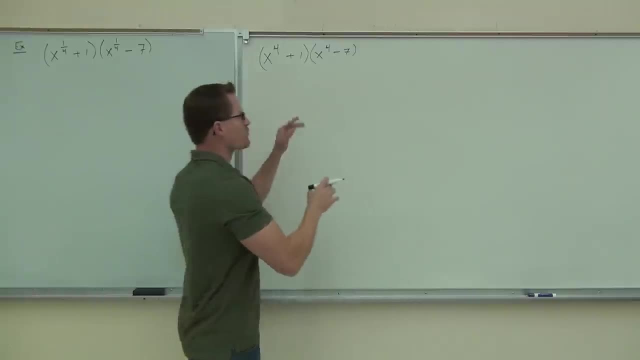 you catch those mistakes, not, you're gonna be with me. So, instead of doing this directly from our head, we're gonna go. okay, I know I'm doing x to the fourth times, x to the fourth. that's here I know I'm gonna be doing. we have a positive times. 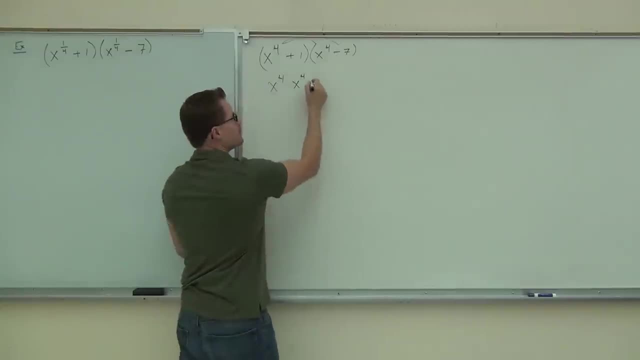 we're gonna consider that negative, because you could write this as plus a negative, minus seven times x to the fourth, plus one x to the fourth, and lastly we'll have our minus seven. You still okay on that one? Then we do the math. 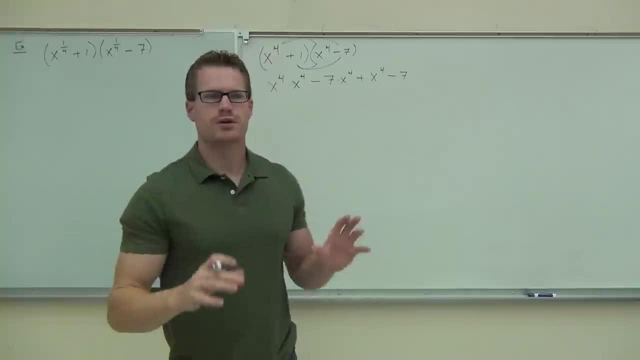 Then we look at the exponent rules. we go: okay, if we have x to the fourth times x to the fourth, we know that when we're multiplying common bases we're not multiplying exponents. That would be an exponent raised to an exponent. 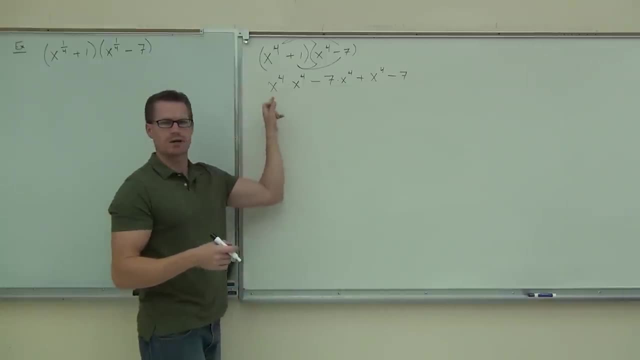 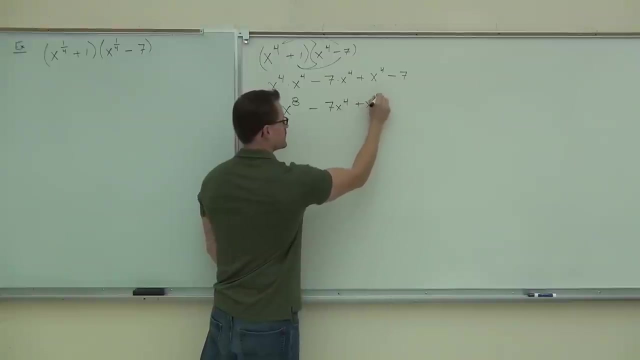 We're actually adding those things. So instead of x to the 16th, we're getting what? here, folks, You gotta play along, You gotta play along, You gotta be here with it Minus Second x. Now, last time, the last thing that I taught you. 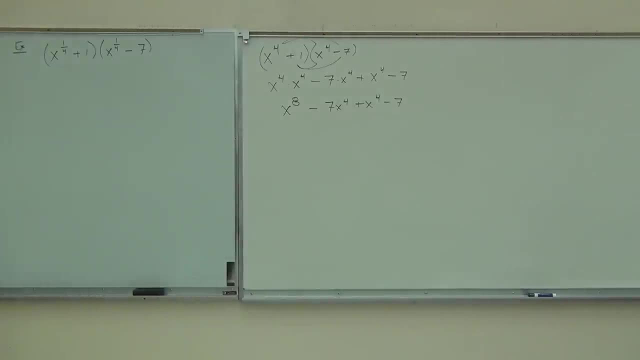 is that we really can't combine any like terms unless we have. I'm sorry, we can't combine terms unless you have exactly the same variable raised to exactly the same x color. So in our case, I asked: could we add together something like x to the eighth and x to the fourth? 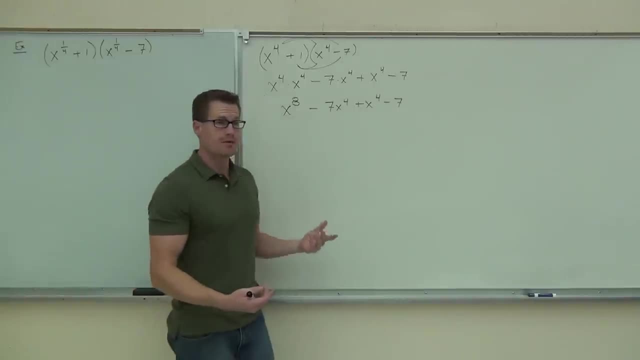 Are those combinable? No exponents are different. However, we do have a couple things that we can combine. What could we combine here? It is seven times one: x to the fourth, x to the eighth. Good, What is it? x to the eighth. 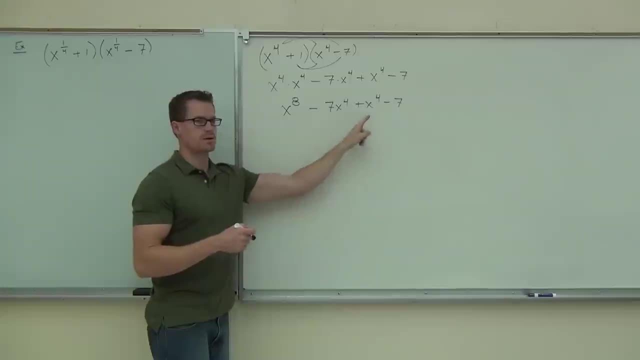 No, This one. No, I'm sorry, never mind. yeah, What are these ones? X to the fourth, seven x to the fourth and x to the fourth. Now listen, you gotta do this properly If you're gonna combine these two things here. 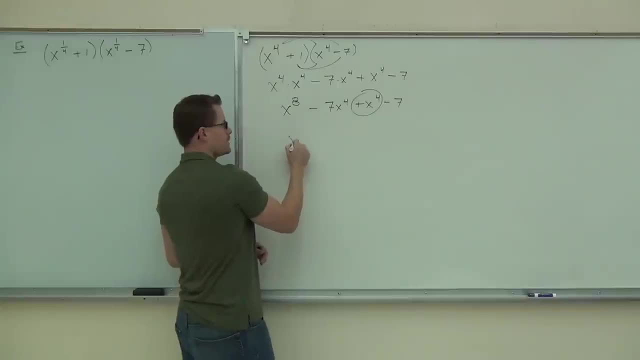 which they are like terms in the same variable, raised to the same power. you're gonna combine these two things here, which they are like terms in the same variable, raised to the same power. you've got x to the eighth minus. do me a favor, combine these like terms correctly. 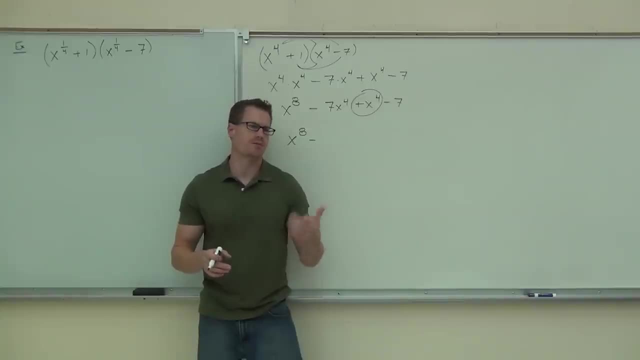 If I combine these like terms, I'm just looking at the coefficients. basically, I have minus seven, I have plus one, I'm gonna get negative six out of that. Am I gonna get x to the fourth or x to the eighth? X to the fourth? 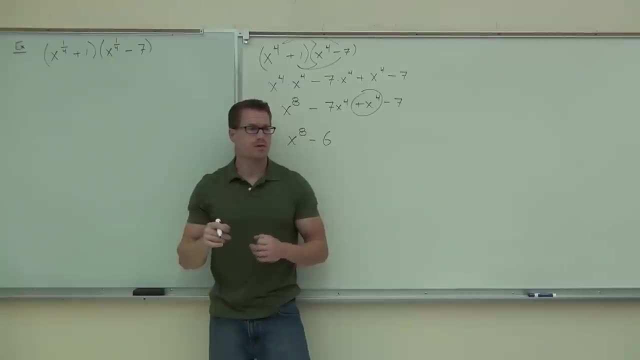 You sure? Yeah, because you're adding that multiple times. Okay, so if I combine like terms, I want you to realize something here: Some of you guys really aren't getting this yet and you're gonna see a crossover in a second though. 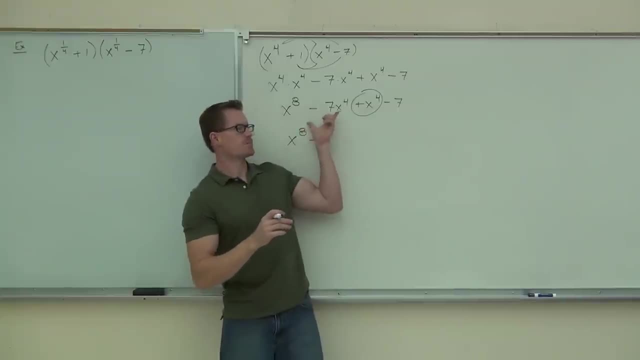 and then you're gonna get it If you don't have like terms here, which means you couldn't combine them right. By combining these terms, it doesn't magically make this like term, because then you would have been able to combine these right. 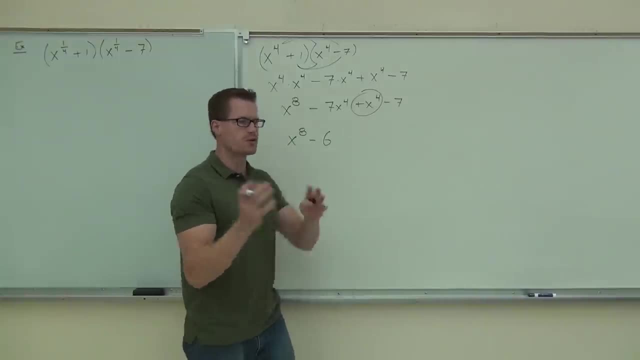 So when you're combining like terms, don't change the power. The power only changes if you're multiplying things. That's when the power changes. With your combined like terms, the power doesn't change. So we are gonna get still x to the fourth minus seven. 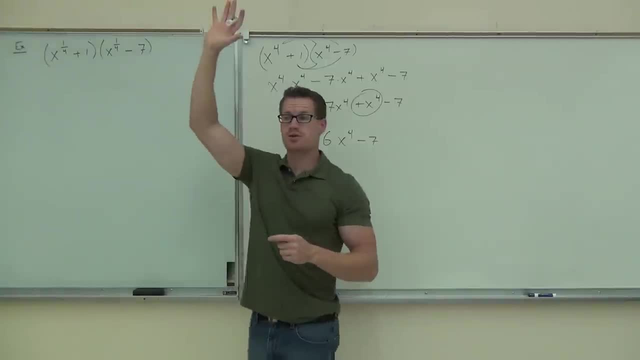 There's no like terms. you're done on that problem or you just can't feel all right with that. Now let's draw some comparison and do that problem First thing we do. if we were to FOIL this, we're gonna do the same thing here. 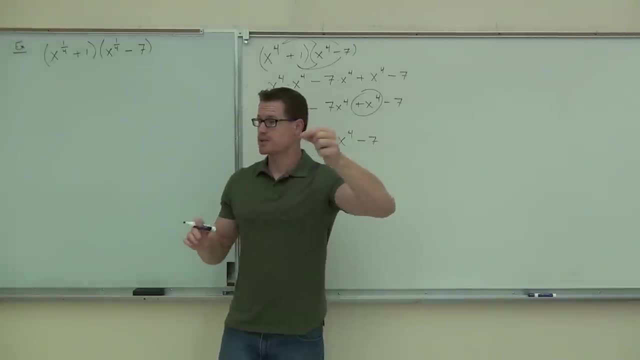 Just don't do the stuff in your head. Go ahead and actually write out this step. that's gonna help you with these fractional exponents. The first thing we're gonna multiply is x to the 1- 4th times x to the 1- 4th. 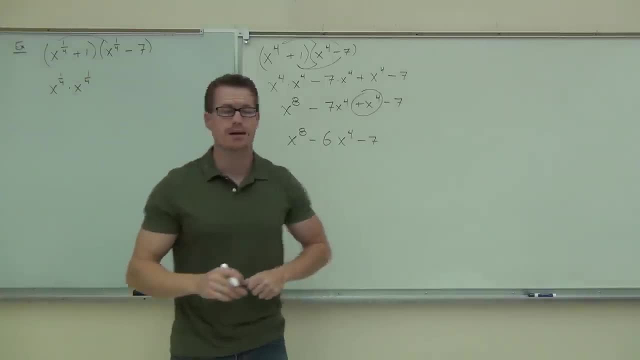 We're gonna write it out. We're gonna write it out. We're not gonna do that step in our head yet. The next thing we're gonna do. you're gonna notice I use the same exact numbers for a reason. That way we can just look exactly. 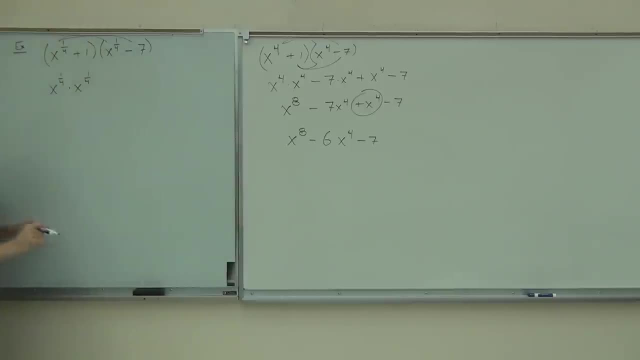 the same process of these things: X to the 1 4th times minus seven. You're gonna get minus seven x to the 1 4th, Just like you're distributing, like normal. Then we get our plus x to the 1 4th. 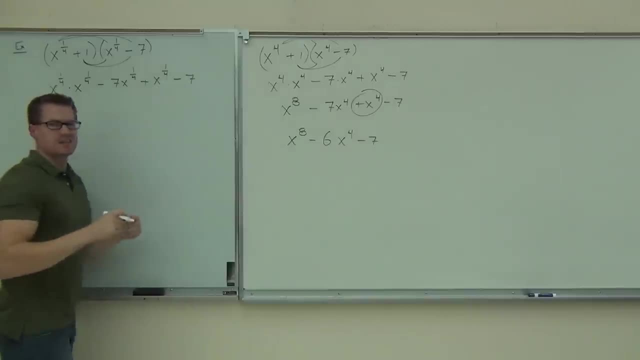 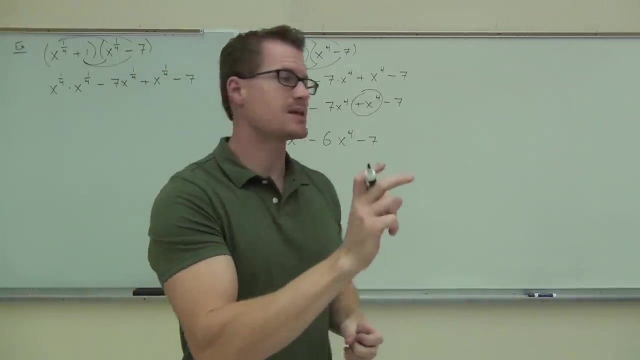 And, lastly, we're gonna get our minus seven at the very end. Do you guys see the similarity between this problem and this problem? Okay, Now, since we've written this out, we can do this process step by step And, as a matter of fact, 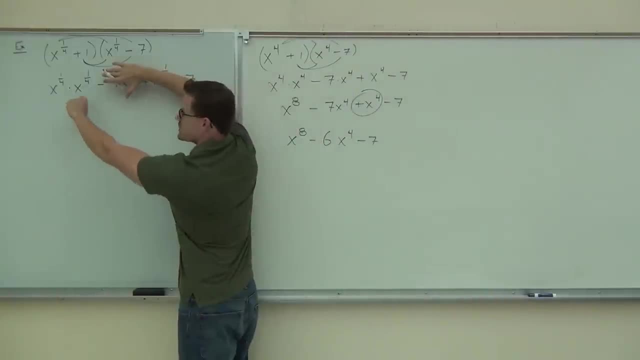 you've seen some of these problems before. I mean, if I just ignore this stuff, you've seen something like that. right, That was in our exponent rules from last time. How much is x to the 1 4th times x to the 1- 4th? 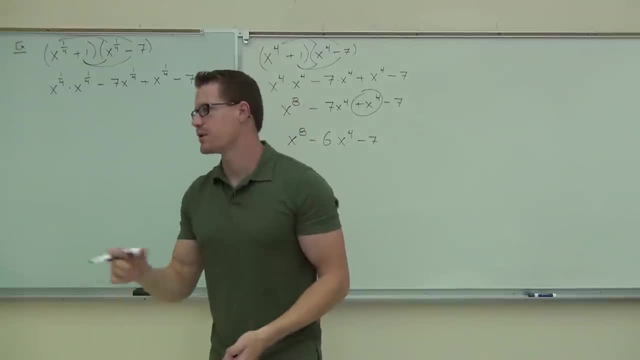 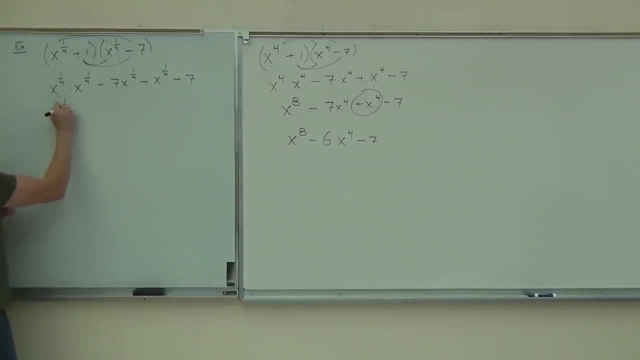 Or don't tell me how much it is, but tell me what we do. Do we add, subtract, multiply or divide those exponents, Add. So really what we're doing, if you're thinking about this, we're doing x to the 1 4th plus 1 4th. 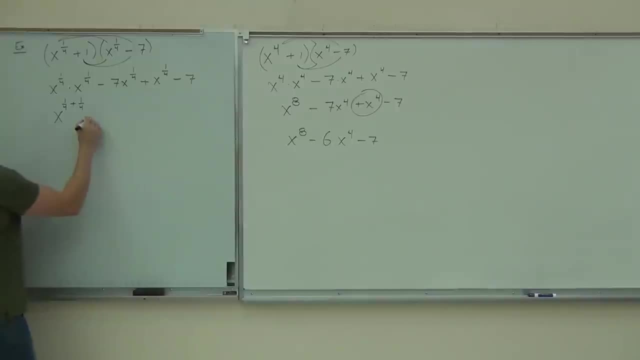 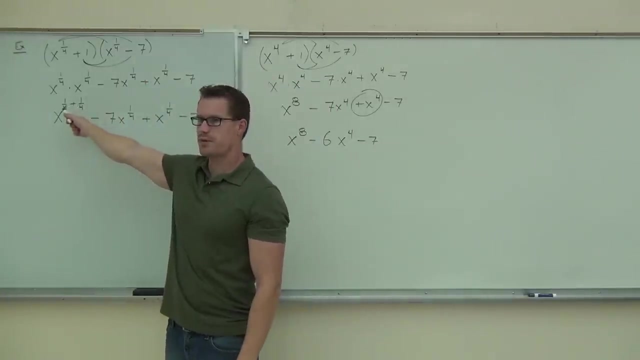 Do you remember that process, that we write that out? You have that Minus. we're not gonna do anything here Or here. we'll save it until the next step. Tell me how much are we gonna have if we do x to the 1 4th plus 1 4th? 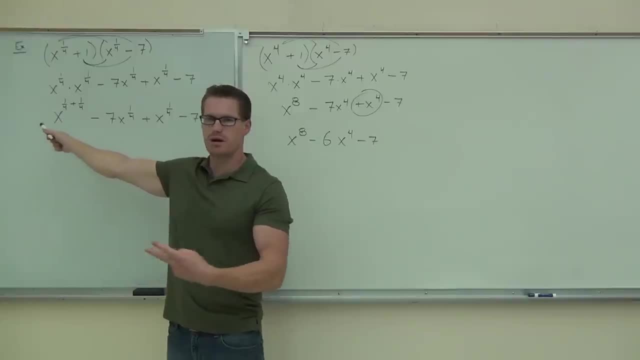 How much is that? One half x to the 1 4th? Good, because you're gonna get 2 4ths right. You get the common denominator already: 2 4ths simplifies to 1 half. 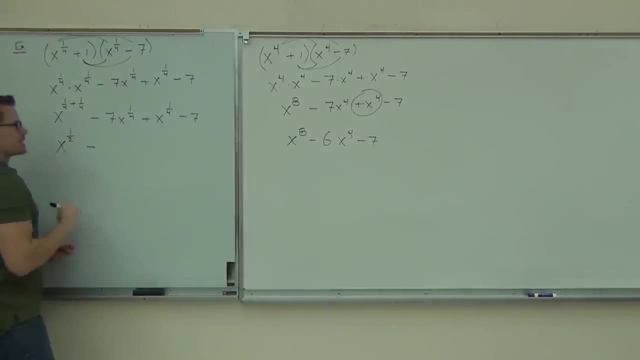 We've got x to the 1 half minus how much is seven? x to the 1 4th plus x to the 1 4th. Now I know I can combine them because I have those like terms. They have the same exact variable. 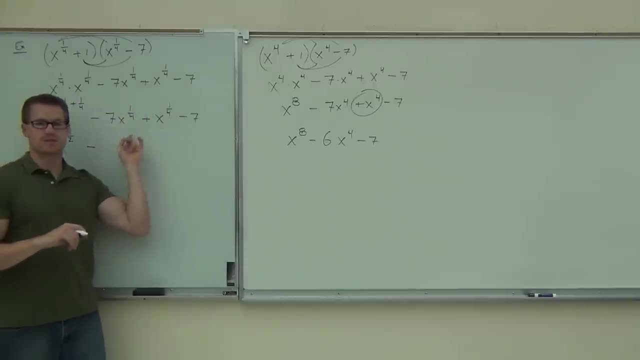 raised to the same exact power. How much am I gonna get here? Negative six and then x to the what? 1 half, 1 half. okay, When you're adding them, Let's see if that works. Does that work? 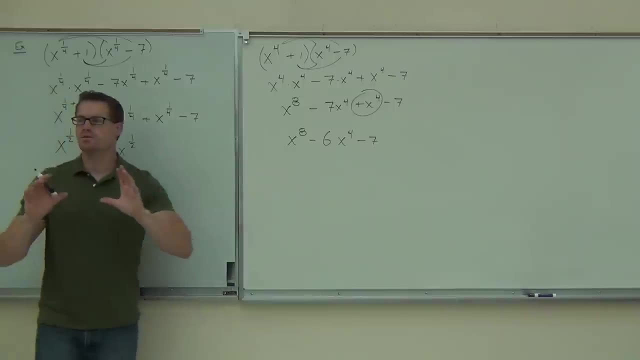 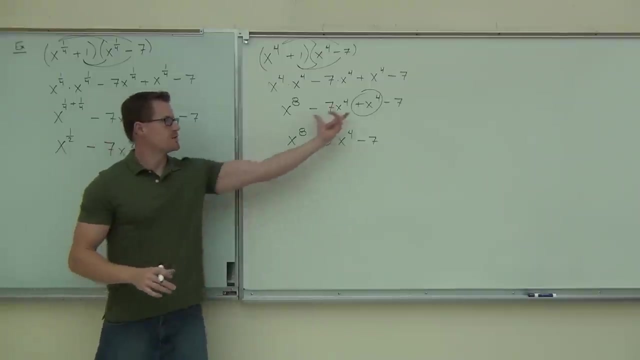 No, You need to really really look at the similarities here, and I just: I caught a few people already. Okay, caught a few people already. Did you add those exponents? No, But for some reason, when people are dealing with rational exponents, 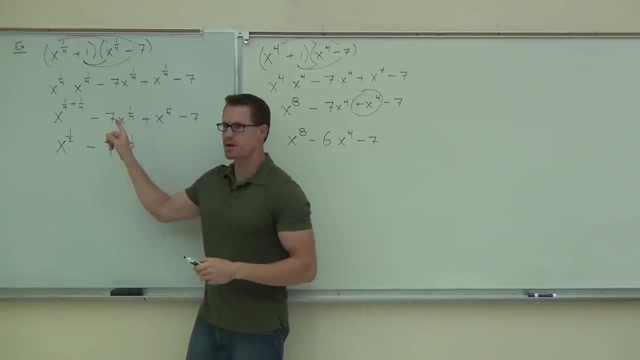 they really, really want to add these. Something in your head goes: oh, that makes 1 half. Okay, it happens all the time, But you need to understand the process, that this is exactly the same as this, If you combine like terms here. 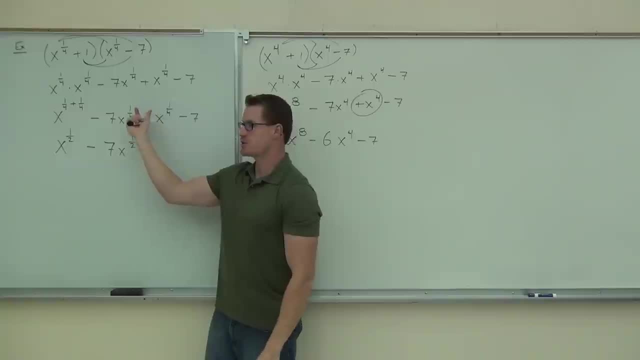 and you get x to the 4th. you are gonna combine like terms here and get x to the 1- 4th. See the similarity. That's why I show this example when I do this problem, because I really wanna make sure that you see. 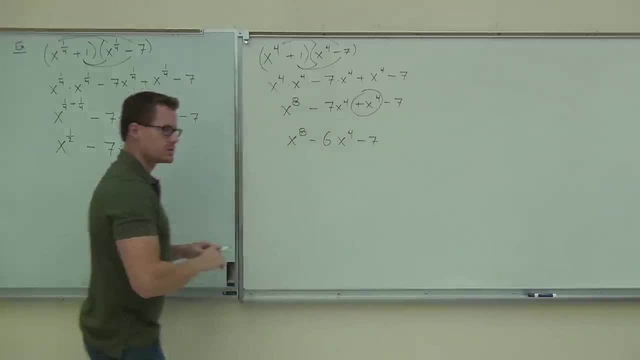 they're the same. They're the same, But people often will do this. If you looked at this, would you be able to combine x to the 1 half and x to the 1- 4th? No, they're not even close like terms. 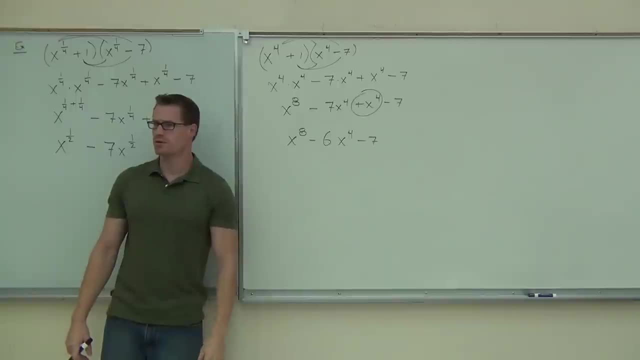 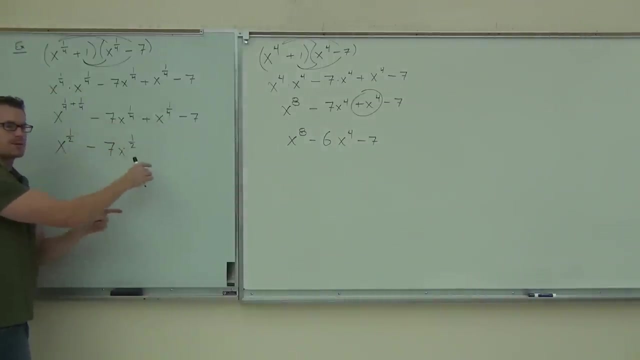 It's like saying: can you combine x to the 8th and x to the 4th? No, not even close. You have to have the same variable, the same exponent. Yet when people do this thing, they will often give me x to the 1 half. 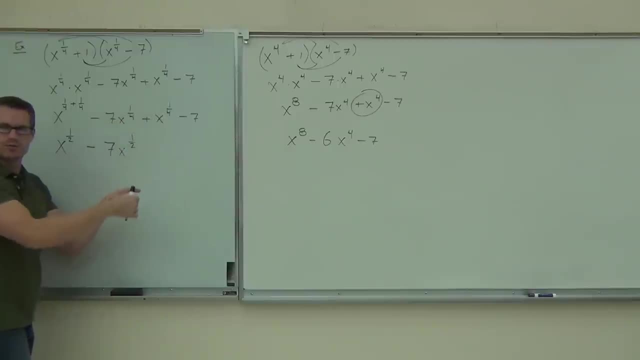 Because something in your head says you're adding: I have x to the 1 4th, x to the 1 4th, that makes 1 half. But we're not doing that, We're combining like terms. In that case you don't actually add those exponents. 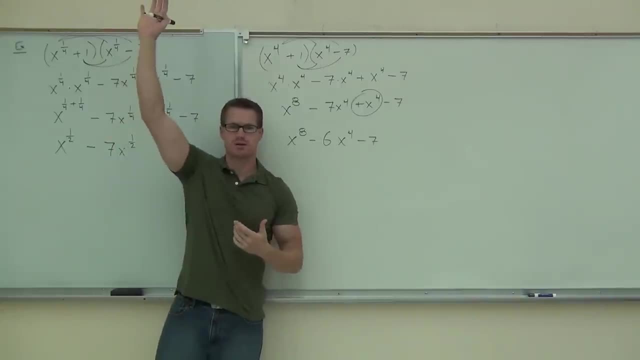 You just keep them the same. You're adding or subtracting coefficients. Raise your hand if you see the difference there. Good, okay. So in our case we're gonna go: oh no, no, no, no, Not x to the 1 half, uh-uh. 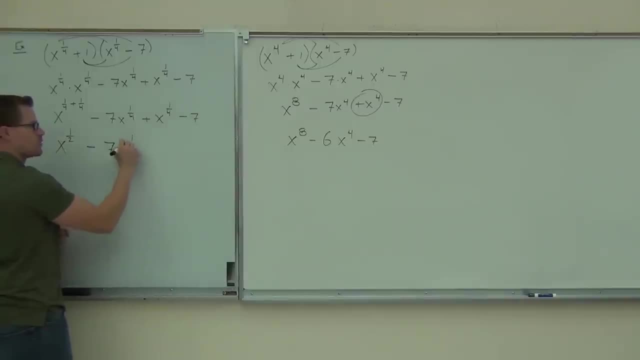 We're combining like terms, like we did there. This should still be x to the 1, 4th and then minus seven at the very end. Now, of course, I screwed that up too. That's what I was about to tell you. 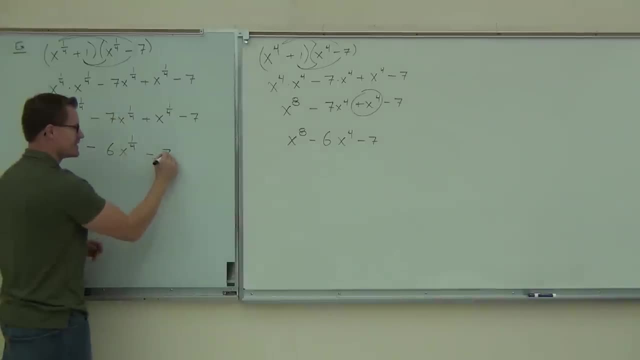 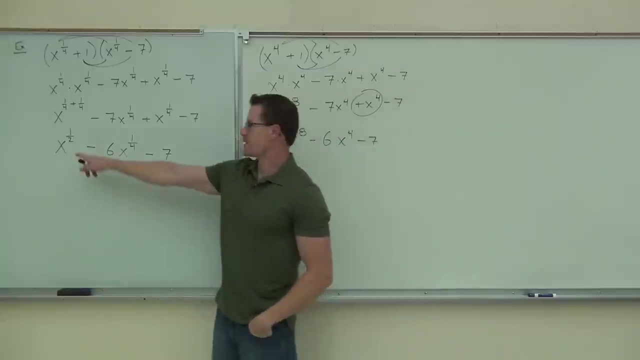 I made a mistake by trying to purposely make a mistake. Ironic, Yeah, this is what I was talking about. the 1, 4th, The seven was just clearly a mistake. Now, next question: I have x to the 1 half. 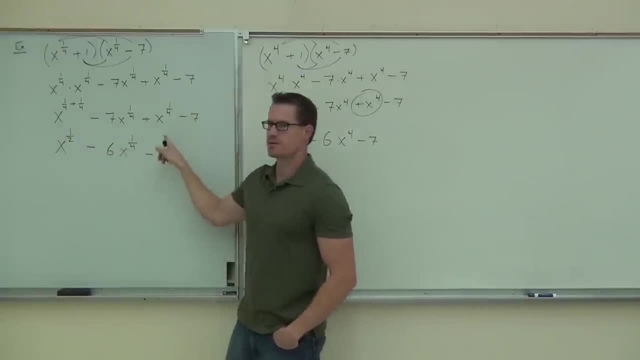 minus x to the 1- 4th. Can I combine those? No, because it's subtracting. That would be like doing this okay, You can't do that. They're not the same power. Did you guys see the? 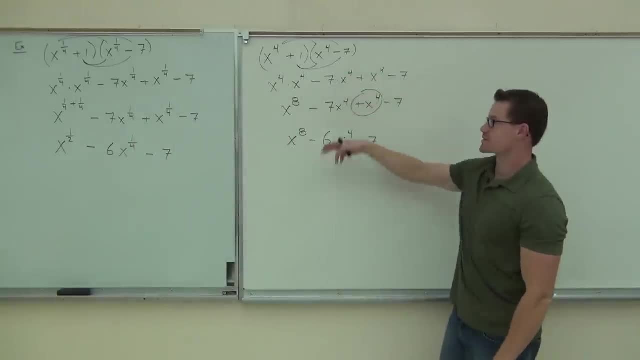 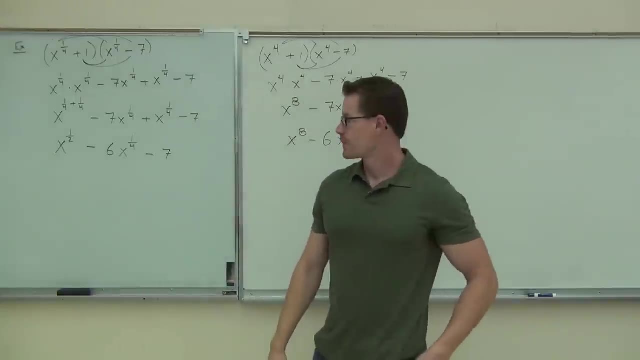 are you okay with that example? Notice how we did exactly the same process. We had one extra step because I want to do that step to show that we are actually adding, but that's it. Sorry if that was x to the 1- 4th. 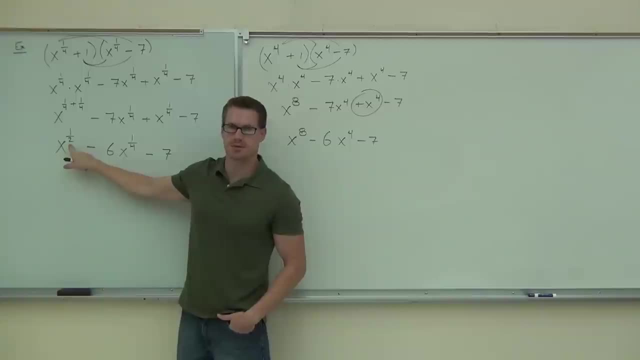 you could combine them right. If this was x to the 1 4th, absolutely, That's it okay. Yeah, For instance, if this was a 1 16th and a 1 16th, then that would be x to the 1,. 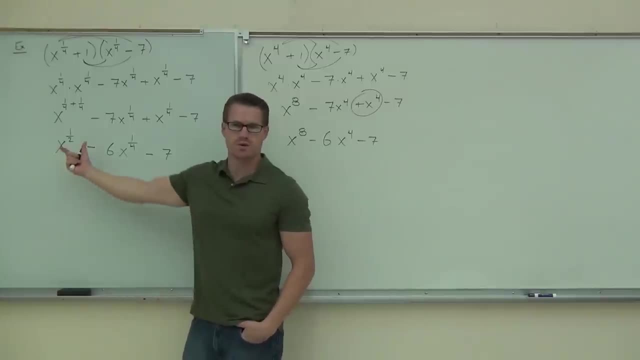 no, it wouldn't be the 1- 8th. Yeah, if that was 1- 4th, then we could. that's the only way we could combine them. Or if this was 1 half, right, But we can't get 1 half out of that. 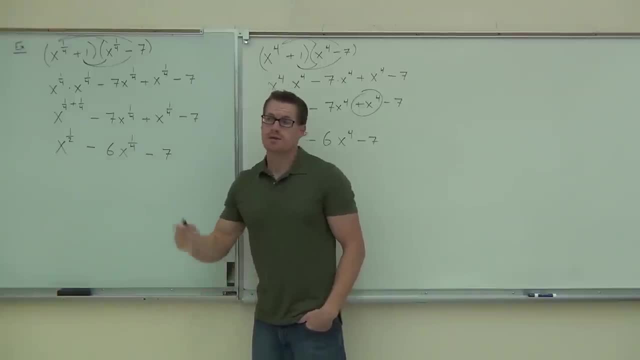 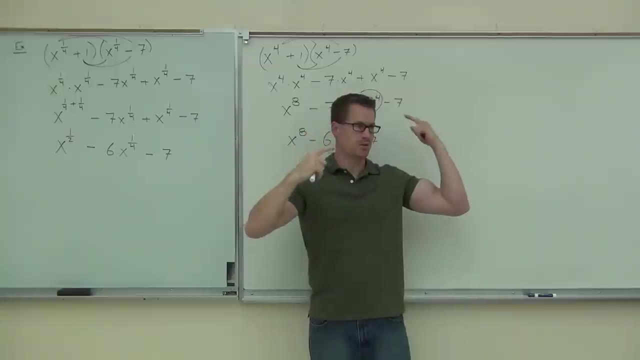 That's trickery, Not trying to be tricky. you know They are the same exact exponent rules you just used here. It's just for some reason your head likes to do different things with fractions than they do with whole numbers. That's why fractions are tricky for people. 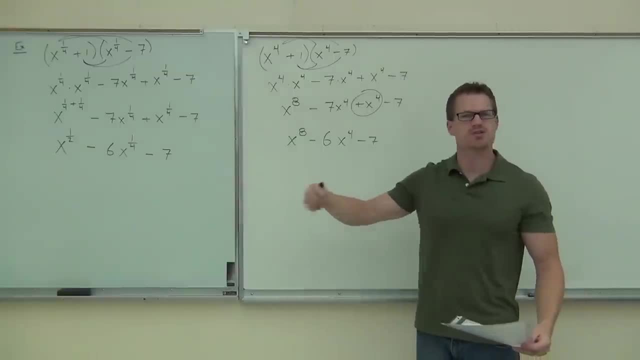 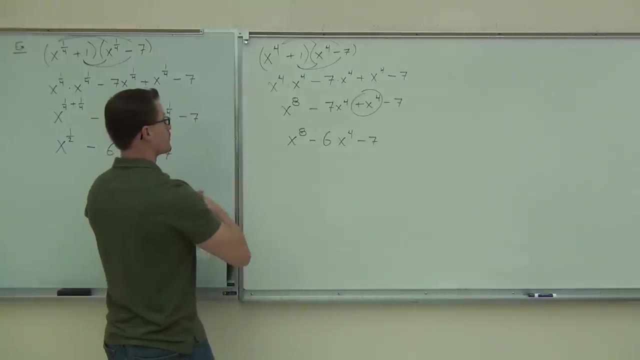 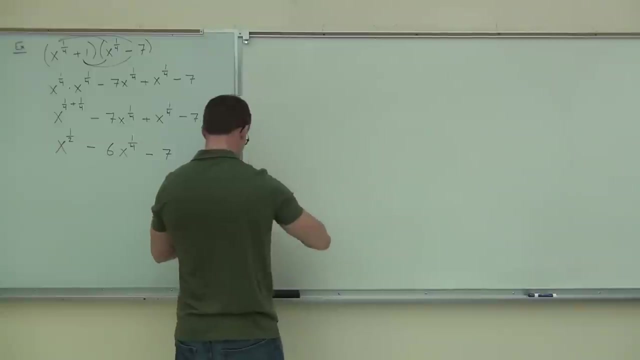 That's why. Are you okay with it? Can you try to keep up on your own? Let's really work through these slowly. You do not have to race through this stuff. Make sure you get them right. Okay, So this is what we did last time. 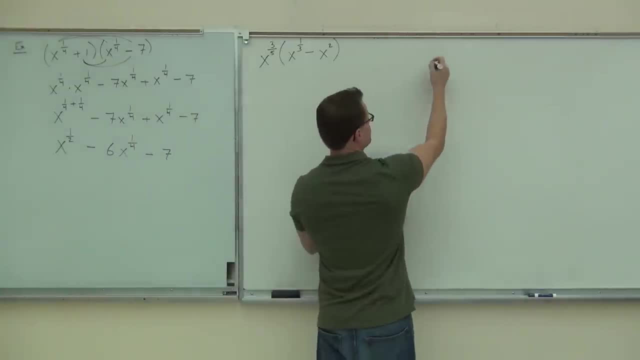 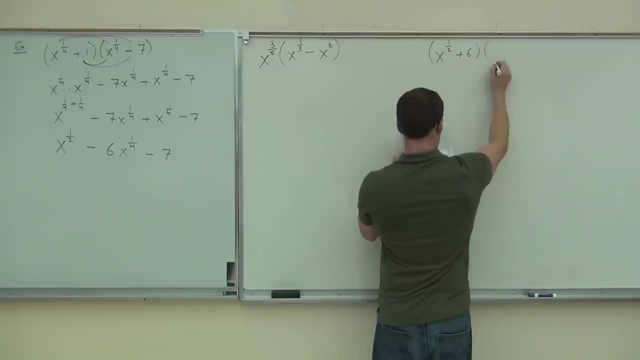 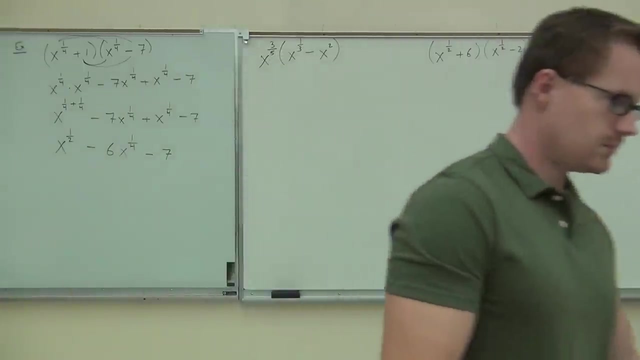 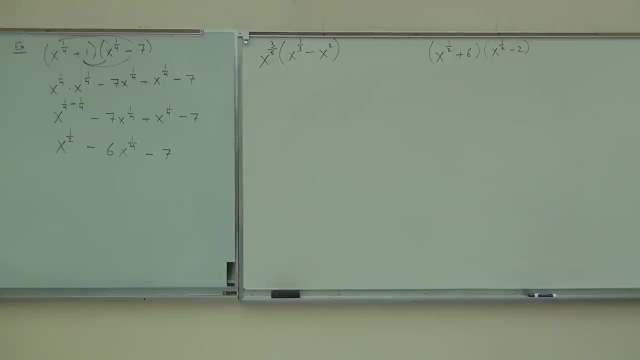 I want you to work on that one, And this is one we just have looked at See if it's finished. So of course, the only difference is just here that we're writing down an extra step we would normally do. in our head It's still distribution. 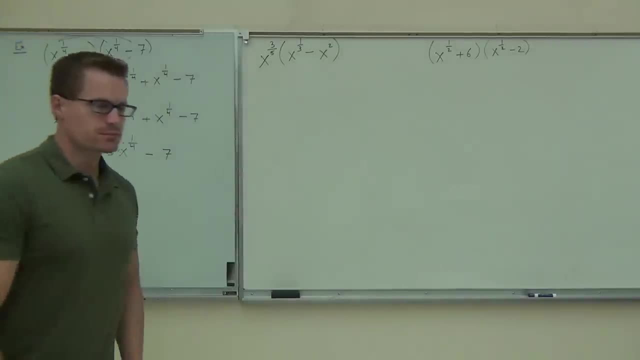 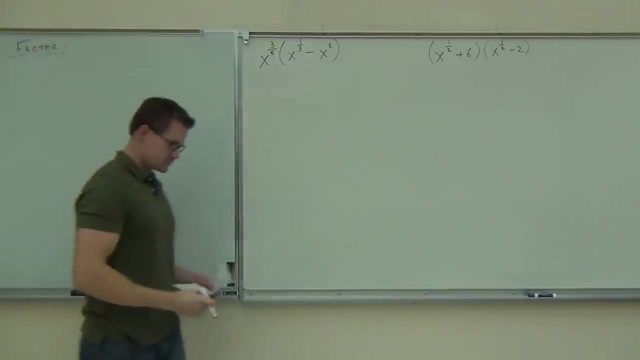 You're still getting rid of parentheses that way, Thank you. Thank you, By the way. if you ever get confused on what to do, sometimes it helps to write out a similar example without fractions, For instance, if I forgot what to do on this problem. 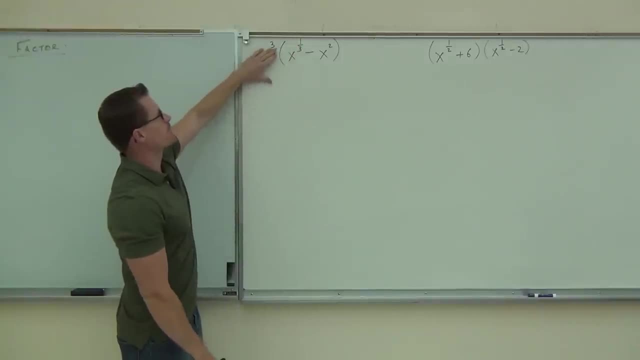 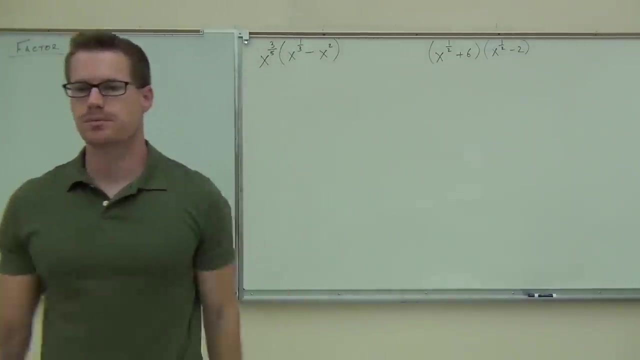 I'd imagine there was no fraction here and say: how would I get rid of x to the third times this quantity? Oh, I'd distribute. You're doing the same process just now. you have those fractions. just carry those along with you. 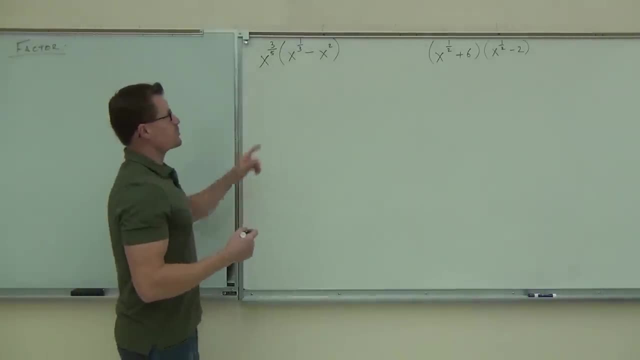 So, on our first problem, we are going to distribute. When we distribute, we're taking our outside term, outside factor, times each of the terms inside our parentheses. So in our case, we're going to multiply x to the three-fifths times x to the one-third. 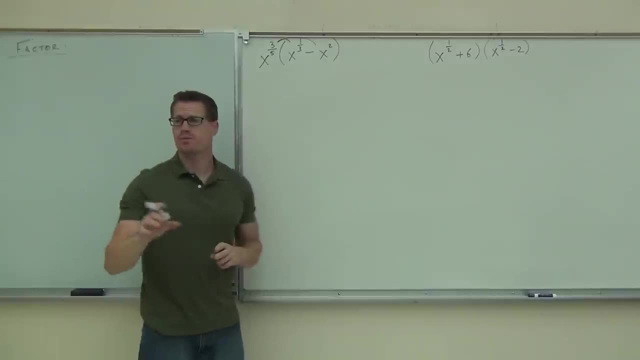 and then we're going to do x to the three-fifths times x squared. Did you all get the process down at least? Okay, We're just going to write that out. Just don't do it in your head, because again, 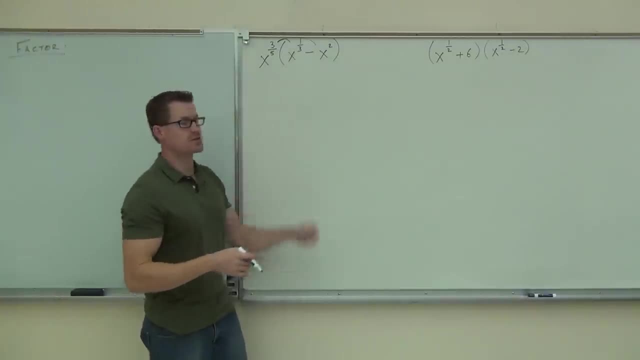 what people like to do on this is they go: oh, we're multiplying. that means I multiplied fractions, I'm going to get three-fifteenths. that reduces to one-fifth. A lot of people give me one-fifth on this problem. x to the one-fifth. 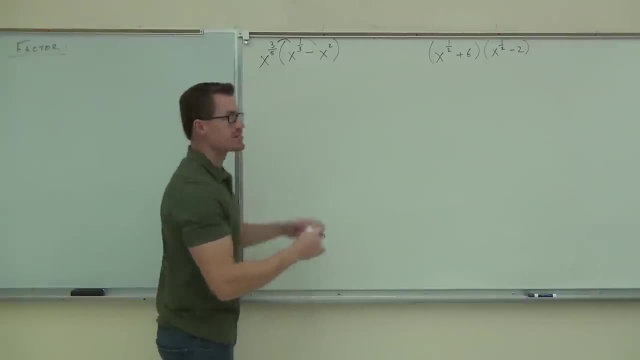 and that's not what we're going to get. Instead, what we need to understand is when we distribute, yes, we are multiplying, but what it turns out is we're multiplying common bases, Like that. And notice when you write it out like that: 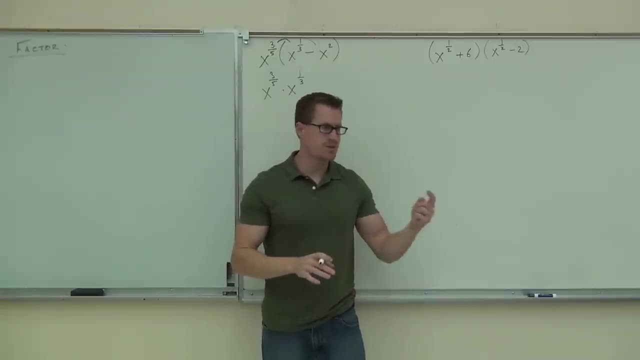 it looks like the excellent rules we just practiced. It just looks like those. Maybe you did those on your. did you do those on your homework? If you just started your homework, I hope that you did. otherwise, you're going to have a lot of homework in the next couple of days. 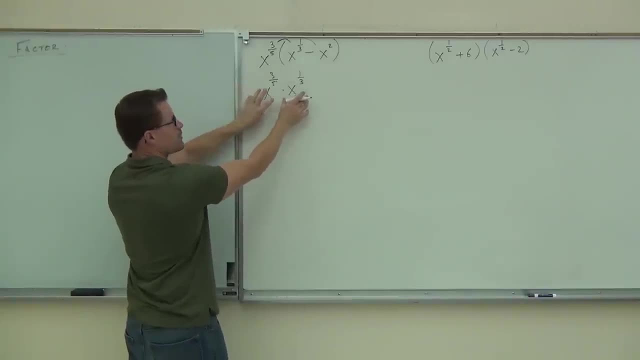 We distribute, we have our like terms, or, sorry, we have our common bases being multiplied like this, and that clues in that we're going to add exponents. Then, of course, we have x to the three-fifths times. 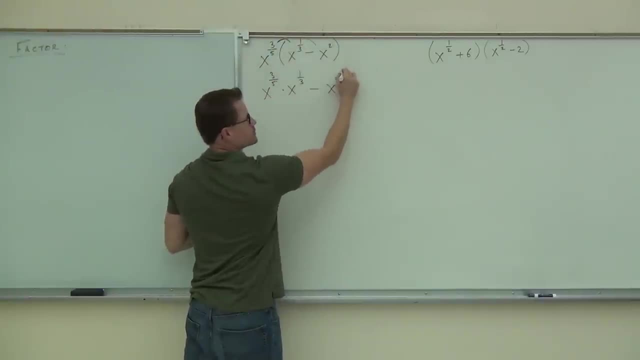 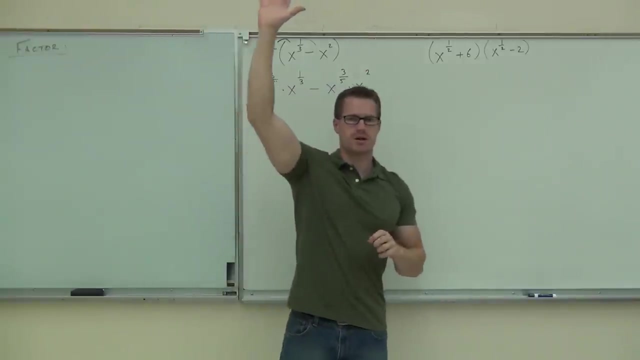 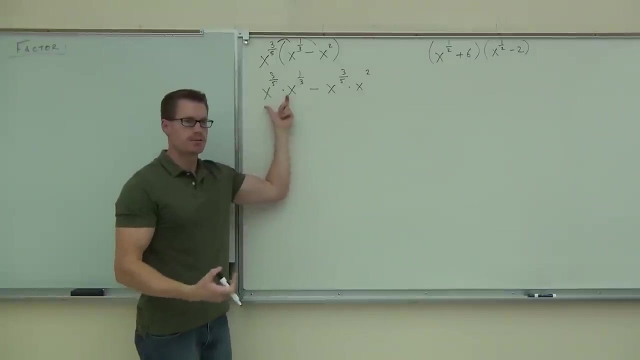 we're going to consider that to be negative. two x. we're going to minus. we're just going to write that out as well, Which means we haven't made it that far and have that on your paper. Okay, Now again, when you have common bases, you don't multiply, you add. you add those things. 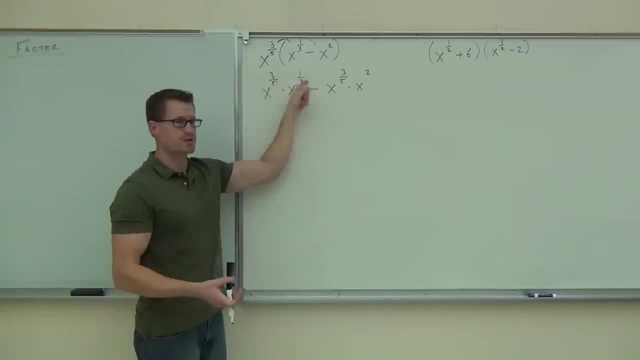 So do this off to the side. Take your calculator out if you'd like to do this fraction off to the side if you want. We're really just doing three-fifths plus one-third. This means x to the three-fifths plus one-third. 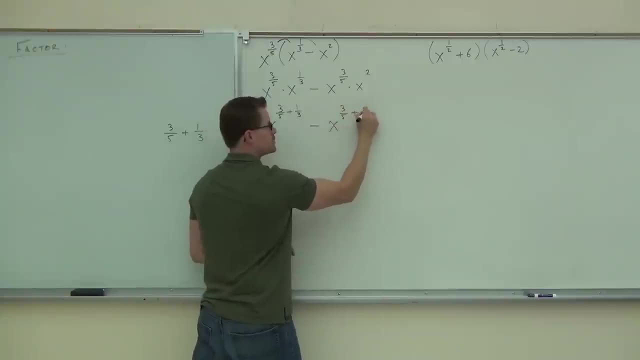 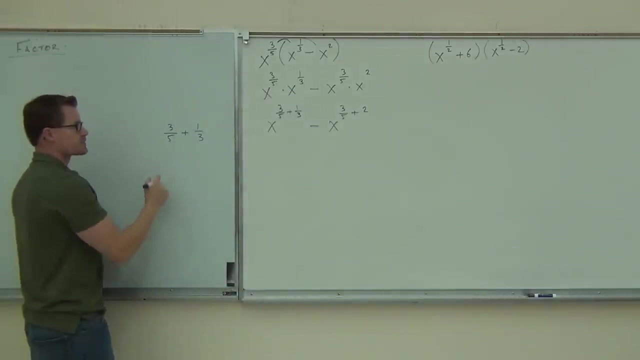 This means x to the three-fifths plus two. You're not going to multiply that either. Don't add one, multiply the other one. We're adding both of them, both those exponents. So three-fifths plus one-third. of course we need a common denominator. 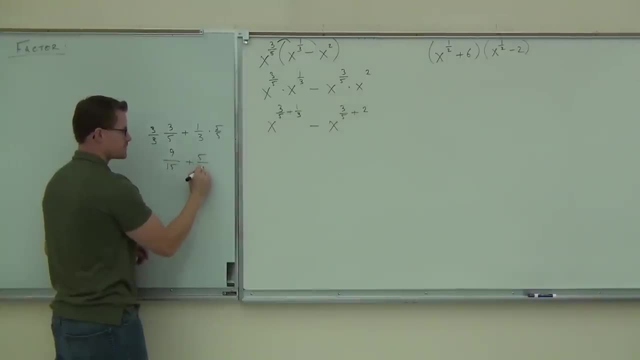 You get nine-fifteenths plus five-fifteenths, So I'm getting 14, 14-fourteenths. That doesn't work. 14-fifteenths- Did you get 14-fifteenths as well? 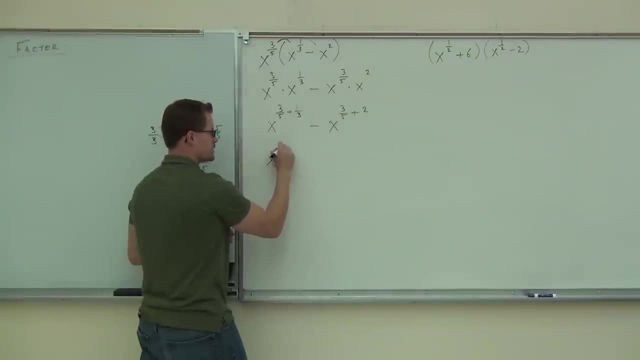 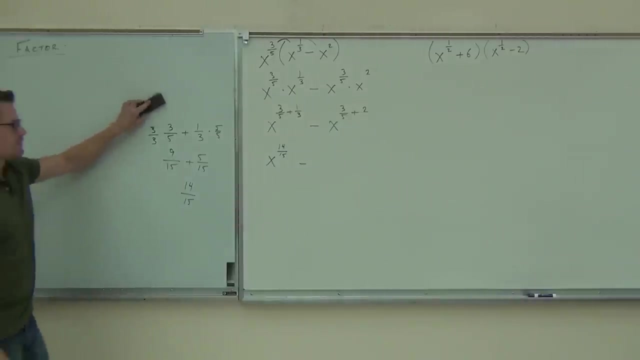 Yeah, So our first expression is x to the 14-fifteenths. That's our first term Minus. We're also going to do the three-fifths Plus two. I'll erase my scratch paper here. 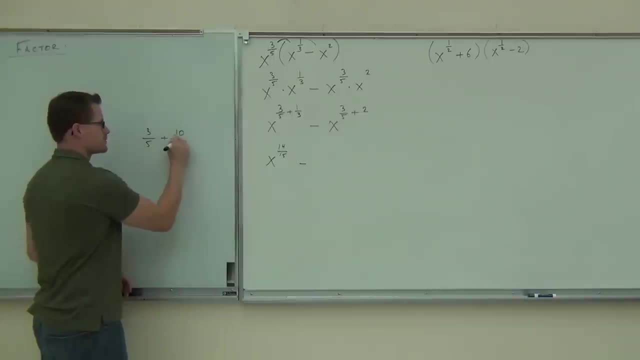 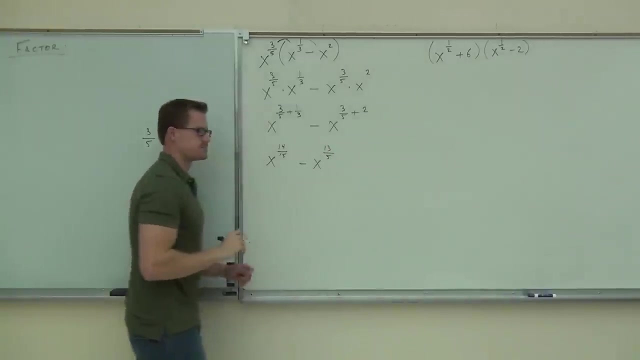 So three-fifths plus two. I know that two is ten-fifths, So I'm going to get 13-fifths If I show of hands. some people got exactly that on their paper. Good, All right. 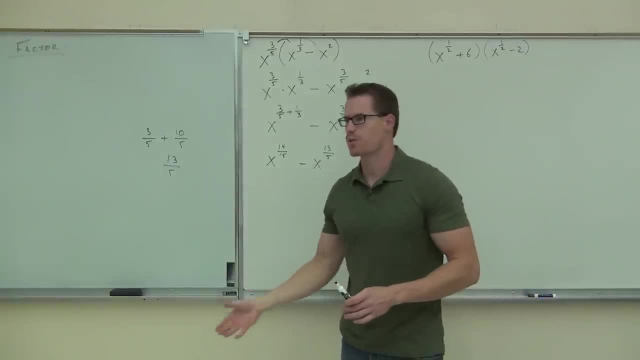 All right, Make sure your fraction work is up to par. Again, this is not fraction class, right? We're way beyond that. We're two classes beyond this stuff. But if you need help on fractions, please by all means come and see me. 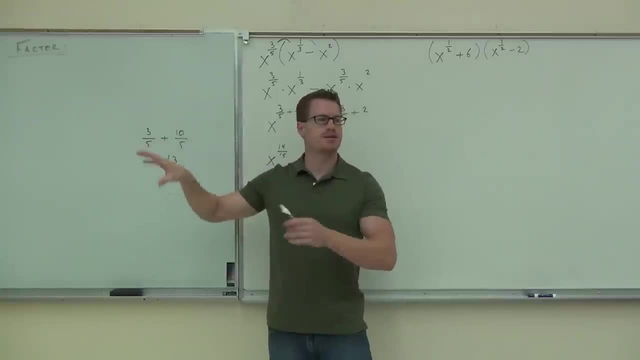 I will help you if you're struggling with this stuff. Okay, I can't spend the time to teach you here- We're two classes beyond that- But I will spend some time on your own time to help you with that if you struggle with fractions. 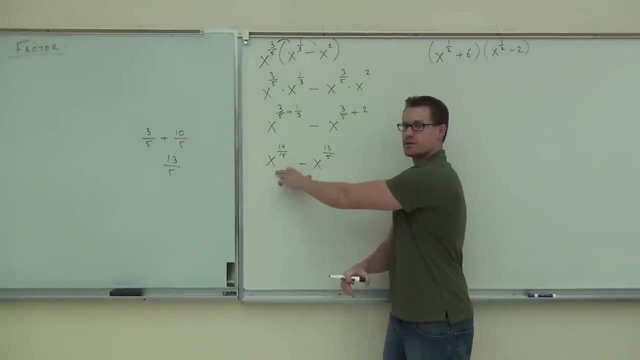 Anyhow, moving on, How do I combine these things, How do I combine those? How do I combine those? You don't know? Oh, They have to have the same exact variable to the same power. Look at it, Look at the board right now. 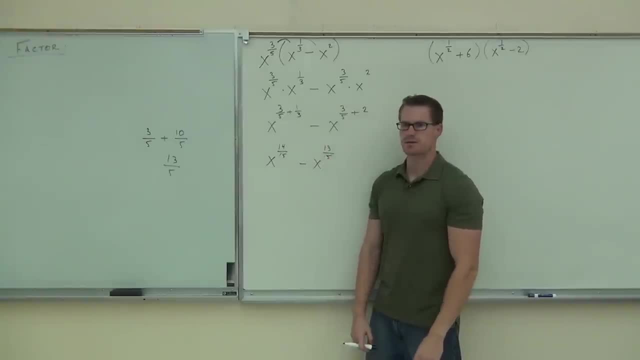 Even if I did this, Could I combine those? No, Even though they would have a common denominator, they're not exactly the same. There's no way to make them exactly the same. You can't do it, You're done. It's kind of nice right. 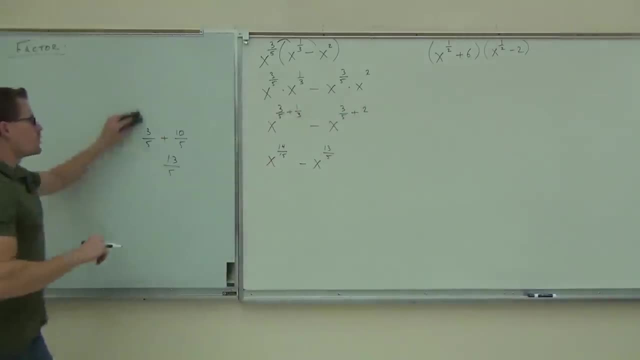 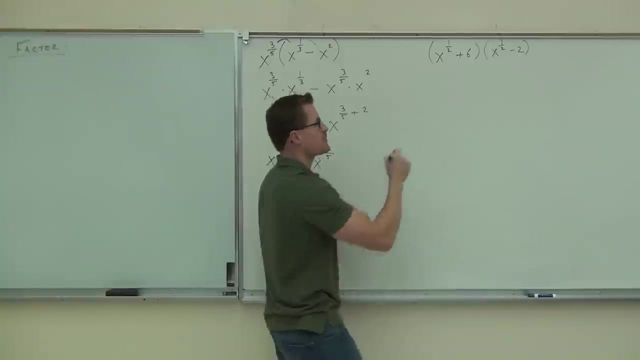 Done, Don't have to go any further. Okay, Let's move on to that one. We have the same process. We are distributing. We have a FOIL situation. as a matter of fact, Two terms times two terms. We're going to do the same process we did over here on our last example. 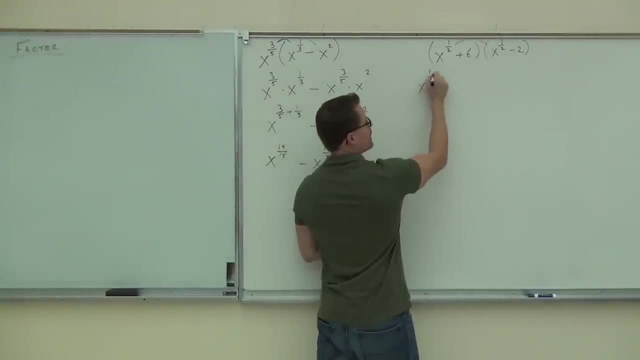 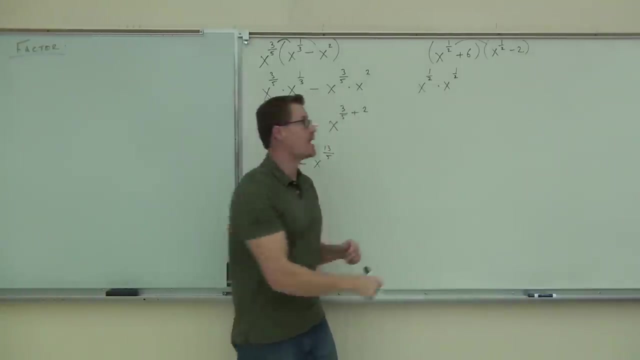 We distribute, which means we multiply term by term. just making sure that we're writing out those steps because I don't want you to miss it, I don't want you to do this in your head, because that's when those mistakes happen. So we have x to the 1 half times x to the 1 half. 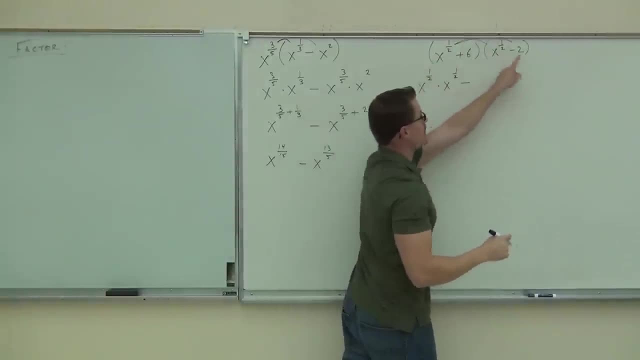 Next step: we're going to have minus, because we have this minus 2x to the 1 half, plus 6x to the 1 half, And then, lastly, we'll get a minus 12.. Did you make it that far? 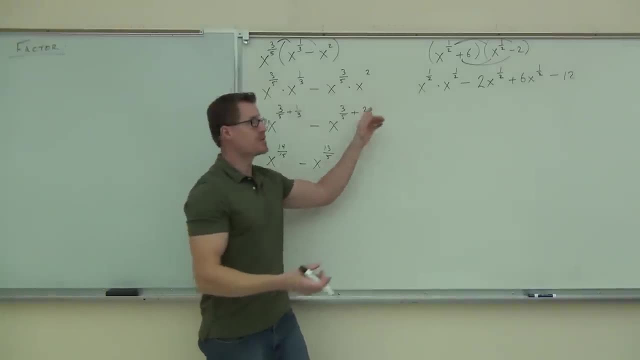 Good, That's partial credit right there. At least you understand the distribution process and you've written out the steps. Yes, Do we have to write it down like that on the test, Please, I want to see it. Okay, I want to see those steps. 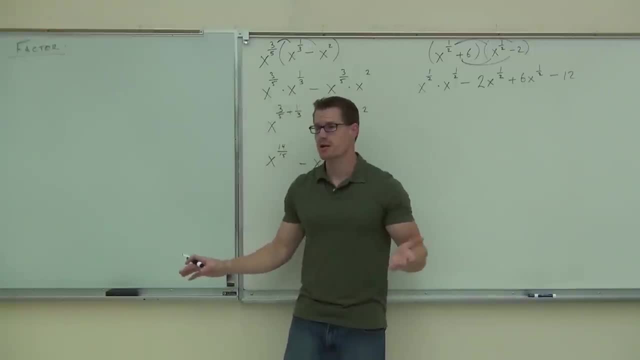 Right now we're learning it right. Later on, when we pass this chapter, no, I don't care, But for right now, yeah, I want to make sure that you guys are getting this. The reason is, if for some reason, you go directly to here, 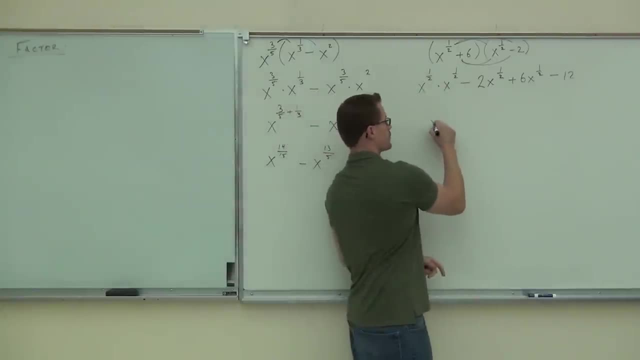 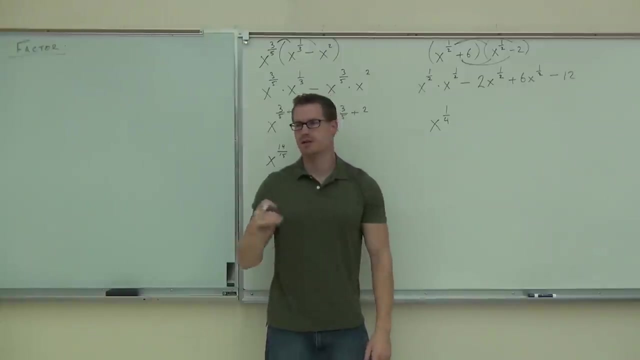 a lot of people are going to give me this on the test. They're going to give me x to the 1 fourth. Guaranteed that this happens every year. I give the same exact problem on the test. People will always give me x to the 1 fourth guaranteed. 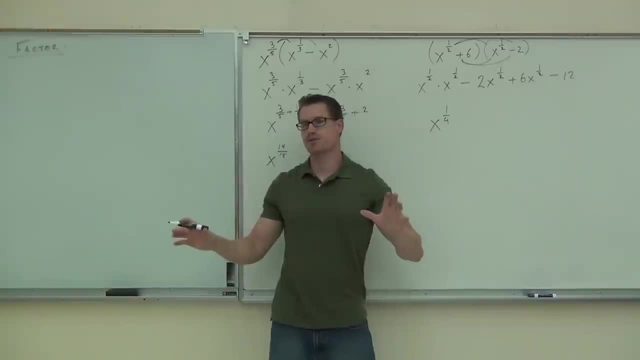 So if you go directly from here to here- I know you don't know what you're doing at all- I'm going to give you zero credit. But if you go from here to here to here, I know at least your new distribution will give you like two or three points. 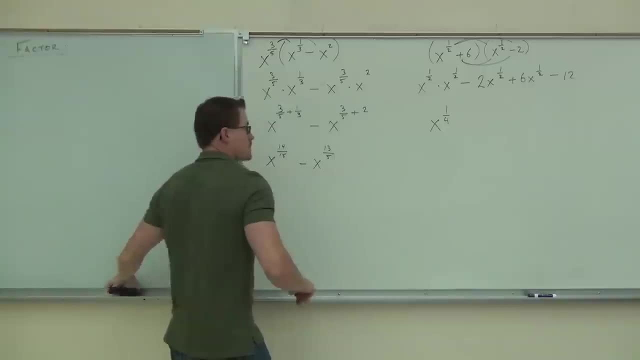 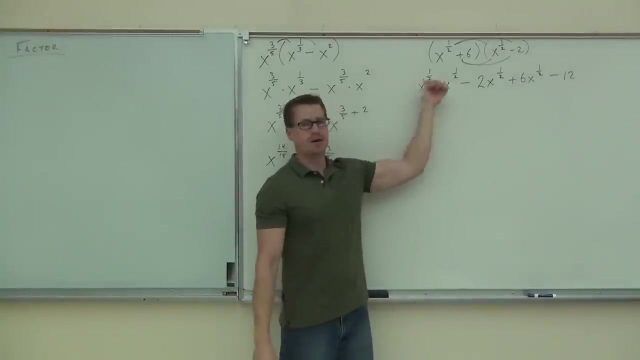 Does that make sense? So I need to see that. Okay, So we're back to this thing. We have x to the 1 half times x to the 1 half. Do we add, subtract, multiply or divide those things? 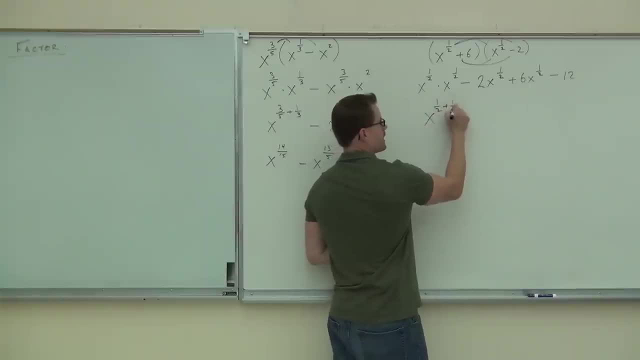 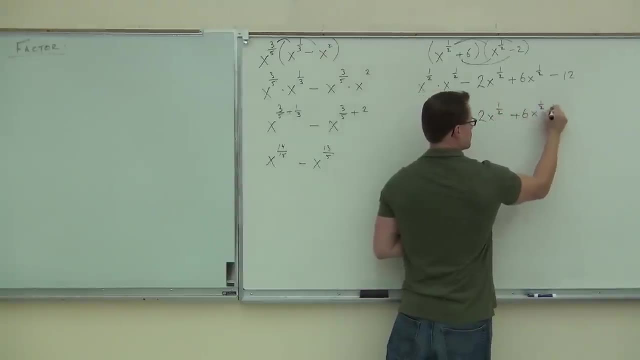 So we're going to get x to the 1 half plus 1 half. Put x or step up there. so you see what's going on. Let's leave the other stuff for just a second. x to the 1 half plus 1 half. 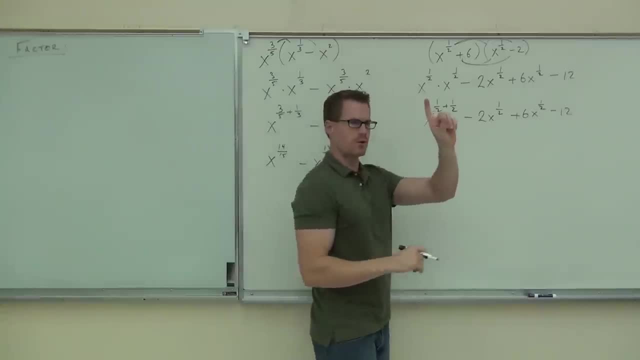 How much is 1 half plus 1 half? We're going to get 1.. Yeah, not 1. fourth, just x. Interesting, isn't it? X? Can you combine these things? We have negative 2 x to the 1 half. 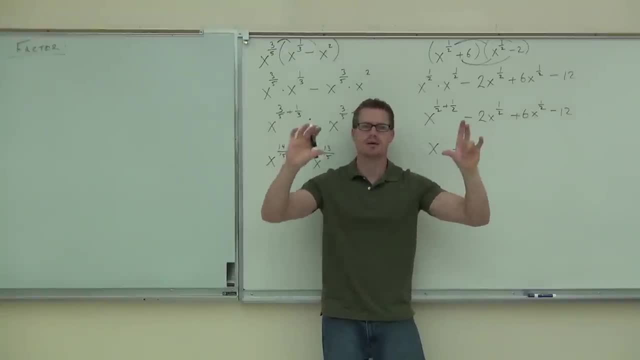 We have 6, x to the 1 half. Those are the same variable to the same power. Those we can combine You're going to get it looks like positive 4, but it's x to what power? 1 half. 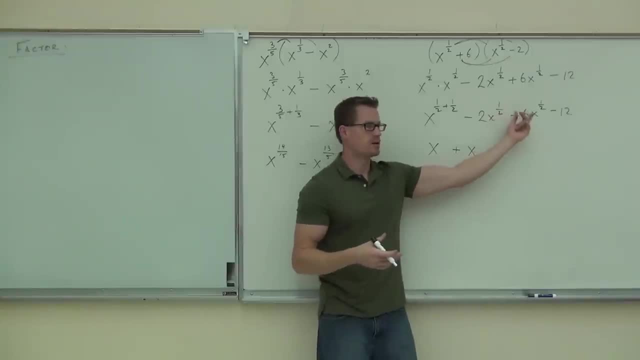 So that doesn't change. So this is not going to give me 1.. I need you to look up here at the board. real quick. Understand something. If you got x to the 1 half, If you got x to the first out of this, then what you're saying to me is: 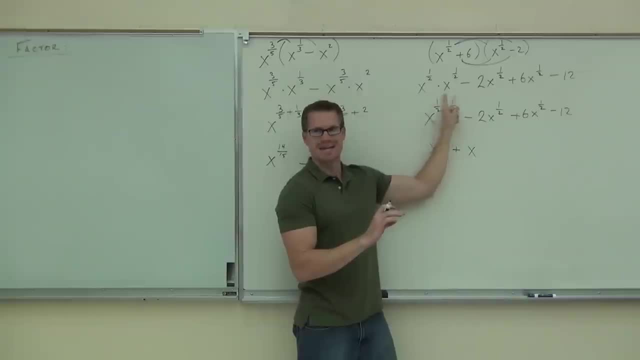 that multiplying common bases is exactly the same as adding like terms, And they're not. Multiplication is not the same as addition. Therefore, you can't possibly get the same thing if you multiply or add. I know I know some of you are saying: well, 2 times 2 is the same as 2 plus 2.. 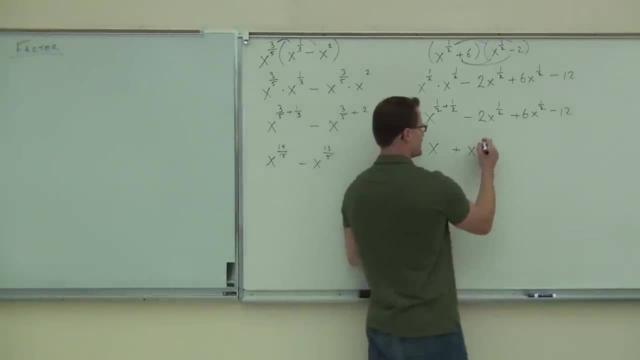 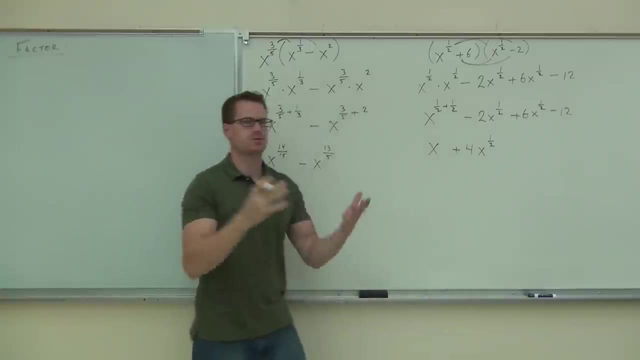 Yes, it is, You were right, But not in this case. okay, So yeah, we get 4, for sure, We get x to the. It's still 1 half, though When you combine like terms, you don't change the x. 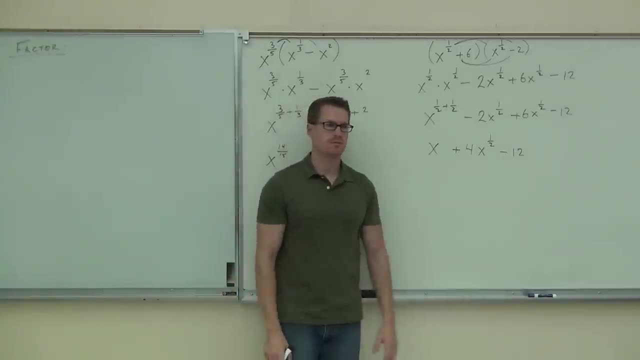 Minus 12.. Can you go any further? No, Yeah, you can simplify the x and just put it in the radical form. Okay, you can, if I want a radical form, but I mean combine any more like terms at all. 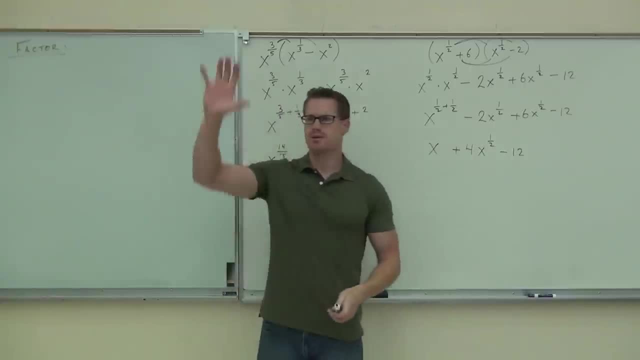 No, Okay, then that's it. You're done on that problem. Raise your hand if you feel. okay with this. so far Now there's an f word on the board. You think you're going to get an f word on Mondays, right? 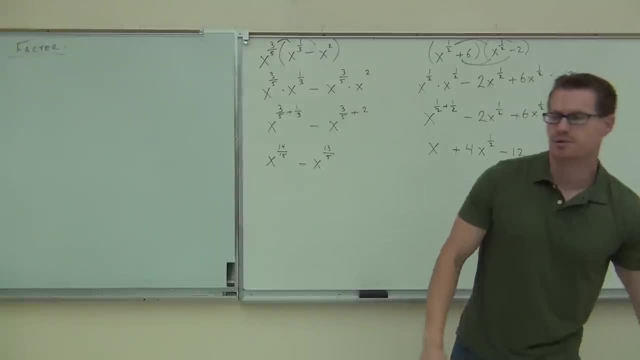 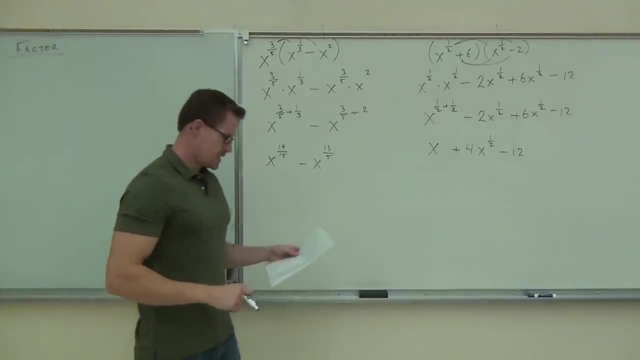 We're going to learn how to factor using these radical x or rational x ones. Now I'm going to do this kind of Slowly. I want to make sure you really get this. We're going to do it step-by-step, just like we're doing our distribution, because if you try to do this in your head, 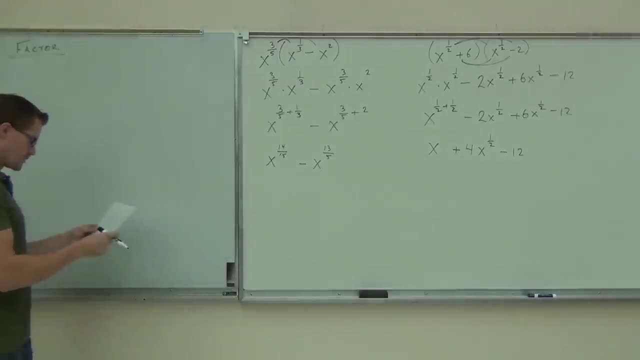 sometimes it gets a little bit messy if you're really not paying attention to what's going on. What we're going to do is we're going to try to factor x to the negative 1 third from Now. this is kind of nice about factoring. is I give you what you're supposed to factor? 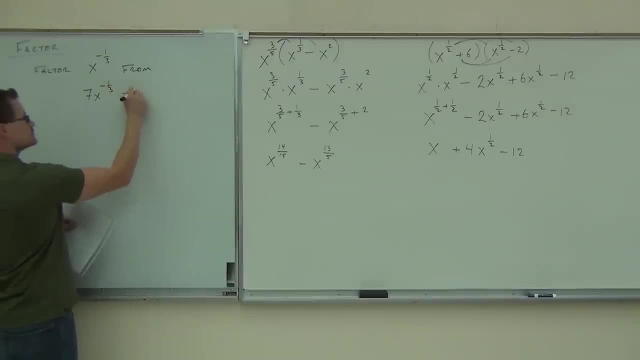 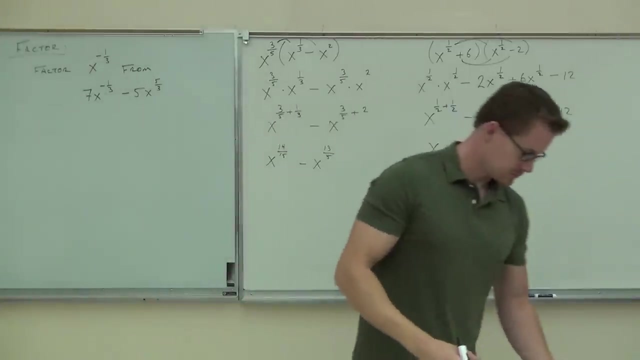 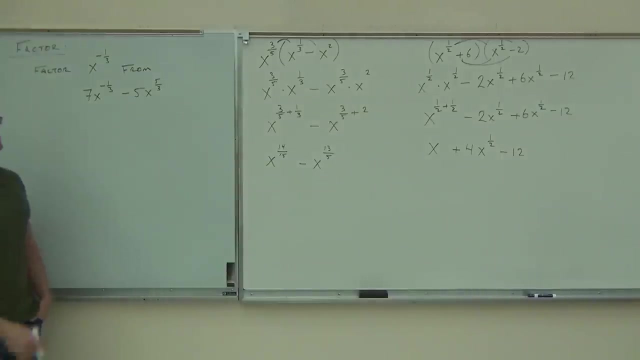 From that factor 7x, I'm sorry, factor x to the negative 1 third. from 7x to the negative 1 third minus 5x to the 5 thirds. Oh my gosh, how are you supposed to factor fractions? 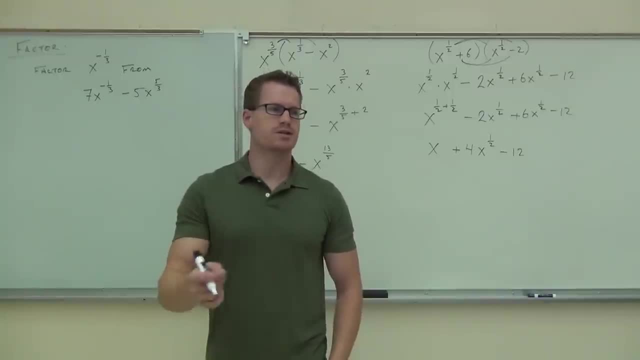 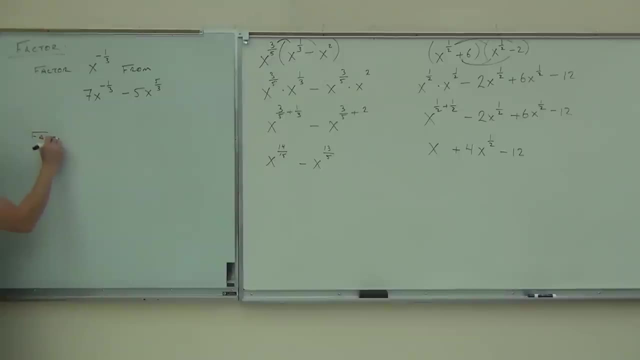 That doesn't even make sense. What the heck? Well, I'm going to draw some comparisons to something you do. you should know how to factor Factor already. Factor x squared from 3x squared minus 10x to the 5th. 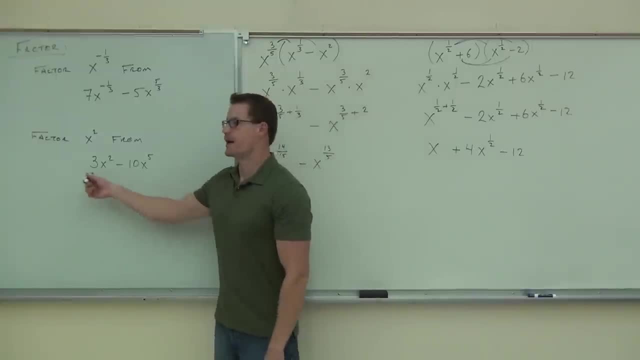 Firstly, I want you to recognize. can you factor x squared from that? Yes, Clearly. Now I need you to understand also what factor means. What are we doing when you're factoring Removing? Okay, removing, That sounds good. 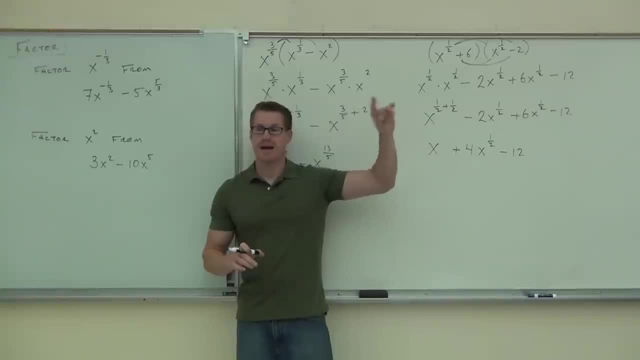 What are you doing when you're distributing Adding? Well, we're not adding, We're multiplying across those parentheses. That's what you do when you distribute right First thing, times first thing, first thing, or outside the thing times first thing. 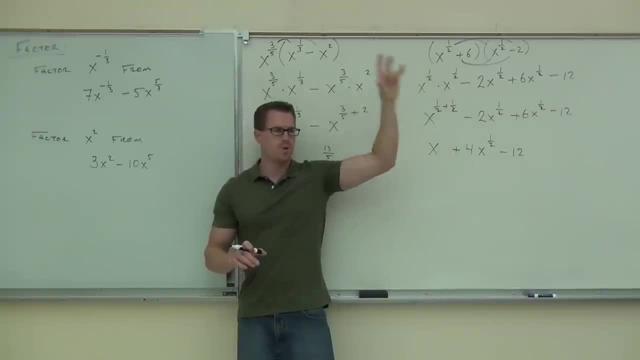 outside the thing times. second thing: Are you with me on this, folks? You are multiplying when you're distributing. Now understand that factoring is the opposite of distribution. right, Instead of multiplying in. What do we do? What are we doing when we factor? 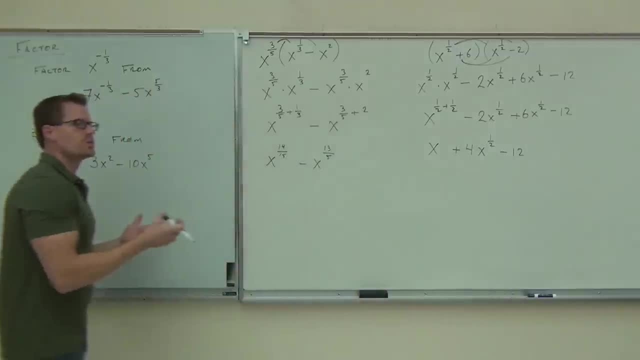 We're dividing out, Dividing, We're dividing here. So what you do when you factor- here's how this works. You're going to understand this because you've done this problem before. What you would factor would be the x squared and you'd say: x squared goes. 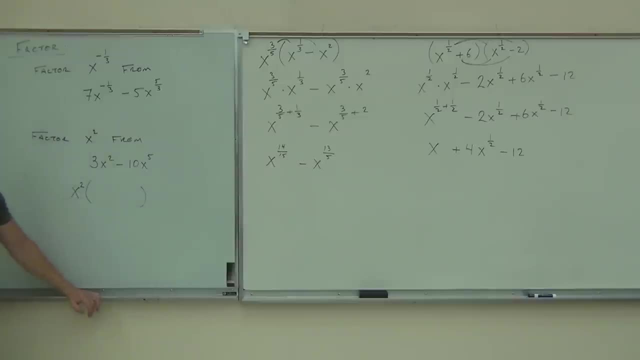 out here and I create parentheses. Now you're going to be still okay. That's how you factor right. Put whatever you're factoring out front. Whatever you're factoring out front, We're factoring out. I can tell you, factor out x squared. 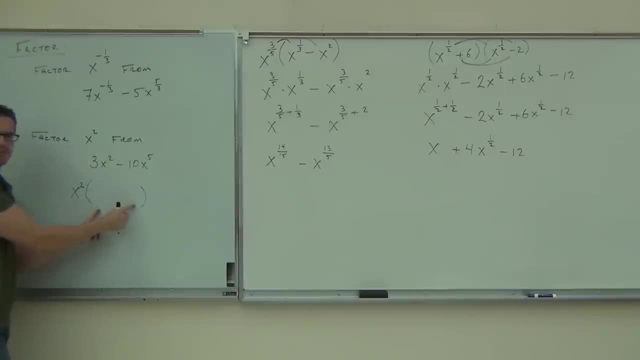 You put that out front. Now, how you get the stuff in here is you take the term and you divide by what you've factored right. That's how you learned at the beginning of this class. You go: okay, what I'm supposed to do is take 3x squared divided by x squared. 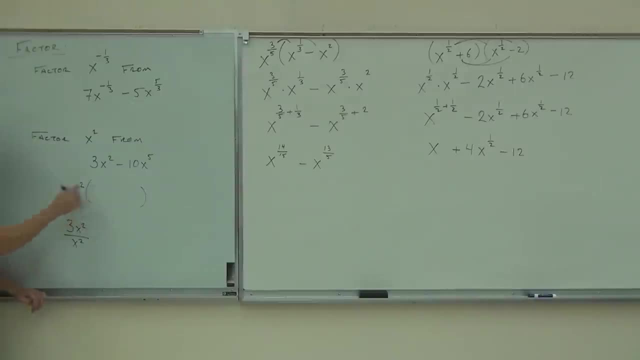 I'm dividing out x squared. Can you tell me what's going to go right here Now? that should be very old news for us. You should not be learning right now. right, This is just review. This is 3.. If you are learning well, okay, learn real fast. 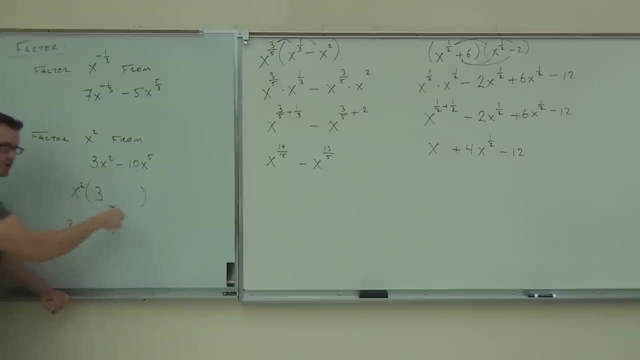 Next up you have. well, whatever this term is- and this term happens when you take my 10, 10x to the 5th or, as a matter of fact, negative 10x to the 5th, take the sign with it divided by x, squared. 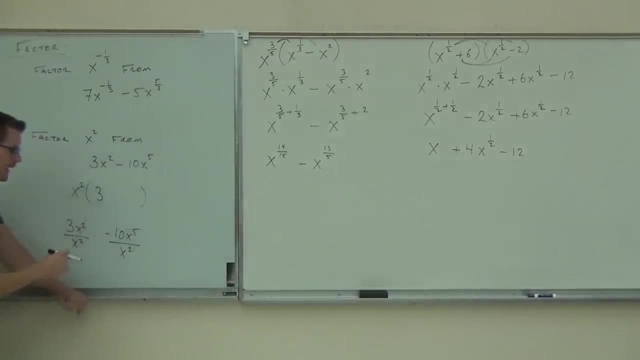 You see, factor means division, and we're dividing out these two of these. What happens when I have negative 10x to the 5th divided by x squared? What happens to those exponents? Oh, you do subtract, Remember that. 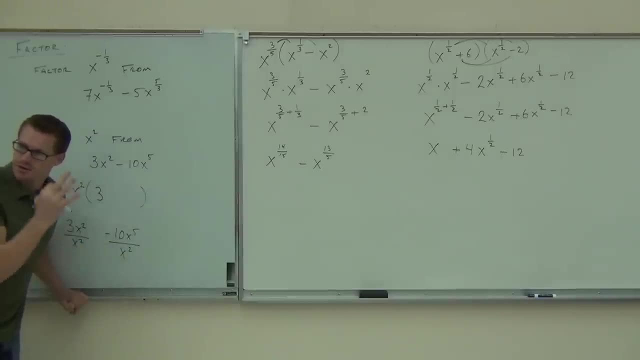 X to the 5th over x squared, you take the 5 minus 2, you get 3.. Some people do that. What are you doing when you do that? Well, you're matching up numbers, But really you're subtracting. 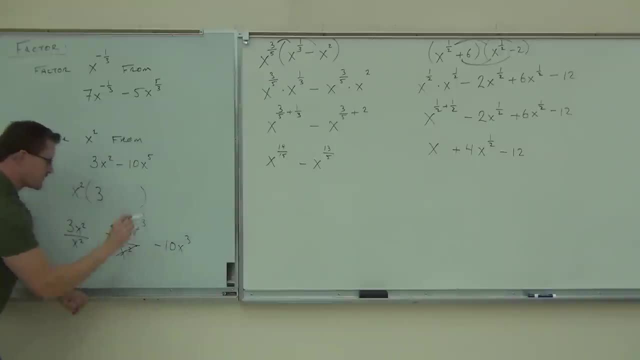 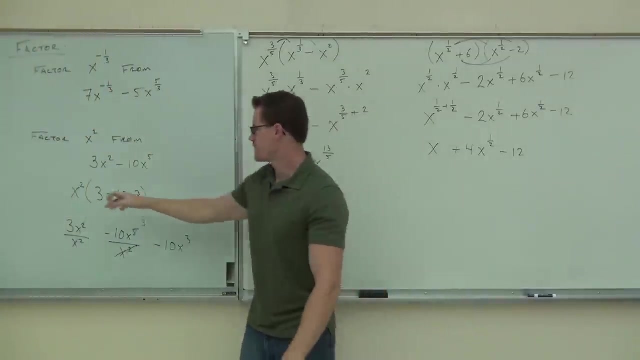 Negative 10x to the 3rd is what you get. That whole thing is gone, And so you put minus 10x to the 3rd. Raise your hand if you don't understand how we got all this stuff And you can check it with distribution right. 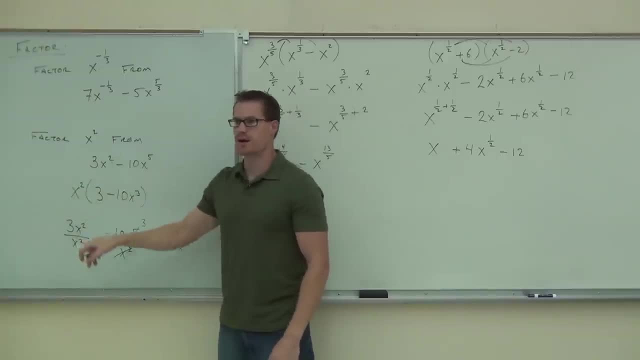 3x squared minus 10x to the 5th, that would be this exact thing. We're going to do precisely the same thing here, only this time it's a little bit easier because, firstly, we have excellent rules. Secondly, I tell you what to factor. 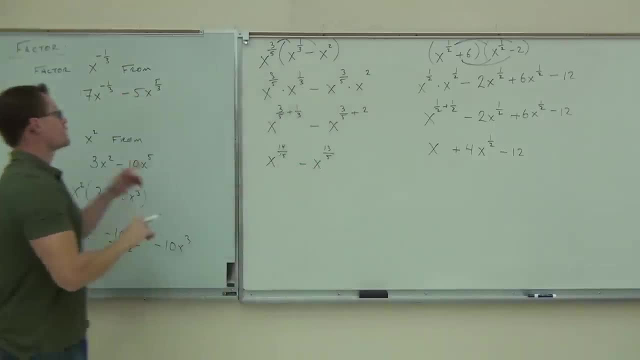 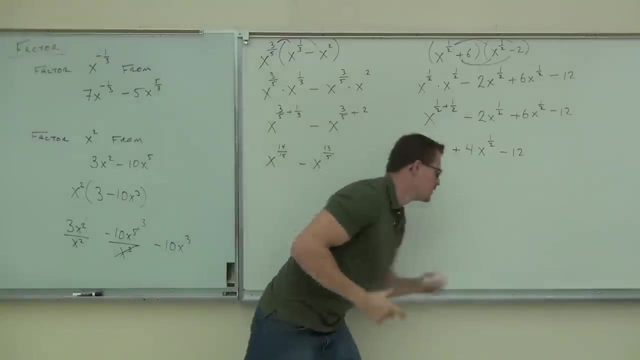 That's kind of cool, so check it out. If we're going to factor out x to the negative 1- 3rd, just like we factored out x squared, when I write my parentheses, I'm going to make that a little bit bigger. 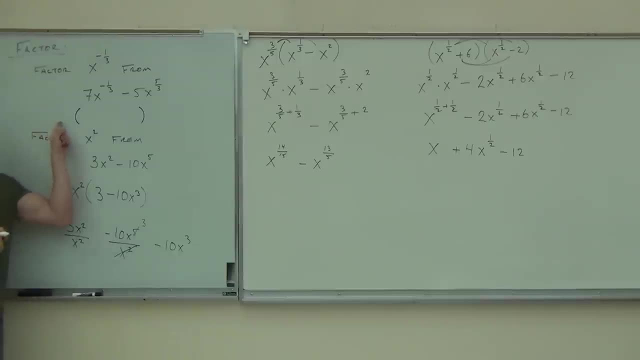 When I write my parentheses. can you all tell me what's going to go on the outside of my parentheses, please? X to the negative. 1, 3rd, Good, Just like we did here. Once you factor out, it goes on the outside. 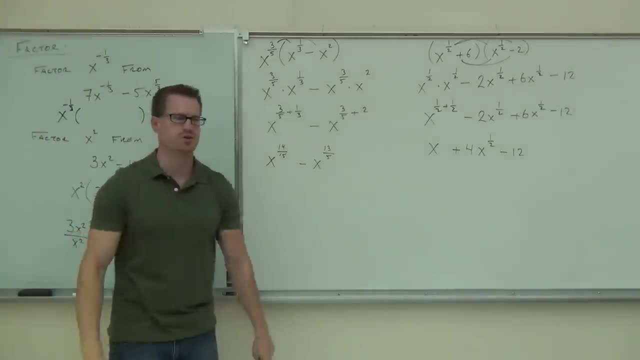 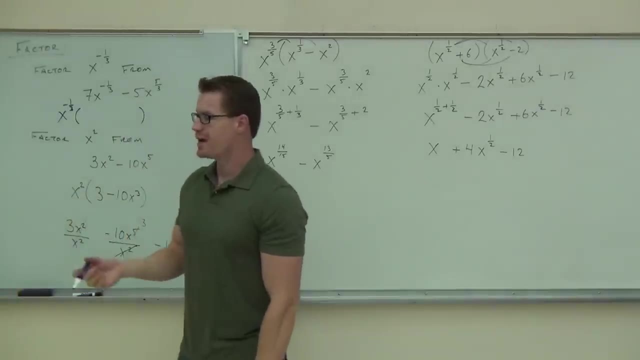 That's why it's called factor out. Right, You're factoring out of your expression. Now, on the inside of our expression, here, what we do is we do this piece by piece. Don't ignore this step. Don't try to do it in your head, because otherwise it gets kind of difficult. 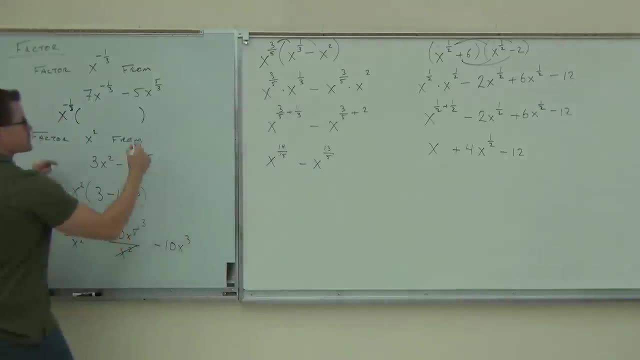 We're going to do the same thing that I showed you right here. As a matter of fact, we're going to take, for our first term, we're going to take 7x to the negative 1- 3rd, divided by x to the negative 1- 3rd. 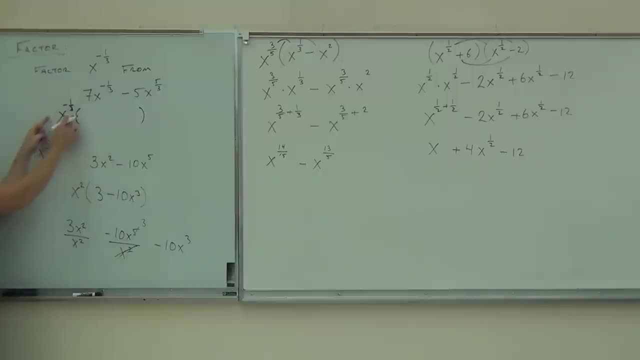 You're taking your first term, you're dividing by what you factored out, because that's what factoring means. Let's look at that. What happens when you have 7x to the one-third over x to the one-third? How much are you going to get out of this? 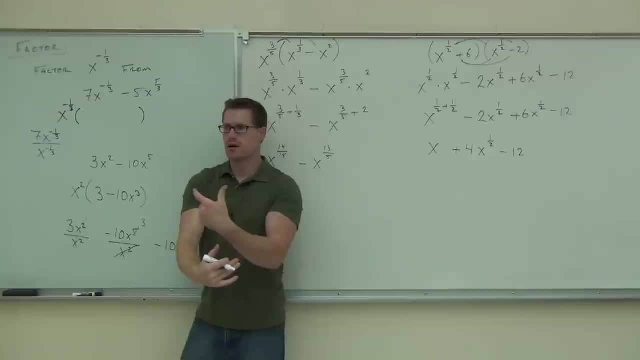 When you have something over itself, it crosses out right. But I want you to think of the rule here. Listen to my voice. watch on the board here real quick. When you have a common base over a common base, what do you do with those exponents? 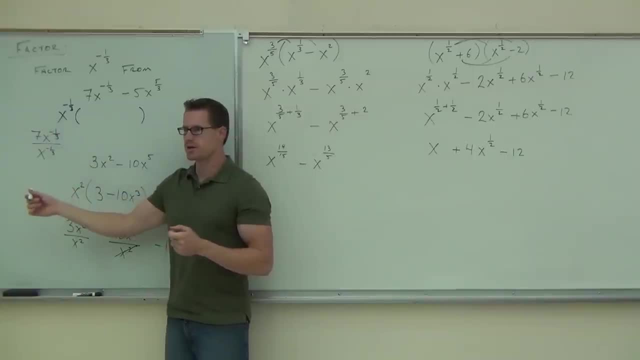 Add subtract, multiply or divide. Subtract You do, subtract, don't you? You'd go. oh okay, This would be x to the negative one-third minus negative one-third. Where are all those negatives coming from? That's negative one-third. You're subtracting exponents because they're on top of one another. 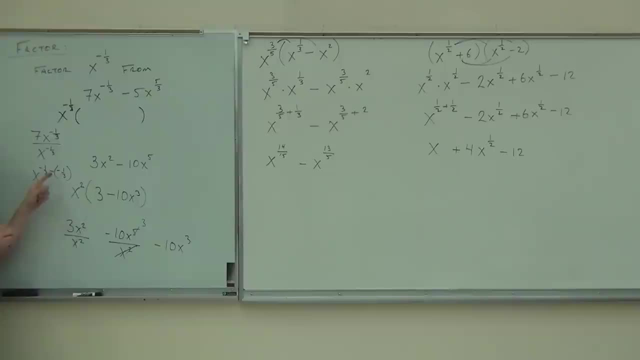 Minus one-third. What's this? minus a negative, do Negative one-third plus one-third. This is x to the Zero. Negative one-third plus one-third is zero. That means you would have just a 7.. Or if you wanted to, here those things are gone, You get just a 7.. 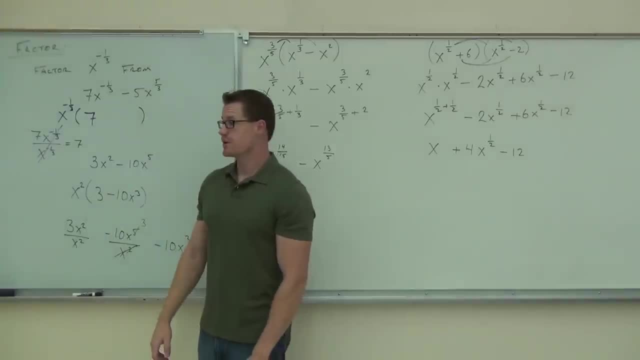 You get 7.. Hey, does that work if you distribute it? Let's try it. If you distribute x to the negative one-third, what are you going to get? Oh look, 7x to the negative one-third. That's cool. 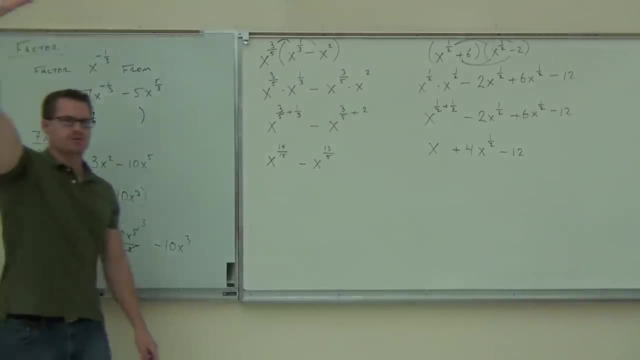 That works. How many people were with me on the first part? People in the middle. are you guys okay with this or no? Okay, Now for the next one. we're going to do the same exact thing with our second term. 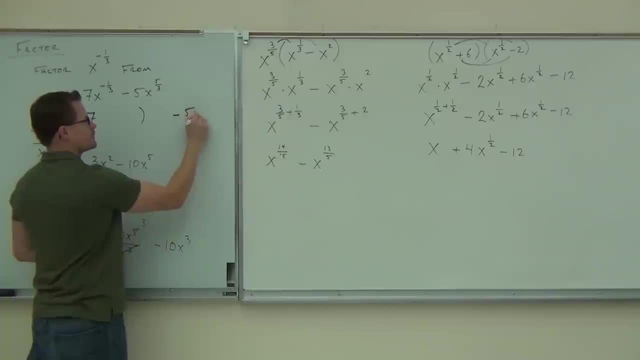 We're going to have negative 5x to the five-thirds over, x to the negative one-third. We take the term We divide by what you're factoring. Hey, tell me something. This one's not going to be as easy as the first one. 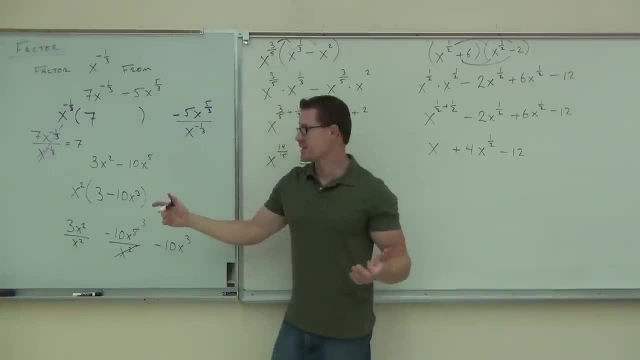 Because that matched up perfectly, But it's going to be the same idea as what I showed you down here. So what do you do when you have a common basis being divided? Do you add, subtract, multiply or divide folks? 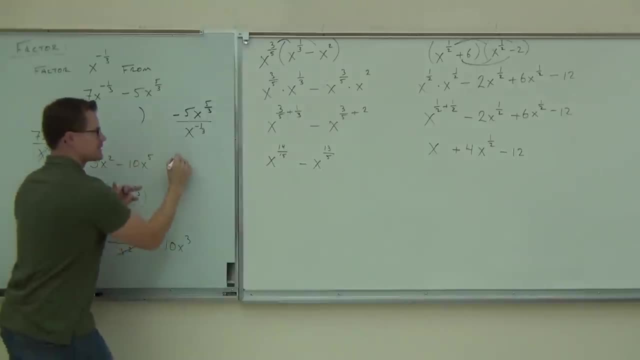 Subtract. So hopefully you see that you're definitely going to have a negative 5.. You all see that right? Yes, We are going to have x. What comes first? five-thirds or negative one-third, Five-thirds, Uh-huh. 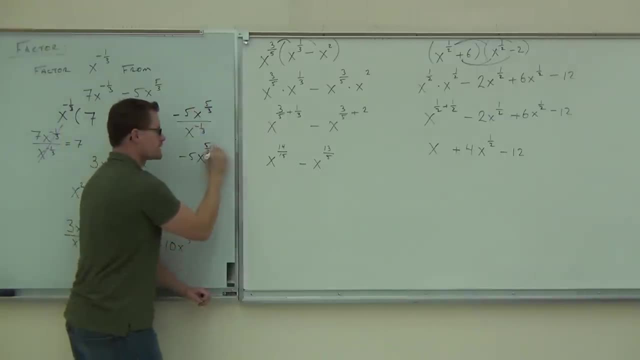 And you said: we subtract right. Yes, What are we subtracting? Negative one-third? We're not subtracting one-third, We're subtracting negative one-third. You see the difference? Uh-huh, Negative one-third. Tell me what happens when you subtract a negative. 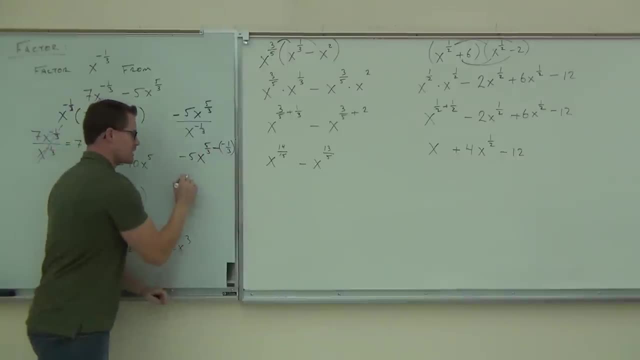 Do you add or do you subtract? still Add. So you get negative 5x to the Six-thirds. That's six-thirds Or two, And you can simplify fractions. if it's an exponent, just like regular fractions, We get negative 5x squared. 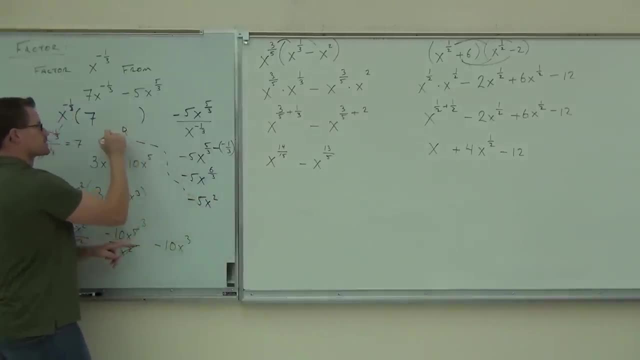 That is what's going on, Minus 5x squared. It's very similar to this process. We took the first term divided by what we're factoring. Second term divided by what we're factoring. That's what's going on in these places. 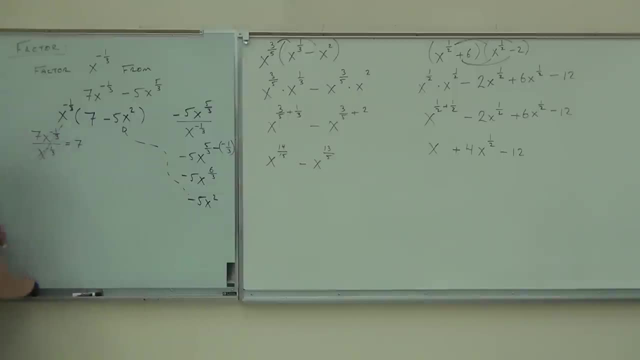 I'm a racist, so it doesn't look as confusing here Why you didn't cancel the x's on that one. When you are dealing with exponents, you subtract those exponents if you're dividing, And that's exactly what we're doing. 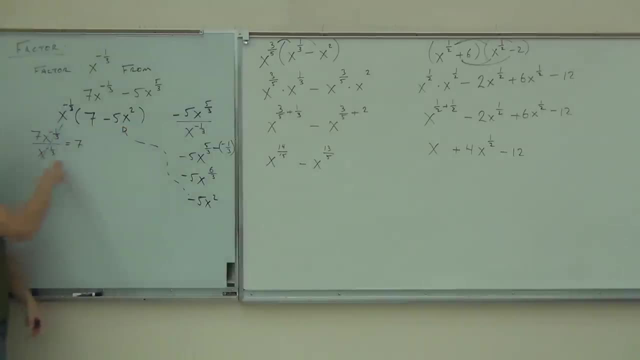 The only reason why we canceled those x's here is because you're subtracting those exponents. Negative one-third minus negative one-third is zero. X to the zero power is one. That's why you can cross them out. That's the whole reason why you can cancel your exponents here. 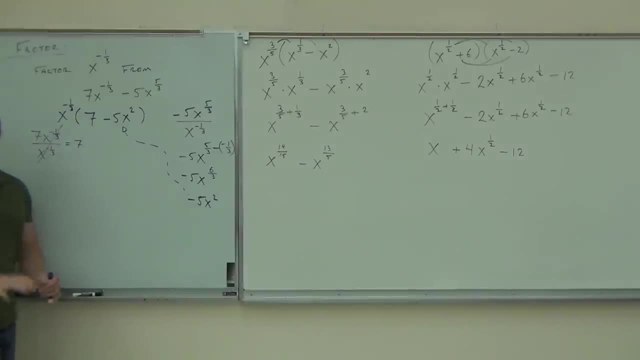 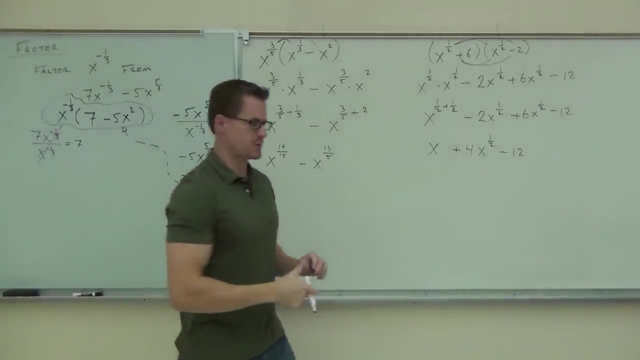 Here they don't match up exactly. You can't do that. Now we've learned to do that example and understand that this is our final answer: X to the negative, one-third times seven minus. Okay, Try one of your own. 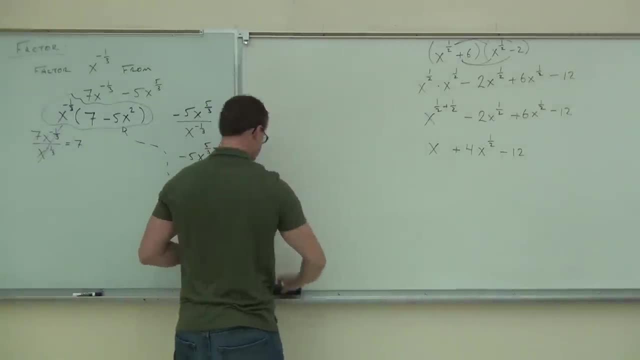 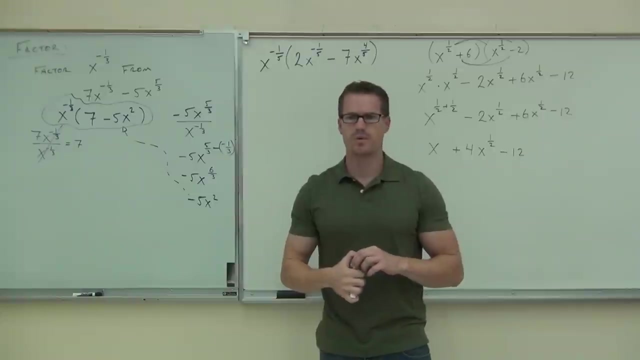 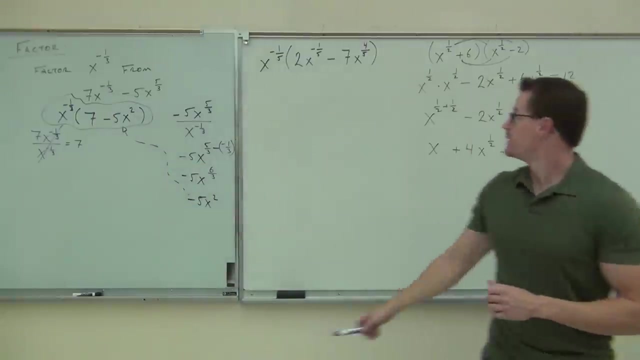 Will the book actually give you what you have to factor out also, or will you have to find that out by yourself? It'll give you what you're supposed to factor out, But almost exclusively it's going to be whatever that is. 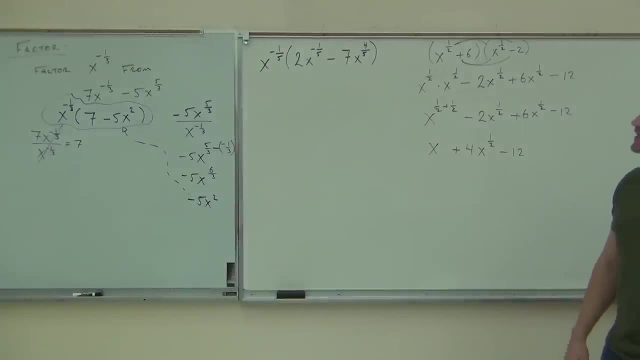 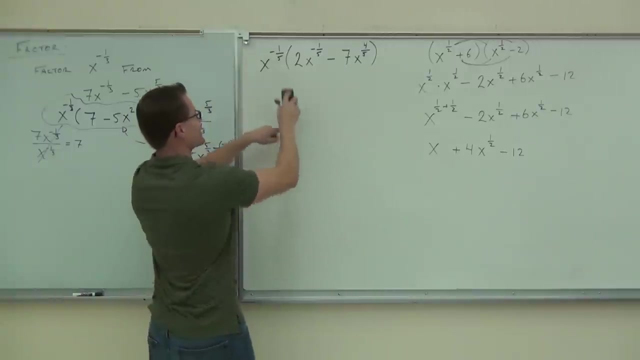 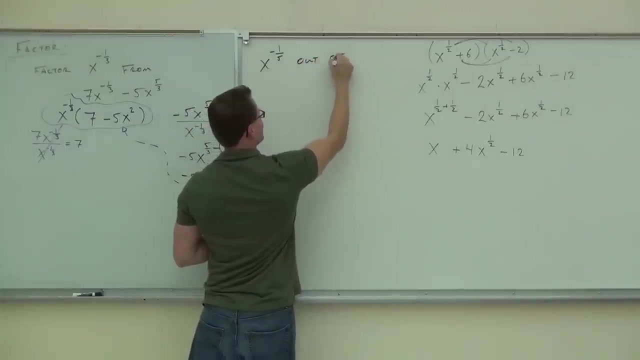 X to the negative. one-fifth times two x to the negative one-fifth minus seven x to the four-fifths. Ah, shoot, I meant to say: factor this out of that. Darn it look. I'm like, oh, this doesn't look anything like what we're doing. Back to this out of. 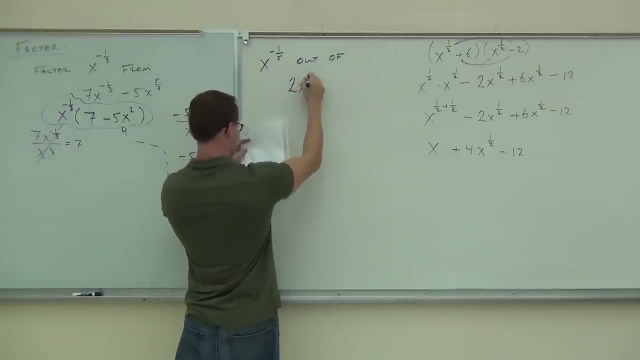 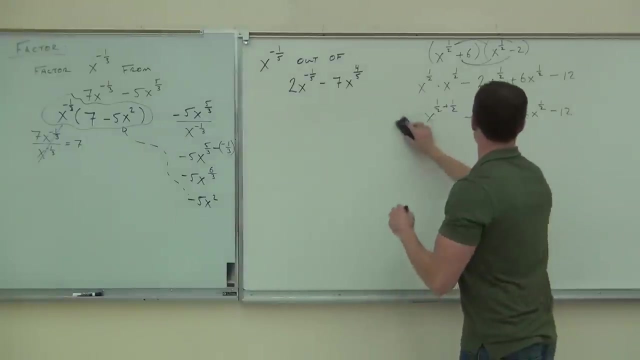 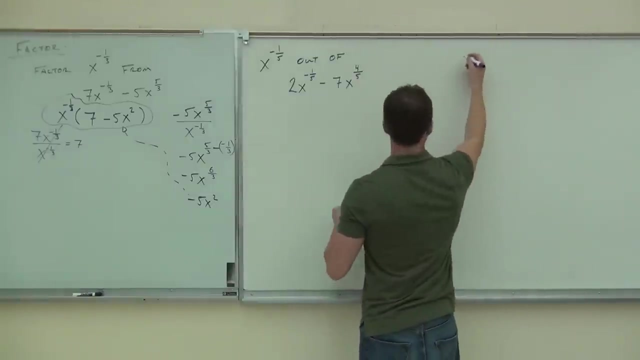 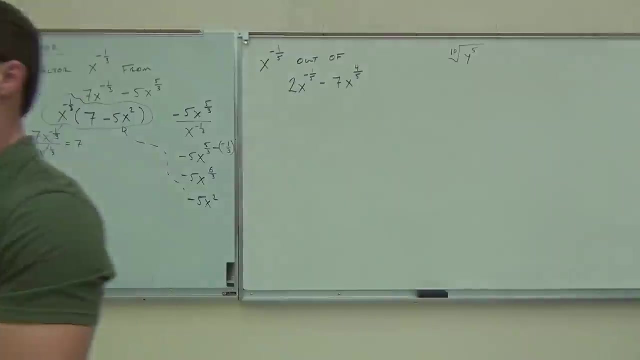 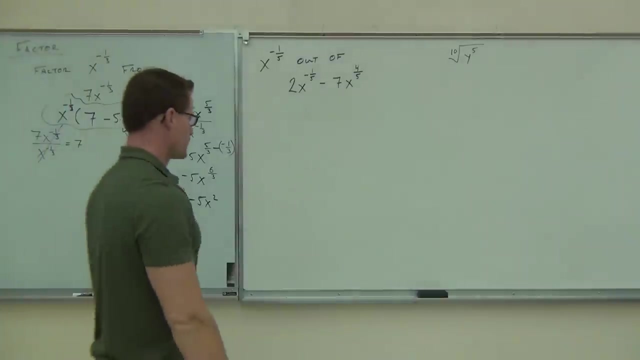 what I gave you next. That's what I meant. Once you get the hang of these, they go kind of quick. They really do. Once you really get the x1 rules, you know what they mean. We shouldn't be rushing through this stuff, but they're going to make more sense start. 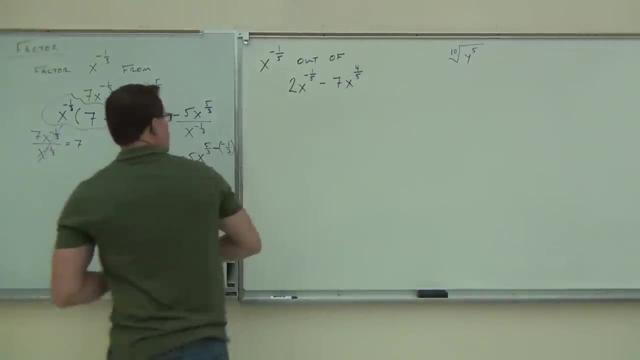 going faster through them. It's kind of nice. So we're going to factor. We're going to factor an x to the negative one-fifth out of this: 2x to the negative one-fifth minus 7x to the four-fifths. 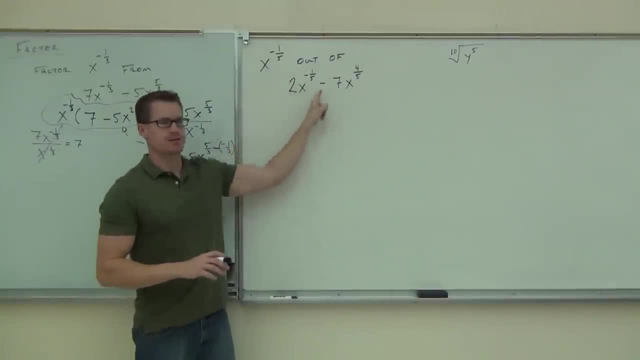 And I told you that most of the time, once you're factoring out, will be this expression right there, or will be one of them at least. So when we factor out, that means we're dividing term by term. So we're factoring out x to the negative. one-fifth, 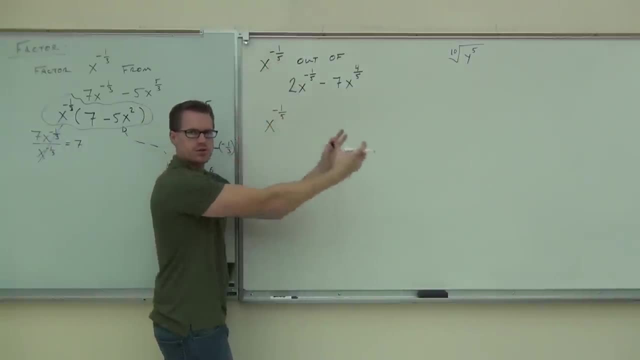 Whatever you're factoring out, whatever they tell you, that's going to go in front of your parentheses because that's what you're dividing out, so it's factoring On the inside. we get those two pieces of information, these two terms, by taking our 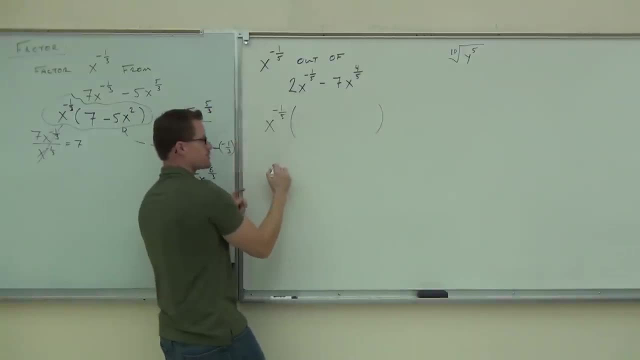 first term and our second term and dividing by what we're factoring. So in other words 2x to the negative one-fifth over factoring x to the negative one-fifth, And also we're going to have negative 7x to the four-fifths over x to the negative one-fifth. 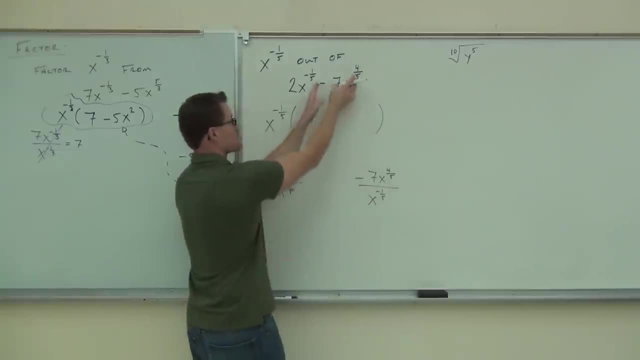 Second term divided by what we're factoring. Did you guys show that on the paper? That's good, all right. Now something special happens here. The reason why we're going to cross these out is because, when you think about it, we 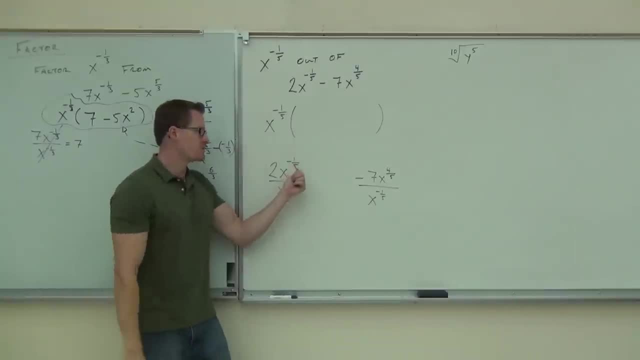 are actually subtracting exponents. But when you subtract exponents you have x to the negative, one-fifth minus negative. one-fifth Negative, one-fifth minus negative. one-fifth gives you zero. X to the zero is one, so this is basically set to two times one. 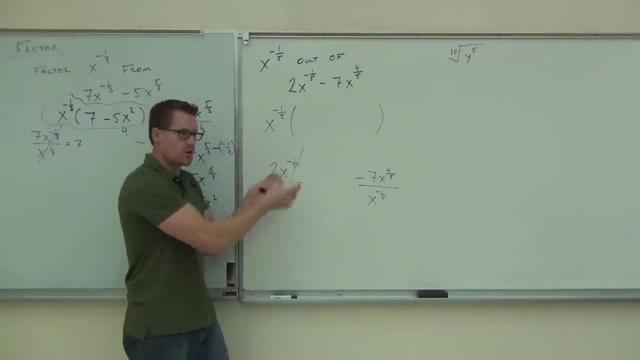 So this is well, that's gone too far. It's gone Just like it works any other exponent. you cross those out because you know those exponents match up And we subtract something that matches up exactly, you get zero. So there's no more x's. 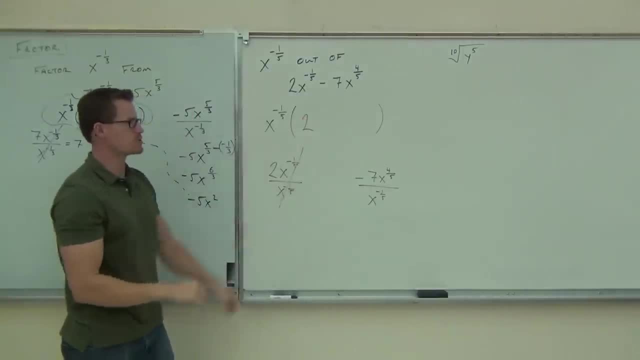 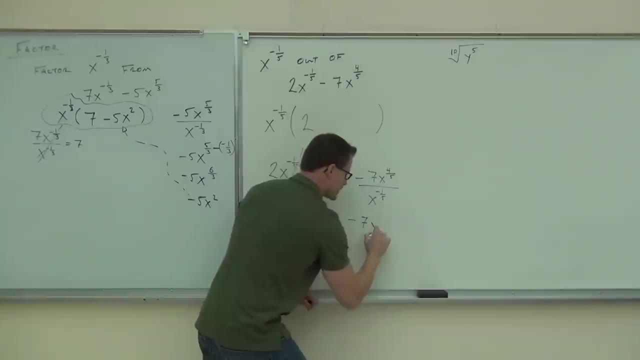 It's one, So we add just a two out of that because we have the coefficient of two there. Now the other one's a different story. The other one says: well, I know I'm going to have a minus seven, I know I'm still going to have x because they're not matching up exactly, but I have the four-fifths. 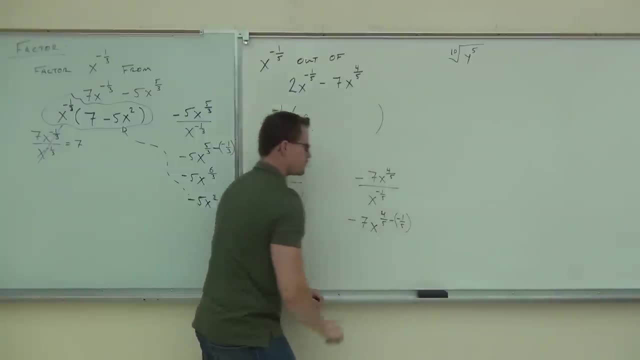 minus negative one-fifth. Four-fifths minus negative one-fifth- I'm subtracting this x one, since we're dividing common bases. Now, when we think about it, four-fifths minus negative one-fifth minus a negative, that's. 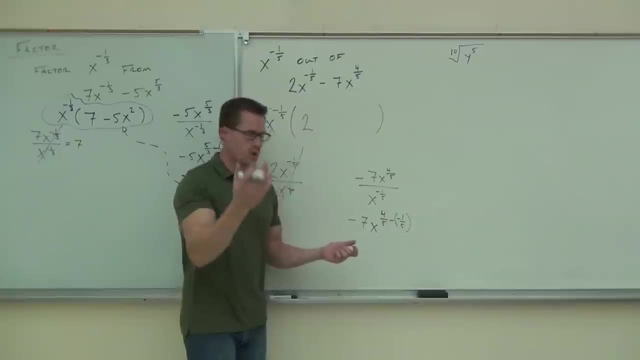 still addition. We're going to get how much? Five-fifths? One, Okay, Five-fifths. or we're going to get One, One, Yeah, exactly Negative seven x to the first power Five-fifths. 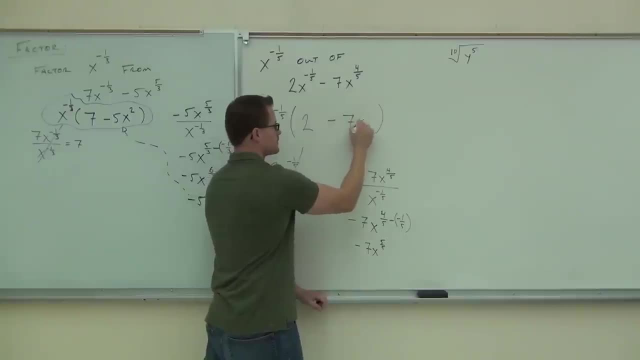 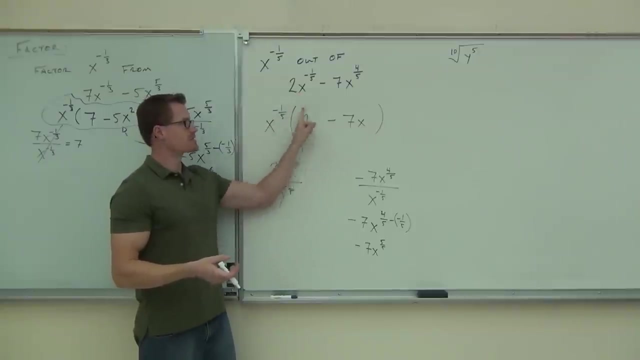 It's going to be seven minus seven x. If you want to check the distribution, you can do it. Look at it: Two x to the negative, one-fifth, That's that Minus seven x to the. That's that. 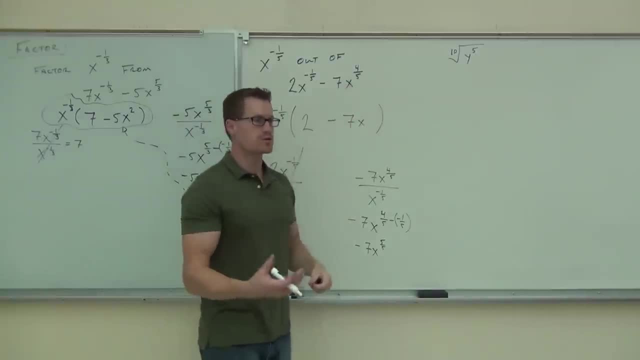 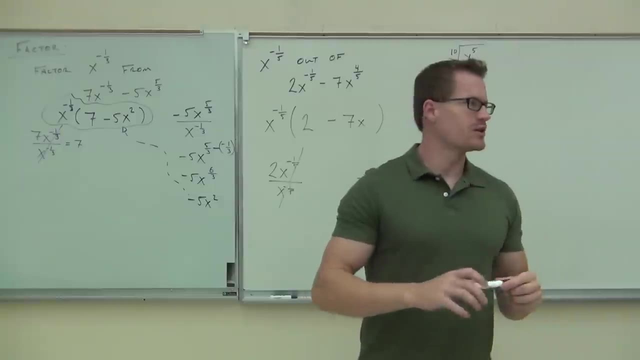 This is five-fifths minus one-fifth, That's four-fifths. So it still works with the whole distribution checking thing, Deleting Very mathematical. Yeah, How many people understood what we talked about so far? Good Patricia, you had a question. 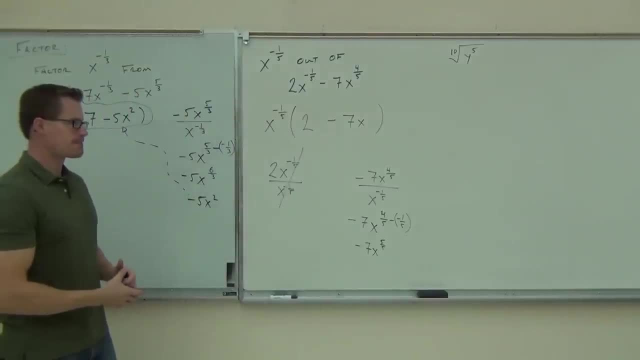 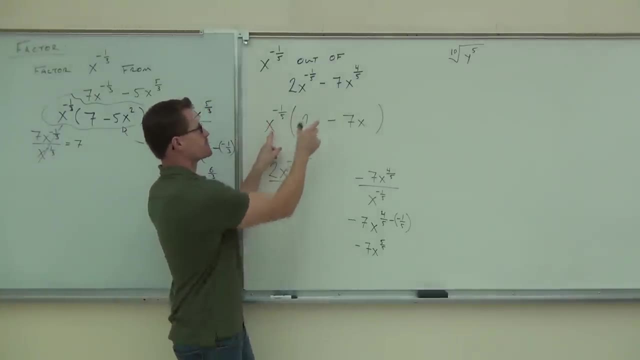 Yeah, I got negative one, So you always have to put the one from the inside first. Yeah, Otherwise you're dividing this by this. We don't want to do that. We're dividing this by this. Okay, So this one has to go on the denominator every time. 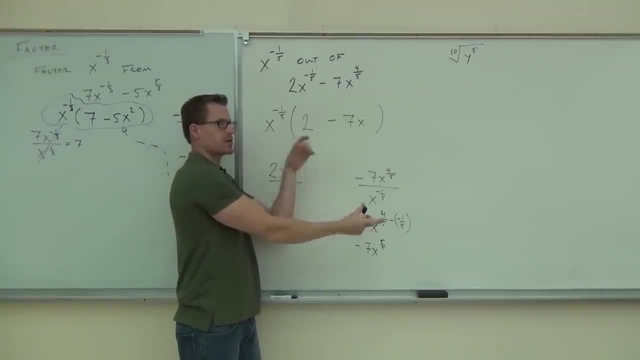 Otherwise you will get the opposite sign on your exponents every time. Okay, Good question. Thank you for that one. Any other questions? before we move on, I want to first remember on something. Do you guys remember how to take a root and write that as a fraction? 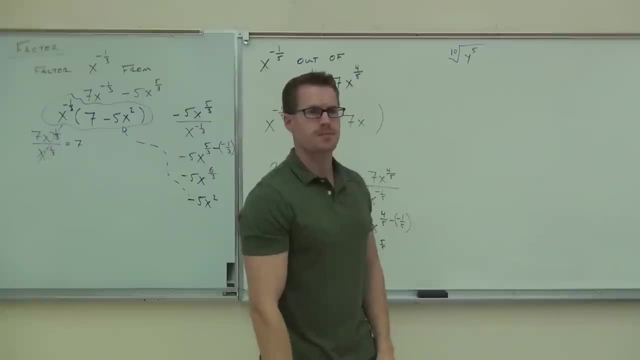 Yes, Okay, We're going to be. does the y change? No, But instead of just having a root around that, I should have some sort of an exponent. It should be. is it 10 over 5 or 5 over 10?? 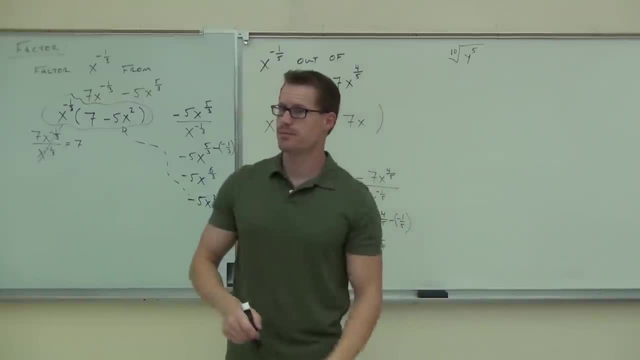 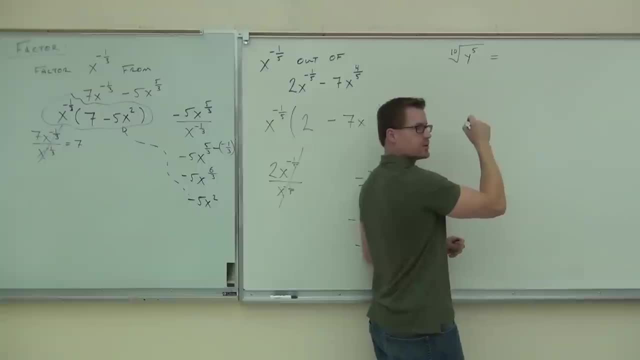 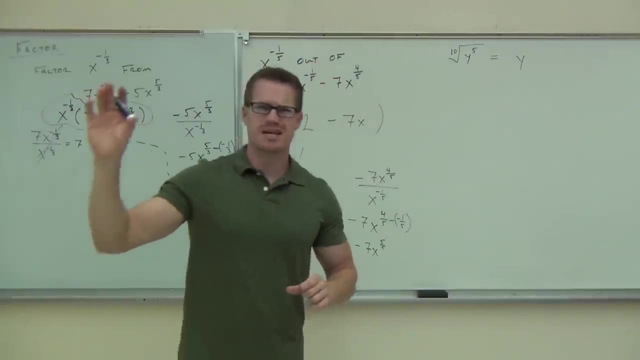 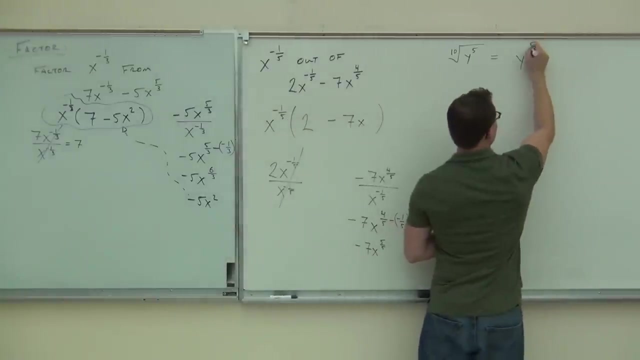 It should be 10 over 5 or 5 over 10.. We're going to do, because we do the power over the root, So we're going to do 5 tenths. Now can you simplify 5 tenths? 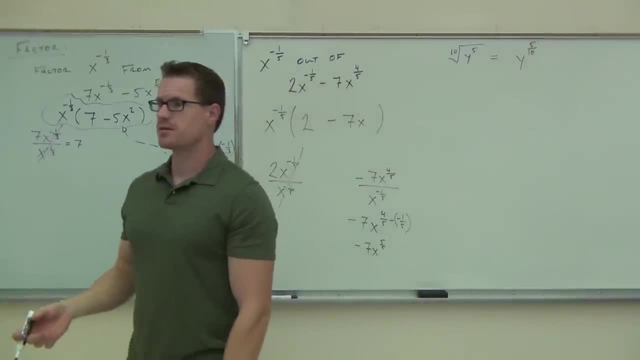 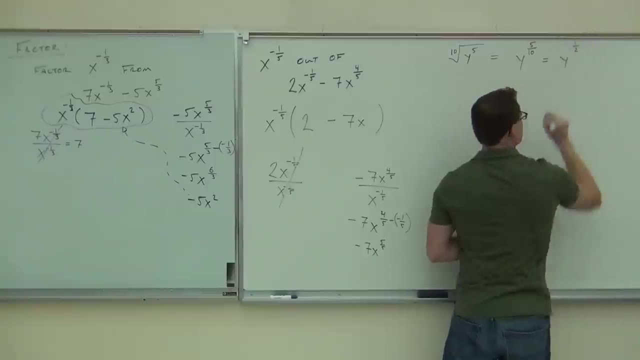 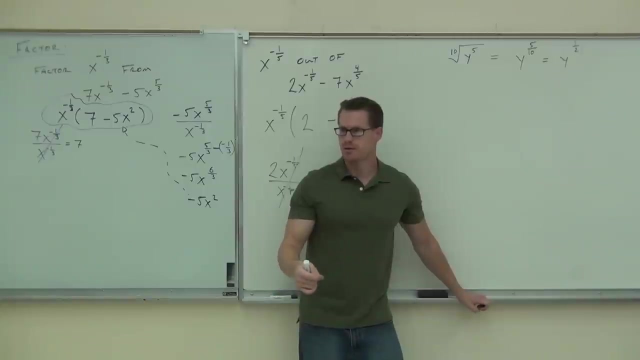 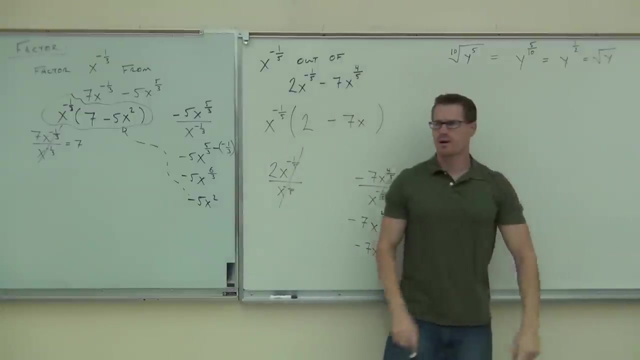 Yes, How much is 5 tenths 1 half? Can you write one half back as a root? What type of root is it? Square root of y, Of y to what power One? Well, that's weird. What this means is the tenth root of y to the fifth actually equals square root of y. 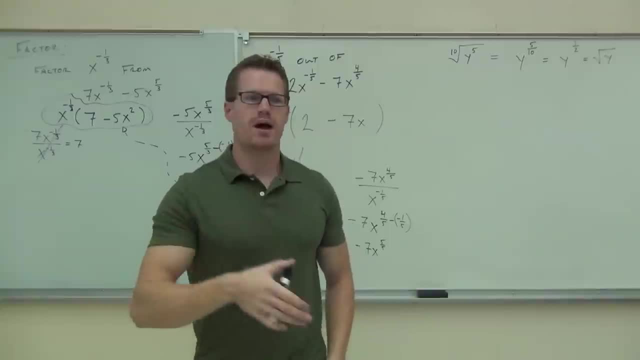 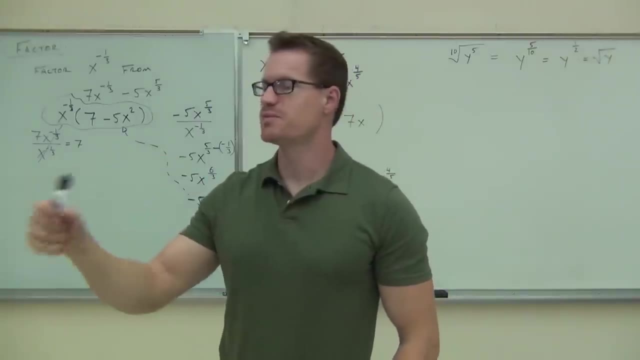 That's kind of cool, right. This is one way that you can use fractional exponents to simplify roots. You take your root, you write it as a fraction, you simplify those fractions, because that's how we know how to simplify, right. 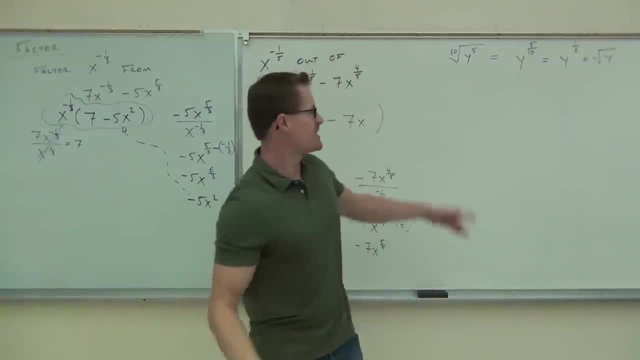 It's fractions. You write them back as a root. It makes things a lot easier to do. Isn't that easier to deal with? Doesn't that look a lot better than that one? It's kind of cool, right? We just did that just by manipulating some of these roots. 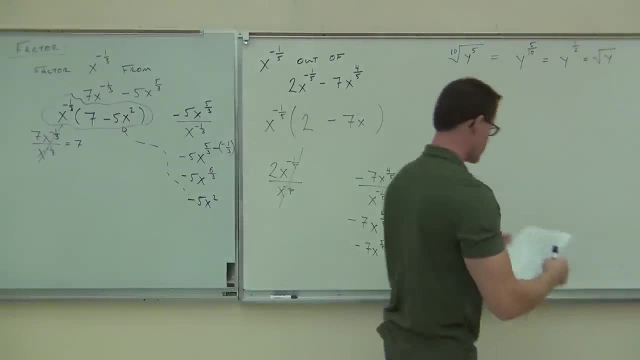 Let's try this with one more Now. does this work all the time? No, No, not all the time. I mean, if you had like seven in here, that wouldn't work. you'd have y to the seventh tenths. 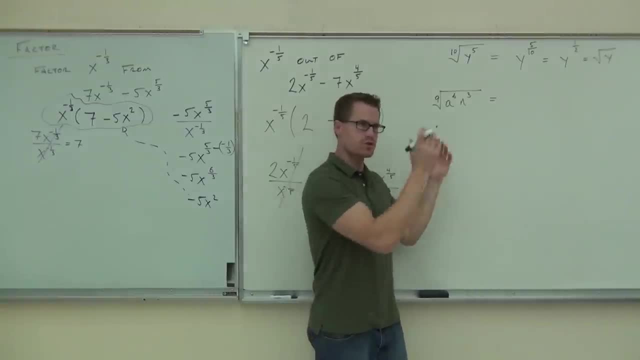 You can't simplify that. However, if you can write it as a fraction that is simplifiable, then of course you can simplify that. Can you write this: Oh, that's a mess of garbage, isn't it? Can you write this as something to a fractional exponent? 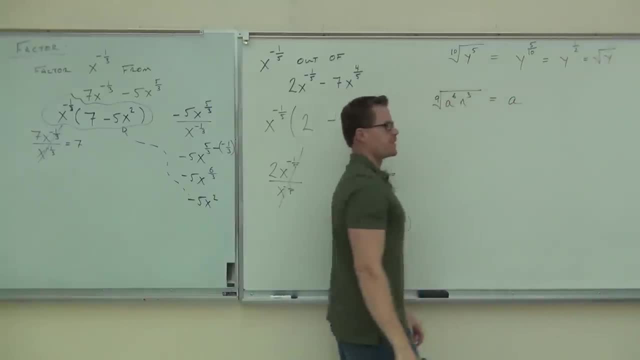 Let's try it. What do you think I'm going to write a to? A to what power? So what we've just identified is that when I have a root, I'm going to have a fraction. So what do you think I'm going to write a to? 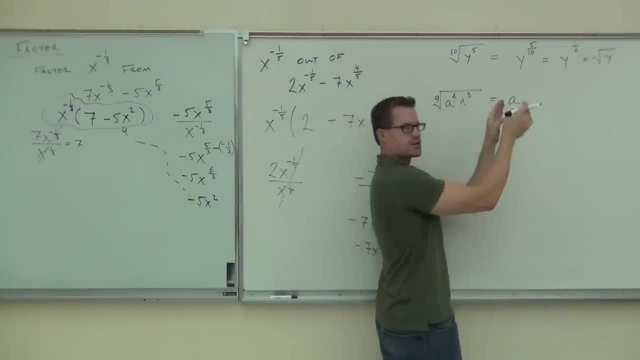 A to what power, 6. A to what power- 6. 6.. You've got a root and some powers in here. It goes through both of them. That's actually one of your exponent rules, Since these things are exponents. 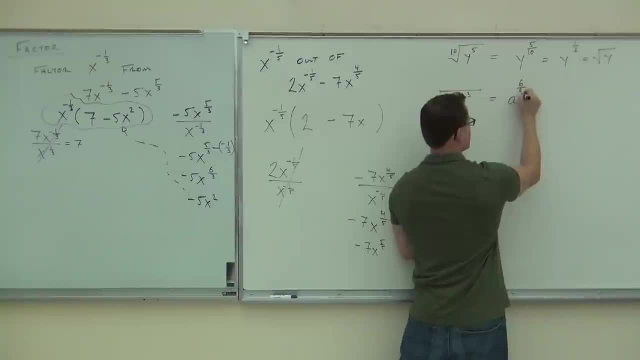 That's an exponent. These are exponents. It goes through both those exponents: A to the 6 ninths, You're right, And then N to the- what do you think? 3 ninths, 3. 3.. 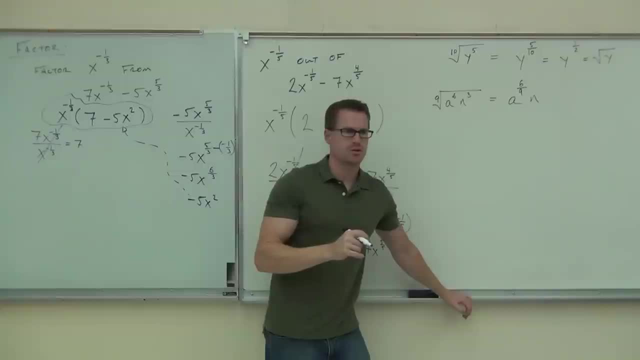 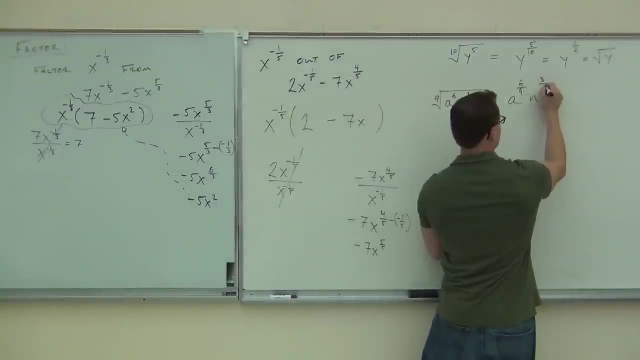 Are you seeing how to get the 6 ninths and the 3 ninths? Are you sure? Yes, So we have the power over root. We have power over root And we're going to do power over root. For example, 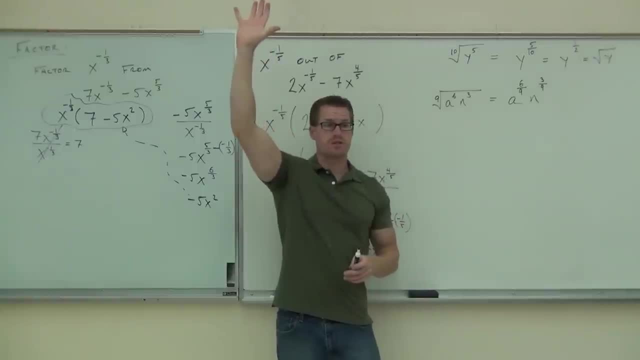 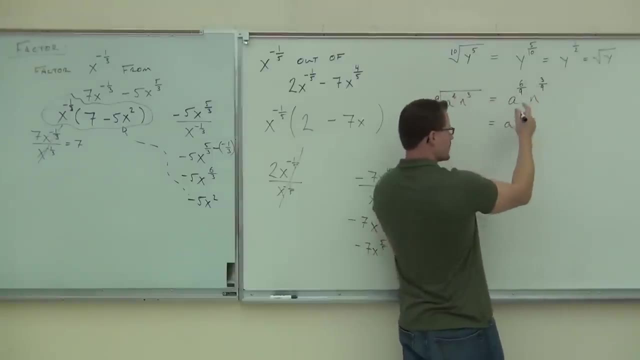 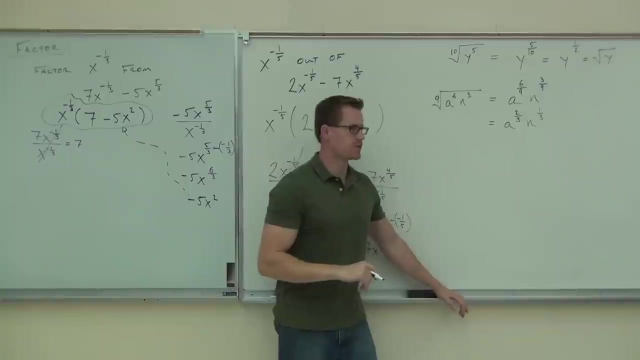 The root. What Do you feel? okay with that so far? Can you simplify those fractions? Yes, Yes, Sweet Yeah. three goes in. all that stuff So far, so good. Yeah, Now can you write that back as a root? 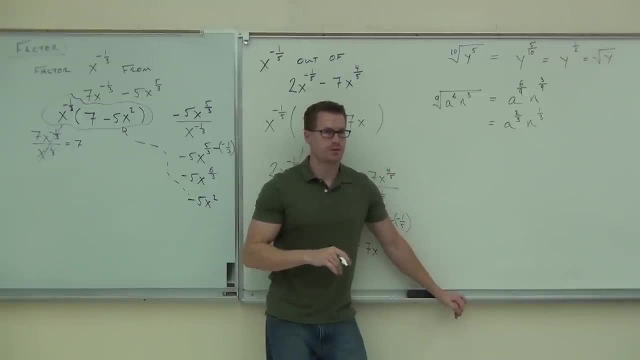 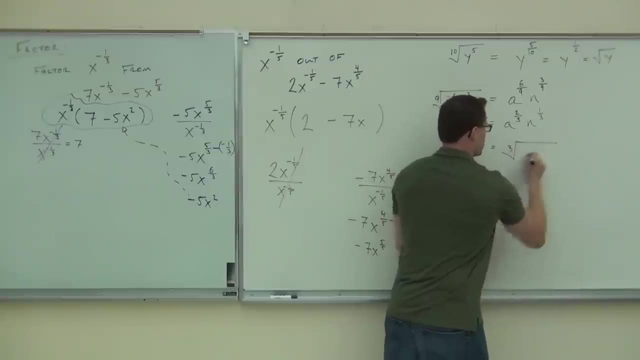 Third root. Third, why a third root? Because that's Okay, the denominators are three. That means that we're going to certainly have a cube root. A to what power, ladies and gentlemen? Square root And n to what power? 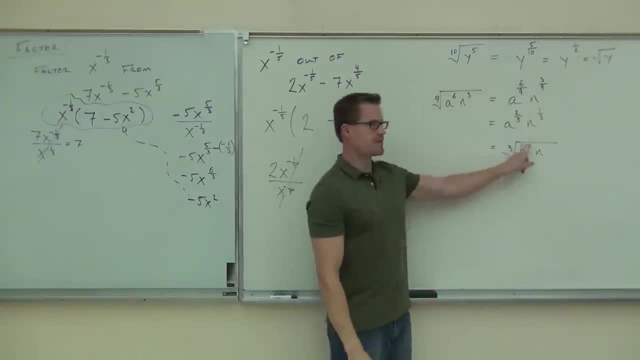 First, Does this represent that? okay for you? Then we're done. Now one thing that could potentially happen: what if one of these is simplifiable and one of them is not? Then could you write that back as one root. You'd have to make sure you have the same denominator. 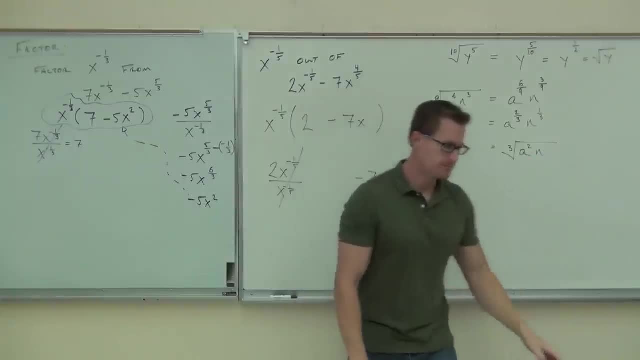 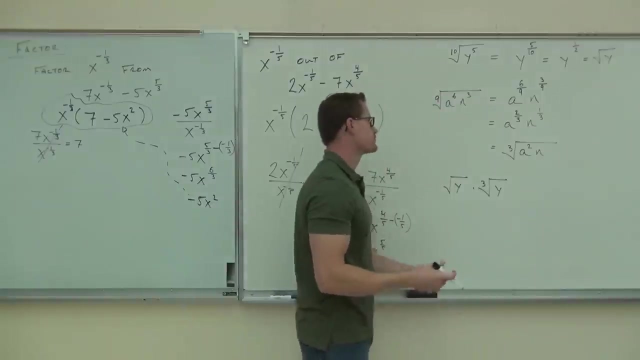 if you're going to write that back as one root. One last thing that we can't, we can't do: How would you write it out for the final answer if, instead of getting both the up there on the bottom, one had like a 9th or something? 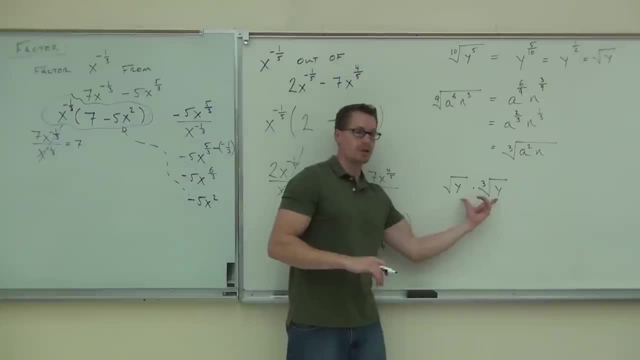 Would you have to have two square roots? Yeah, you'd have to have two different roots, You'd have to have. it'd actually look a lot like this: Oh, okay, Okay. However, I can show you kind of what to do with this. 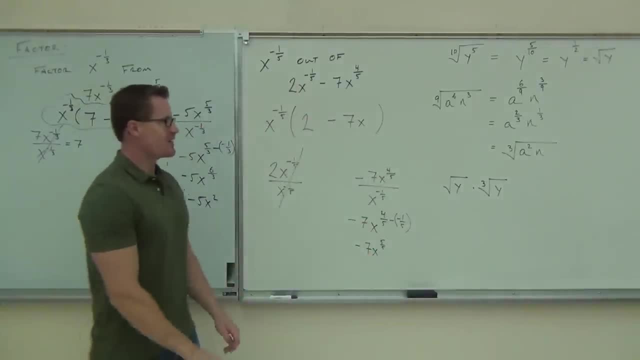 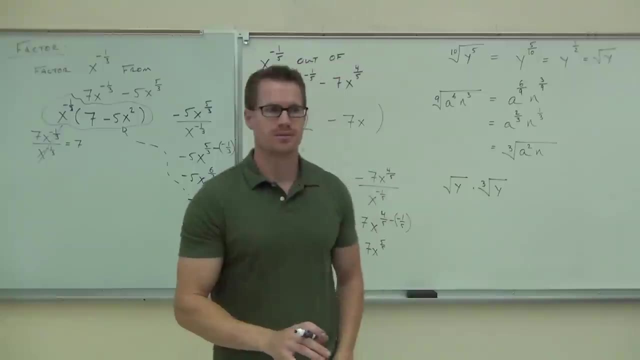 Okay, Which I'm going to do. We have a square root of y times a cube root of y. Is there any way that we can write this as one root? I don't know, In order to see that maybe we're going to translate this. 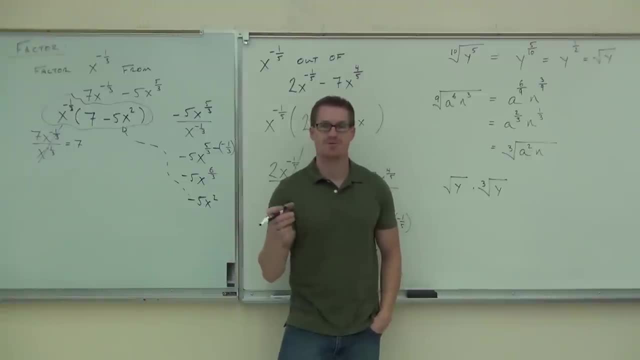 into some fractions, because we know that fractions are, ironically, a lot easier to deal with than these roots in our head, because we're familiar with fractions at least. So let's go ahead and let's write square root of y and a cube root of y as some fractional exponents. 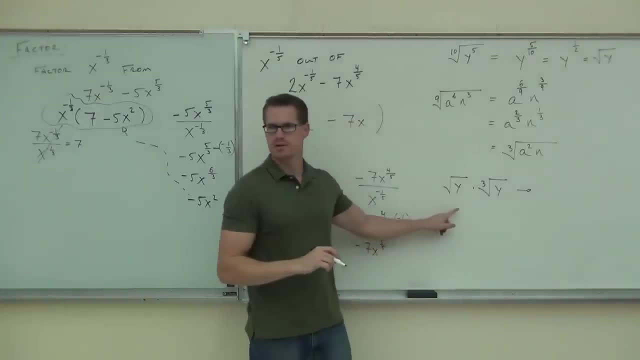 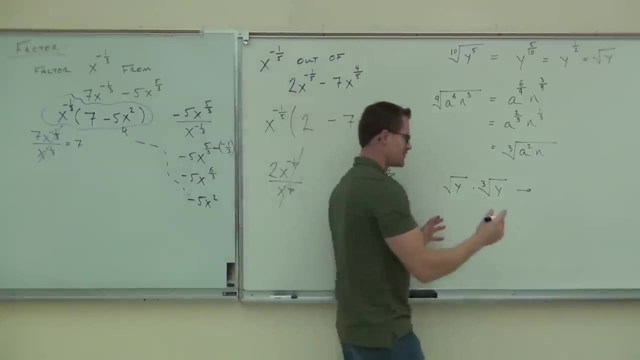 Everybody in here. what's the first one Y to what power? please, That wasn't even close to everybody. Oh my gosh, We're tired. Come on now, folks. Why do we have one half times? we have times, so times. 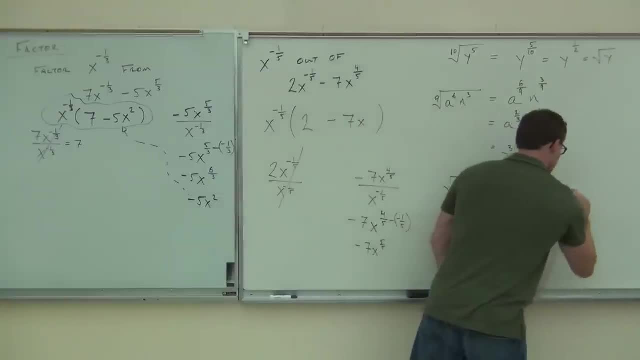 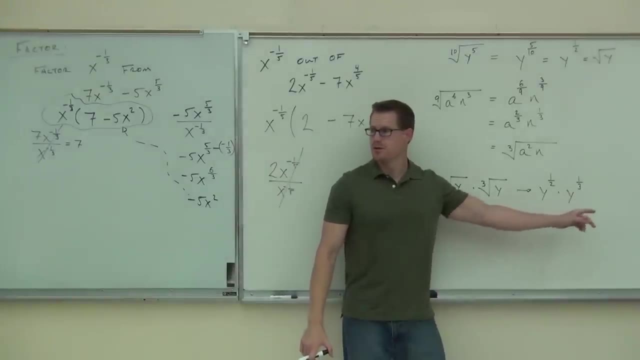 Y to what power for the next one? One third. Okay, that's better. Hey, hey, can you combine those? You have common bases. you have exponents. add the direct one by the byte, Add them, We add them. yeah, just like we did over, not over there. 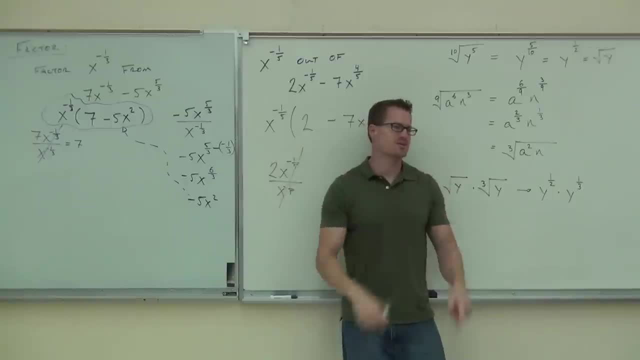 Previous example: redistributed. You add those exponents. So if we add these exponents, what's one half plus one third? Can you do one half plus one third? Well, not the way it is, but maybe find a common denominator. 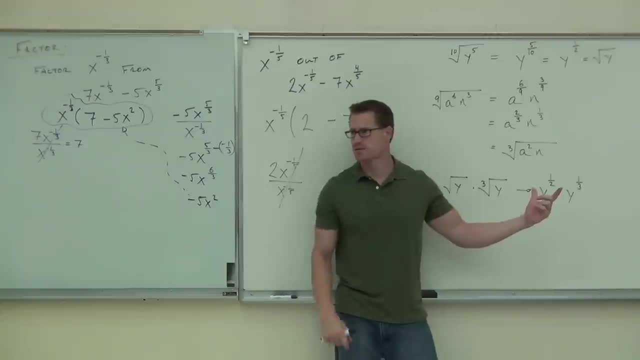 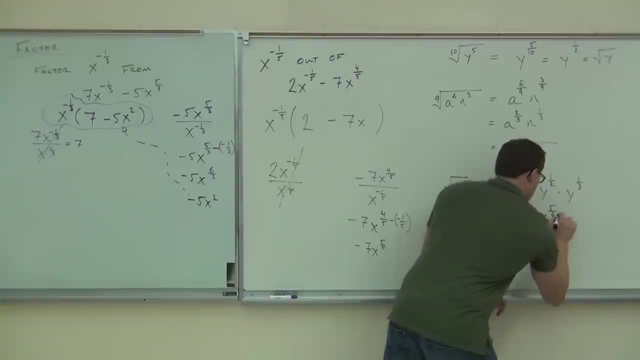 You can do one half plus one third. Do it in your calculator if you'd like. Five-sixths, Five-sixths. You got five-sixths, Y to the five-sixths. Can you take y to the five-sixths and write it back as a root? 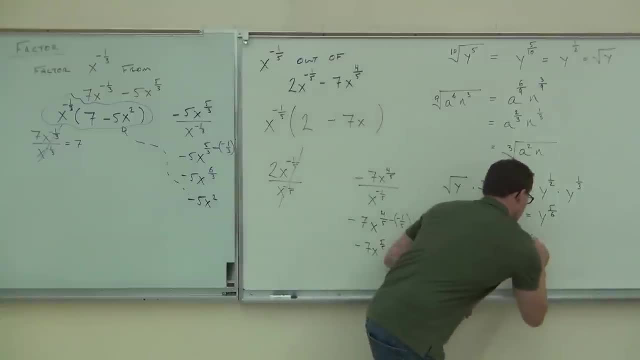 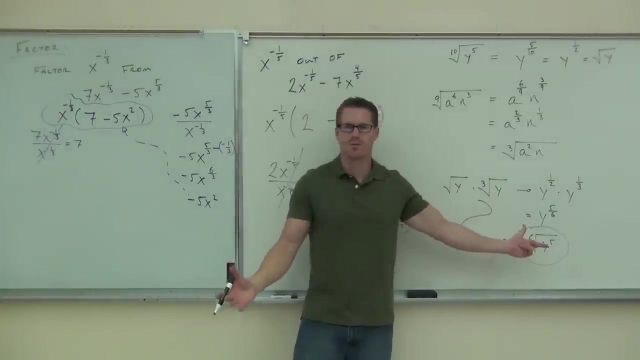 What type of root do I have? a fifth root or a sixth root? Sixth root: Y to the fifth. Here's what this says. this equals that You can take two roots and make it into one root. Now, what? how? one root. by the way, that was a lot in this class. 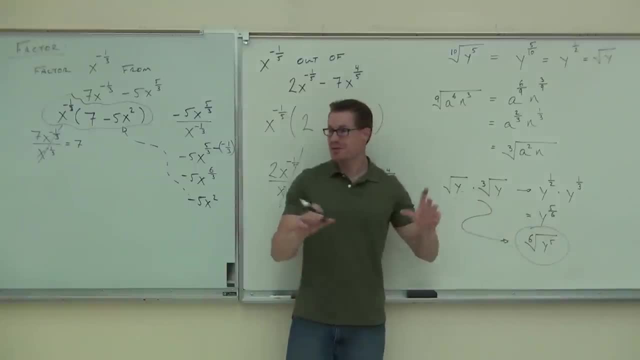 Okay, How do you? what's the whole process? When you think about it, these are fractions. If you have a look at the board, if you have a different root, what you have is a different denominator. So the process of combining roots is the same process. 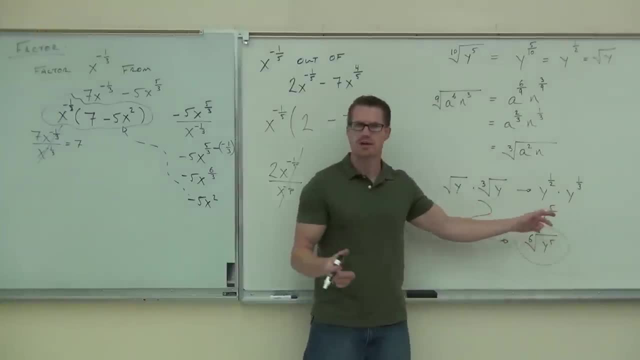 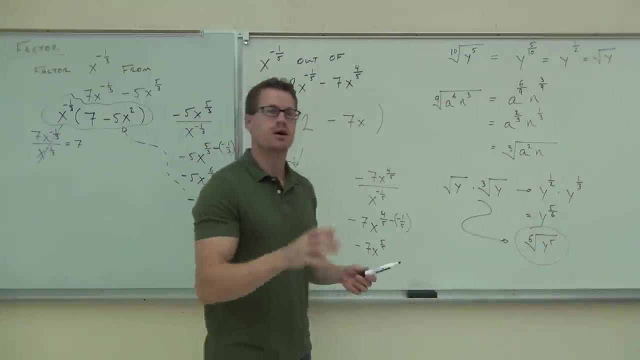 as finding a common denominator. That's it. That's really all this is. You're finding a common root. That's the same thing as saying a common denominator. That's what you do when you combine those fractions. You make them into fractions. find a common denominator. 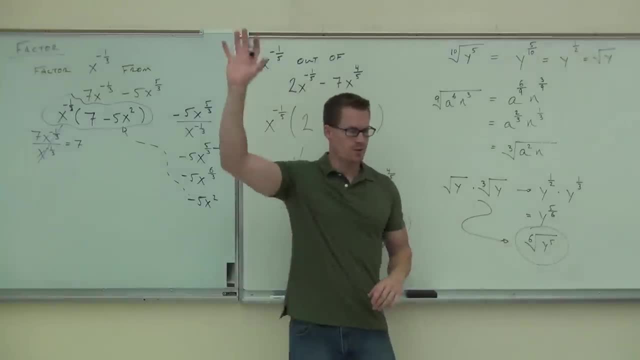 use that to add them together. it will give you a common root. Rich, do you have a feel okay about what we've talked about so far today? I got a quick question. Yeah, So, like you know, in the previous example, 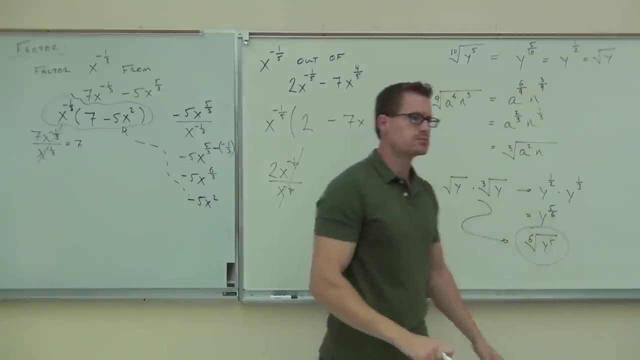 if you would have two square roots? would that be the second step to actually get your final answer? Yeah, Except what's going to happen is most likely in this case, you'd probably get this back again. That's what happens, or something that looks similar. 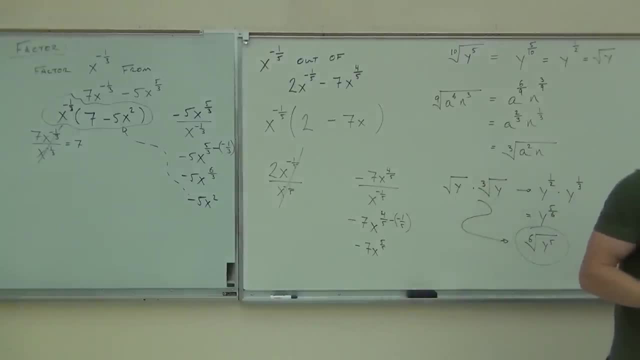 that may be reduced by a certain factor. Now, what we just did here, we kind of are simplifying these roots. We're going to take that another step. We're going to keep going on how to simplify this stuff. Are you ready? 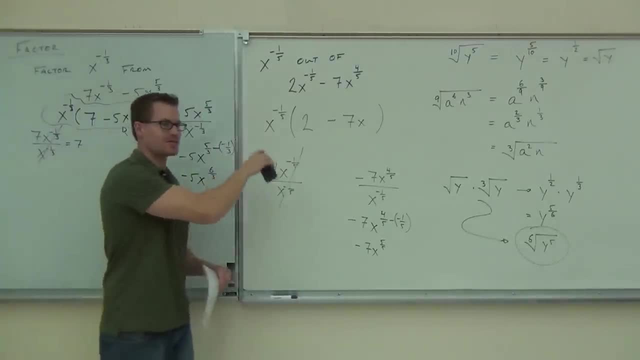 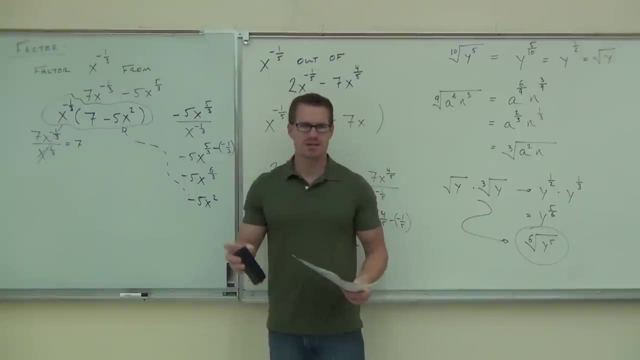 Did this all make sense to you? Good, Remember this stuff. You need to go back and look at this. A couple notes on how to simplify How to study for because I was talking to some students and no one ever really teaches you how to study for math. 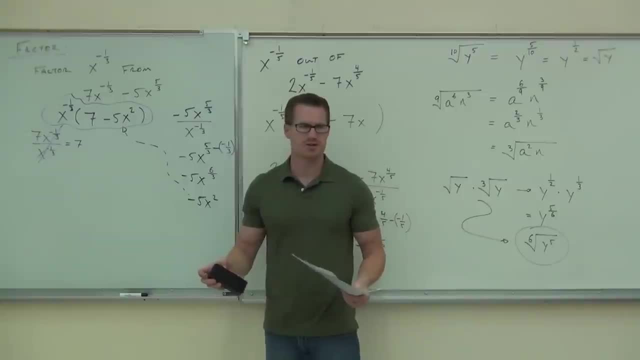 Right, You study for English, study for science, use flash cards and all that stuff. It doesn't really work all that well for math. Here's some ideas on how to study for math. First thing: studying has to be spiraled. 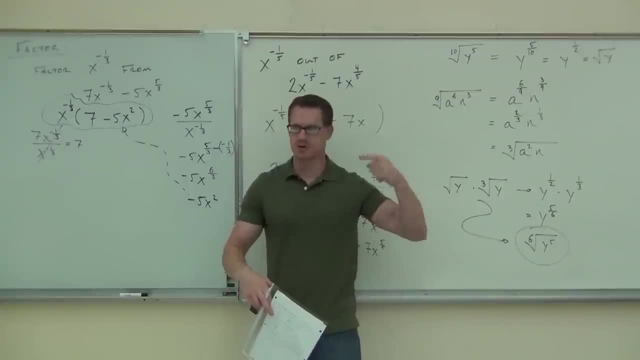 which means that you cannot just look at it once and have it perfectly in your head for the test. Math does build on itself, but we cover many, many different topics and different examples. So the week before your exam, the day before your test, what you should be doing is going back. 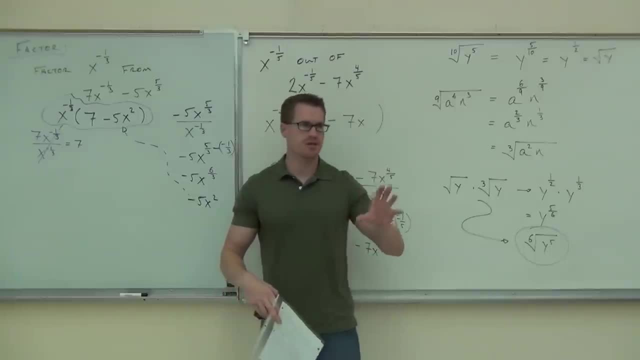 and reviewing the first section that we covered. Every day spend 15 to 20 minutes looking at the old stuff before you start the new stuff. Does that make sense to you? You have to do that because you will forget it. I guarantee it. 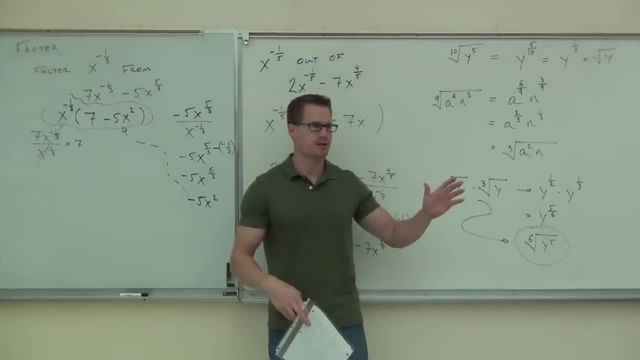 Even I forget this stuff. I forgot all about Math 4C, That's calculus. I forgot all about third-year calculus. I can't even do it anymore unless I really really look at it. all right, And that happens for you guys, because I know that stuff. 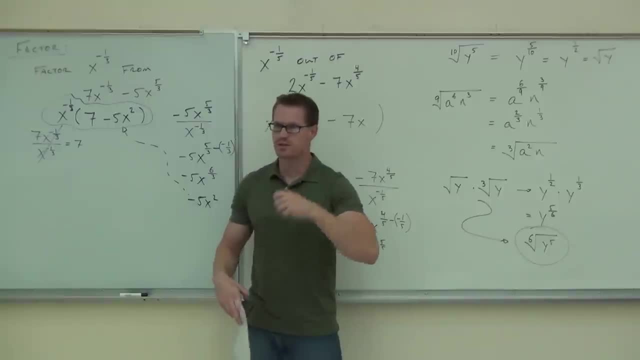 I know it very, very well. You guys are just learning this right. You need to spiral that information. Also, when you're studying for a math test, don't spend four hours studying the night before a test. It doesn't help you. 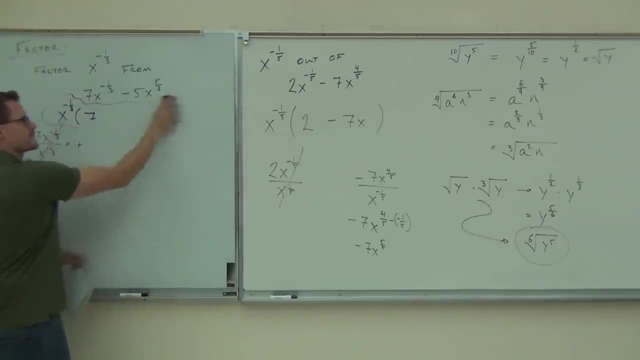 Instead what you should be doing. spend 30 to 40 minutes. Take a break. Your brain cannot absorb math for that length of time in a row, So study for a little while, Take a break, Come back and study some more for it. 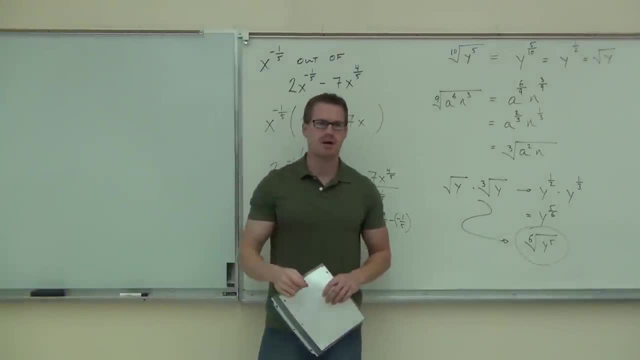 Also, you need to be practicing the stuff that I give you for your review. If I give you a review sheet, you need to know it's going to be very, very similar to your test. Practice those problems Also when you're doing your homework and the review sheet.